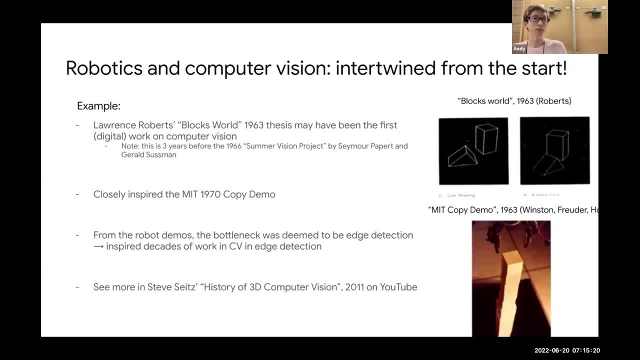 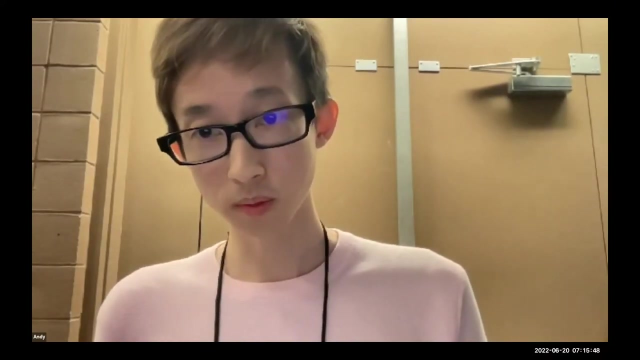 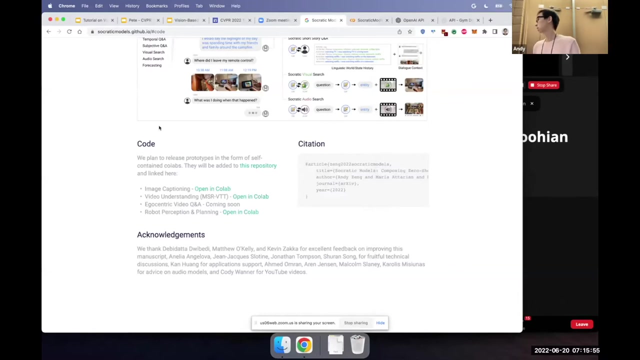 interactive, so if anybody has questions, you're running things on your laptop and something breaks, please feel free to you know, wave your hands and ask us to slow down or what not. You need to share the tab. Oh okay, Michael, can you see the screen? 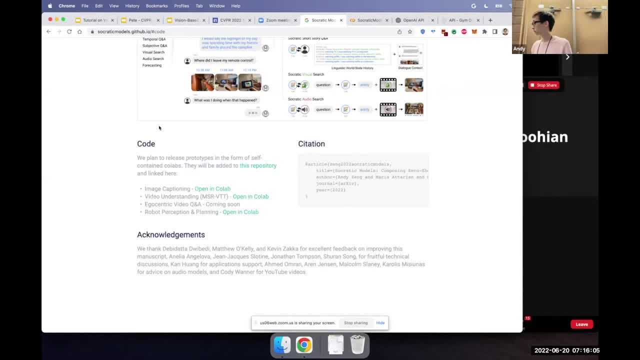 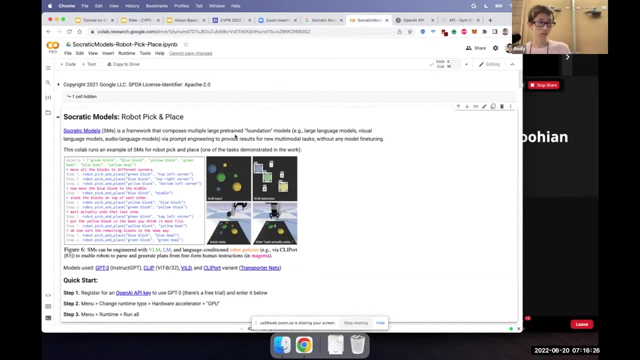 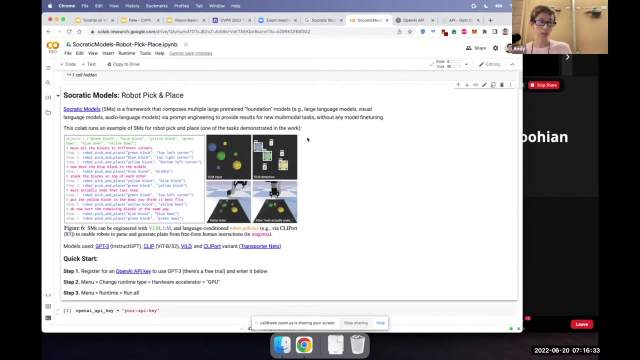 Okay, You can see that people. All right, yeah, so, Okay, cool, Yeah. so once you've got the links, then this is what it looks like. This is a copy that's running on my instance, but yeah, some of the headers here are just giving an intro to Socratic. 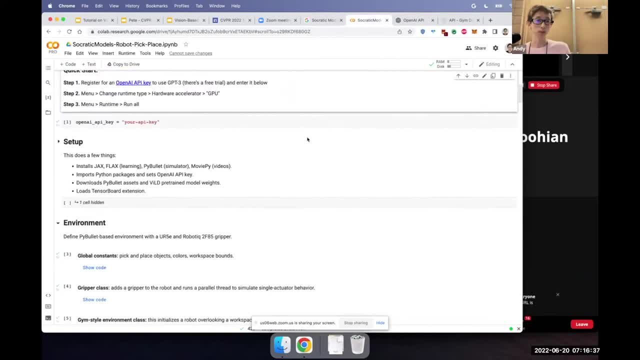 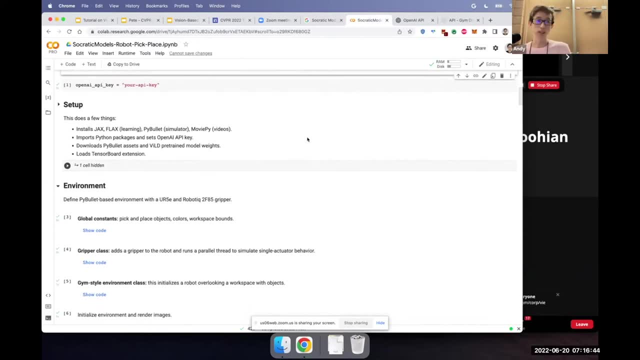 Models. but I think we'll get to that a little bit downstream. So the first thing to note here is that for the setup section it's going to install a bunch of things, Notably in this collab there's going to be a simulator, so that's PyBullet and that'll be running in the next couple of weeks. 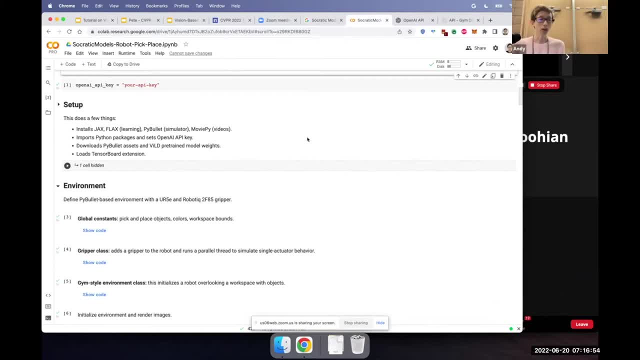 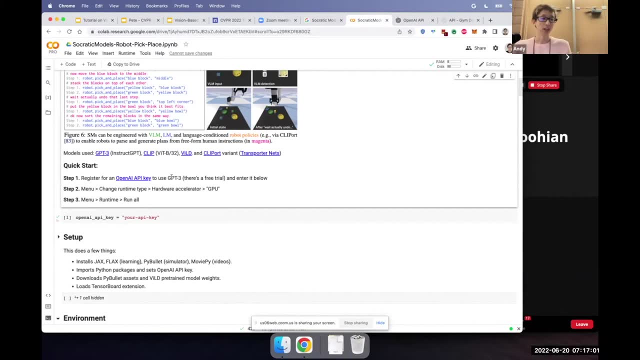 So it's going to be running in server side. Oh, and actually, before jumping into a list of packages, for those that just want to get something running already, there's three steps for the quick start. First, registering for an open AI key, a GPT-3 access When you register for an account there. 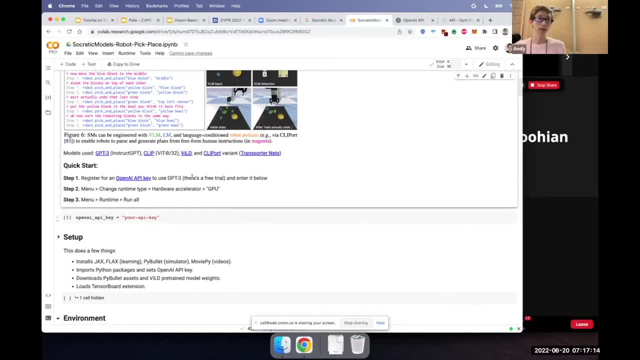 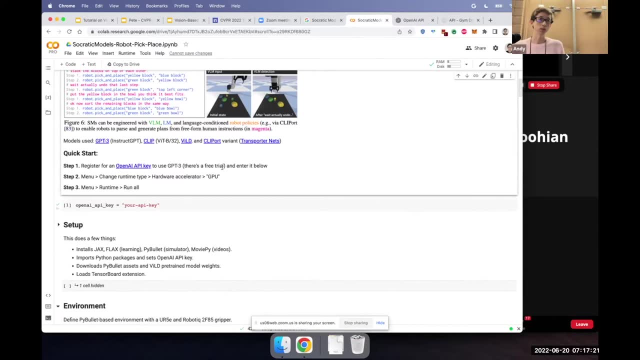 is a couple dollars that are free, so that's enough to run the demos that are in here, And really it's only needed for the very last step. but some of the sort of human to robot type interactions are fairly interesting, and as only possible because of this. 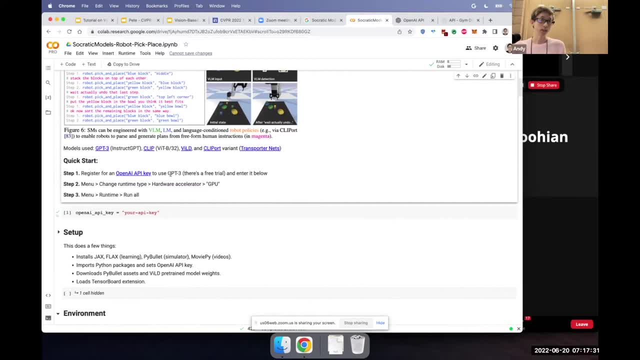 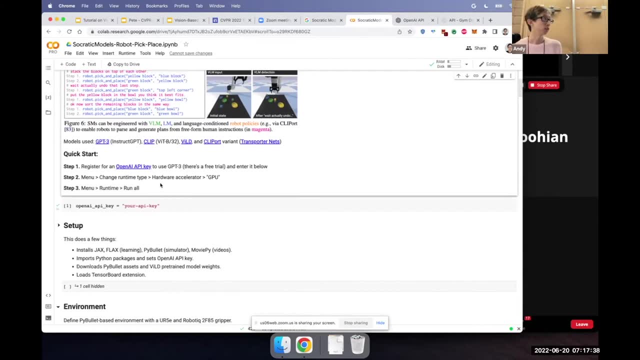 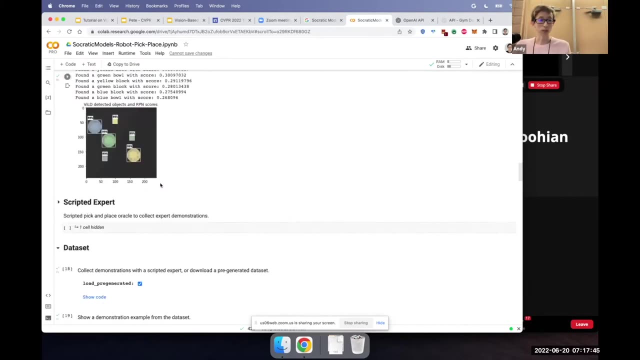 and so I definitely recommend- It's not strictly necessary, but I think it's definitely recommend- trying it out- Changing run type to GPU and then run all So the GPUs. this collab also has training code baked into it, so if you scroll all the way down, you'll start to see tensorboards and there is. 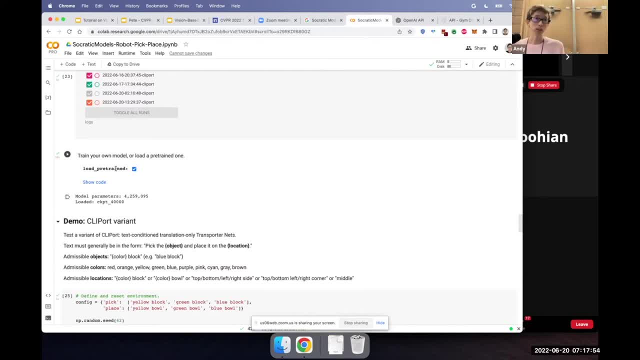 pre-trained. so if you just run all, it will download pre-trained weights and it'll use those. But if you wanted to train your own, you can also just untick that box and then run all. I think if you have you want to periodically check your. 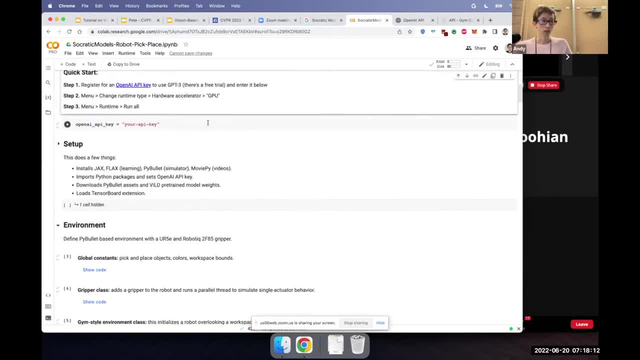 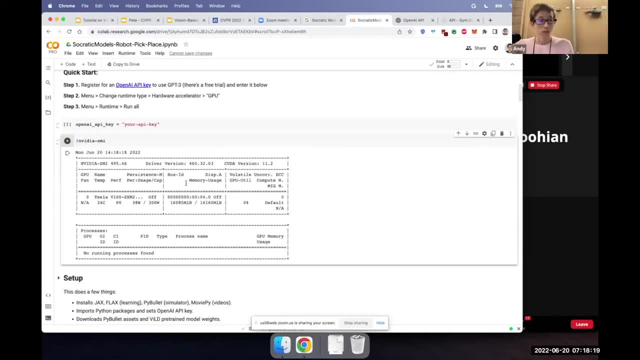 GPU. so if you want to do that- I'm sure some folks here know- but doing a NVIDIA SMI, So I have a v1.0.. But sometimes when you're connecting with public collab, you might have access to Tesla T5s, P100s. 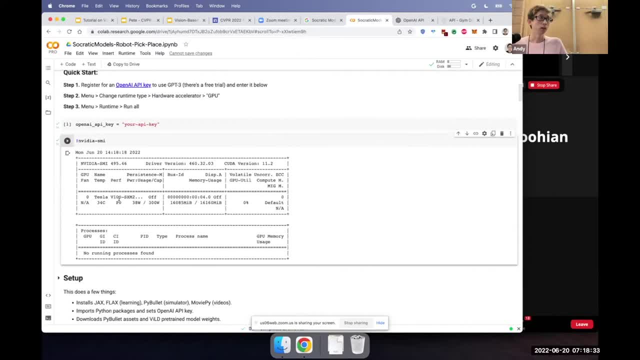 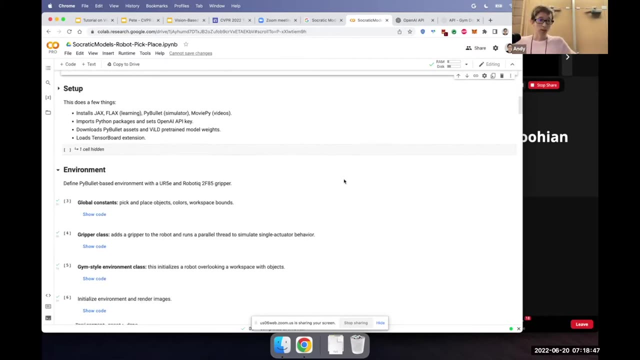 and in order to successfully train you want a P100 or above, I think for T5s. we tested it and sometimes it does have memory leaks, so just letting folks know. Okay, so in the setup we've got the simulator running. We also have several packages to kind of generate visualization. so that's what MoviePi is. 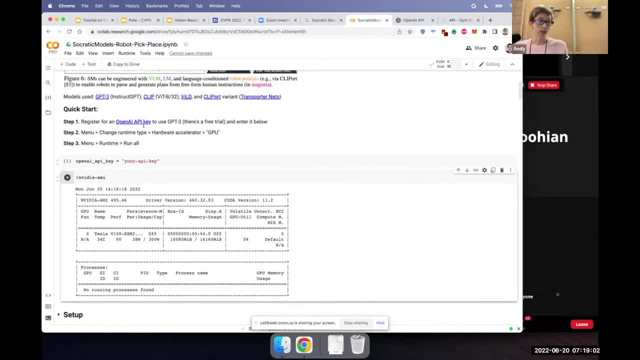 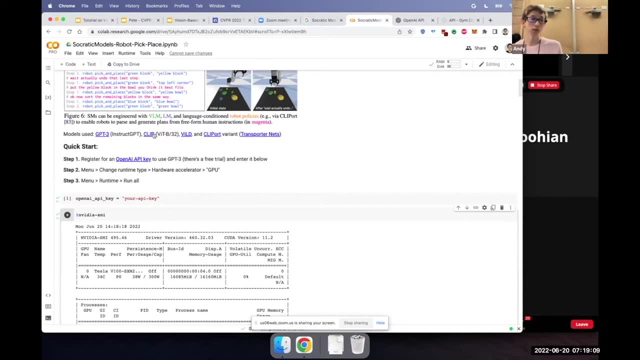 And we also have, notably, all of the packages that are needed to run several models, The first being GPT-3, the Instruct series. so that's DaVinci OO2.. VIT, V32 for Clip, and that's a precondition to the next two models, Vylde and Clipboard. 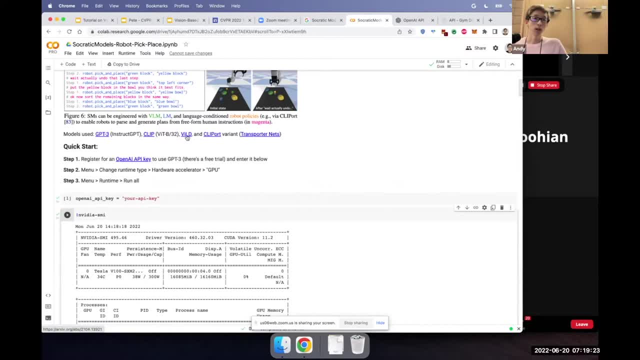 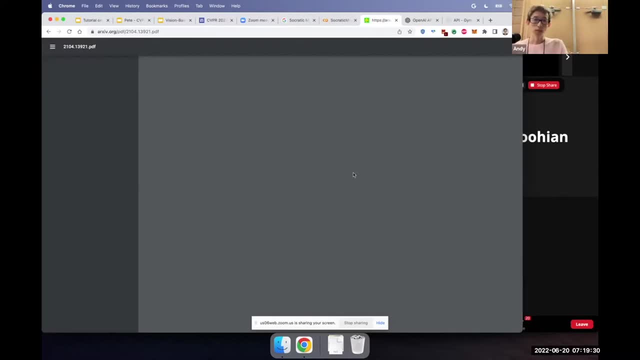 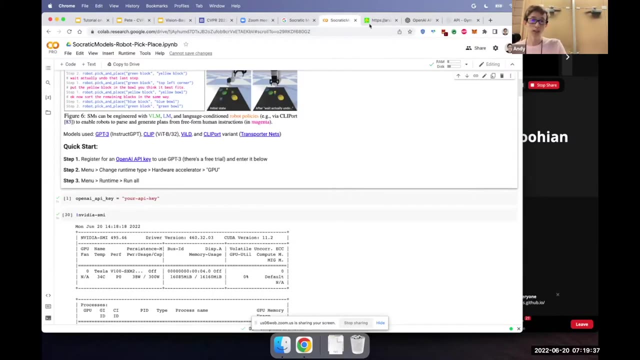 Vylde is a open vocabulary, object detector, so they've got some. if you read their paper, they have some pretty cool examples of that. Literally, you can feed in a list of strings and it'll start to detect objects. Okay, and Clipboard is a clip conditioned transporter nets, So transporter nets. 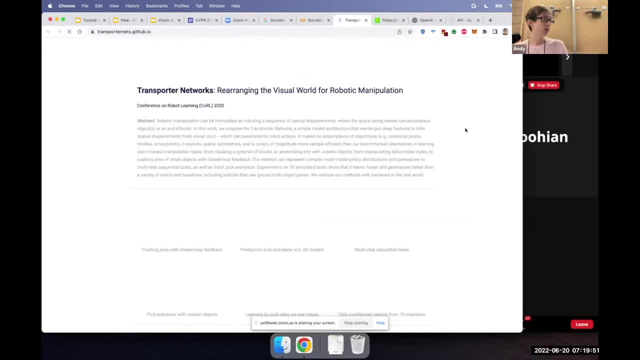 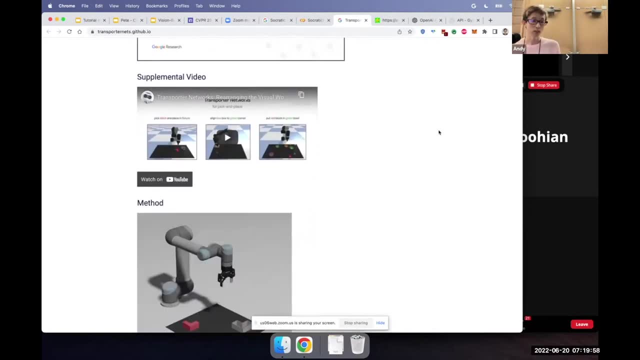 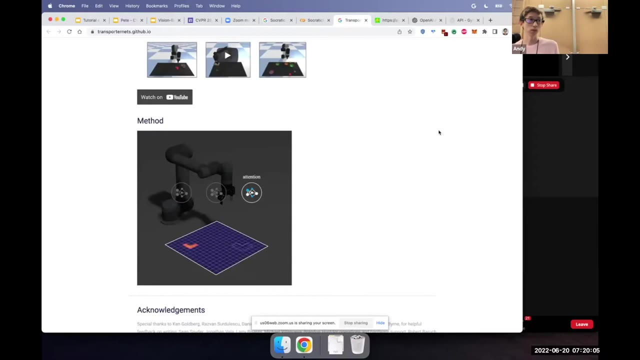 what that is is a framework for pick and place, and what it does is that it captures a top-down view of the scene and then uses a sliding window as a way to figure out how to reorganize. first of all, figure out where to grasp, and then, once it's grabbed something, it's going to construct a crop. 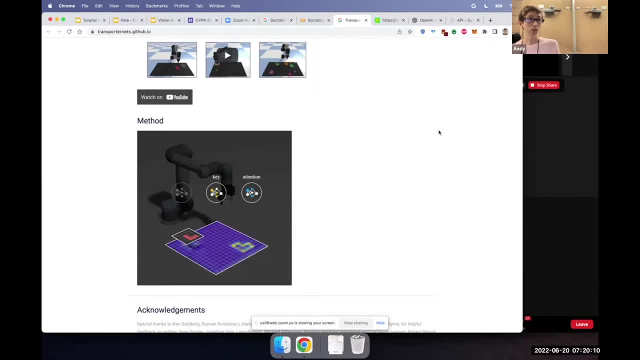 around the local region of the crop region, treat that as a crop and then slide it over the scene. So what this gives you is essentially a pick and face, pick and place framework from the top-down view to help you decide: okay, where's the place that you should put something? and this is: 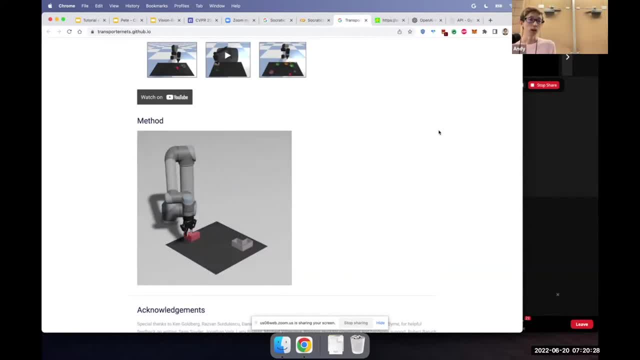 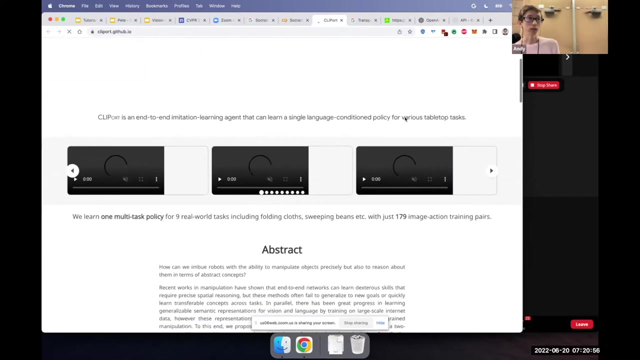 generally useful for robotics tasks like assembly but kit assembly or in all the other sorts of simplistic pick and place tasks, but all of this is trained from pixels to actions, and one thing that it lacks by itself is the ability to condition on language. So that's where Clipboard comes in, and what they do is they show that you can. 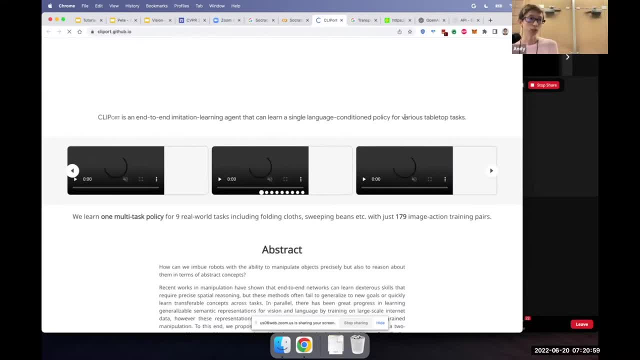 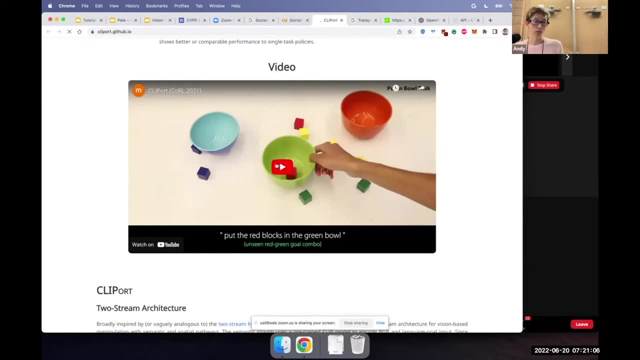 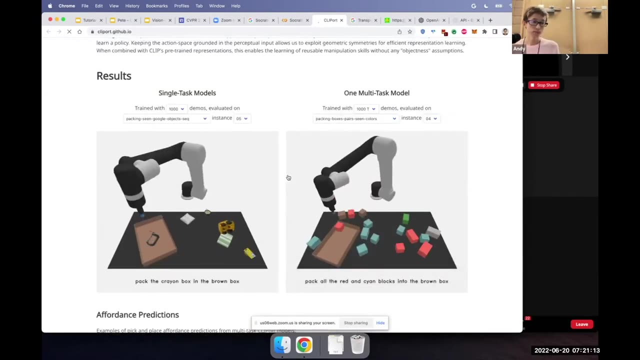 condition this model on clip text features and so you can end up doing some pretty awesome demos where you're sort of asking the system to put the red blocks in the green bowl and sort of pack objects and sort things here and there. so it's very cool to see some of this stuff, So how these models kind of interact with each other. 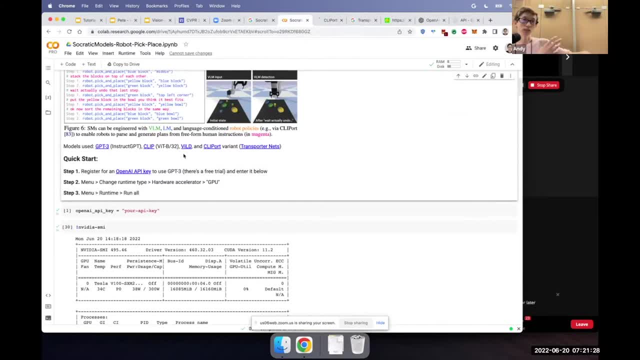 is that you have something like GPT-3 processing human commands and turning it into a list of steps, and then it's only able to do this in context if it has, for example, a scene description and that's being generated by Viald. Once it breaks down the steps, then it sends each of those steps. 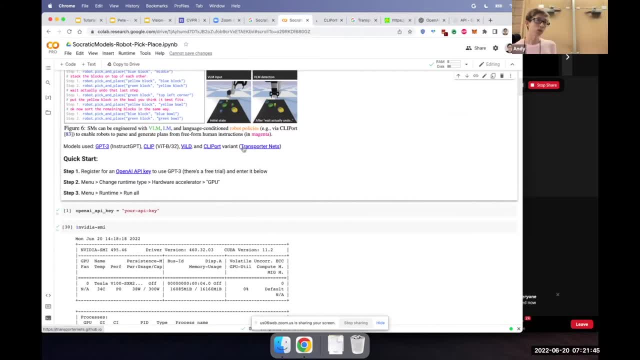 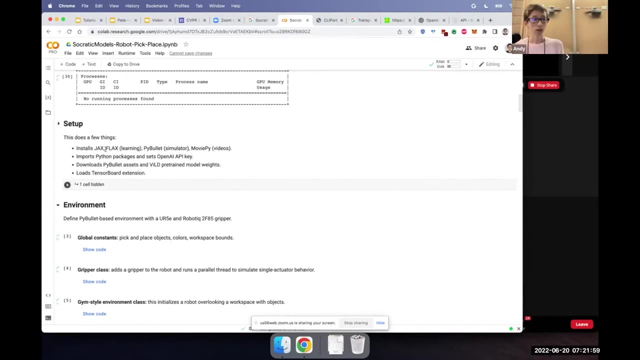 into Clipboard, which, since Clipboard can only do sort of one pick and place at a time, GPT-3 enables you to break it down into those individual steps and then you can run Transformers. So the JAX and the FLAX here for the learning side, what you're training is just mostly the 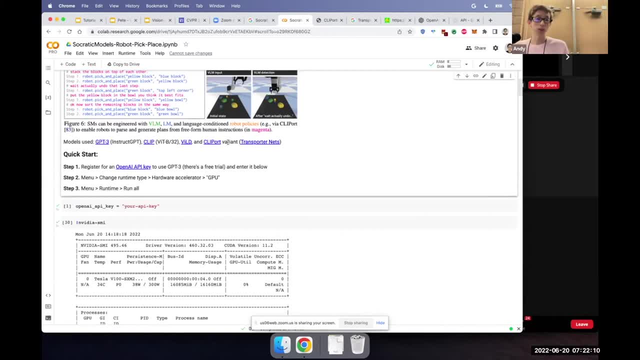 Clipboard, and this is needed in the simulation world because at least in that domain, some of these models do need a fair bit of fine tuning. It's pretty key right. so that's one of them. just to get a bit more clear about 있는 batteries, on how to practice Clipboard and then when we follow them. 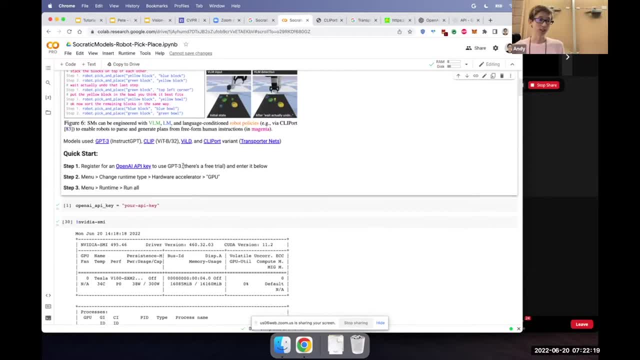 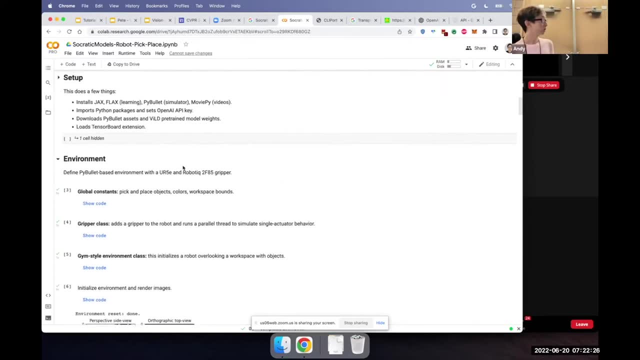 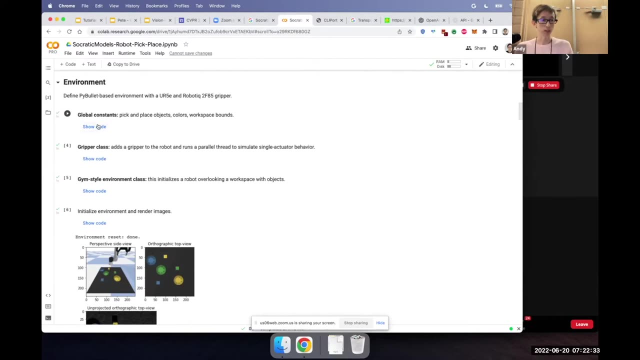 Some of these models do need a fair bit of fine-tuning to cover the real system gap. Cool. So, following the setup, the environment code is here and I'll quickly go over some of the things that you might see Here. there's global constants and these are defining the set of. 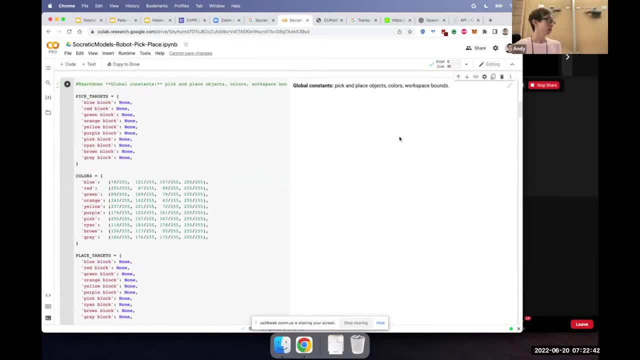 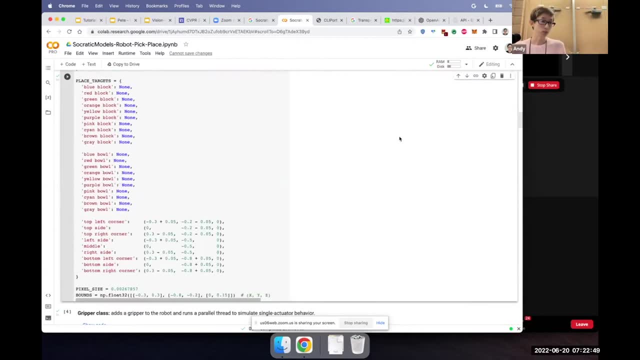 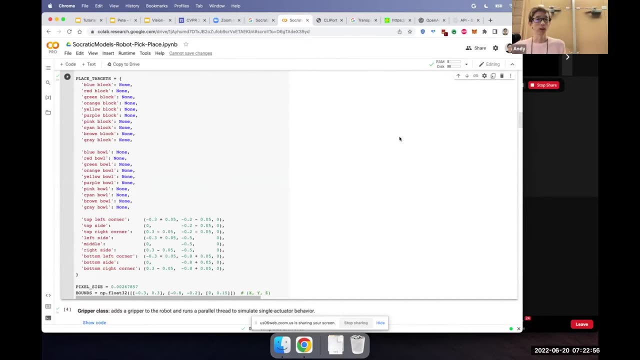 objects that you would see inside the environment. In this constrained colab at least, there's only blocks and bowls potential some definitions for spatial locations, which is useful for your scripted demonstrator, which we'll talk about a little bit later as a way to generate training data, But you're free to add your own objects. This: 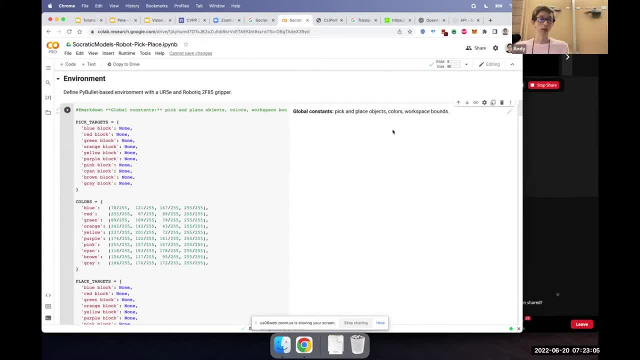 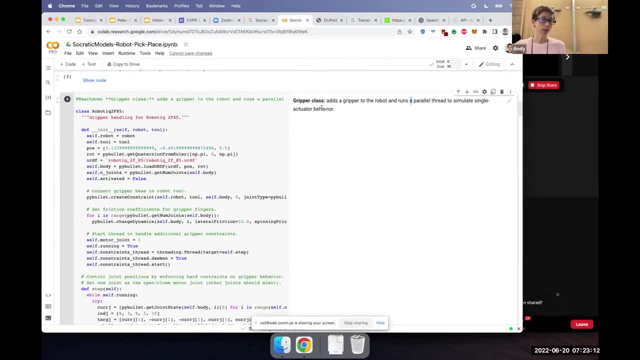 is just regular PyBullet, so you can. if you have URDFs, you can go ahead and load that in. There's a gripper class and this is particular. this is specific to the robot arm. So unless you're really into the nitty-gritty of how the robot gripper actually works, you can skip that. 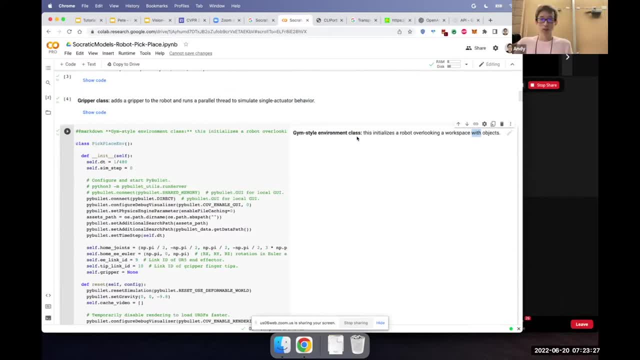 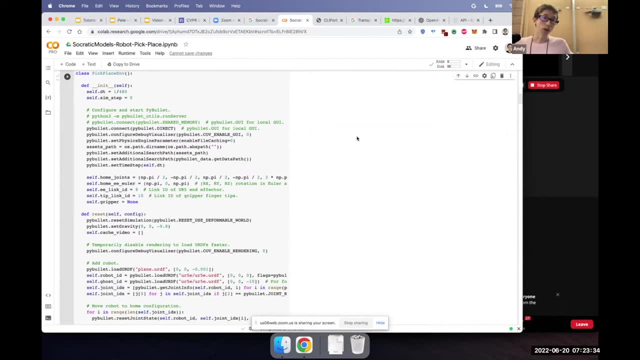 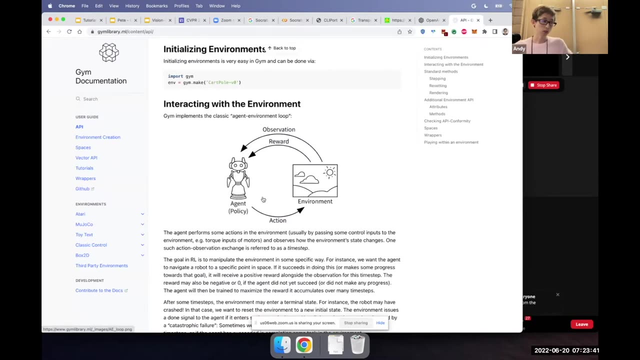 In the GIMM style environment. so in a lot of environments that roboticists like to play around specifically for robot learning, like to use the GIMM-based API, And what that is is that it's assuming you have a discrete time. 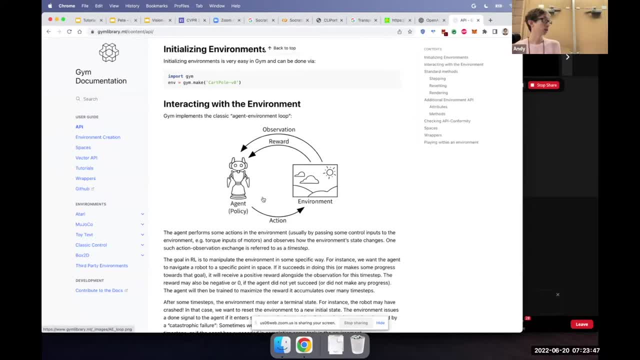 Markov decision process. It's assuming you have a discrete time Markov decision process. so you have an agent that's interacting with the world and it's operating one time step after the other, And at each time step the agent makes a decision. 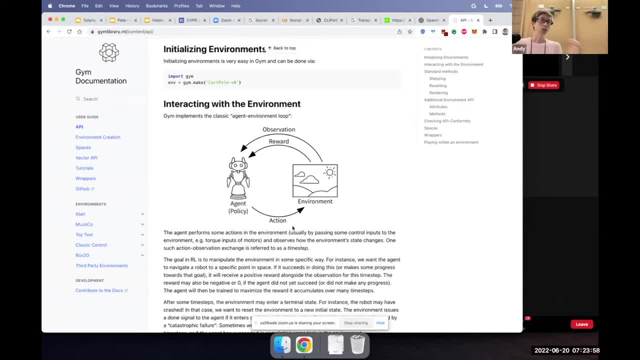 which is what action it should execute. next You put that into the environment. the environment simulates what would happen and then ultimately, you get some reward and some observation out of that. So this is specifically: the reward is useful for reinforcement learning. but if you don't have rewards, you can still study things like behavior. 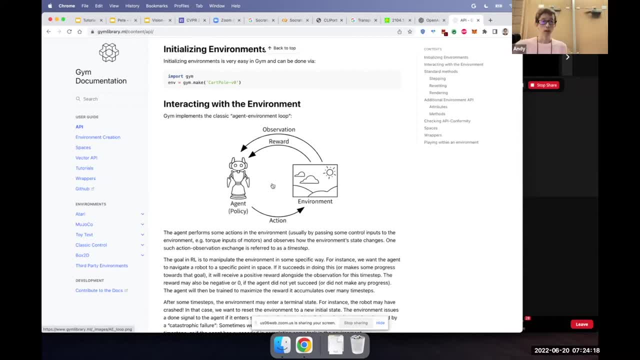 cloning, learning from demonstrations, imitation learning. So the format of the environment is very much the format of these GIMM environments, which ultimately have APIs and functions that return observations when requested. There's a step function that ultimately takes into account action as input and then outputs the next observation And then you have a policy which is 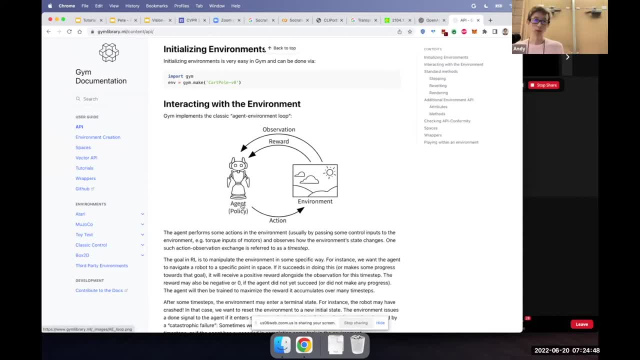 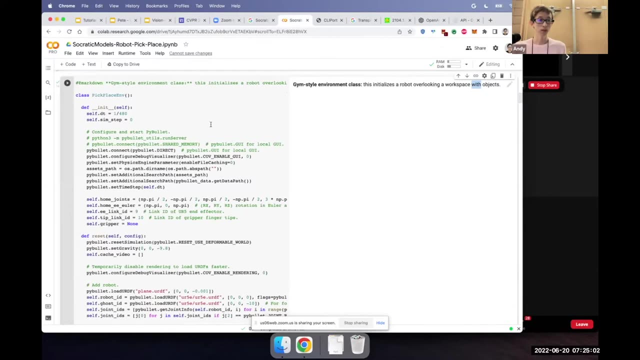 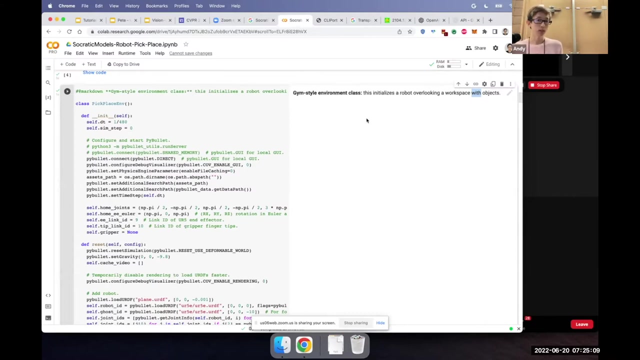 for example, the one that's making the decision about where to pick and where to place. That is our policy in our case. So here we have a particular GIMM style environment class. We also didn't strictly follow its GIMM style, as opposed to strictly a GIMM environment, so that you can also modify your. 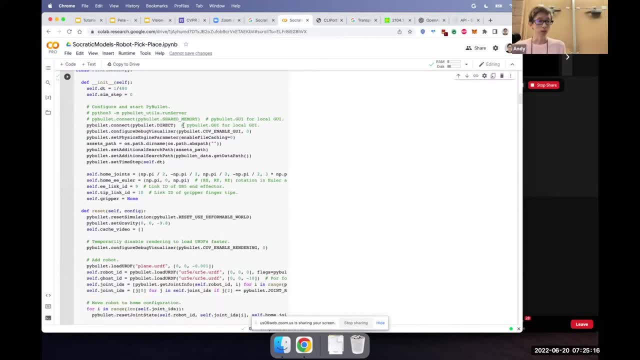 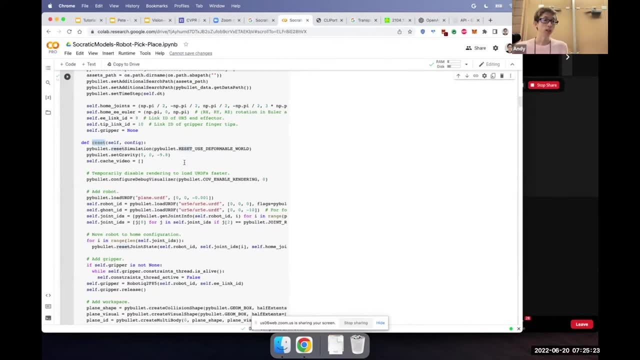 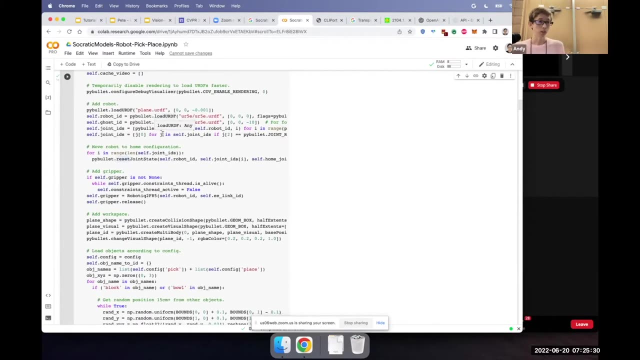 environment to your own desires. So a couple functions that I'll just quickly go over. During a reset function, this is going to instantiate a world set gravity. this is going to add in a UR5, which is a robot arm. It's going to attach a gripper to the UR5 robot arm and then it's going to add a bunch of objects. 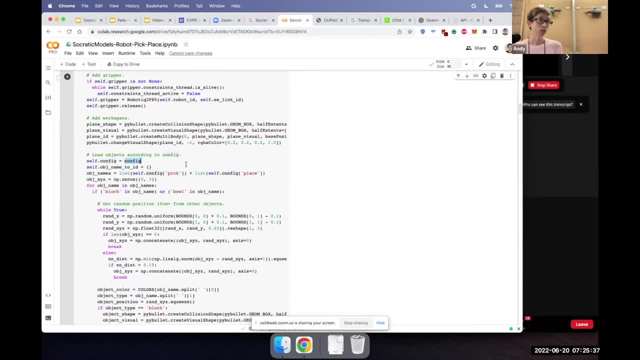 randomly according to config, which is a parameter that just contains a dictionary of all the objects you want to load in, So you can preset that with respect to whatever you want to load it, whatever random seed that you have, And then, once it loads in all the objects. 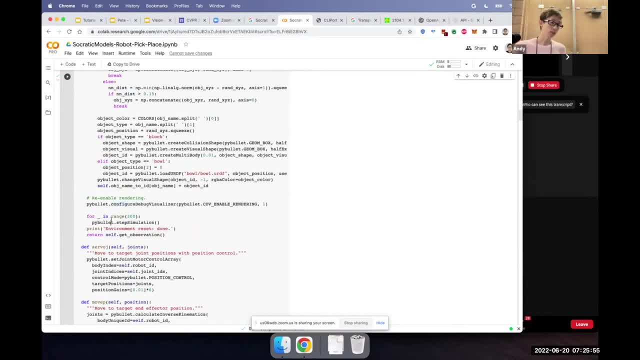 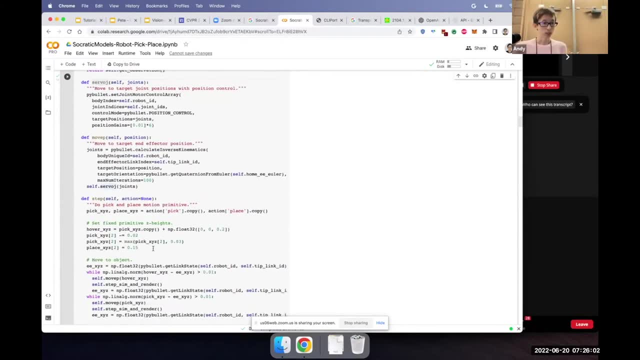 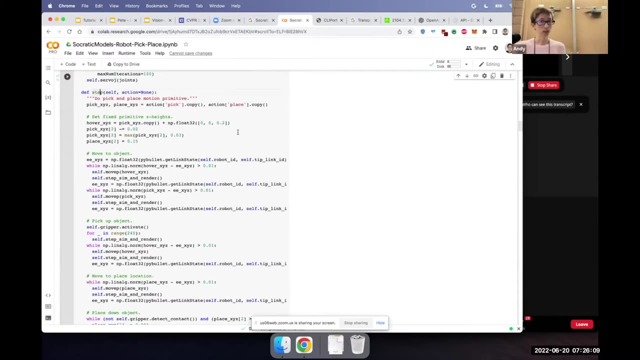 boom, the reset is done. Oh, give it a couple steps so that the simulator sort of settles and all the objects sort of land on their feet. There's a couple functions in here. Another one too is the step functions. So that's one of the main gym functions. 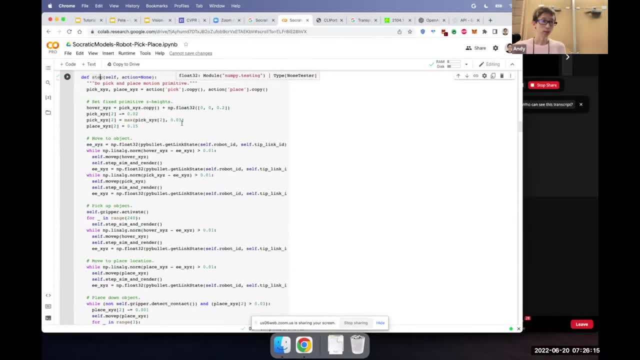 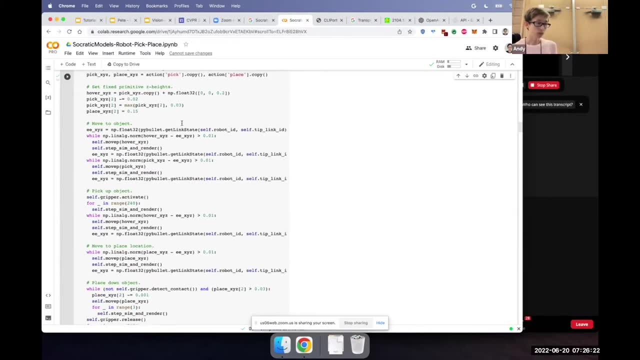 that I talked about earlier. You're feeding in the pick-and-place action and then it's going to specifically the And, depending on your problem statement, your step function might do different things. So, for example, if you're in a continuous control setting, 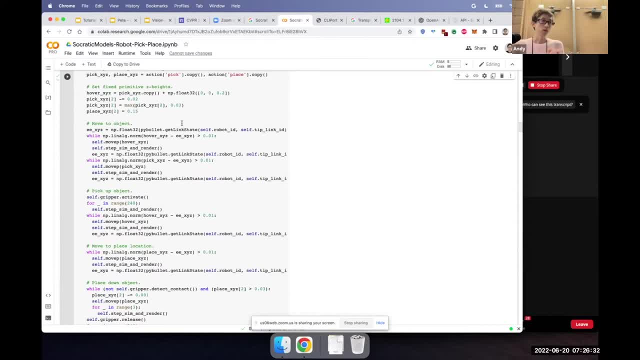 your DT is going to be very small and your robot might only move a little bit each time step. Specifically in this environment, we call it sparse control, which is that it's literally executing an entire pick-and-place action, So it's like a pick-and-place trajectory for each time step. 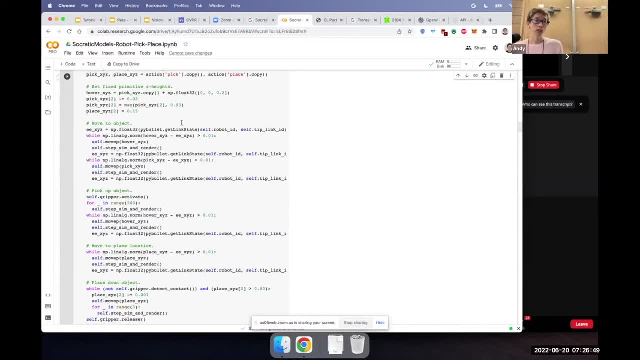 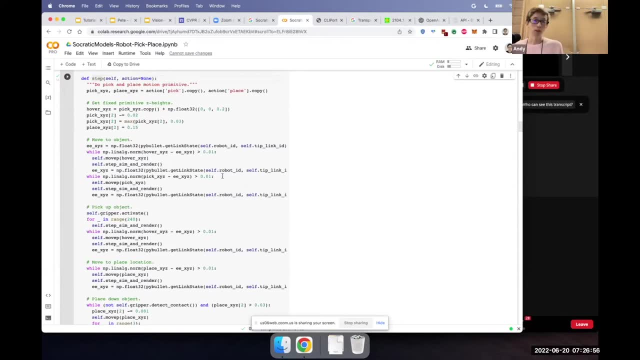 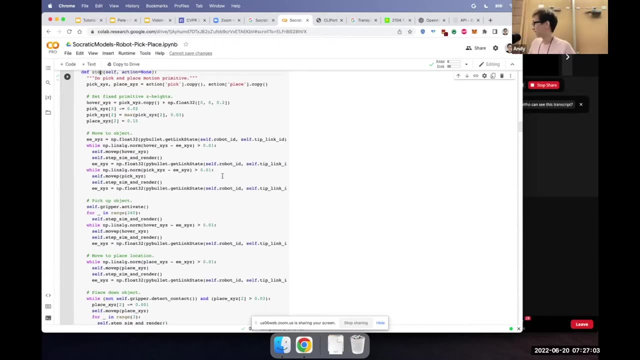 So the decision-making only happens in between each pick-and-place action. So this is particularly to this environment, It's particular to transporter nets and clipboard. But in the future you can modify this however you want The way to control robots and P that you want. 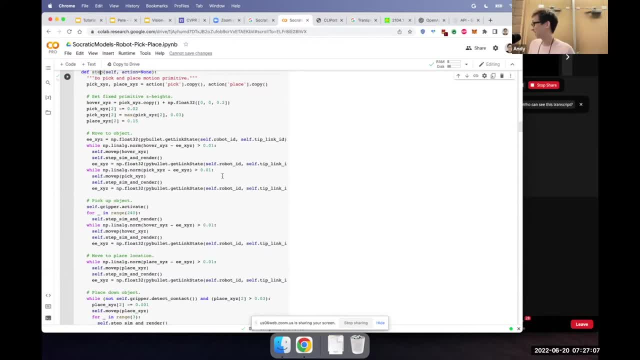 I was going to say: do you want to? You have a servo J and move J function in there. That's right, So you could call it how It's actually quite close to controlling the real It is. So on the UR5,. 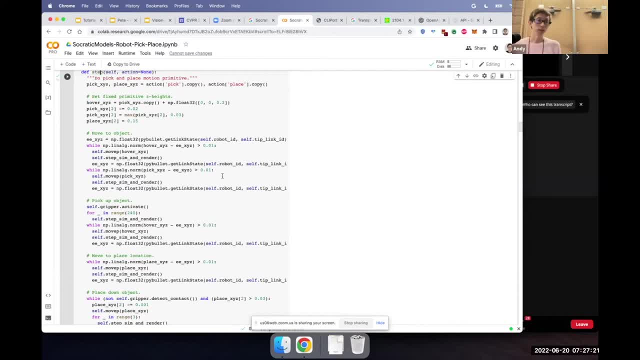 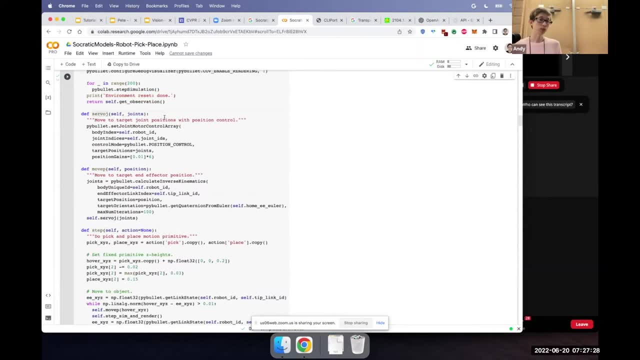 the way to control it is through joint commands. Up here there's move P and servo J, Servo J- the description here- move, the target, joint positions with position control, Each arm. typically you'll find either 6 degrees of freedom. 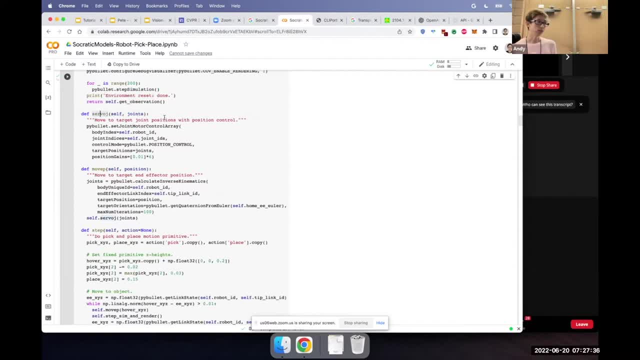 or 7 degrees of freedom, And usually the limits of those is moving between negative 2 pi to 2 pi and really you're just controlling What's the configuration that the arm should be in. now There's also move P, which is specifically move the target in defective position. 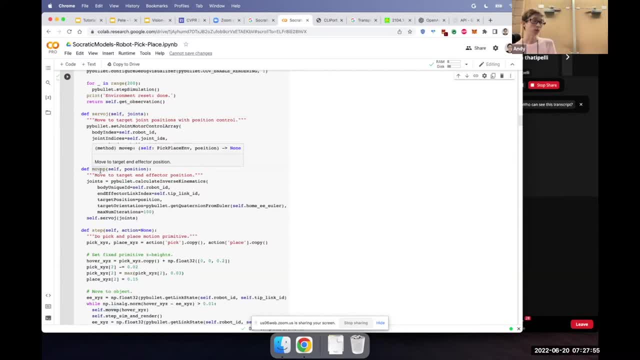 And this is running inverse kinematics as a way to give back what the joints should be, And then internally running a servo J to move the robot to that target configuration. So if you, for example, have a gripper and you're doing manipulation tasks, 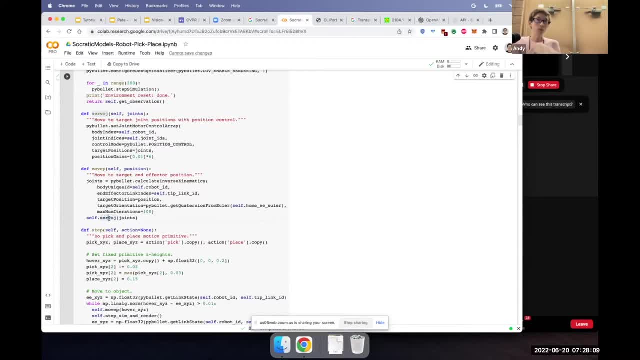 and oftentimes you're moving in this Cartesian coordinate space XYZ, then you can, You can, You can Use move P as a way to move your gripper to wherever you want And, as I mentioned earlier, you can set this to. 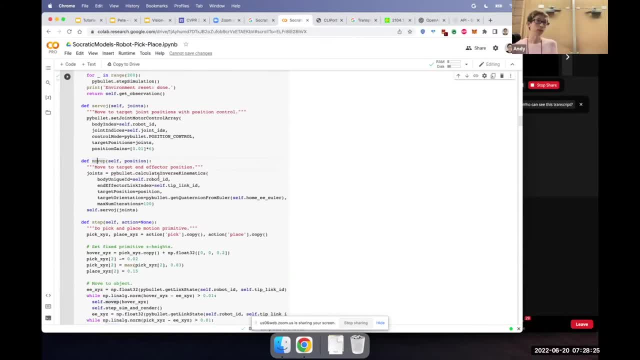 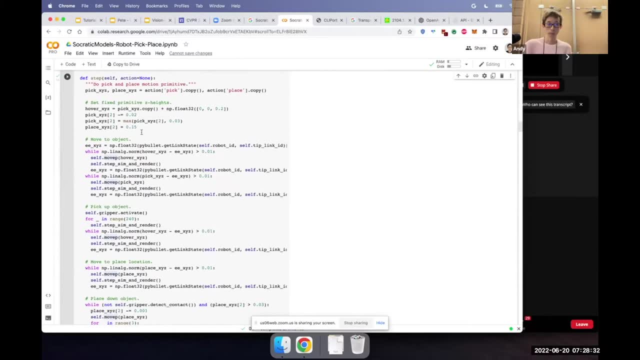 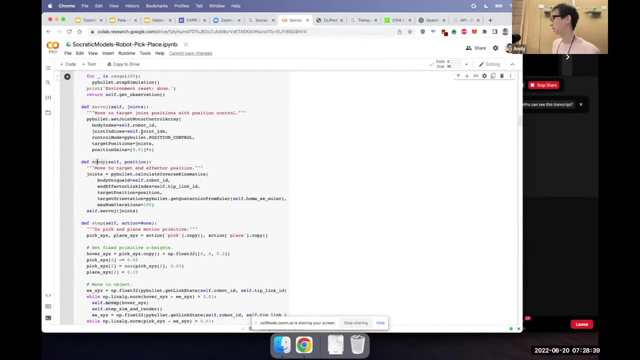 You can be moving a lot in a time step, but you can also be moving very little in a time step, and that leads to continuous control type settings. Pete, do you have any other comments related to that? A lot of the rest of it is handling rendering images. 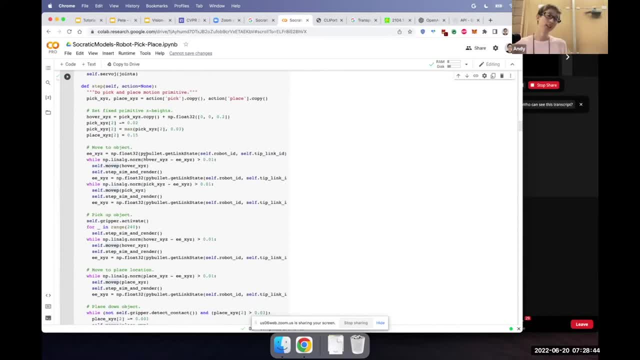 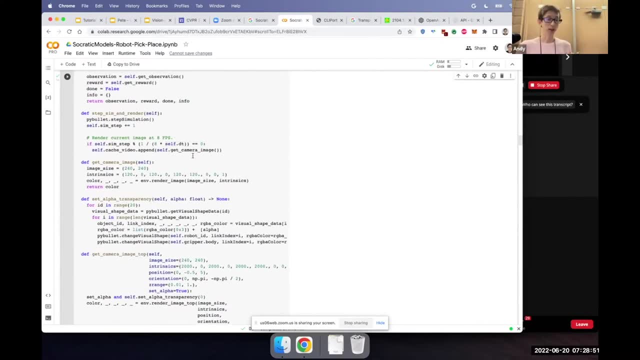 Okay, Yeah, yeah, I'm sure you can talk through a little bit, Okay, So the rest of this goes through how to render stuff, And I'm sure that many folks in this audience already knows how to do that. You want to set intrinsics? 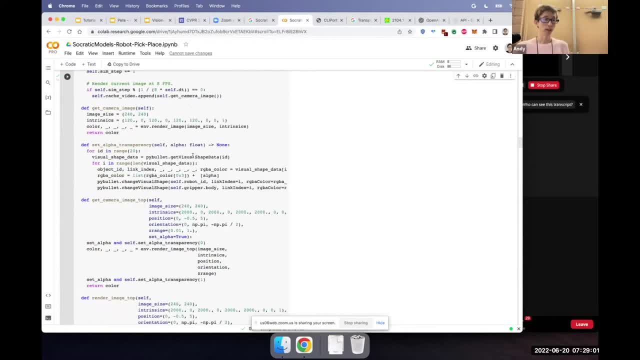 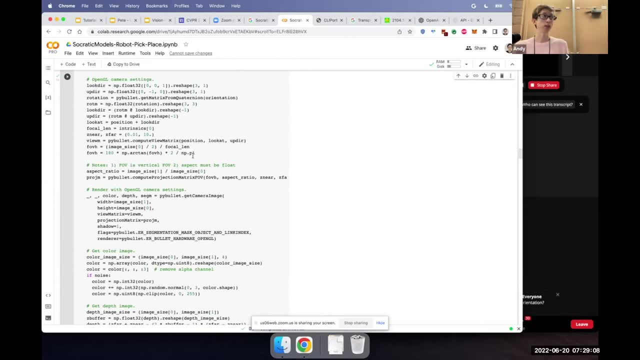 and you also want to set the pose of the camera, And there's two types of cameras that we're working with here. One is perspective and that's just your regular typical camera and physical camera at least- And then you have something more challenging. 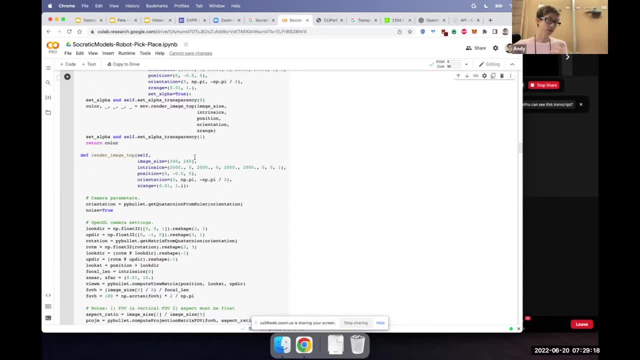 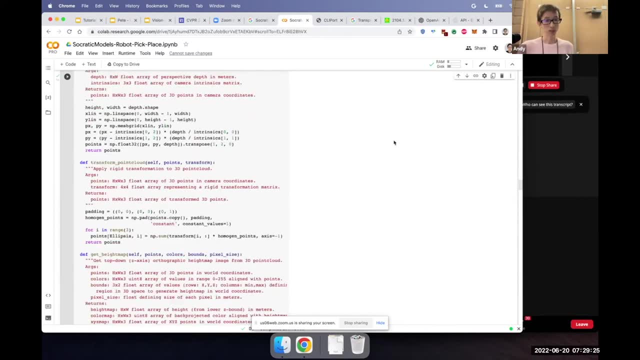 which is the Or more challenging to build in, the, I'd say it's possible to build in the real world orthographic cameras, which are essentially these top-down views. Let me scroll down real quick and give you an example: These top-down views. 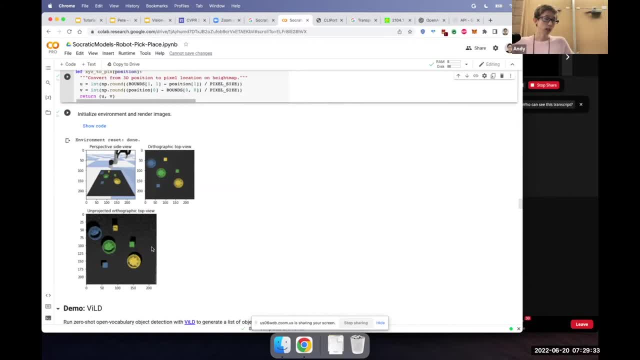 And specifically in the context of robot learning. these top-down views are great because you don't have perspective distortion. So if you're running, for example, a fully convolutional, a fully convolutional network, to make a dense prediction of where to grasp. 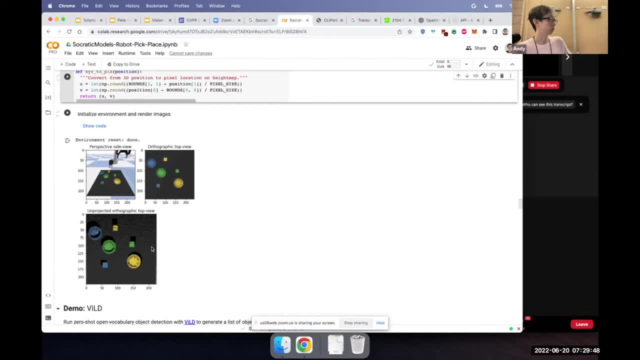 you can be sure that your convolutional kernels will not be subject to the biases from learning over perspective distortions And, if you wanted to, Each dense prediction at least has a very nice inherent bias: that every pixel coordinate represents a fixed column of 3D space. 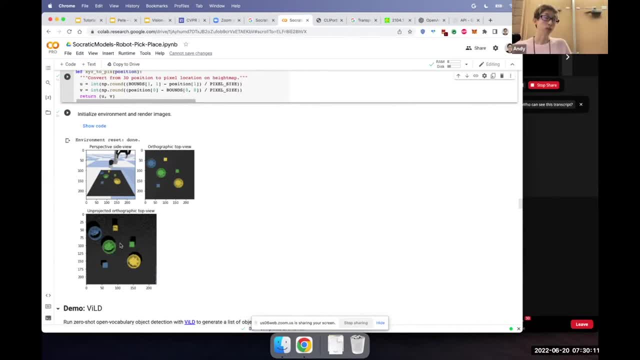 So, for example, every pixel here represents around two millimeters, which is nice if you're doing planning or if you're in the context of navigation, for example. a top-down view is quite nice in that setting too, to do shortest paths, et cetera. 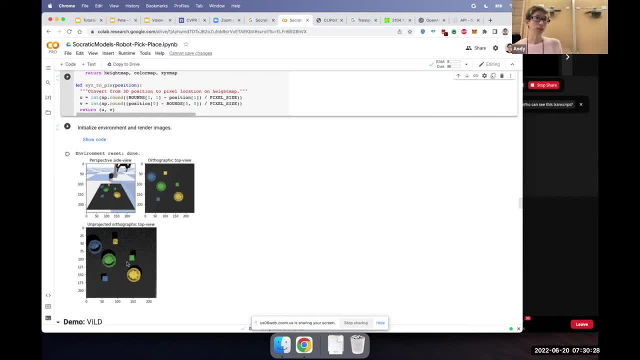 So really, this is just a proxy of a 3D representation that we would typically want. But the way to get this is we would take an RGBD camera and it has to be calibrated so you know the pose, project it into point clouds. 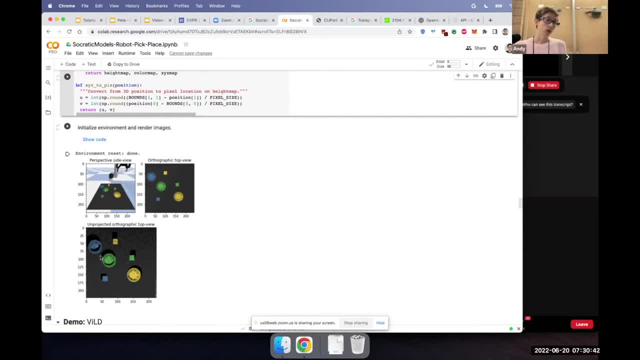 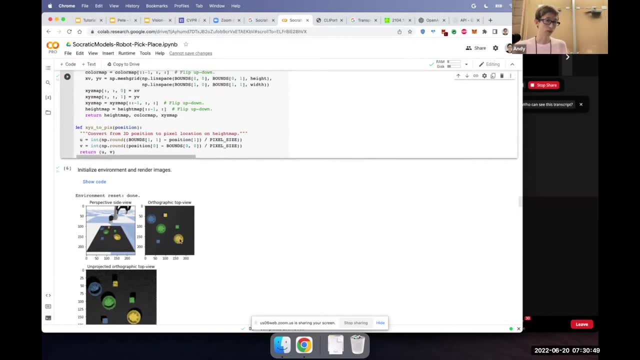 and then re-render from this orthographic camera So you can see the view point. So oftentimes you might get artifacts with spot G dots here, but then if you wanted to get a perfect orthographic view, you can do that in simulation. 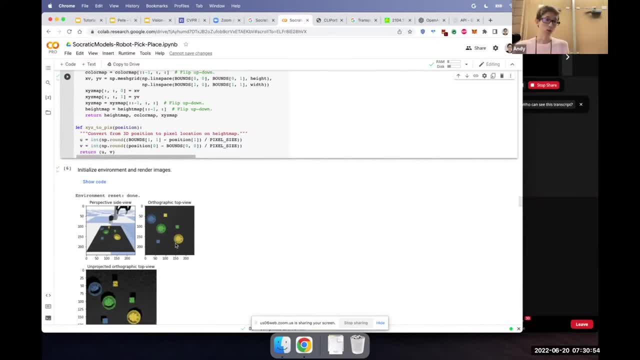 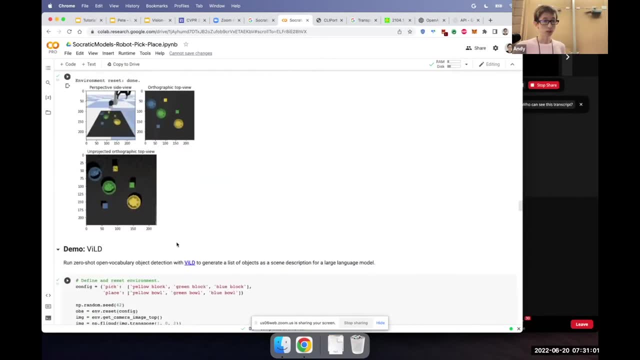 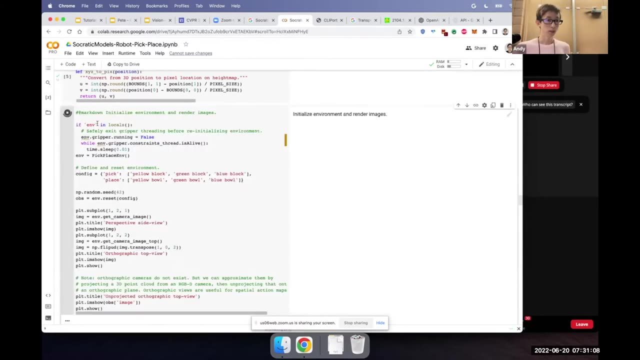 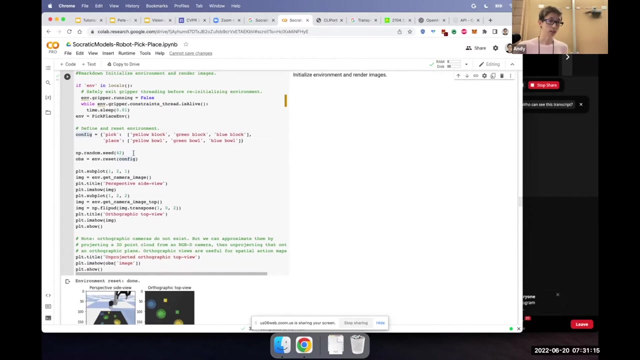 but generally getting these types of views is harder, or you need to have some particular setup. Okay, So that's most of the environment code. Yeah, And essentially, to initialize an environment, you want to define what are the objects that exist in the environment? 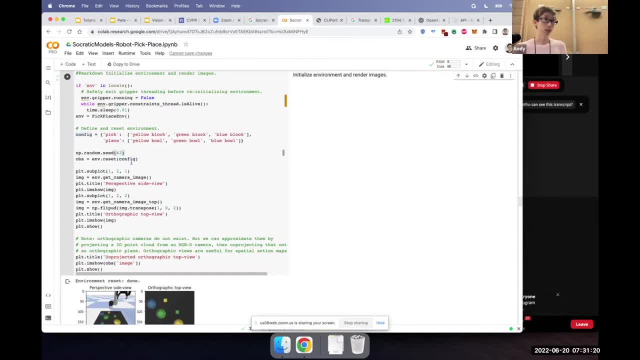 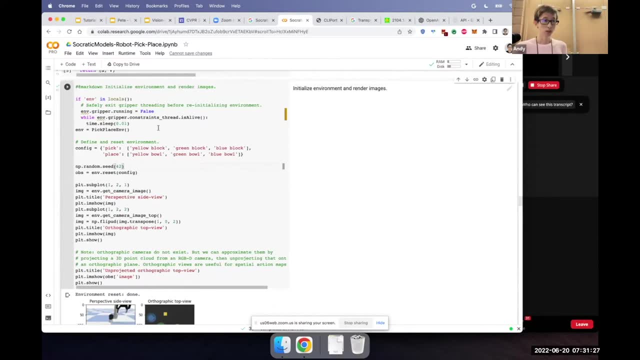 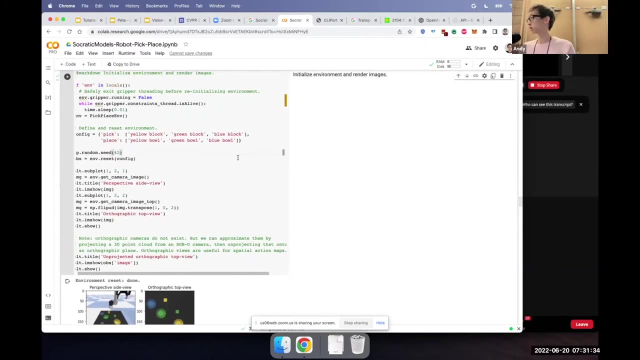 You can set your random seeds, arrange the objects and it'll randomly arrange the objects with respect to the seed. So are there, before moving on, are there any questions so far in the audience? Any questions on Zoom? There's some questions on Zoom, yeah. 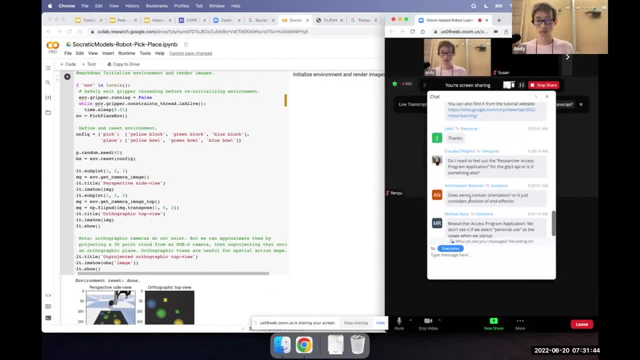 Yes, Okay, Is servoJ contained? Yeah, that's a good question. ServoJ is just the joint configurations, So each degree of freedom, which is, for example, elbow, really only has one degree of freedom, The orientation, which is. 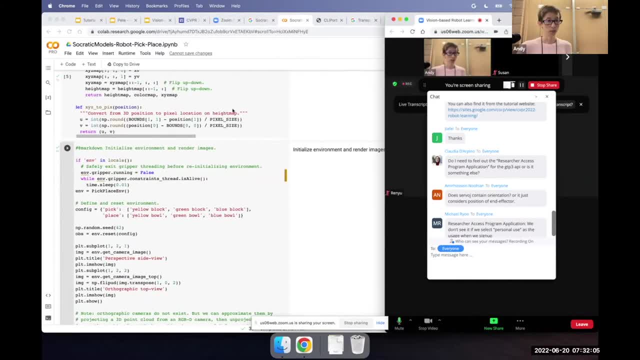 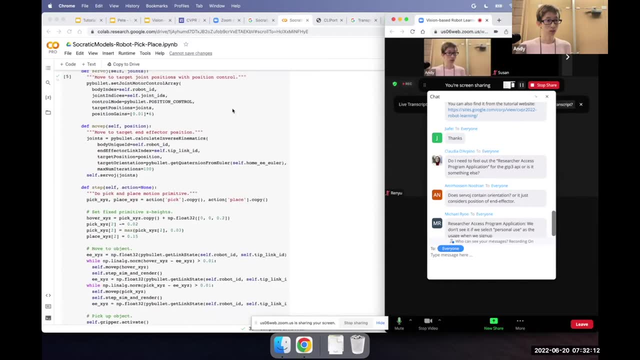 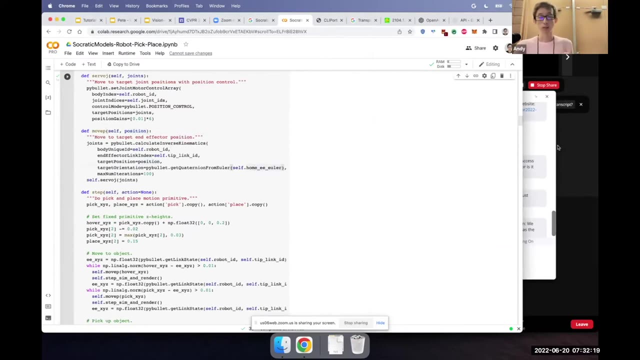 if you wanna control the orientation, you can do that with moveP. So I believe the code as an example of that. Oh Turns out it doesn't. Okay, I see Okay. So if you want to control your own orientation, 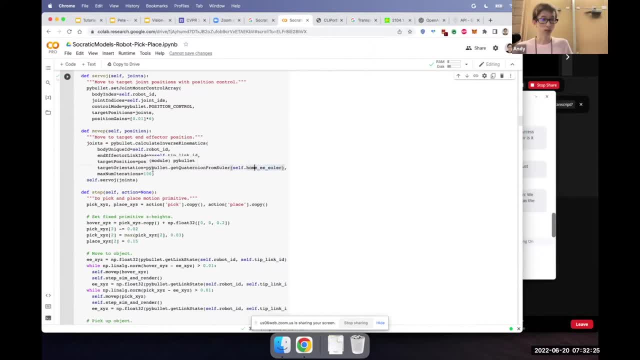 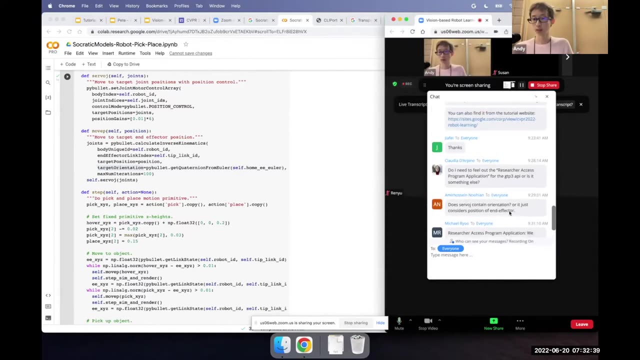 you can, but you want to set the quaternion which is target quaternion here, parameter Here. we have it fixed to be always top-down, but you can definitely change that to something else. Good question, Yeah, good question. Any other questions? 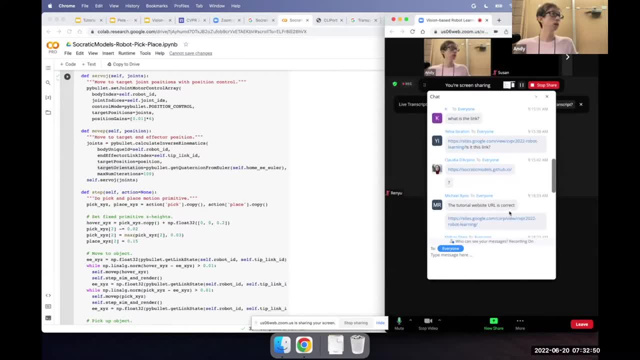 Hi, Yeah. So do I understand correctly that if you give the target coordinates to the pipeline then it will handle the out-plumbing? So it'll tell you the target joints, but then the Yeah. Yeah, So it'll tell you the target joints, but then the Yeah. 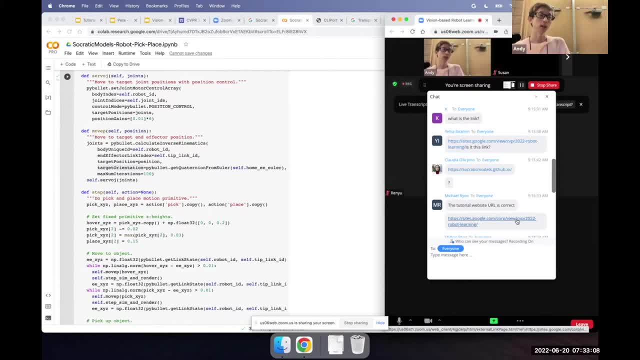 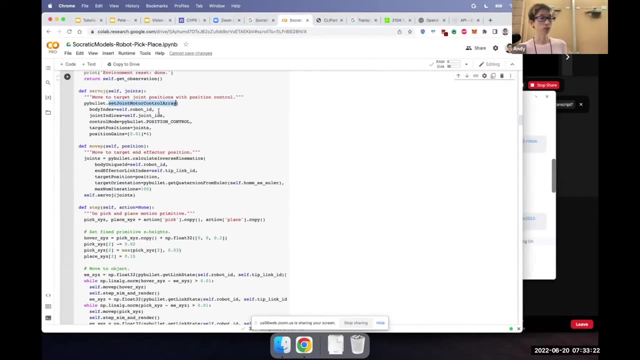 So it'll tell you the target joints, but then the actual path planning of dodging obstacles. it might not So with just a simple PD control where it closes the loop so that it goes to the target joints. yeah, that's already taken care of, So that specific command is set, joint motor. 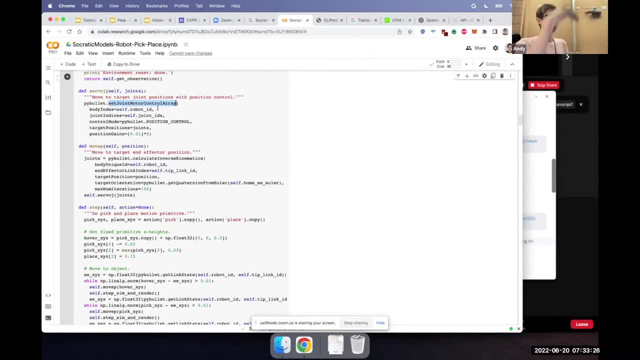 control array So that actively moves your robot to the target joint position. But if you have obstacles in the way, it won't be able to handle that. So which part of the pipeline is handling That'll be in between sort of these lines of code. So if you wanted to have it, 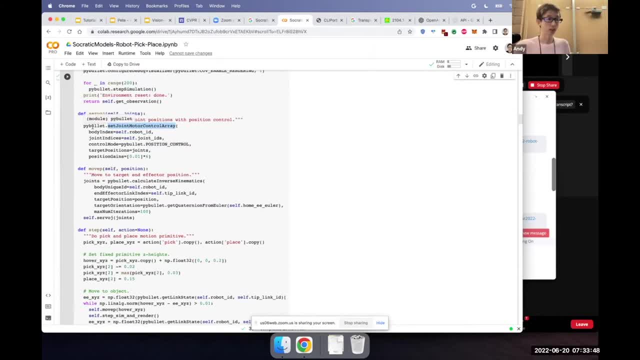 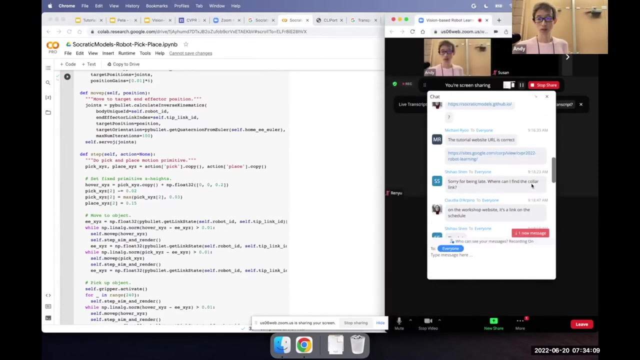 be aware of obstacles, then within this function here, servoj, you can have it take into account additional information so that, So this one doesn't do it, This one doesn't do it. Okay, Thank you, Yeah, Yeah, Okay, Moving on. Oh, does the simulator take singularities into account? 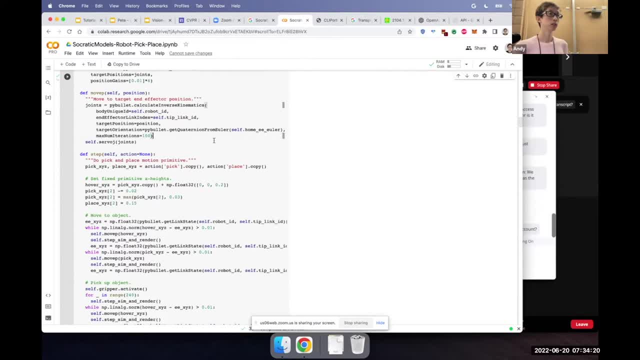 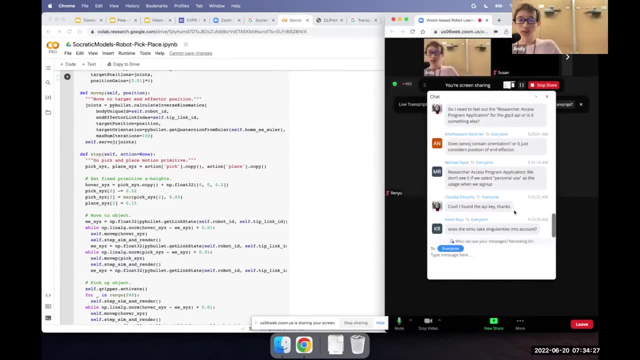 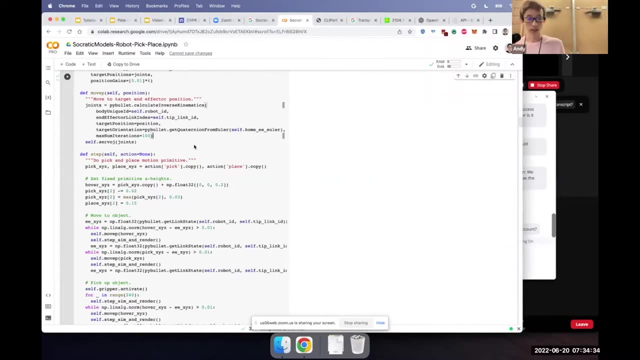 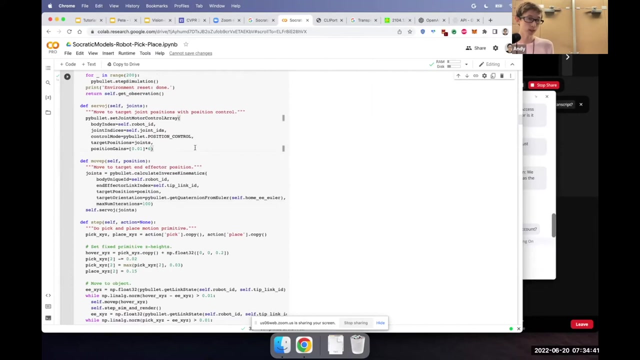 Also sorry, Yeah, Can you speak a little bit about it? Yes, Yes, So does. the simulation takes singularities into account. It does not, So specifically, with the inverse kinematic solvers. here it uses cyclical coordinate descent, which means that it's an optimization-based algorithm. 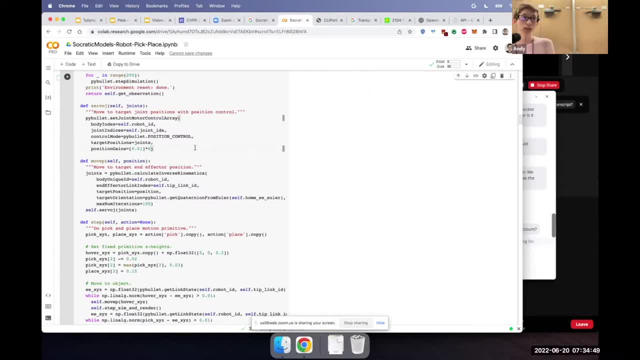 So you have an initialization of the joint pose and then it's going to compute gradients on that joint pose as a way to iteratively move to your target joints. So you do have some inverse kinematic solvers that are not optimization-based. Those are the analytical ones. These ones would tend to fall into singularities where you need to have some way to strictly handle those. But the PyBullet inverse kinematic doesn't. but it does require you to have a good initialization in the beginning. So if you're constantly moving your robot smoothly throughout 3D space, then it's usually okay for most purposes. 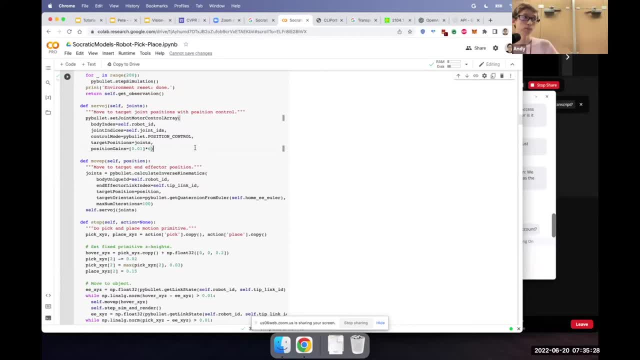 Um, But if you're jumping to a very far position, then the robot might not give you a solution that you originally intended it. So it's good to keep in mind that, if you want to- for example, if the robot had one particular pose on one side of the workspace- 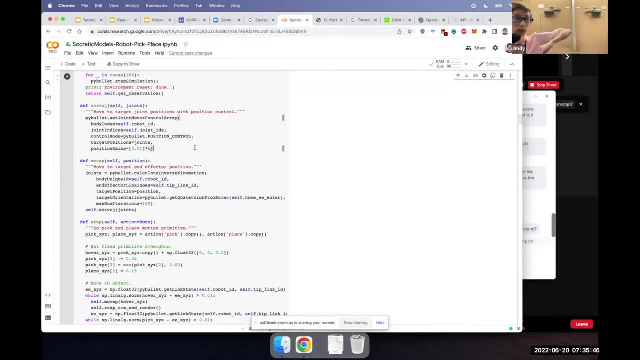 and then you wanted to move it to the opposite side of the workspace. if you see that in transition of moving over, the robot sort of flips its elbow upside down, that's because the object optimization didn't find a plan that was at least keeping the elbow up the shortest path. that didn't necessarily. 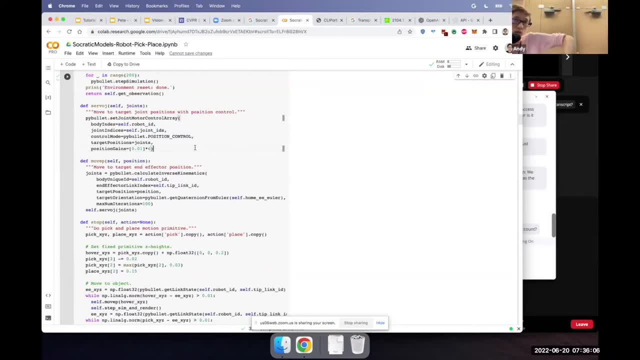 get to that. So you want to add additional waypoints in between so that you can keep the arm elbow up. That's a specific thing for path planning. Do you also want to add a couple things? Okay, To add a couple things, And there's been some good questions. 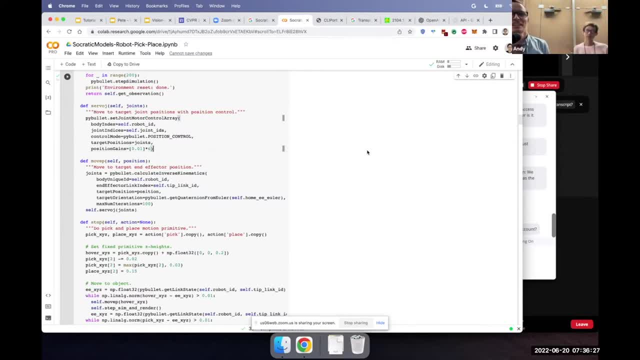 So I think one thing that's helpful to keep in mind is like there's good questions about like, oh, is this doing obstacle avoidance, and oh, or like you gracefully handling singularities, And you know, robotics is very hard. So I think whenever you can kind of like ignore certain problems and focus on other ones, it's very helpful. 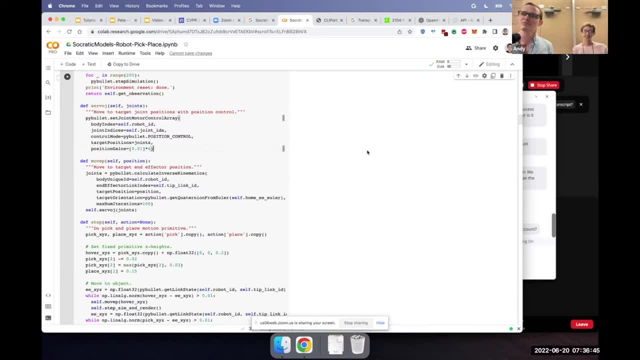 So like there's actually a ton of robot demos that you'll see And you might think like, oh, that robot probably can do everything, But actually it basically can't do anything. that it's not showing often, And so there's a lot of robot learning research. that happens where you have a robot sitting next to a table and it can't handle obstacles. 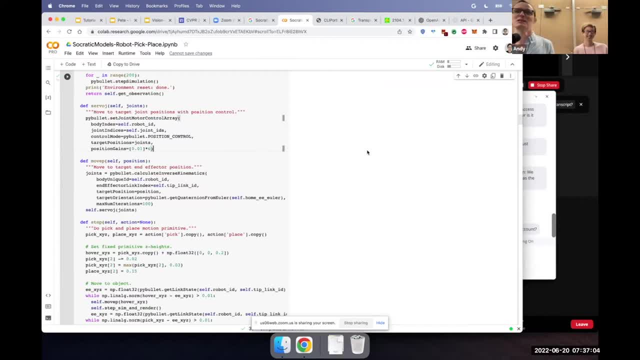 And like everybody knows that we could engineer it to handle obstacles. But then that might be like actually obstacle avoidance and path planning is its entire own, like massive subfield with many decades of research and very challenging. So if we were to add in obstacle avoidance here it could potentially double, if not more, the size of this co-lab. 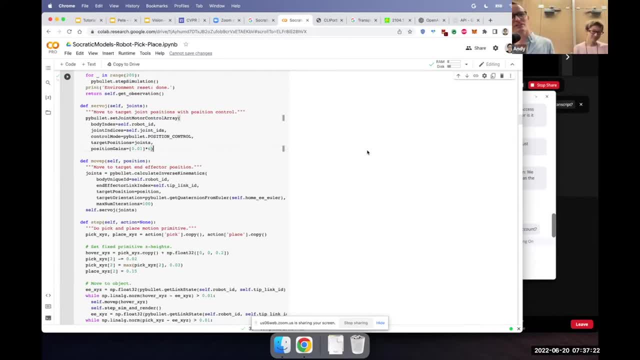 And so it's just helpful to sort of like you know when when certain things happen. Yeah, So you know when, when certain things can be studied in isolation, it's helpful. And then, another thing that I wanted to call out too is Andy was walking through kind of how the simulator is set up. 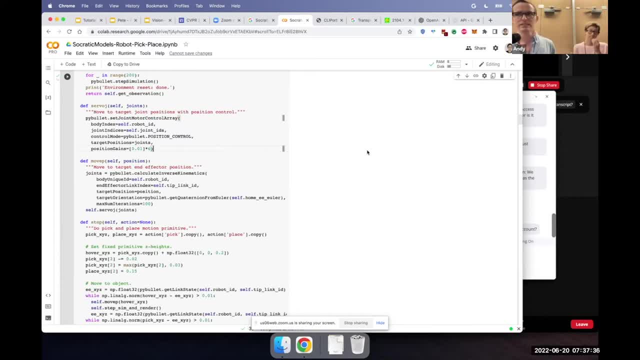 I think it's a really nice, like you know, easy to play with simulation setup. One thing to call out as well is like the actual choice of what are we simulating and like. what are the objects and what does the scene and the environment look like and what can we do with that. 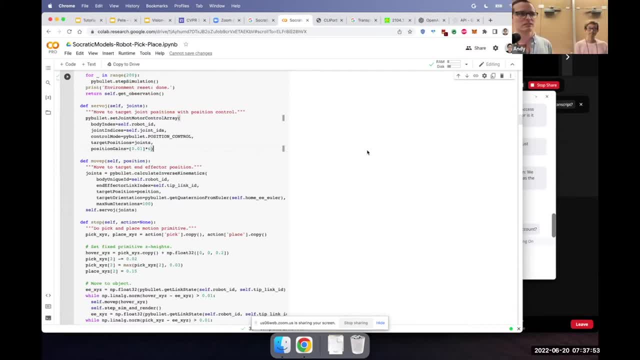 Yeah, Yeah, I think that's a really interesting question. I'll cover some of that more in my talk later. And here you know it's pretty simple. We've got a robot sitting next to the table, got some blocks, got some bowls. 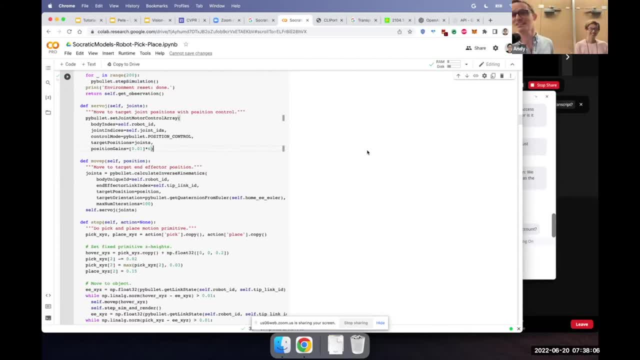 And, importantly, some of the blocks are color different than other blocks and some of the bowls are also color different And you'll see later. as simple as this is- just a few blocks and a few bowls with different colors. It's sort of a really nice level of complexity where it's complex enough to actually do some really cool like language condition, pick and place tasks, which we'll get to later. 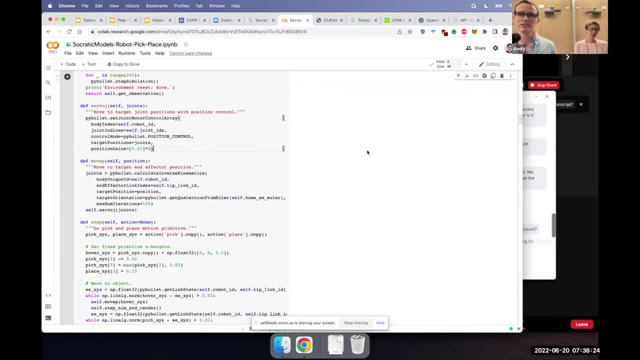 But it's also not. you know too too much. We're not doing some like. you know GTA 5, you know triple platinum video game environment, So I just wanted to call out those things Cool. Thanks, Pete. 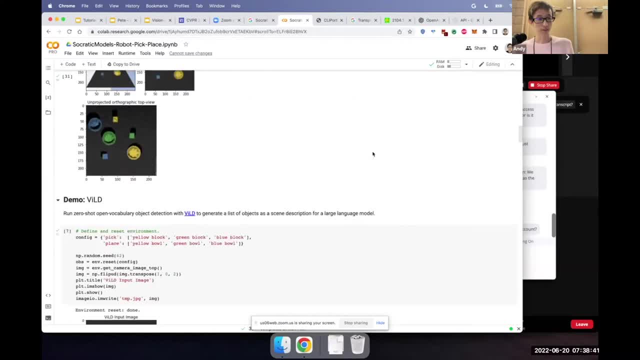 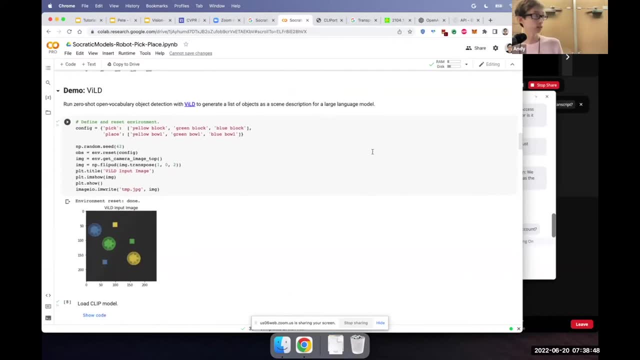 All right. So, moving on, The next part of the CoLab hops into running Vyld, And a lot of this code comes from the Vyld codebase itself, So you can go ahead and take a look at their paper, as well as their GitHub links, if you want to learn more about their code. 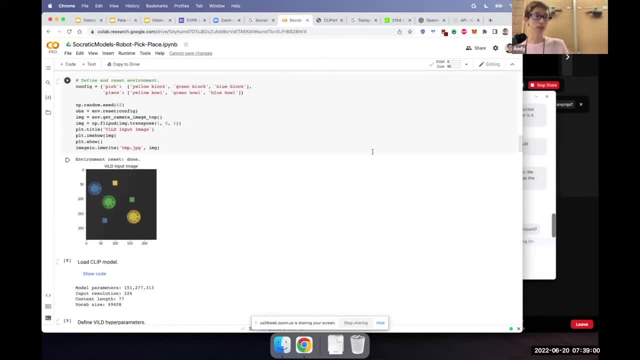 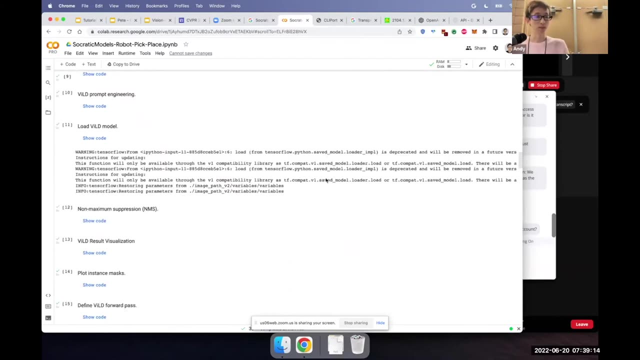 But specifically how this is being used is to generate, convert from an image to a list of objects that we would see in the scene, And this is helpful for providing language-based context to the planner. So this whole section here, demo Vyld- sort of just goes through that. 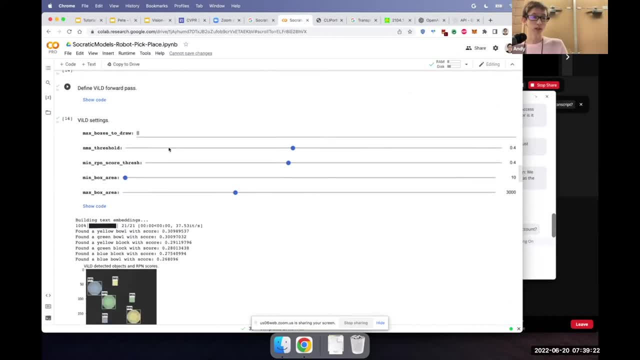 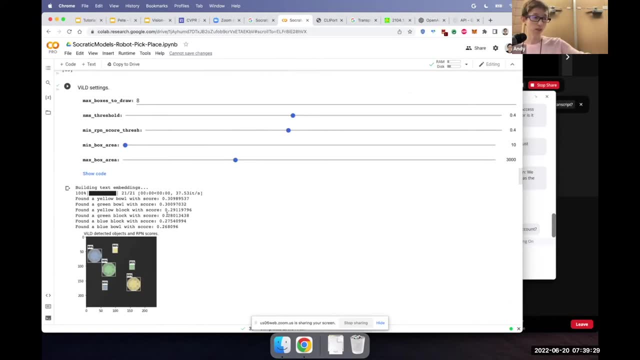 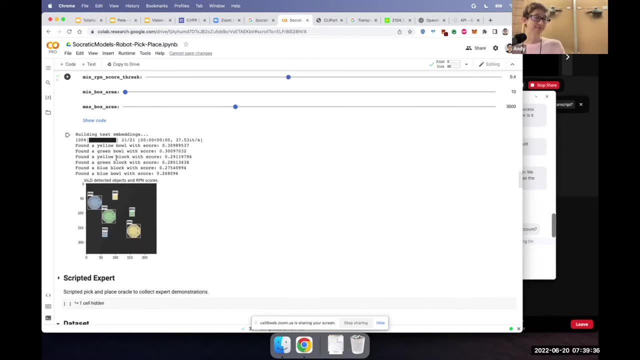 Loads of Vyld demo downloads runs forward, pass. You might want to play around with this hyperparameters in case you need to set the object detector in a specific way, But ultimately we're using it here just to you know, discover where the yellow bowl is, the green bowl is and the blocks are. 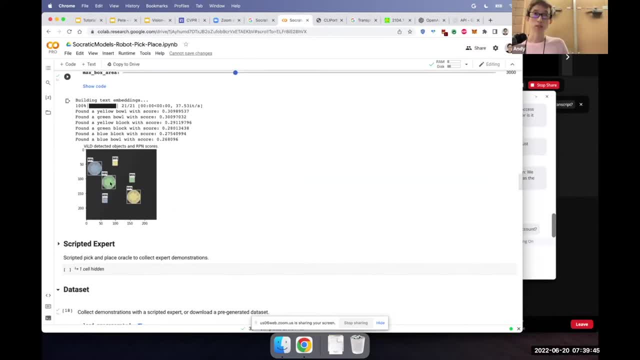 And we're not taking into account the spatial information. currently We're just formulating this list here. Later, downstream, we'll have a robot policy be able to figure out where it should grasp or where it should pick and place. So the spatial information actually gets tossed out the window. 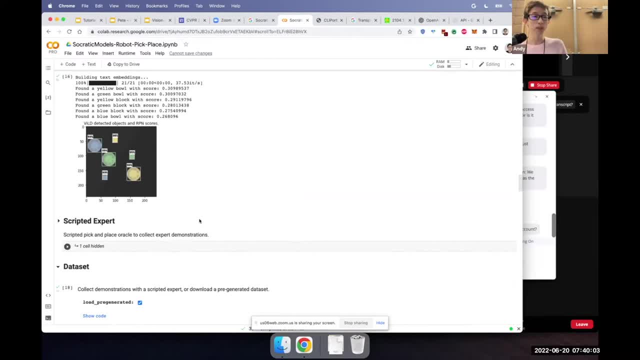 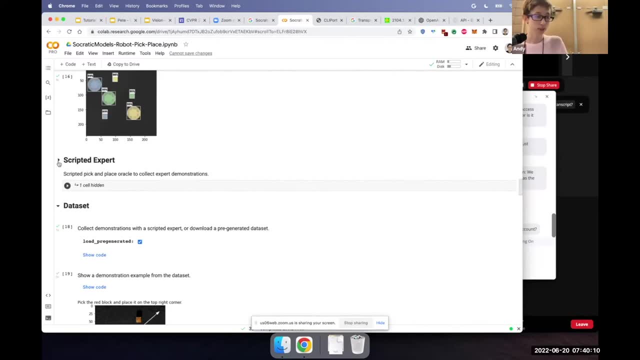 So really only using it for object recognition. currently We have here a scripted expert, So I guess a lot of paper terminology uses this term- scripted- Which just means that somebody hard-coded a couple of heuristics or maybe even potentially writing some complex algorithm behind it. 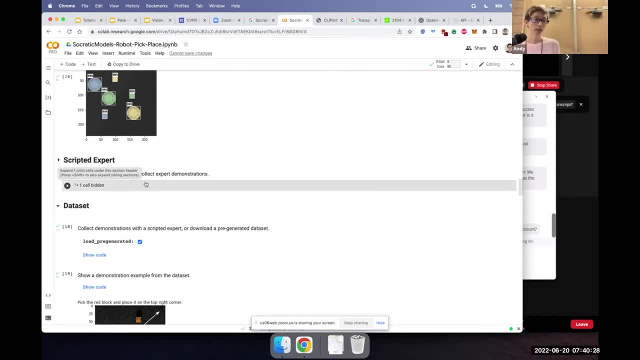 But ultimately it's manually engineered, And what we mean by scripted expert is that this is an Oracle system that is able to execute pick and places And you can use it to collect demonstration data- And there are, at least in the context of learning from demonstrations. 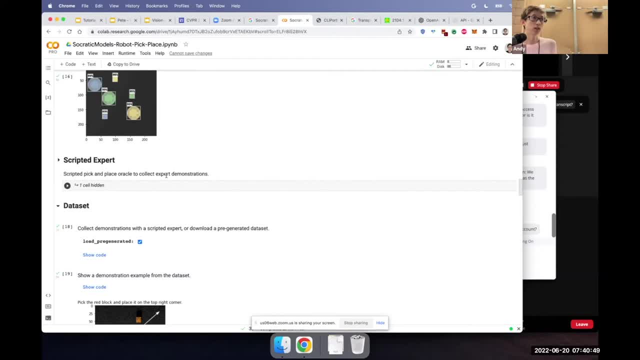 if you're studying it inside of a simulation environment. there are various different ways to get those demonstrations. You could either use a scripted expert which has access to the ground truth poses of the object so that you can pre-compute where you want to pick and place. 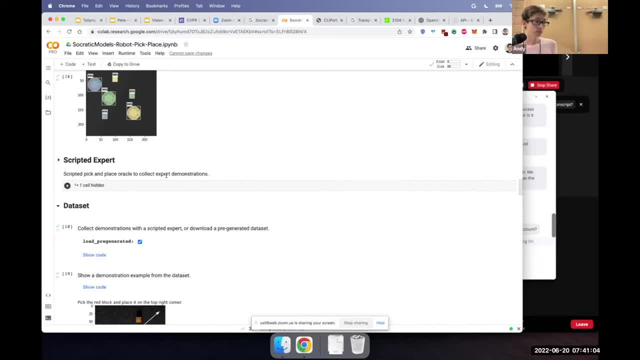 But you can also, for example- and very good work from, for example, NVIDIA's lab, where you can have a person hand, track their hands, or maybe even using teleoperation tools to try to control the robot, whether it be in real life or in sim. 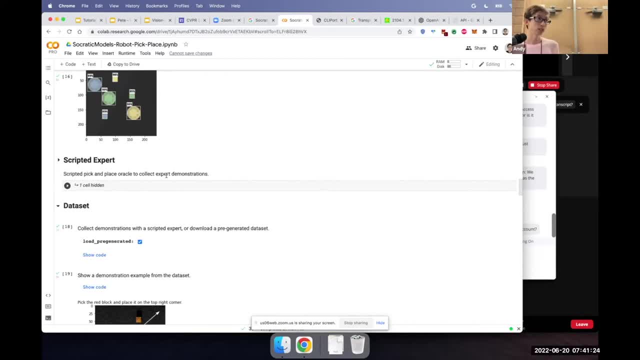 you can move the robot to do various tasks, And that's one way to get expert demonstrations. And another way to get expert demonstrations, too, is training an RL agent to solve the task first, And then, depending on the seed, you might have good expert demonstrators, maybe medium demonstrations. 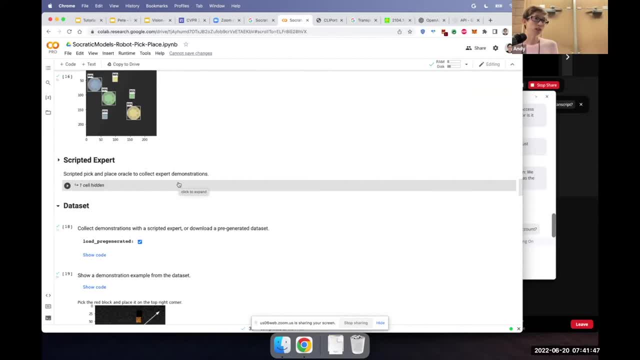 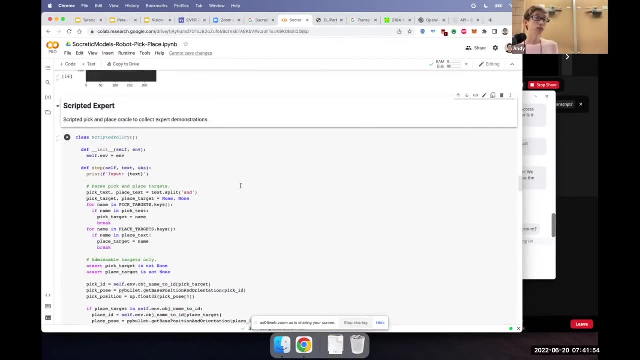 You can use all the trajectories that they come up with as a way to provide expert demonstration data. But yeah, in the context of this collab, we're just using a scripted one that uses the ground truth state. This is access to privileged information. 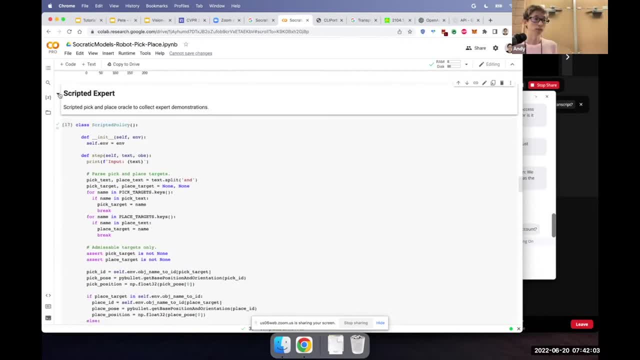 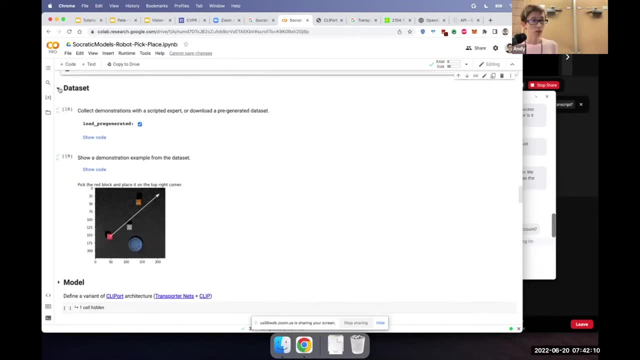 So this is only for generating training data Later on. the policy that trains off of this does not have access to this information. The data set section: you can either. There's a check mark here for load pre-generated. We did pre-generate a data set of 10,000 pick and place examples. 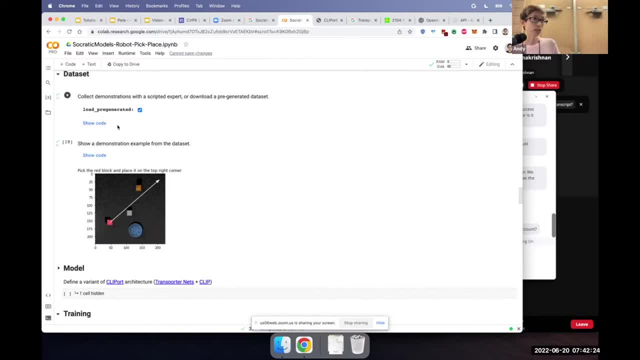 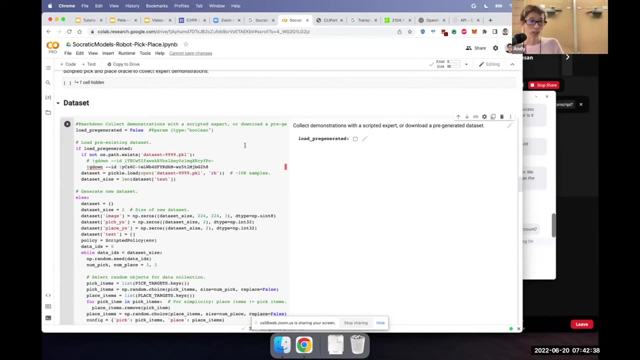 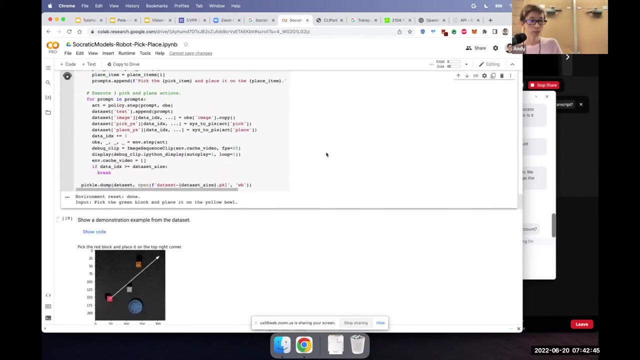 So that when you run, all with this checked, it'll download it by default. But if you uncheck this, then you can generate your own too. So, just to give a quick example, we'll uncheck this, So it'll generate a random instruction. 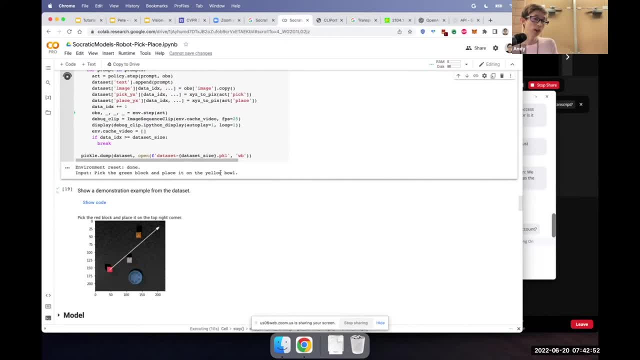 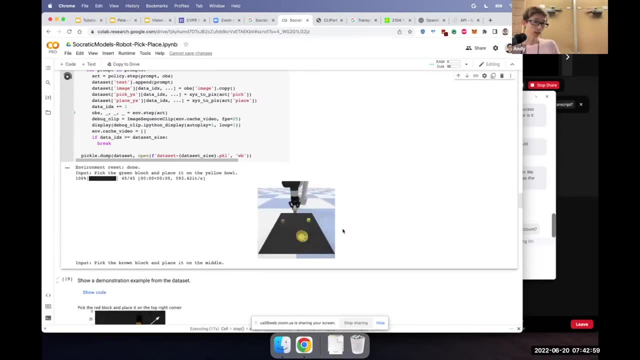 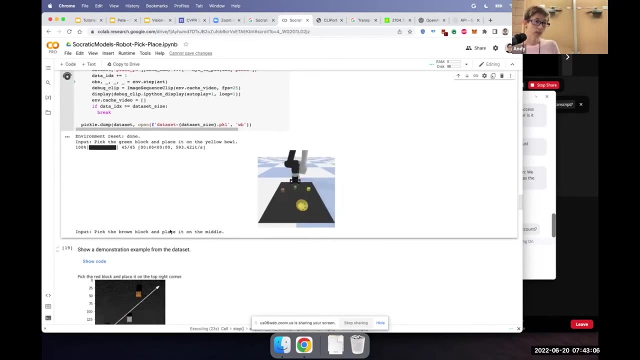 Pick the green block and place it on the yellow bowl And then the simulator will run. The video recorder will record what the simulator saw And then I'll put it inside the collab notebook So you'll see the robot executing this. So, specifically here, I chose to generate two. 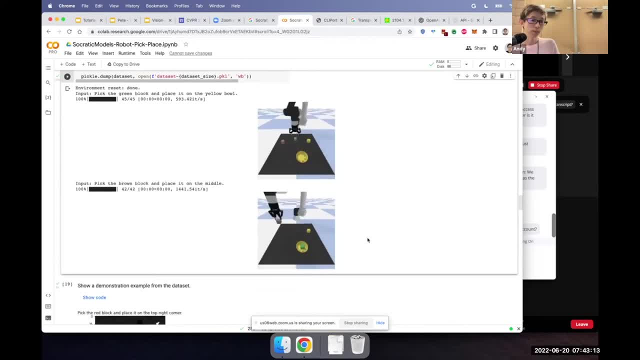 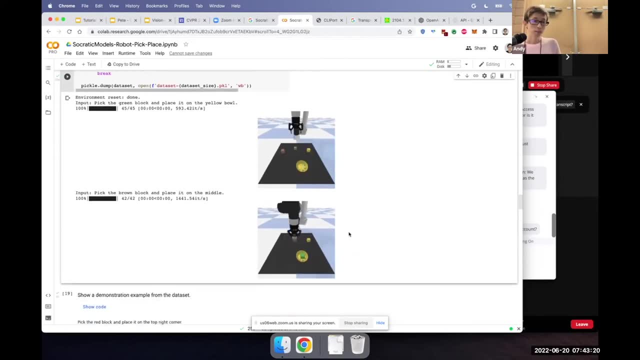 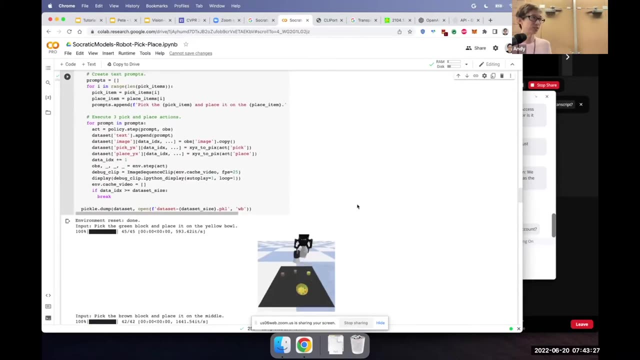 So that's why you're seeing two videos here And every now and then, while you're generating training data, you want to reset the environment with new objects, new bowls, et cetera, And it's funny because resets in simulation are so simple. 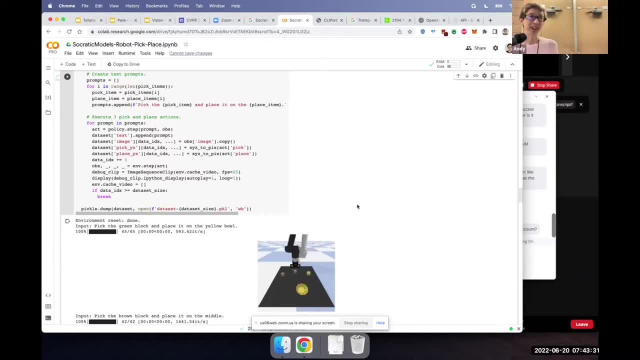 You can just code it up, But in the real world they take a lot of manpower. You've got to have somebody who's next to a robot all the time, wrangling, resetting objects and trying to move them in similar places. So it's. 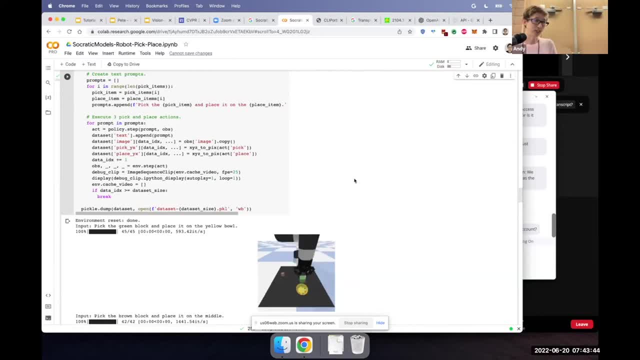 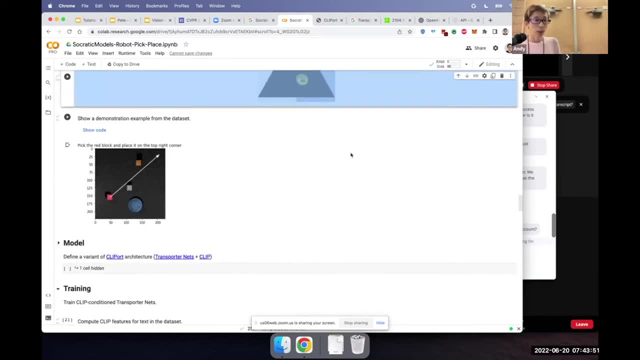 Anyways, in simulation it's quite nice. It's nice to have this, And you can literally also debug with it too, because if you set the random seeds, then you can control it to however you desire. Cool, So the information that gets saved whenever it executes a pick and place action. 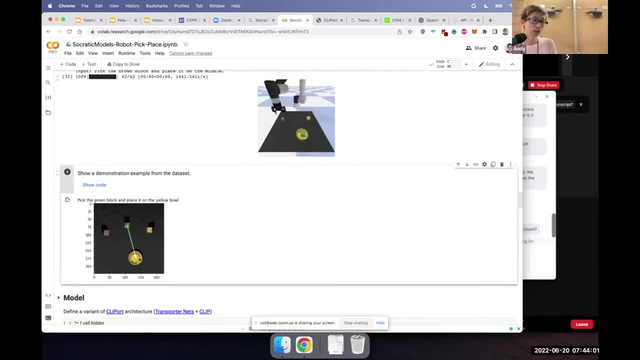 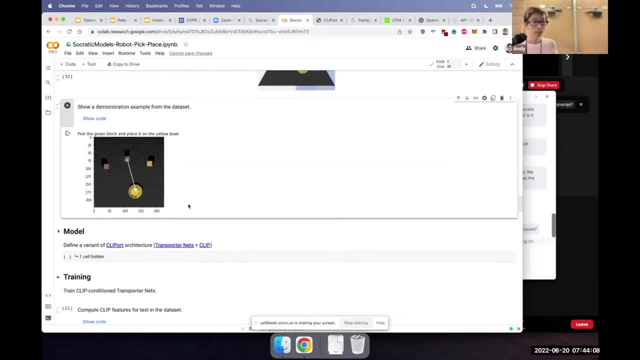 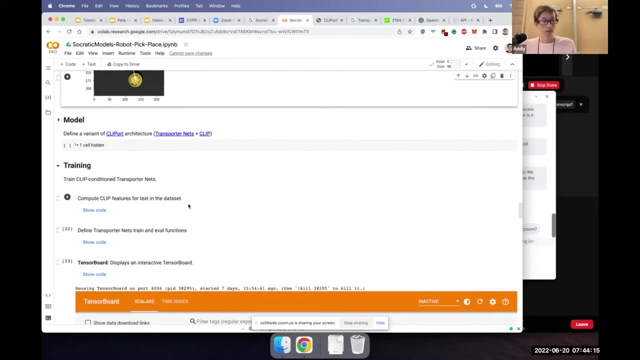 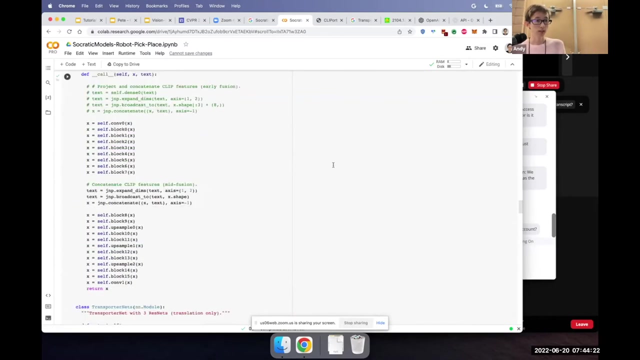 is the pixel location for which the pick was executed and the pixel location for the place, as well as the textual command that was received as input. Okay, So there's a Here we have a section on model, And all of this is. By the way. I also want to call out that 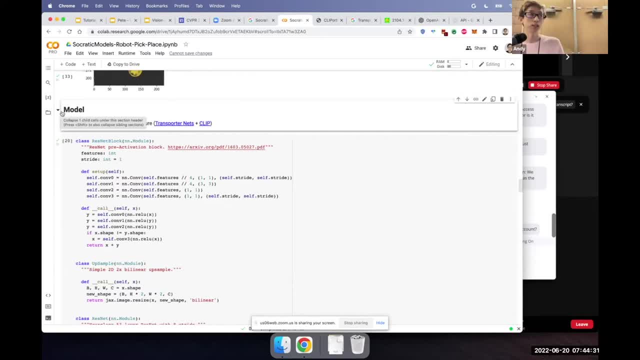 we'll be talking about limitations of the stack too, later in the talk. So if you're interested in what are interesting research questions that people can tackle using this Colab, then I think we'll go over that a little bit later, But for now, in the meantime, 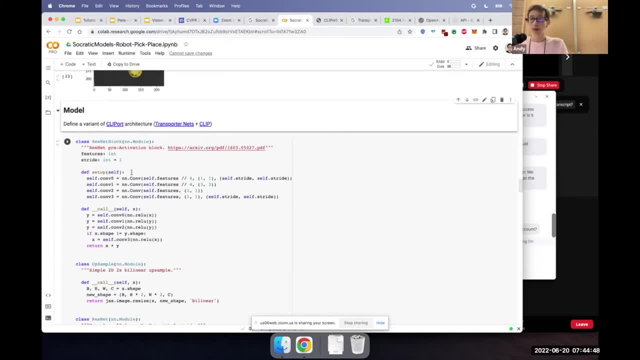 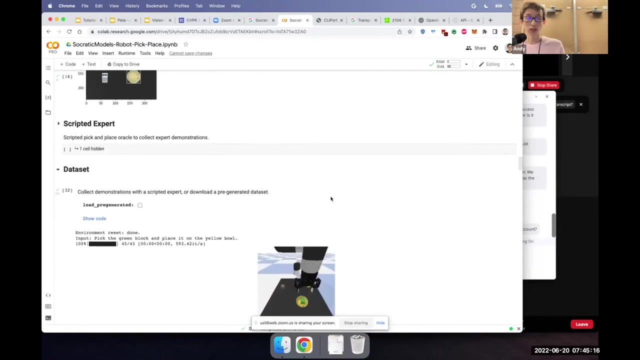 we'll just sort of go through the rest of this Colab. Any questions so far? Yeah, Hi, So How I generate the Yeah, Yeah. My question was: how did I get the 10K demonstrations? that was on a local PC. 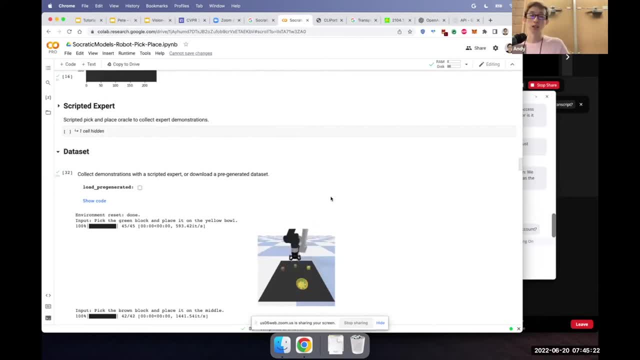 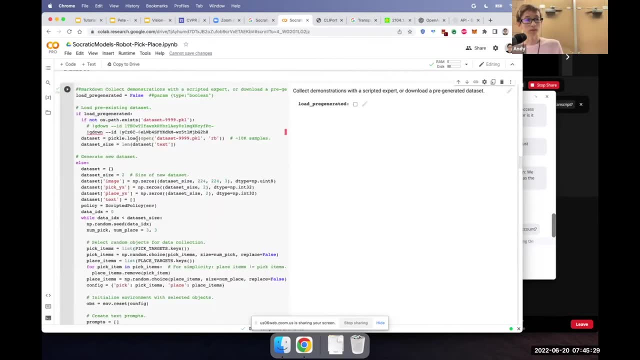 and just running it for a couple hours. You can also do the same here in this Colab too. So if you go ahead and Up here, So uncheck the load pre-generated and then set your data set size to 999.. Oops, 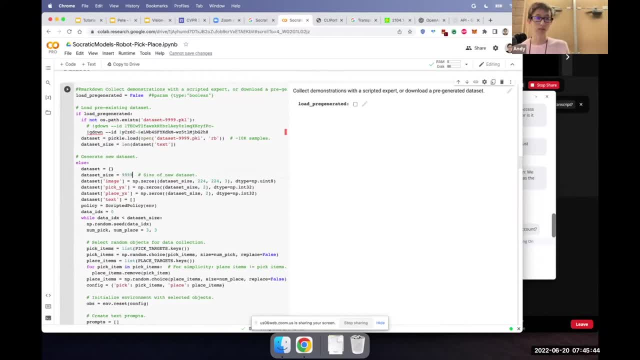 And, Yeah, You'll get the similar data set In general, something like clipboard which takes into account the textual command and outputs to pick in place if you want to generate. The more data that you have access to, the better the model becomes. 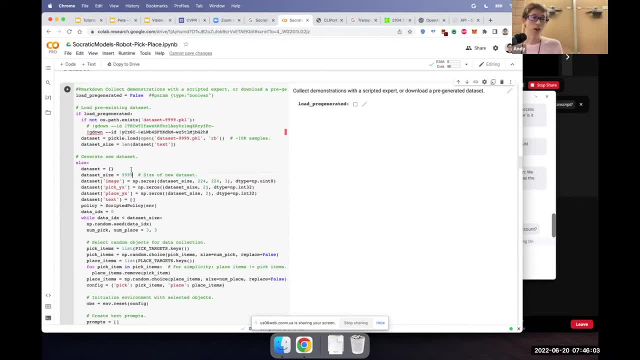 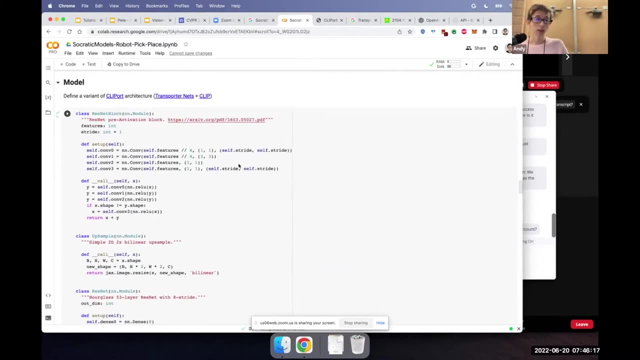 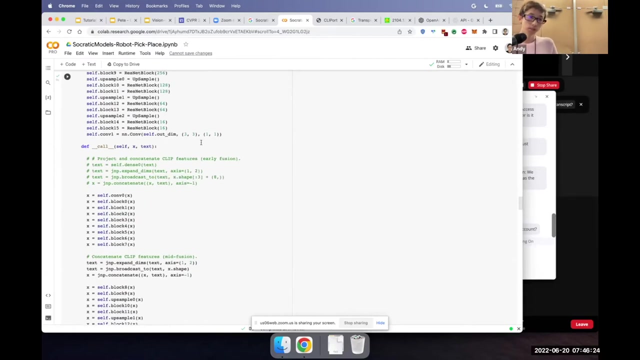 So 999 was just on a whim. We wanted to generate enough data in an afternoon, but you can increase this to 100,000 and I'm sure it'll be better, Okay, Okay, In the model side we have an architecture that is. 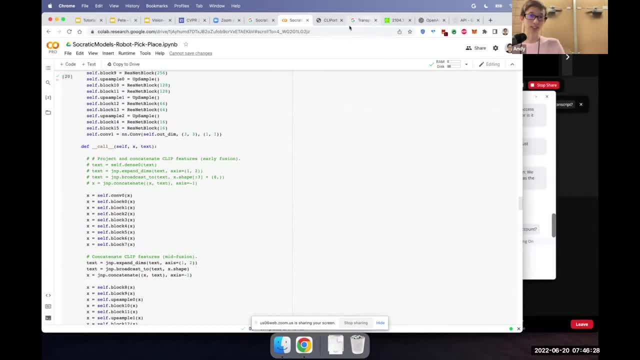 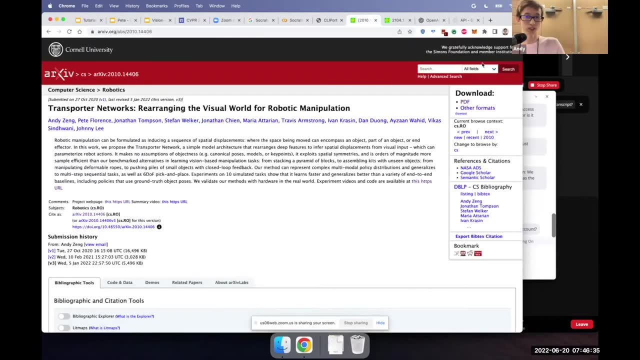 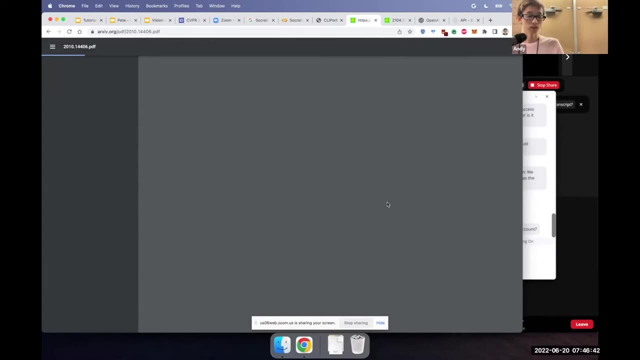 So I guess, to provide some context, there's a bunch of con blocks here, but let's just go into the paper for TransporterNet so that we can go over what the pipeline is really doing to do pick in place. So I'm gonna go ahead and get started. 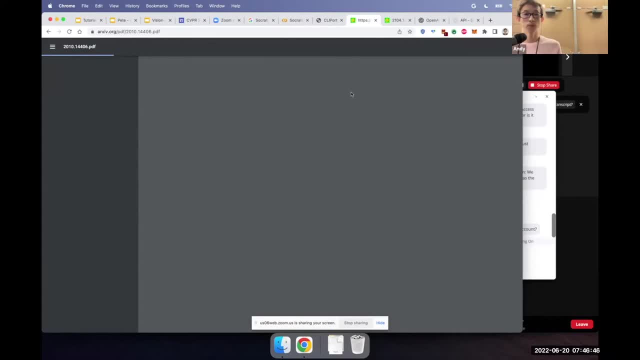 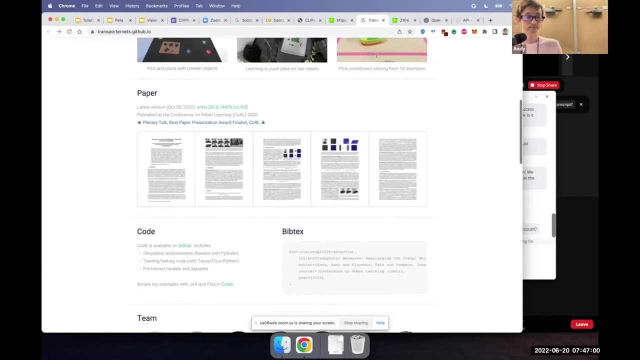 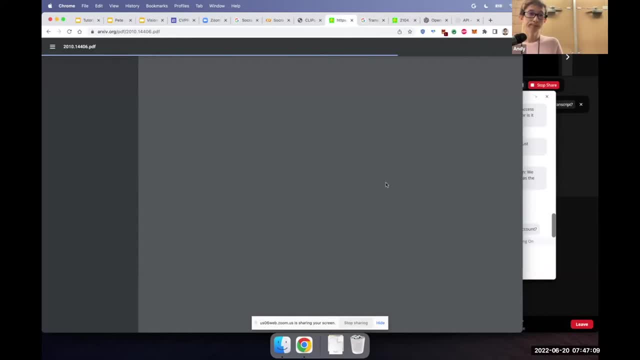 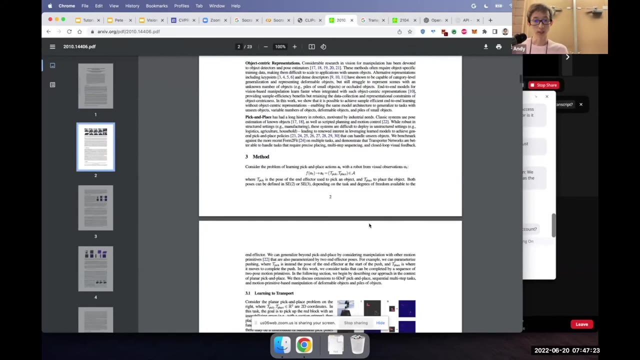 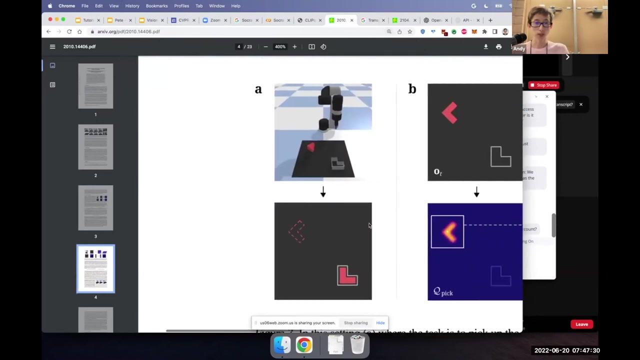 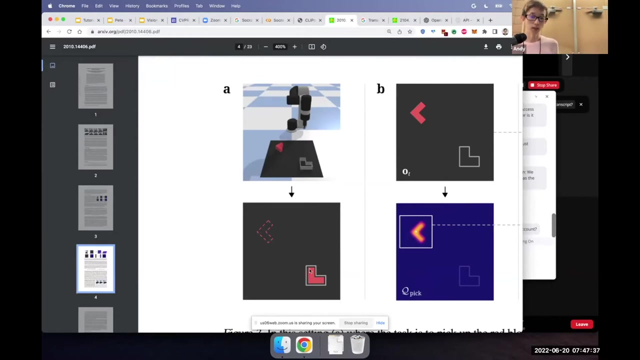 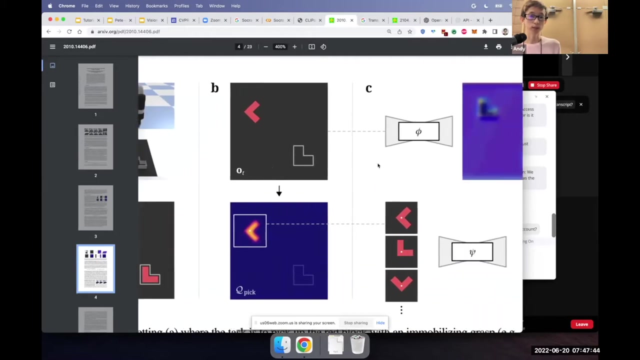 so so, so so Okay. so the key thing to look at is this diagram: Suppose that you have a system and you wanted to put the block and reorient it into the correct spot here in the fixture, Specifically what the pipeline does is. it takes this top-down view and it feeds it into 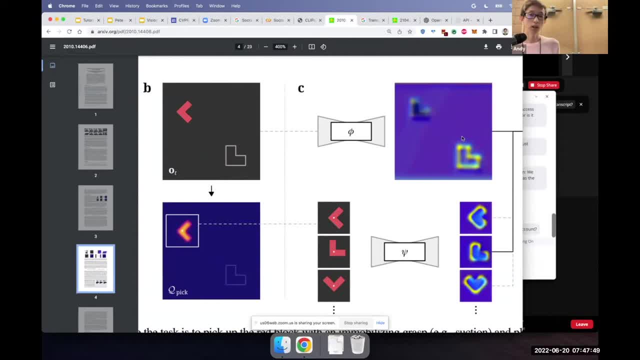 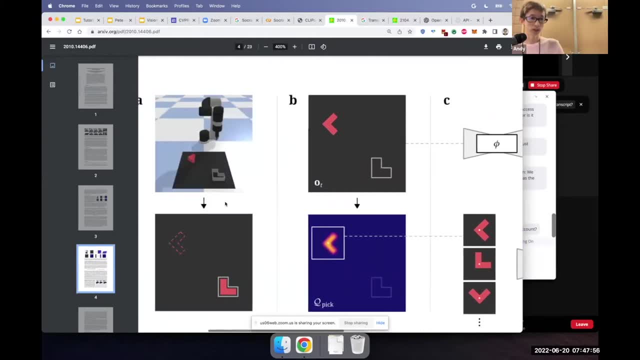 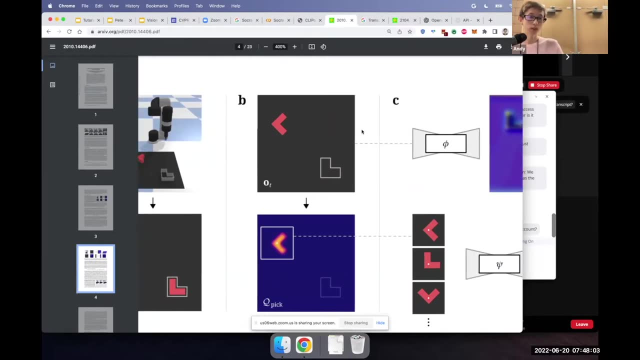 a fully convolutional network to compute dense features And we visualize the dense feature here, And this is specifically right before this. we also have a similar network architecture to this first part. here that predicts a picking location or how the system would grasp a. 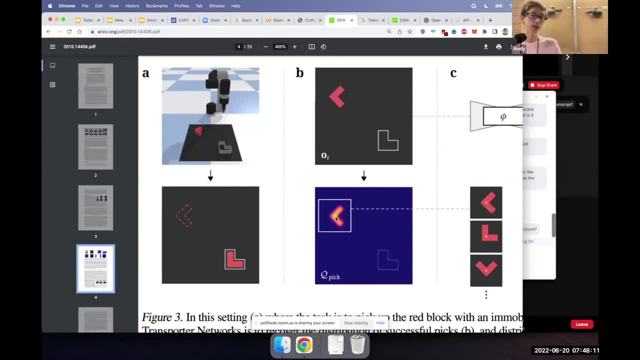 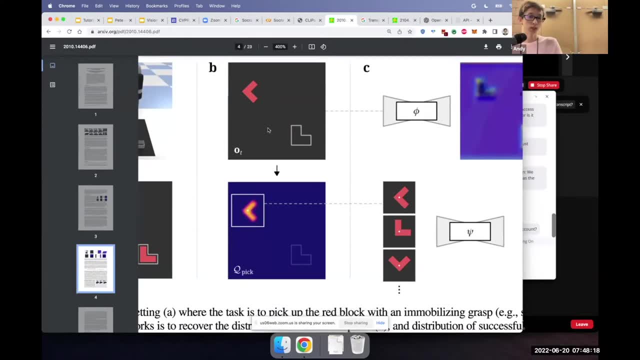 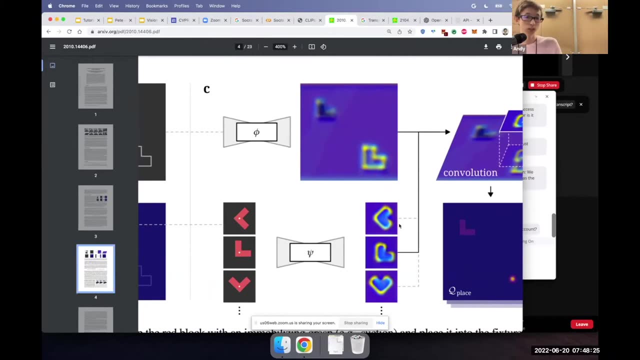 object And suppose that it predicted the center of the object. So what the transporter network does is it crops out this local region in the input image. It, for example, rotates it in various different angles and feeds it into another, fully convolutional network to generate dense features. 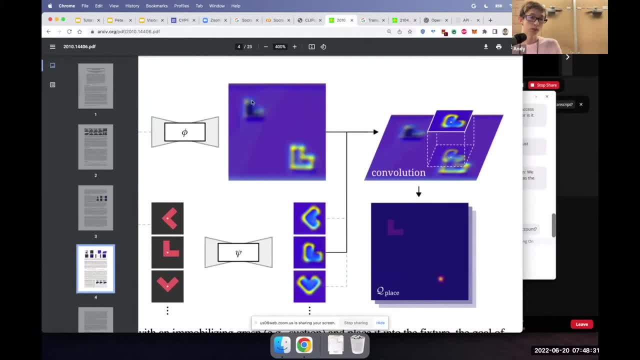 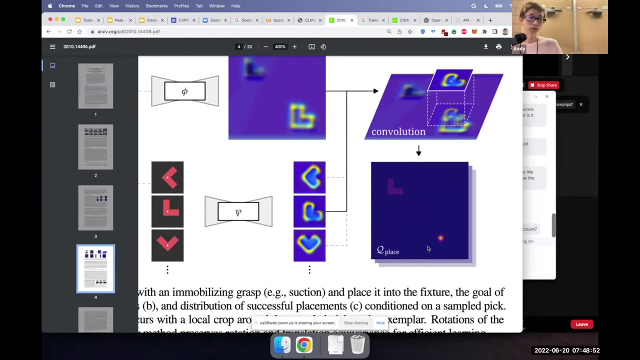 And then you apply a cross-conf on the crop over the placing features. This is in a sliding window style fashion, So ideally the object that's correctly oriented on top of the fixture sort of generates the highest cross-conversational values. And ultimately you generate this single image plane of logits and you can match that against. 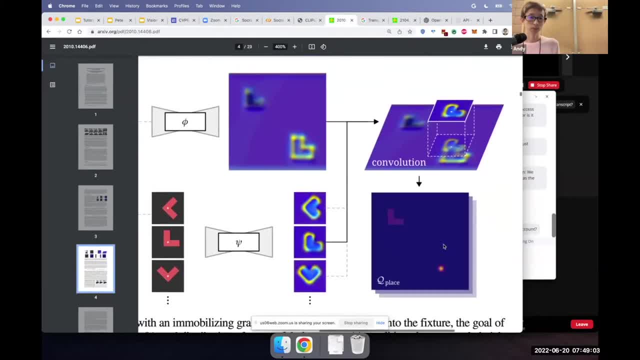 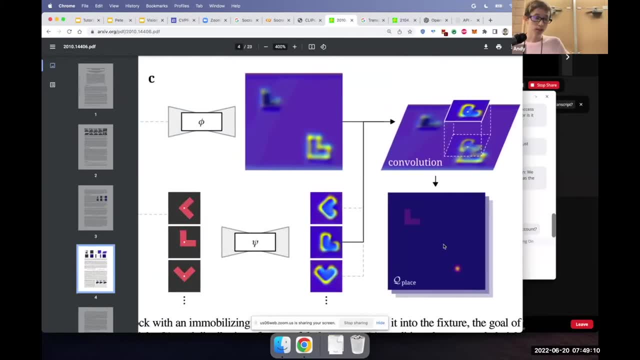 a one hot pixel map with cross-entropy. So that's it, Thank you. There's a lot of nice benefits to this in the sense that, although so, there's interesting nuances in the sense that when you're doing robot pick and place for every possible input. 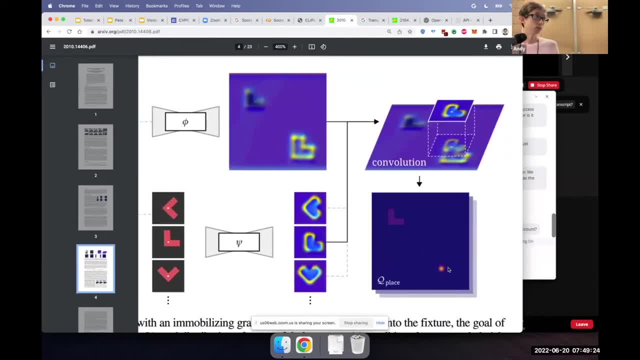 image that you have, you only have one action that was really executed by the robot. So if you were learning from demonstrations, you really only have one pixel. But what's interesting is that if you have a lot of training data, You can actually get these things to also reflect multi-modal distributions, which is 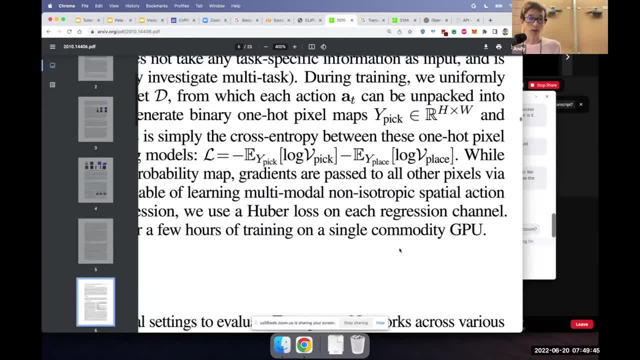 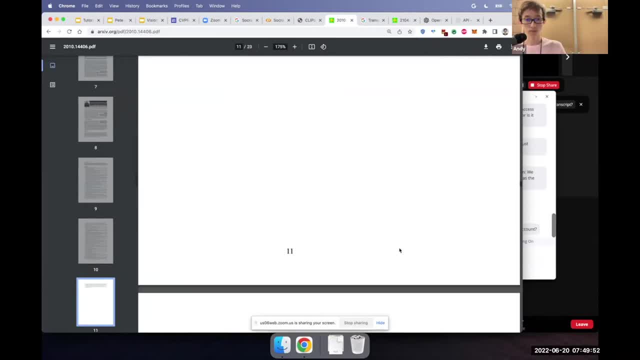 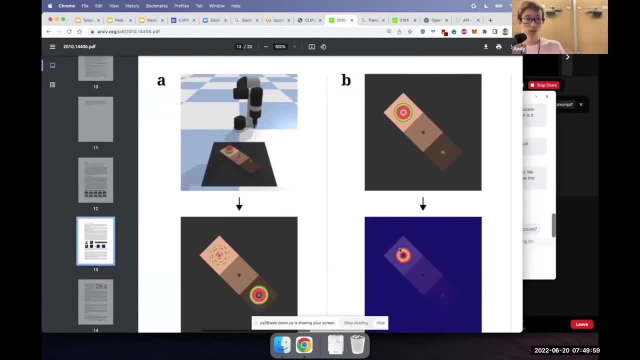 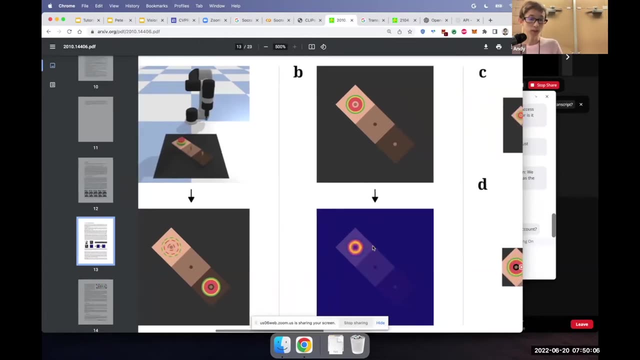 what we're really after. So a couple examples: for example, you can have picking locations that are located all around the disc And it's, Okay, Pretty cool to see that picking spots would generally be highlighted around the disc. And this is just if you. this is also. there's a couple of things at play here, but another. 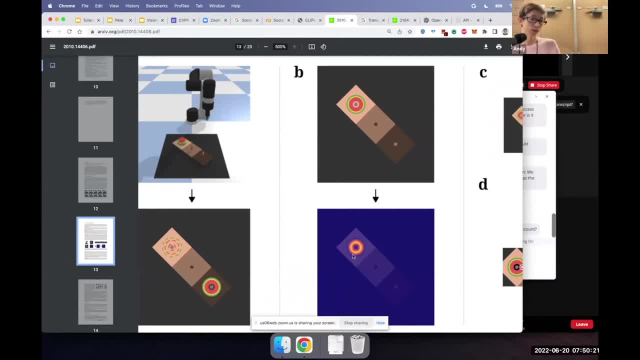 thing that one part is particularly the loss function, but another part is that there's inductive biases that are at play, because this is a fully convolutional network. then you have this spatial prior. So for example, here it's likely using red pixels, for example, as a way to figure out. 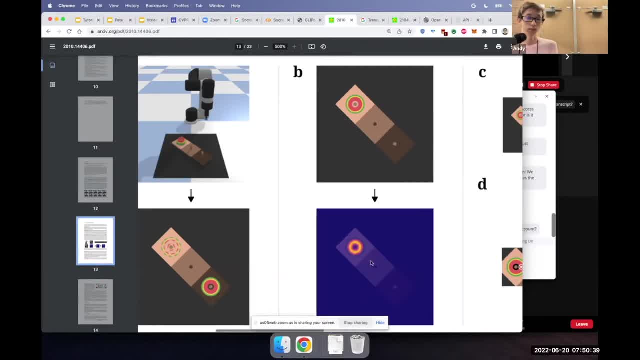 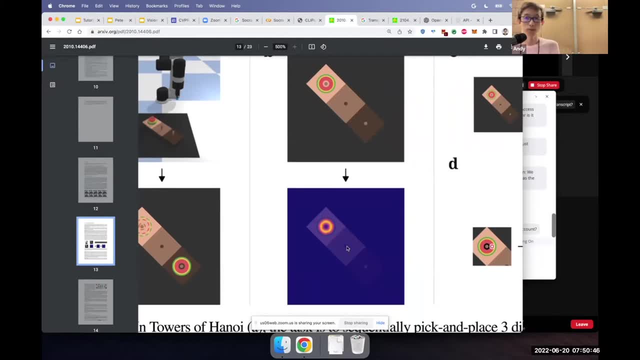 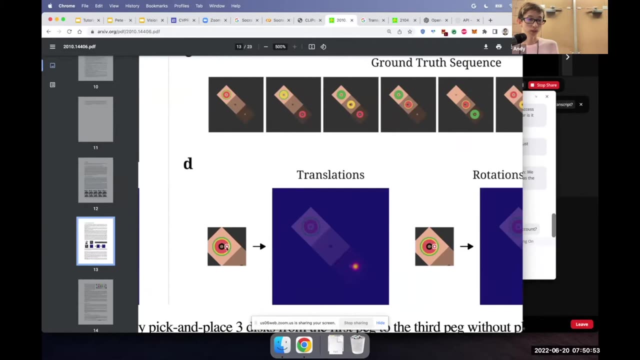 that All the pixels that belong to the object. So this is good for grasping, because all of those are valid grasps with a suction cup gripper, And here this just shows that if you, for example, at least with transporter nets, if 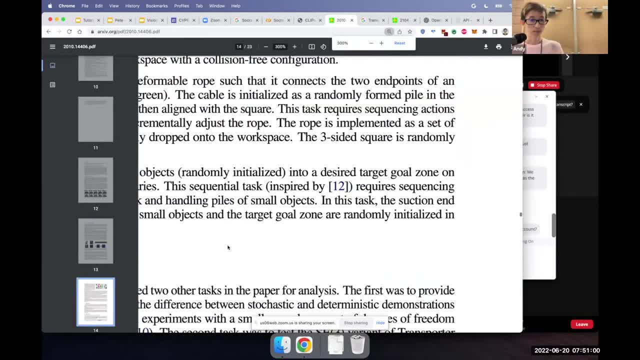 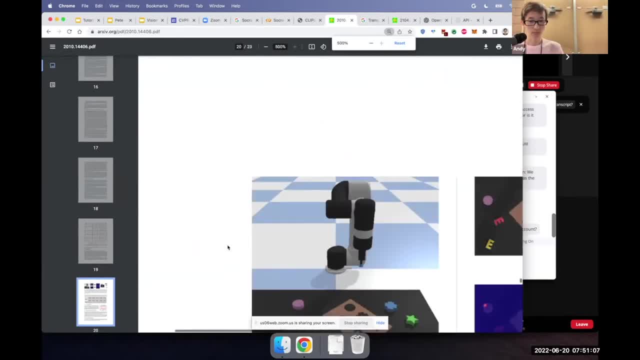 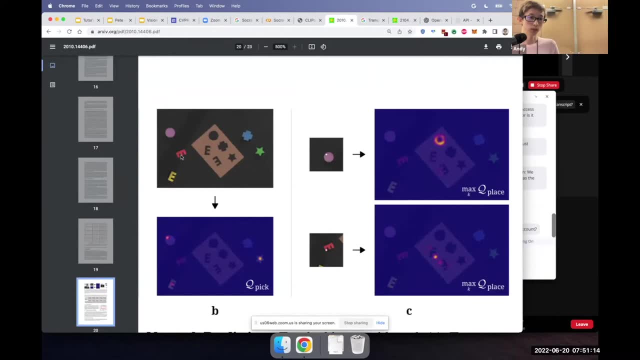 you're pick condition placing. see if I can find a better visualizations. Okay, Okay, Okay. So what this shows is that say that the task was to take the E shape block and put it into two target V shapes. The last function can correctly encourage two spots that you need to place the object. 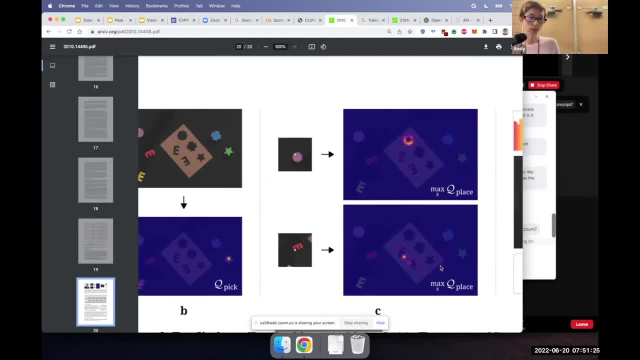 that. So that's just a byproduct of both loss function and the spatial biases. Similarly, if you are, it's subtle, but if you grasp an object by that's off center, for example, Okay, So that's just a byproduct. 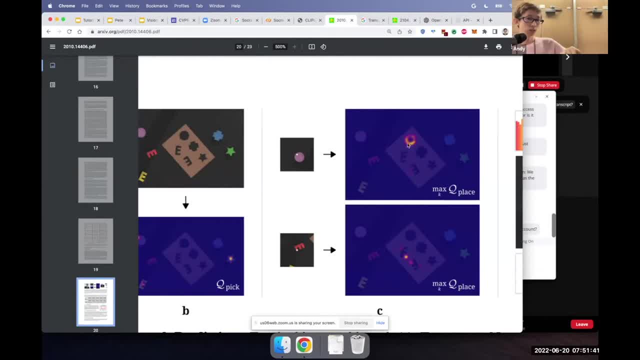 So it's actually a disk, So the way that it was placed is that basically it's located on the edge of this disk. Then the way that you place it actually needs to be sort of different Each time. you kind of have to orient it correctly, and also translated respectively, so that 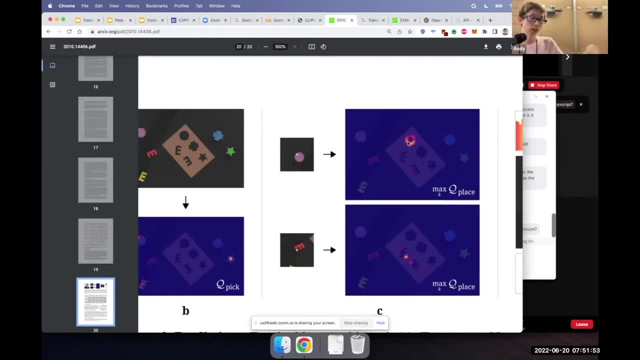 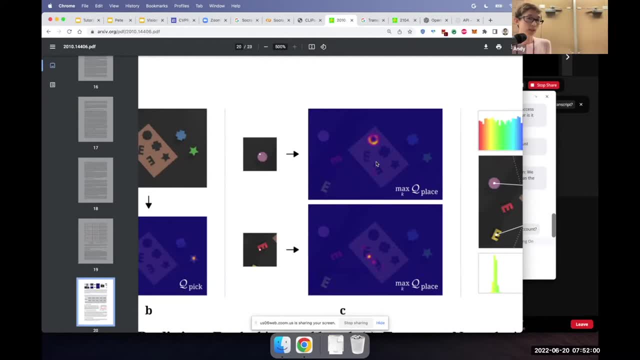 against the edges of the whole of the kit here. And what we're showing here is that across all the rotations, if you take all the heat maps and you collapse it, you form this donut shape. But if you expand it back up and you imagine that it's sort of 2D heat maps, which mean 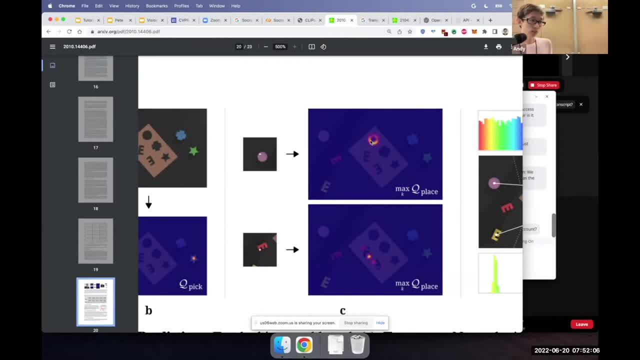 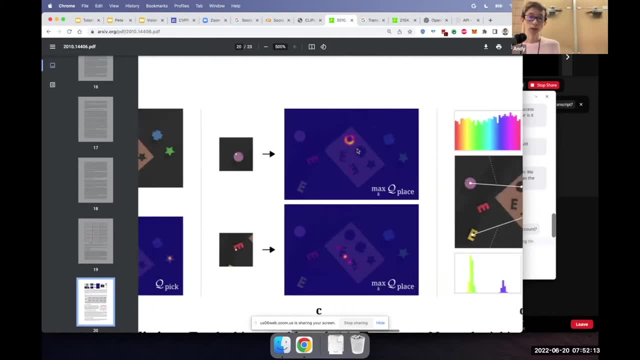 that you can't turn it like that. You can't turn it into a knitting shape. So that's part of the reason of 2D heat maps with a rotation at every layer. then it forms a spiral in that 3D heat map in SE2.. 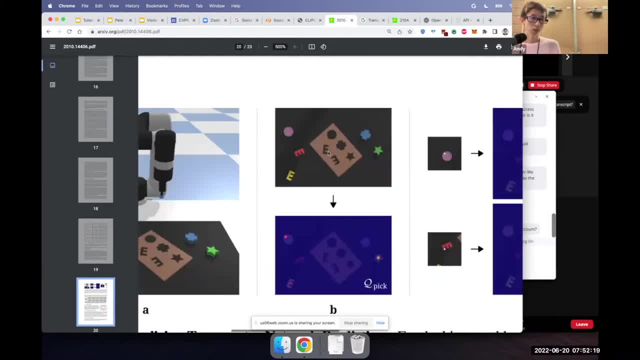 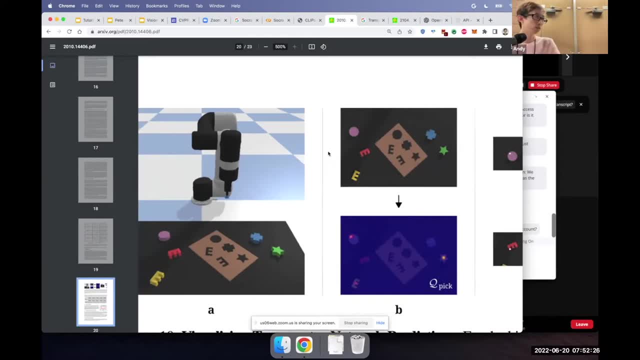 So that's just to show that these systems are pretty good at learning multimodal distributions, And I think that in general robot actions, there are always so many different ways to do the same thing, And making sure that our policies can reflect multimodality is actually very important. 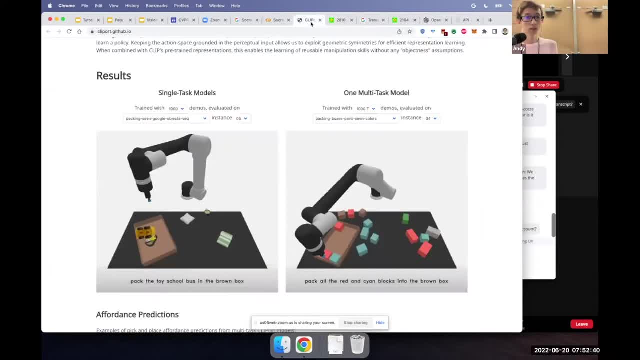 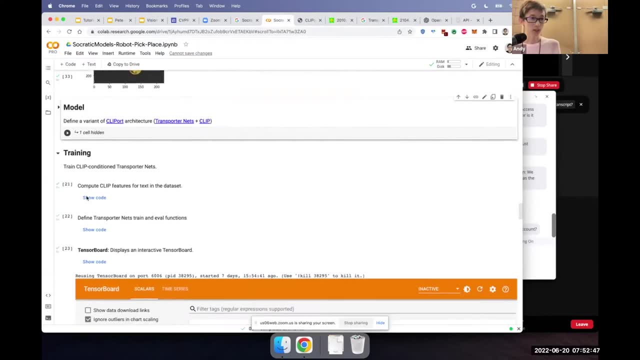 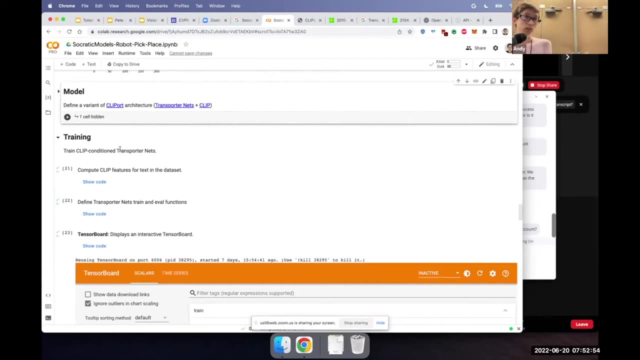 for robot learning. Okay, so that was a quick spiel about the transporter nets architecture, And what clipboard does is that it broadcasts the clip features of the text and brings that into all of the layers inside transporter nets, And that's exactly what we try to do here. 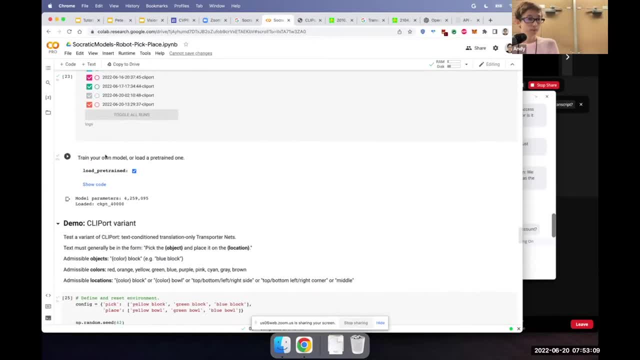 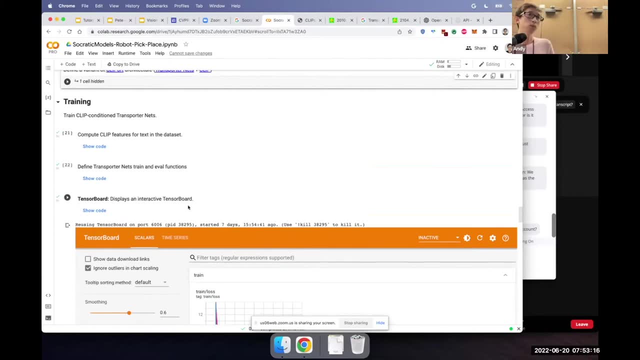 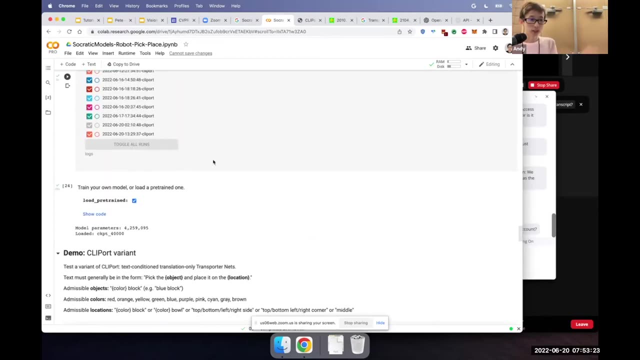 and we try to train it over time. One thing to note here is that this architecture that we have in the colab here is similar to clipboard, but not exactly the one that clipboard has. So yeah, just a heads up. So there's a tensor boards to sort of track training over time. 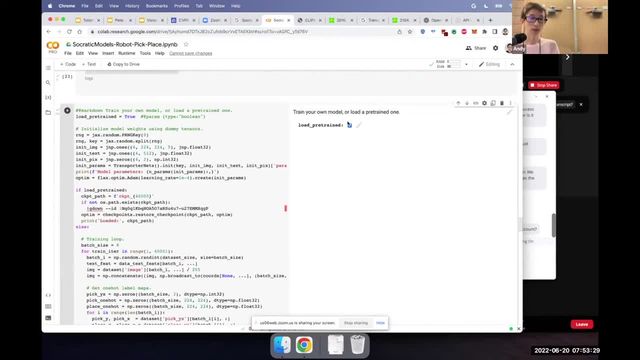 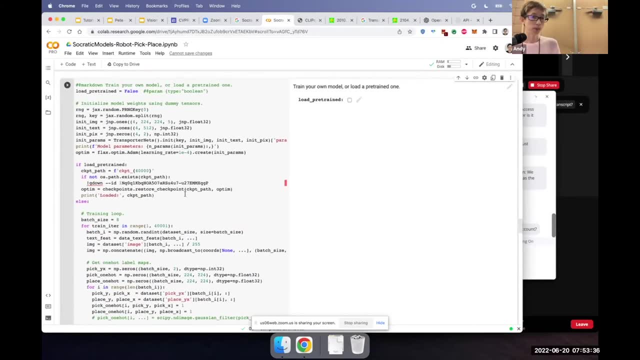 And if you want to train your own model, then you just take this and then it'll. it'll run through, it'll generate batches of eight And it actually requires quite a bit of memory to train. So batch sizes are not. 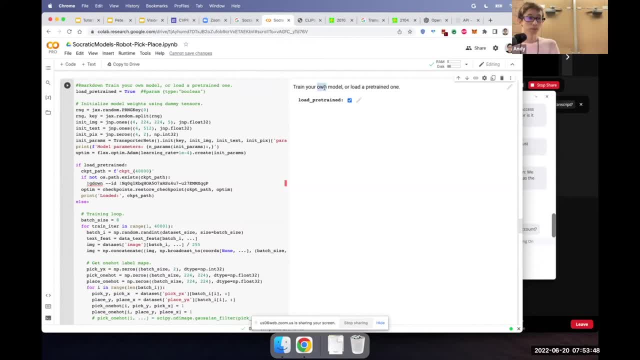 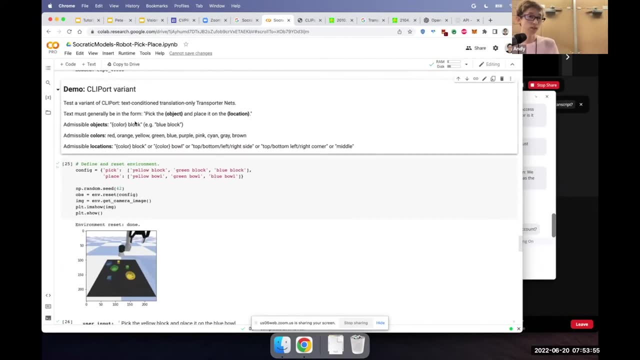 very large. So here is a demo of a trained clipboard. So we already have that loaded in memory. So, yeah, this is a demo of a trained clipboard. So, yeah, this is a test variant of clipboard text. condition: translation only transporter nets text must. 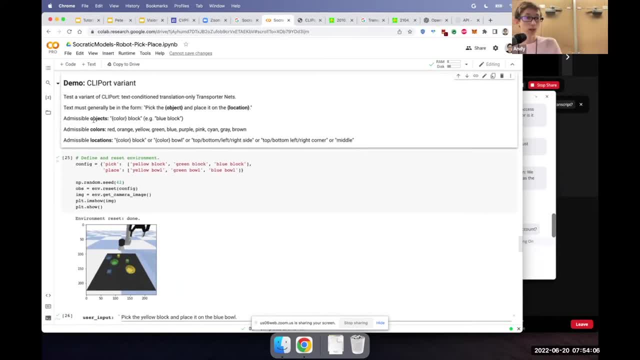 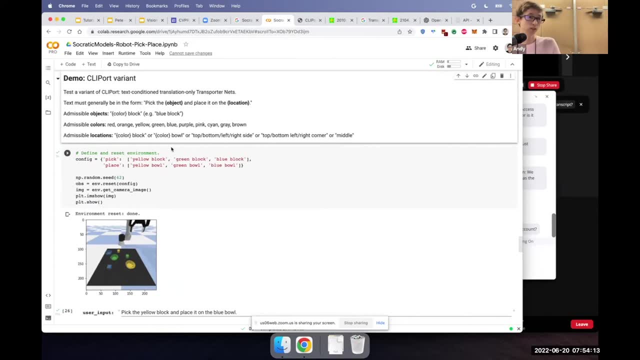 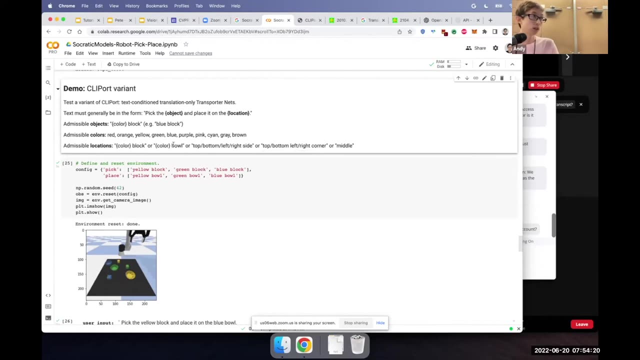 generally be in the form: pick the object and place on location. admissible objects are the objects that you've defined up in the top of the config and also the objects that have already been trained in the training set and admissible locations, so at least in the simulator, the scripted demonstrators. 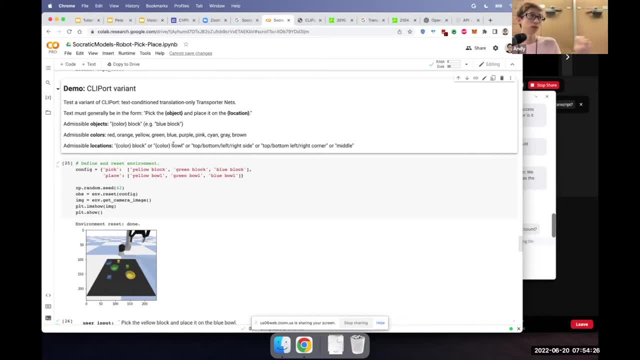 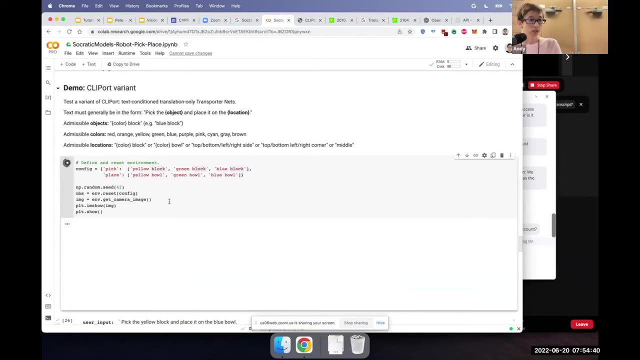 also have done things like put the block in the middle or put the block on the side, put the block on the corners, so that's to the extent that the placing locations are also spatial locations. so there's some training data for that in here too. yeah, so ultimately you can define and reset the environment and then you can ask it to. 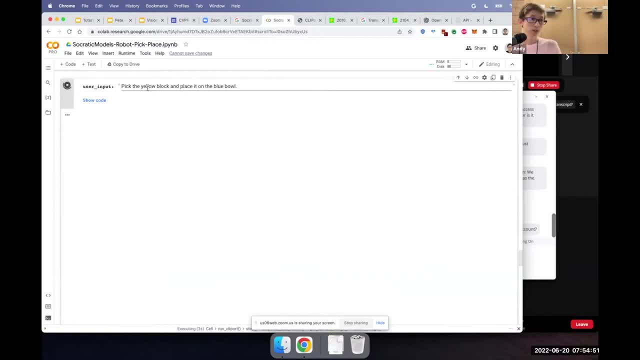 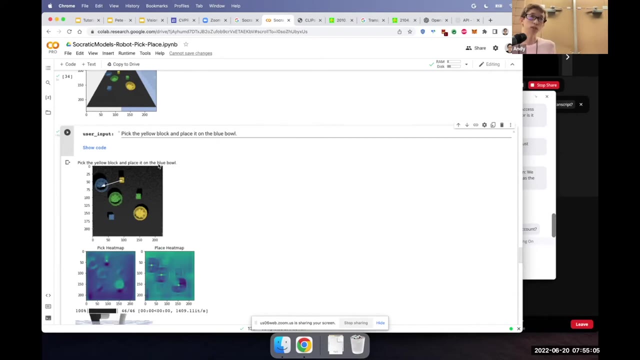 execute some of the things that it's seen before. so this is a testing scene. so let's see here. the system will execute the pick and place and then it'll try to generate a bunch of visualizations so that you know what's happening. um, first and foremost is generating 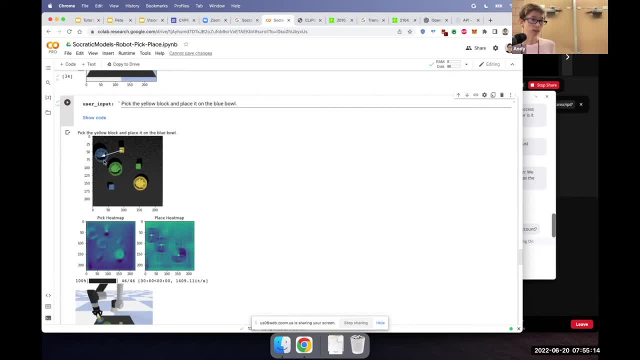 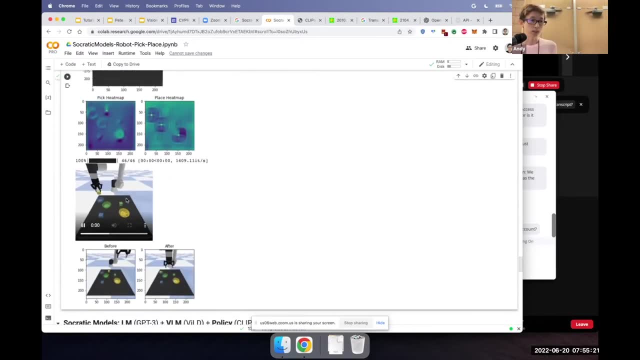 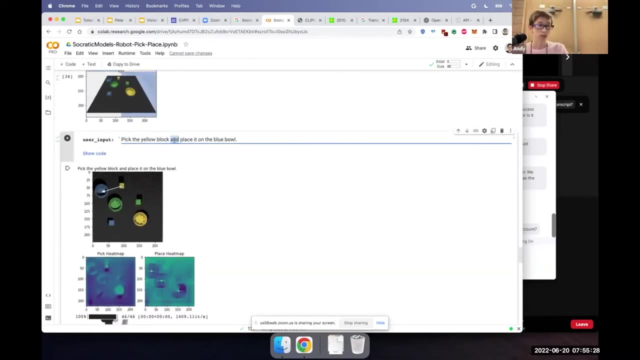 what the robot thinks it did, that's, executing a pick here and then a place here, the picking heat map and the placing heat map as outputted by transporter nets, and then executing the actual actions and a before and after image, And then, without resetting, we can subsequently add ASCA2.. 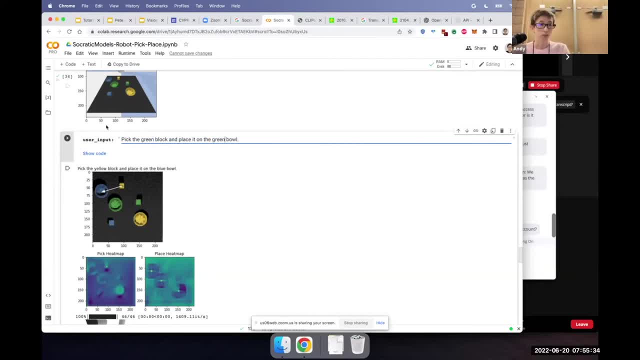 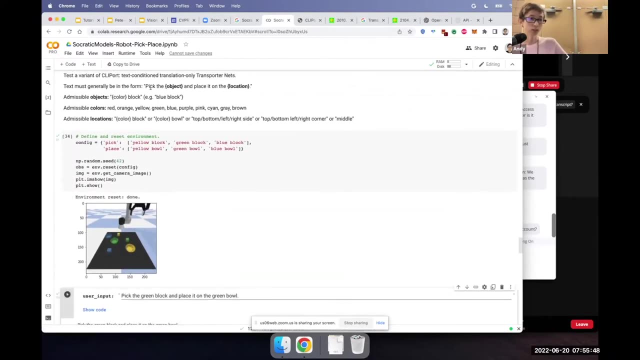 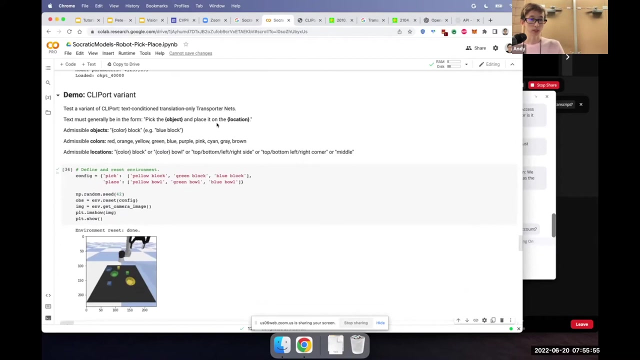 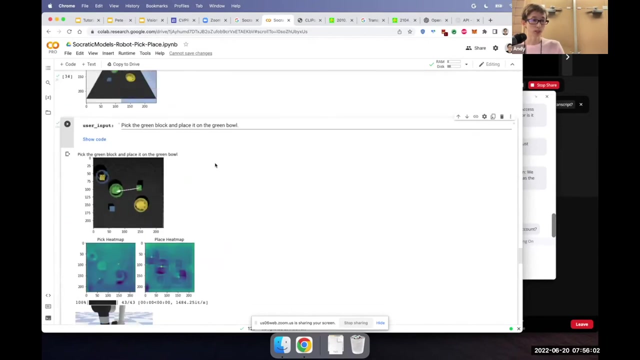 Put the green block, place it on the green pole And note that the text instructions have to generally be of the form Pick the blank and place it on the blank. And that's just because that's what Clipboard has been trained on. Yeah, so it executed the correct pick and place action. 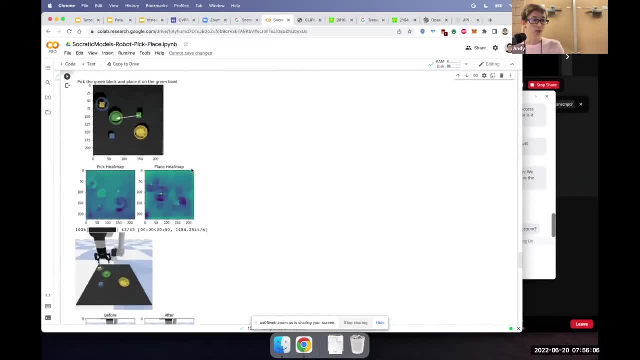 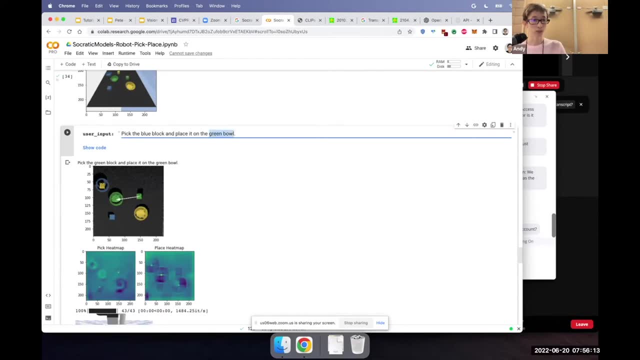 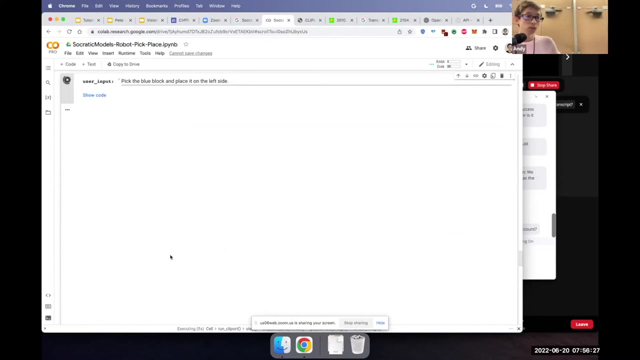 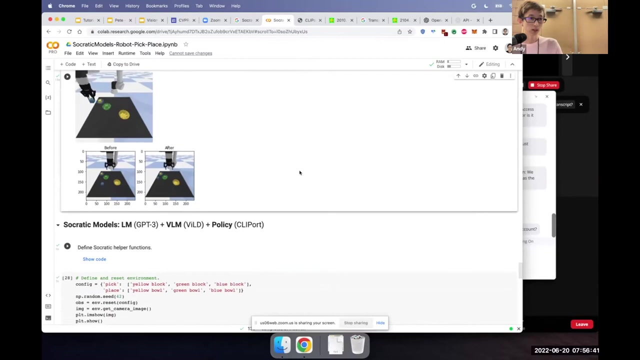 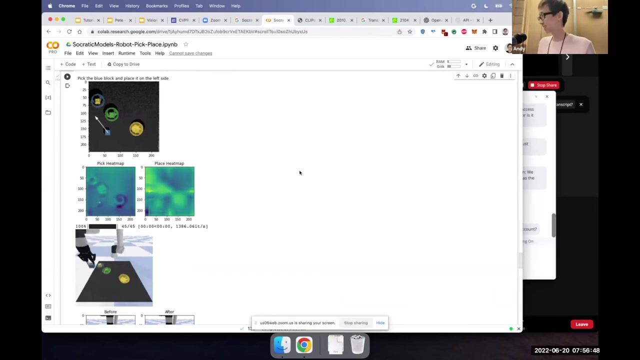 And now let's put the blue block and place it on the left side. Cool, so it looks like it did that. All right, so I guess yeah Would be to call out like what it can't do yet. Yes, Because we have like four minutes until coffee break. 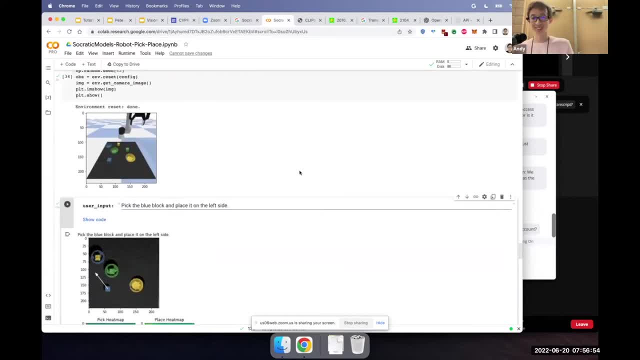 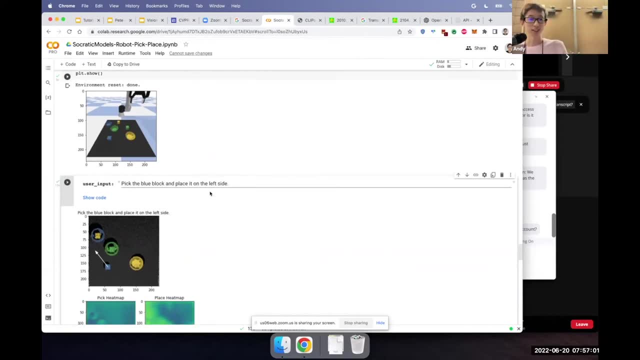 Yeah, And then we could suggest people to train their support models if they want. OK, And then we could do it more on like bell and stuff. at the end Sounds good. If you want an option, Yeah, All right things. that it can't do a great suggestion. 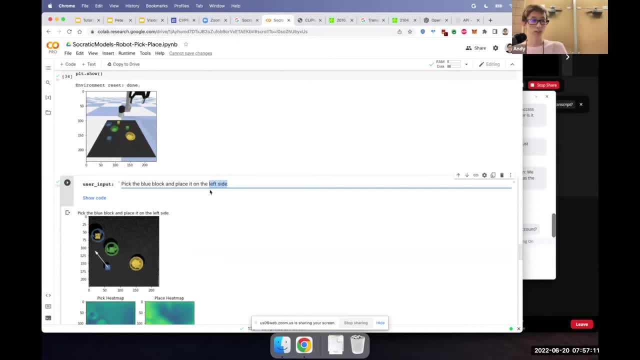 Pick the blue block and place it on the. Or like undo, Would you call, pop up on the blue. Yeah, on top of another block works, Yeah, undo, the last step is definitely not going to work. So undo, the last step. 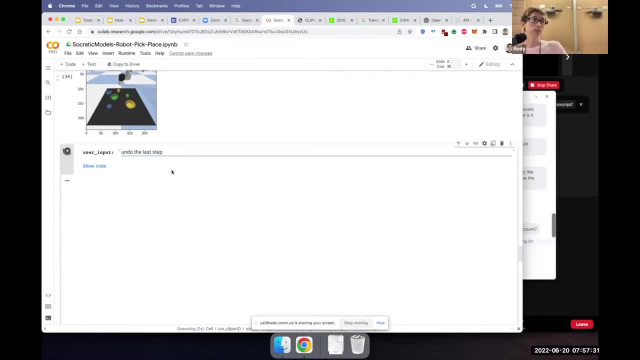 And this is with clipboard only, So it's not using a GPT-3 to translate commands into things that clipboard knows. So if you just straight up fed the text, the model can take it in as input, but it won't know how to undo. 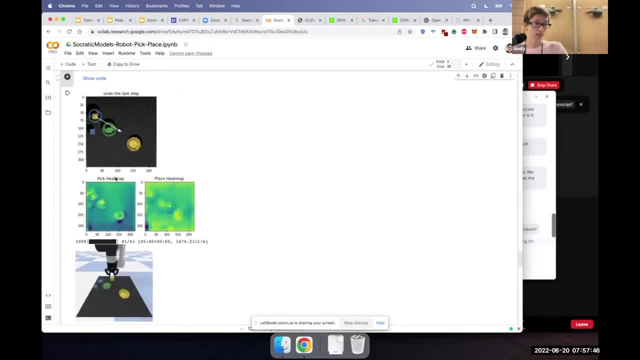 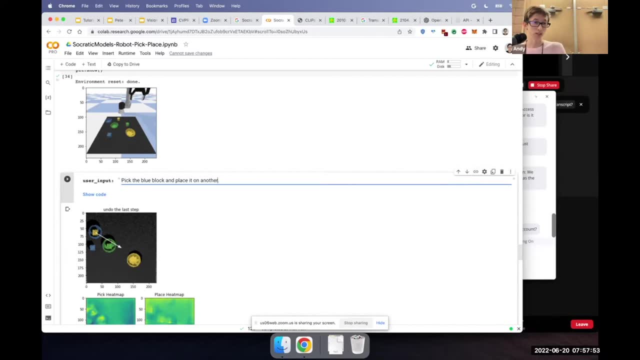 So it- yeah, it's just picking out the yellow block. I guess, If you also put decide to put in words, though, that you're not going to use the words that it doesn't know like: Oh yeah, that's true. 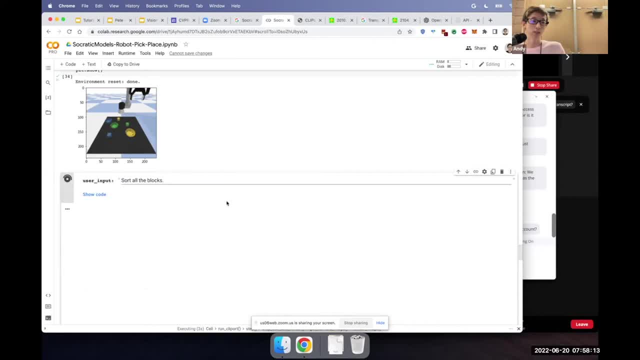 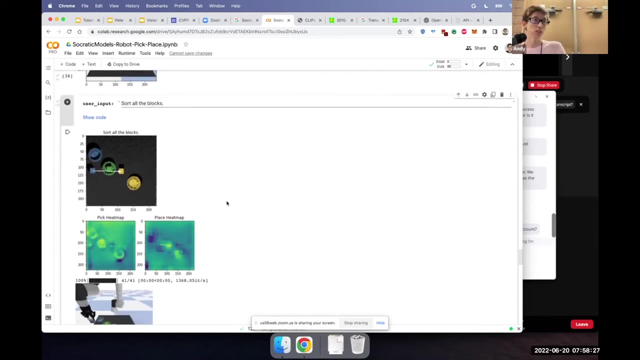 Yeah, so just out of the hard constraint that it can only execute one pick in place from the textual action sort all the blocks without GPT-3 is not going to work, Unless maybe you've trained clipboard to actually recognize that command. But that might take extra data generation. 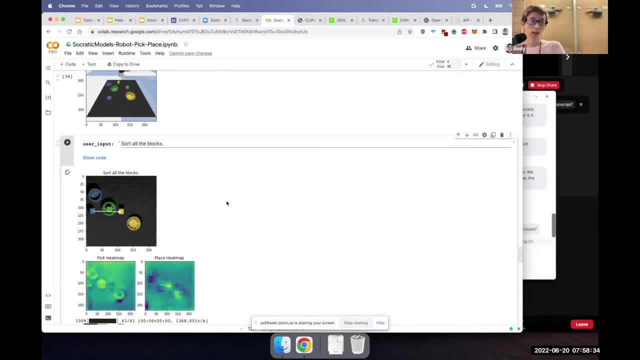 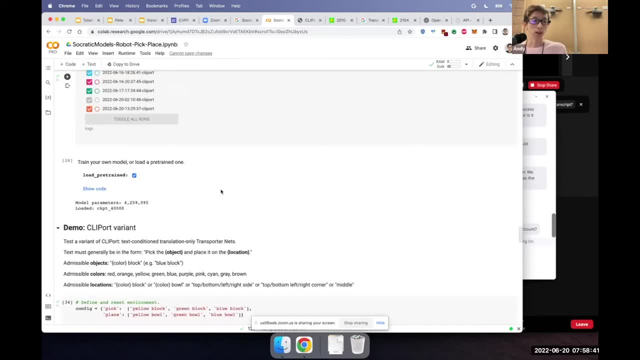 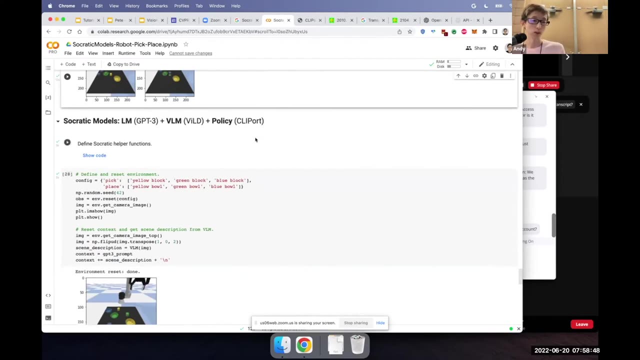 Yeah, so it's just stacking blocks, which is not what we want. OK, so these are things that clipboard on its own cannot do, And later we'll get into why combining it with language models, VLMs and policies can get it to work. do some of the undo and sorting tasks. 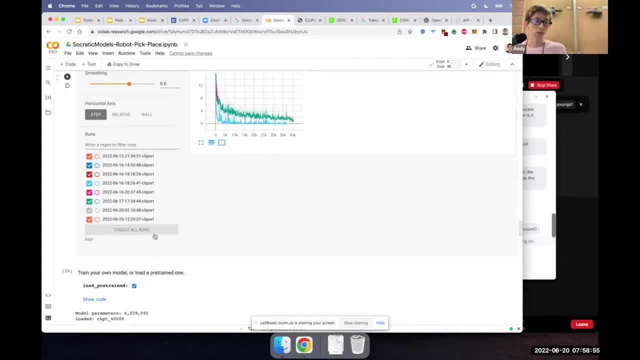 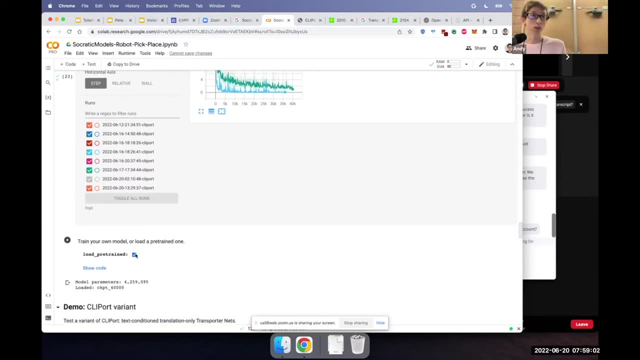 And then for now, if you want, you can do that, Since we're going to have a sequence of talks throughout the rest of the tutorial, you can also go ahead and train your own model too. It'll take a couple hours, but hopefully by the time that we're done with the 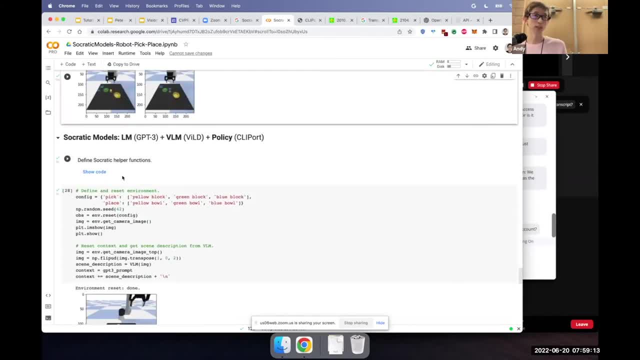 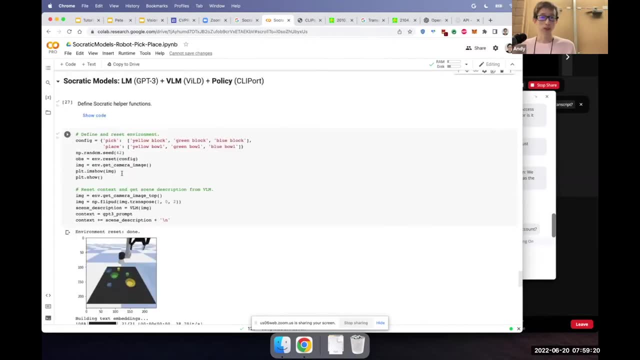 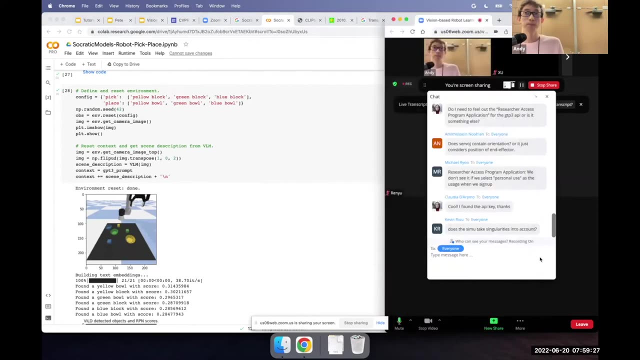 get to the point where we're going to talk about the language model stuff, then you can ideally be able to run with your own trained model. Yeah, so I think we can let you go on your coffee breaks. Yes, same questions. Any additional questions from the crowd? 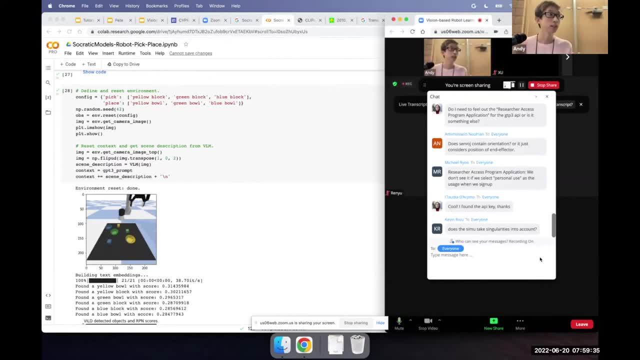 Yeah, That's a great question. The question was how much of this tutorial is inside Colab. You can copy Paste this entire thing into your own Python script and just run it on a local machine with a GPU, and it should work as well. 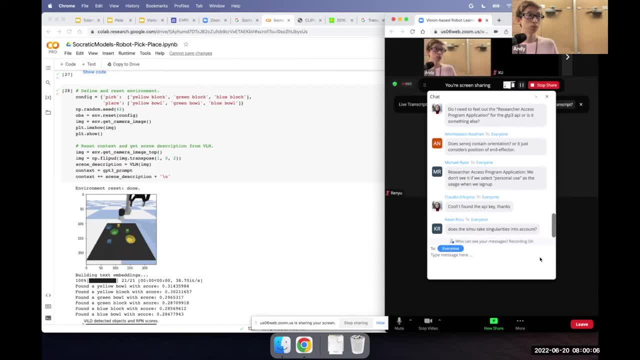 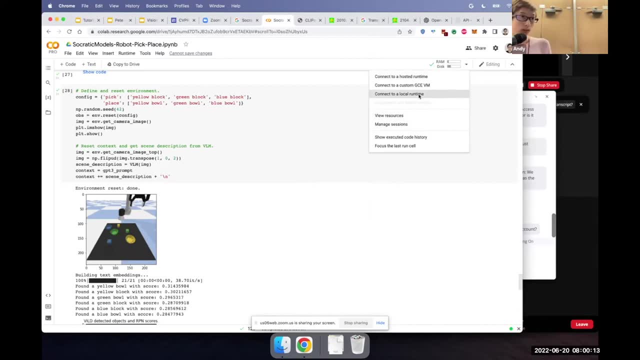 And I think that you can also use this in the style of Jupyter Notebook. So, up here, if you say that instead of connecting to a hosted runtime, you connect to a local runtime, then that's essentially doing Jupyter Notebook And that's how the video was recorded. 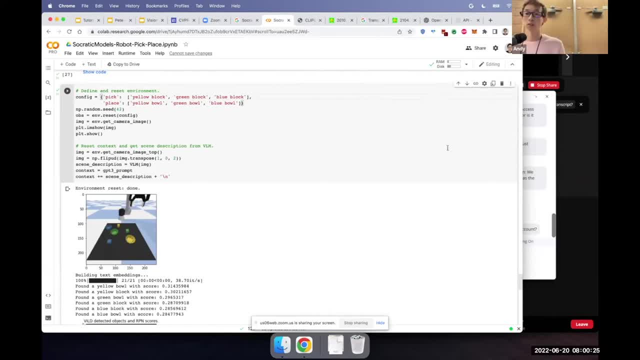 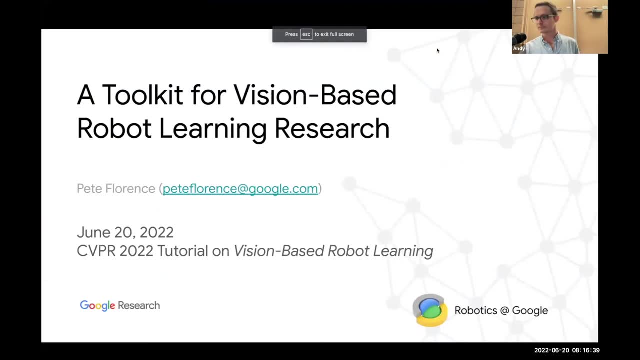 Any other questions? OK, cool, So we'll see you back after the coffee break in 15 minutes. OK, Everyone can hear me here. Can we just check that it's streaming online? It looks like it. Cool, OK, great. 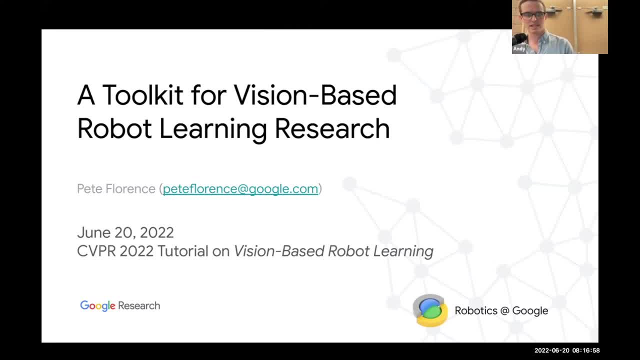 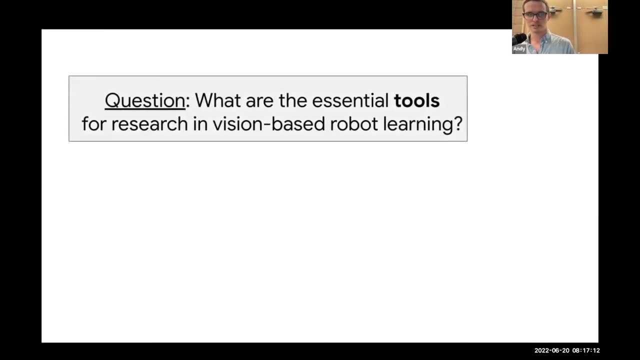 Thanks everyone for coming back And we're excited to keep going here. So my name is Steve Florence. I want to talk today about a toolkit for vision-based robot learning research. So what do I mean by a toolkit for vision-based robot learning research? 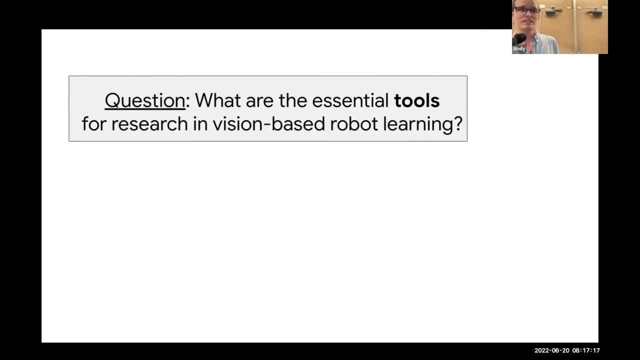 The question that I'm putting forward here, I'm going to try and take one shot at an answer with, is: what are the essential tools for doing research in vision-based robot learning? And I'm going to try to connect some of these ideas back to the Colab that we've been working on. 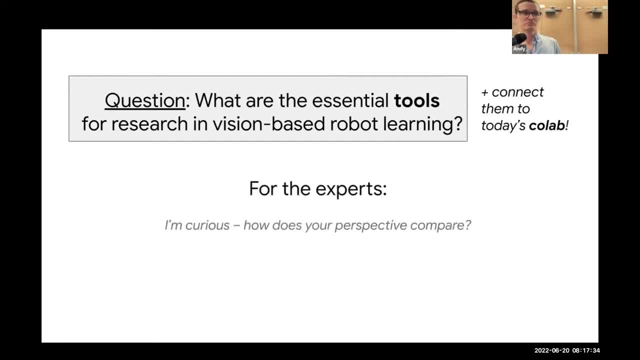 Looking at today For the experts in the room, I'm genuinely curious. Maybe you already know all these things, But in terms of the way that I'm going to try and put together what is kind of the short list And what's the relative emphasis on different things, 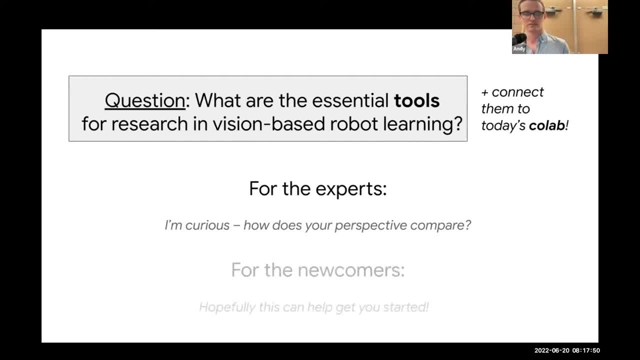 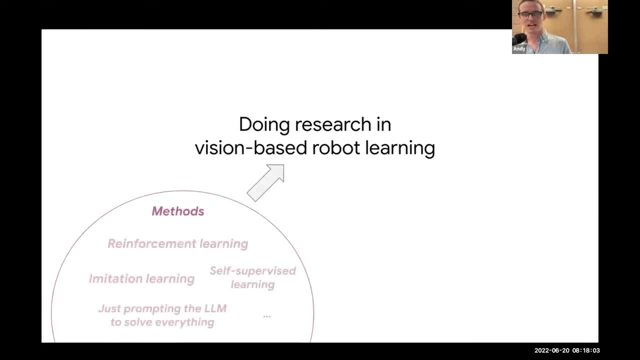 Thank you. So doing research in vision-based robot learning, I think what the majority of the emphasis is often about is with the methods, So the reinforcement learnings, the imitation learnings, the self-supervised learnings, or just prompting the LLM to solve everything. 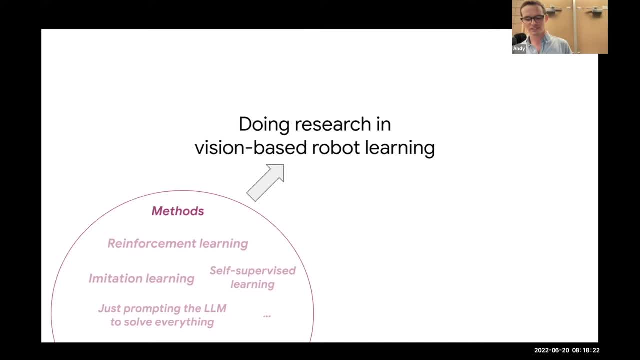 Whatever it is, whatever the method is that you use. these are the things that I think we talk about a lot, And there's all this other stuff which all come together as tools, which are sort of agnostic to the methods themselves but I think, are incredibly. 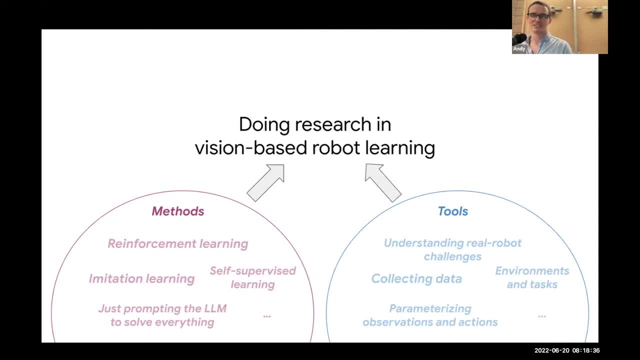 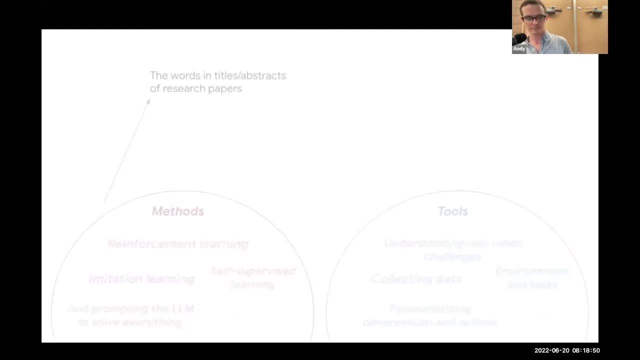 important in sort of actually making robot learning research work. They're sort of the behind-the-scenes heroes here of robot learning research. things like understanding real robot challenges, collecting data, environments and tasks, things like that. things that are agnostic to the methods. 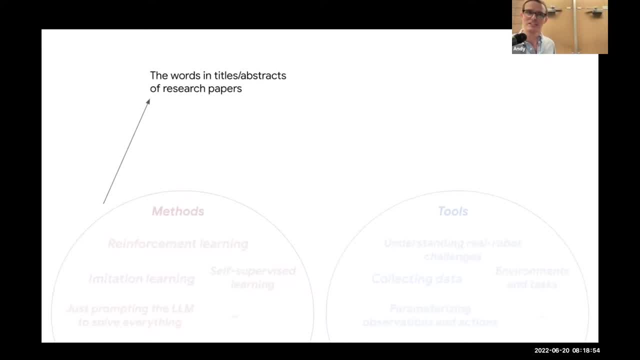 And I think it's the methods that they often get a lot of the glory. And they're the words and the titles and abstracts of research papers And they're covered ad nauseam, And they're your formulation and method sections And they're the key ideas that we talk about. 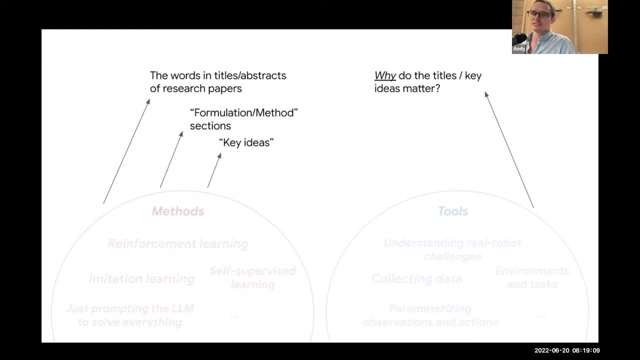 But it's often the tools, I think, that inform us. why do the titles and the key ideas matter? They also explain the reasons why things can come together so quickly out of productive groups of people, And they power the experimentation that shows that things work. 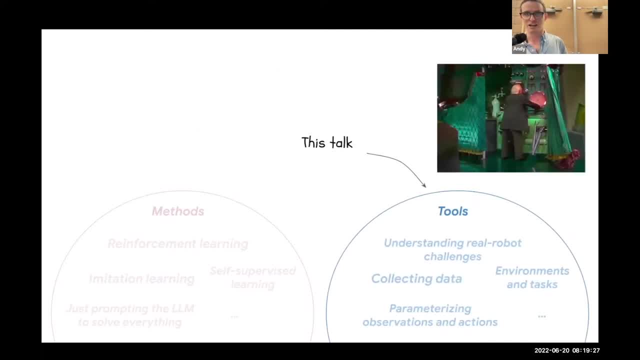 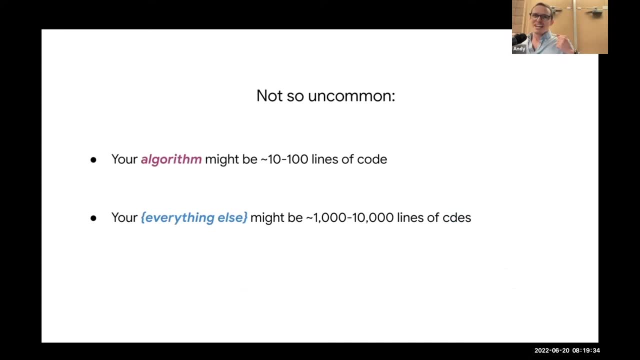 So this talk is going to be about the tools, And for those of you that know The Wizard of Oz, I sort of feel like it's like the man behind the curtain here. So I think this is actually pretty common, though not so uncommon that you might end up. 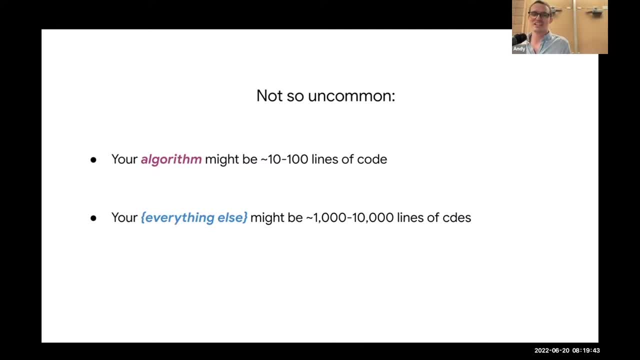 in a situation where this is just a little bit more motivation here. Your algorithm might end up being 10 to 100 lines of code, maybe in that range. It's fine if your algorithm is more, But it's legitimately a thing I see often. 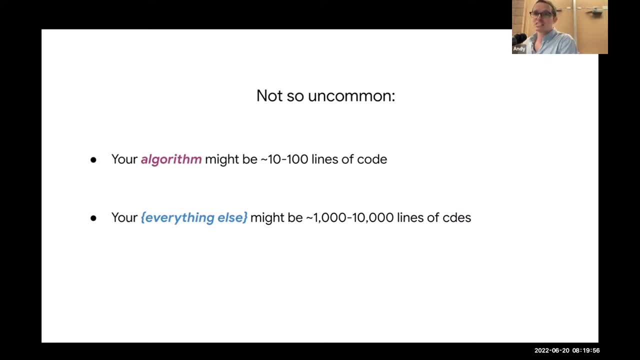 where people's algorithm is tiny, But then your everything else could be orders of magnitude more: 10,000 lines of code, whatever it is, And I actually think this is totally true for the co-op we're looking at today in terms of kind of at the end there. 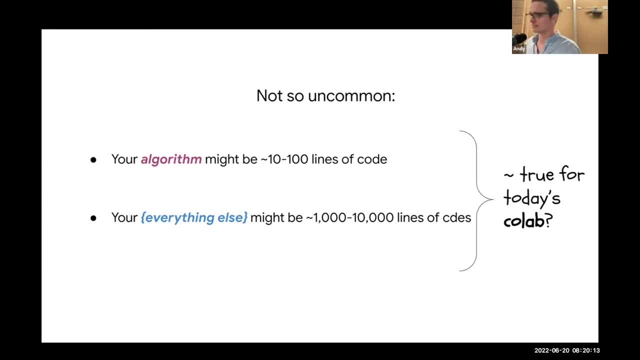 which was kind of the contribution of a thing that Andy and I and others worked on recently. It was just kind of wiring a few things together And there's not that many lines of code, But the rest of it that's like a 2,000 line co-op notebook. 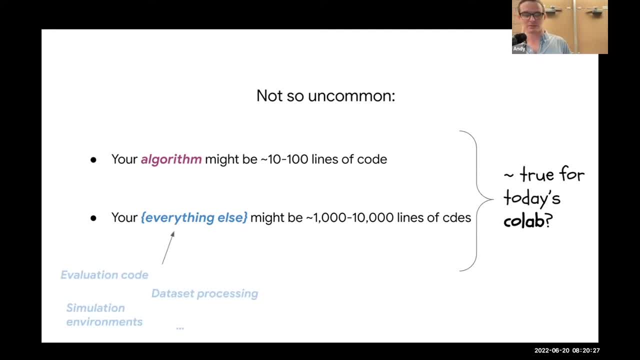 So, yeah, what is this? everything else, Evaluation, code, data set, processing some environments, these types of things. Another thing that I think is not so uncommon, especially, I think, for vision researchers, And if you haven't run into this, this is especially for you. 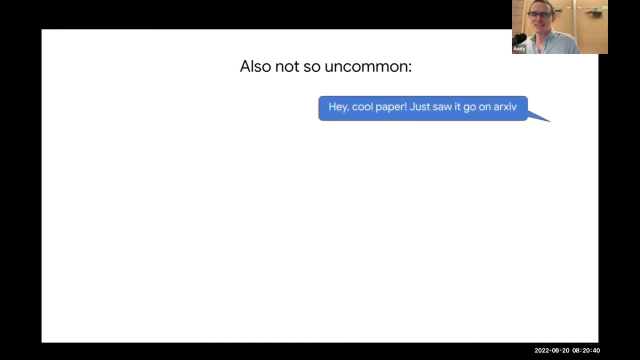 And if you have run into this, well, I don't know, Maybe you'll get a laugh out of it, But I feel like I often have this situation where I'll text a friend or a colleague in some other lab And I'm like, hey, cool paper. 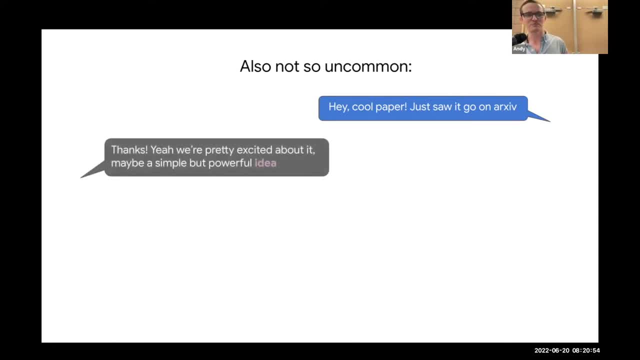 I just saw it go out on the internet- pretty cool stuff- And they'll say: thanks, yeah, we're pretty excited about it. It's like a simple but powerful idea talking about the method, And then you think to yourself: yeah, cool. 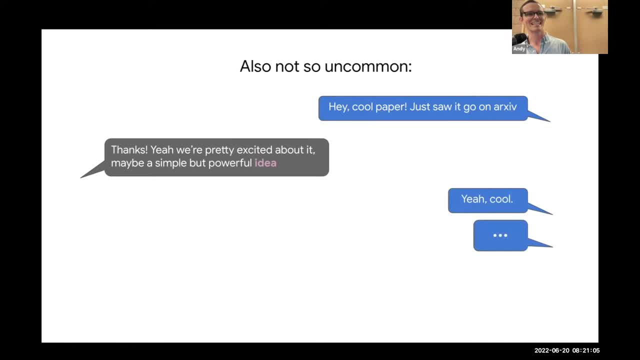 And then you think to yourself and you're not sure how to say it, But you're like man, it just seems like so much work And you're not envious of all the evaluations that they ran, And so you're maybe a little passive, aggressive. 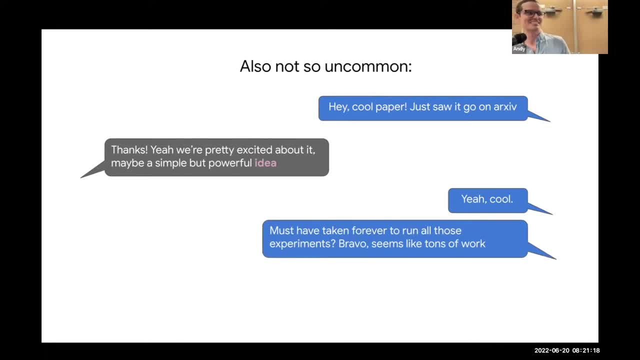 And you're like it must have taken forever to run all those experiments. Bravo, seems like a lot of work. But then, if you've never run into this type of comment before, I think it's very helpful to know that this exists. 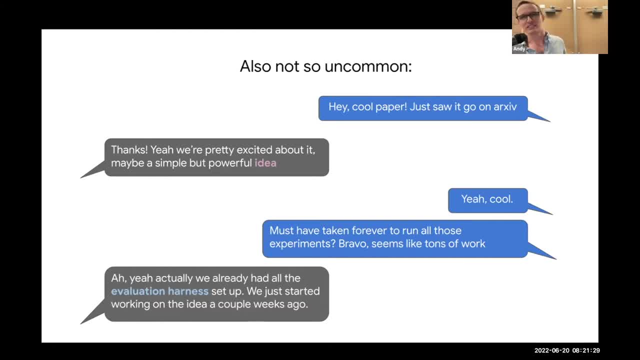 That sometimes when things look like a lot of work, there is actually very quick to iterate on because they had everything else set up. So something like I feel like it's often said: oh well, we already had all the evaluation harness set up. 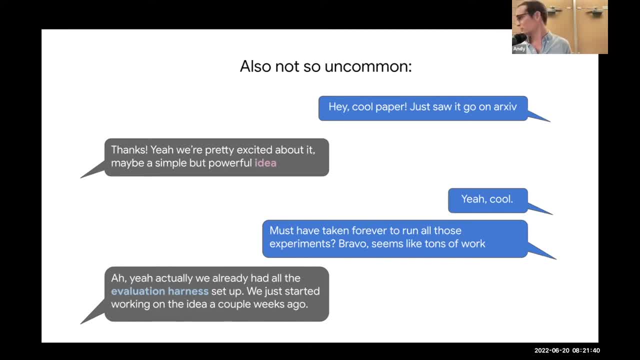 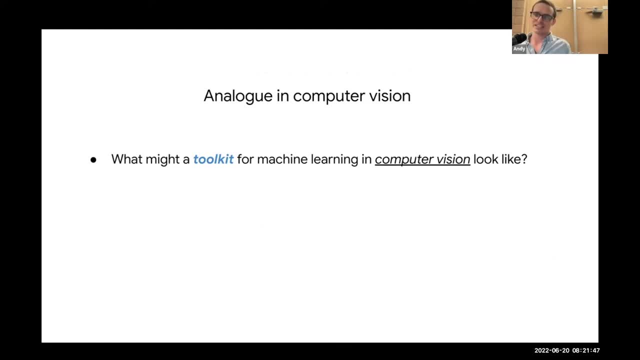 We just started working on the idea a couple weeks ago, So I think it's how that highlights the importance of tools. So what's an analog in computer vision? What might a toolkit for machine learning in computer vision look like? Just a few ideas: access to data sets, evaluation harnesses. 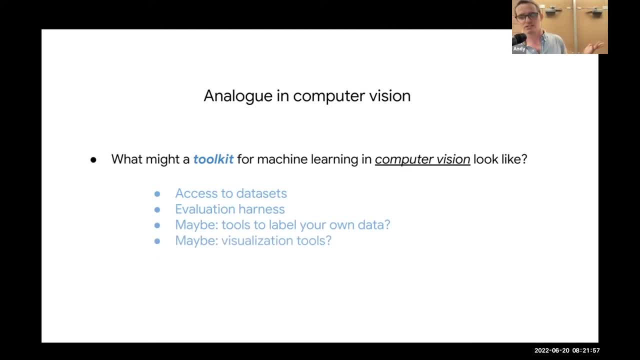 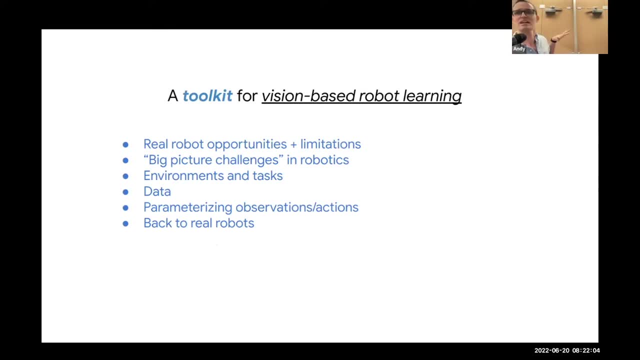 that we were just talking about, maybe tools to label your own data visualization tools, these types of things, just as an analog In vision-based robot learning research. this is kind of the toolkit that I'm going to talk through today: Relative emphasis on different things. 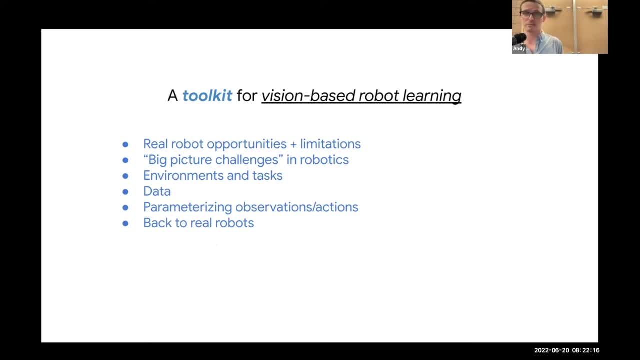 So real robot opportunities and limitations, the big picture challenges in robotics, environments and tasks. data- It's kind of a niche, but I think it's really important: parameterizing observations and actions and bringing it back to real robots- A balancing act that I want to call out. 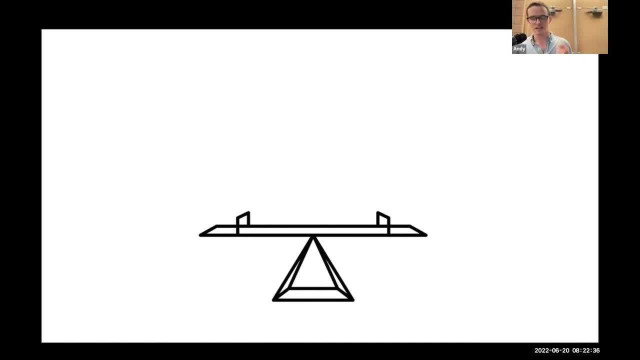 that I'm going to be trying to do here is, on the one hand, real robots are sort of, ultimately, I think, the thing that as robot researchers, as roboticists, we should care about. I think they should motivate our problems. 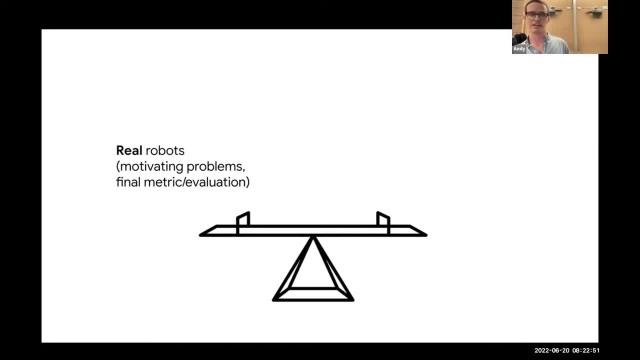 They should, sort of the robots working, should be our sort of final actual metric evaluation. But on the other hand, as many of you may know, sort of simulating robots is very helpful for evaluating a large amount of things, getting high throughput metrics, things like that. 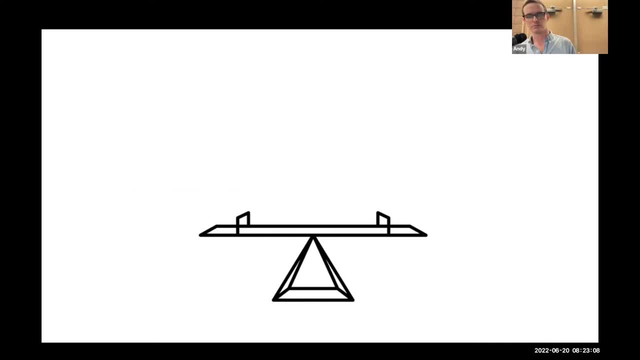 But there's another related but different balancing act I want to call out as we walk through this sort of toolkit I've put together is, on the one hand, having access to real robots and actually running real robots is very important, but there's a certain amount of resources. 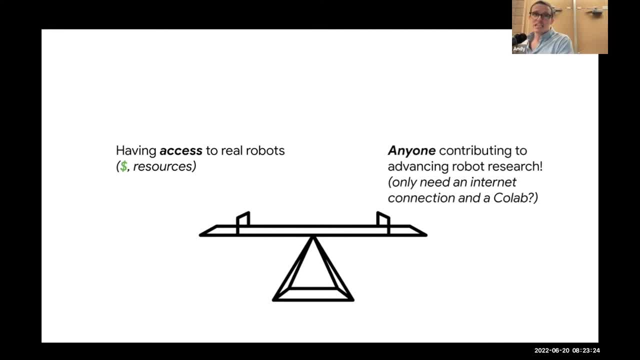 that are required to be able to do that And, on the other hand, to the extent that we can frame problems in terms of being approachable via just simulation, then we can be in this place where anyone can contribute to advancing robot research, which I just think is awesome. 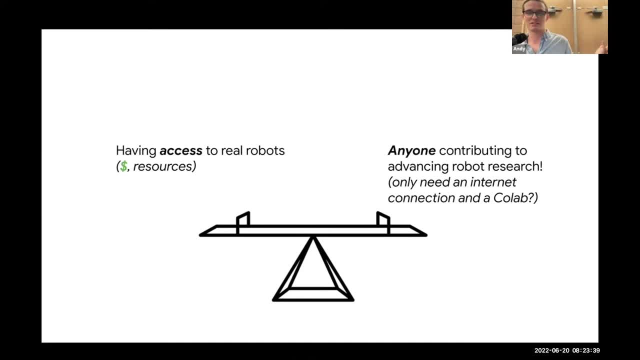 in terms of letting anybody in the world, some kid halfway across the world, where you only need an internet connection and a co-lab to contribute. So, when possible, I'm going to try and phrase things in terms of: hey look, you could do this sort of thing, just. 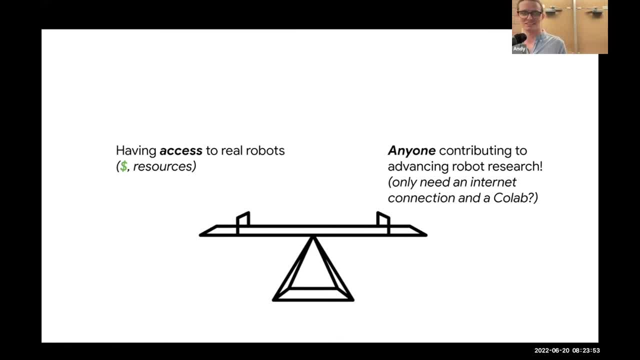 with an internet connection and a co-lab, or you don't need to use a co-lab. That's just a simple, easy example and gives you access to free compute resources. But also Sometimes we do have to ground things back in real robots. 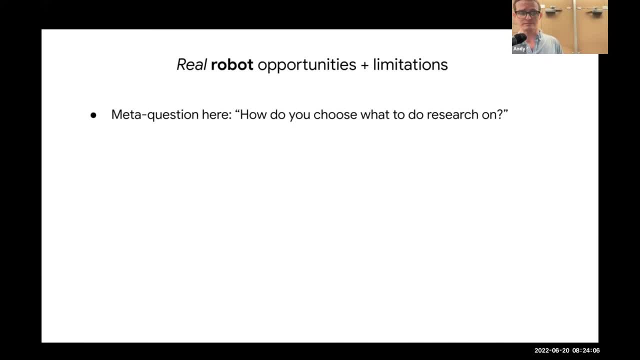 OK, so real robot opportunities and limitations. The real meta question here is: this is sort of the question of how do you choose what to do research on, And the question is: what mountain do you want to go climb? What do you want to go to research on? 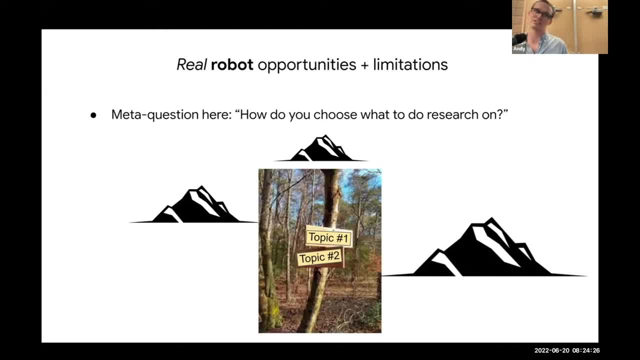 And when you're wandering through the forest and you've got topic one and topic two and your advisor wants to work on topic one but you're like I don't know about topic two, How do you choose what to work on? 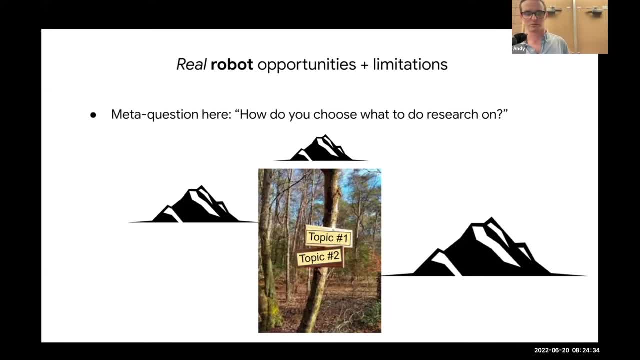 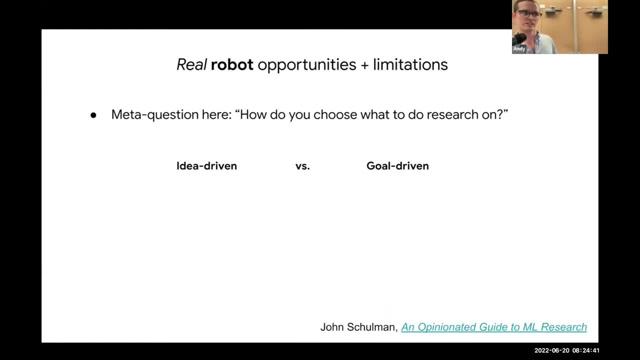 This is one of the key, key things in research and applies across everywhere, But I think it's especially interesting to think about in robot research. I think one framework that I think is very helpful. it doesn't cover everything, but I think it's a very helpful framework. 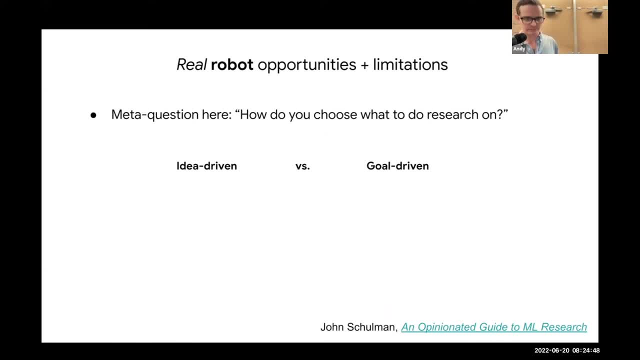 I have the link at the bottom there. This is from a blog post by John Schulman And it puts out that framework of idea-driven versus goal-driven ways of choosing what to do research on- And John actually himself he's a professor. 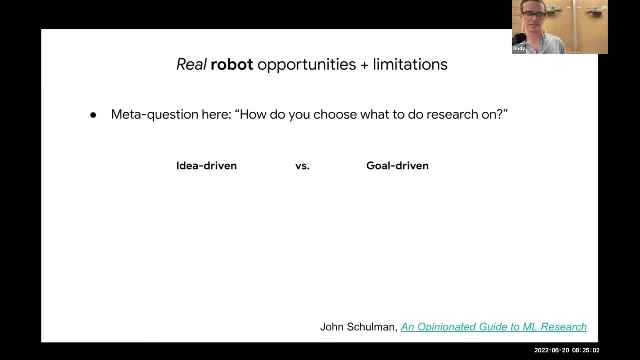 did robotics, at least at the start of his PhD, And so I think part of this sort of framework is inspired directly from working on robot learning research. So just to define what these things are, idea-driven is: you have some hammer, you have some method. 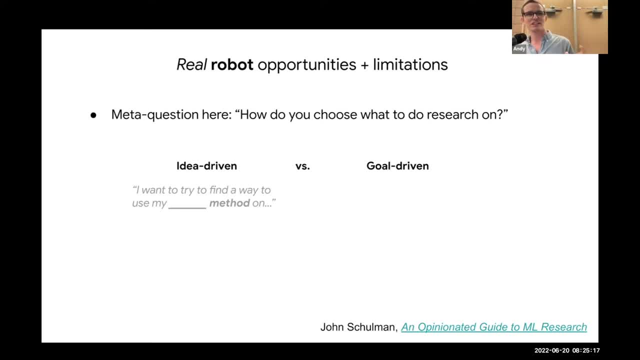 you have some algorithm or some cool little trick idea and you want to go apply it to something and see if it's useful and write a paper about it. That's kind of idea-driven. On the other hand, goal-driven is you just? 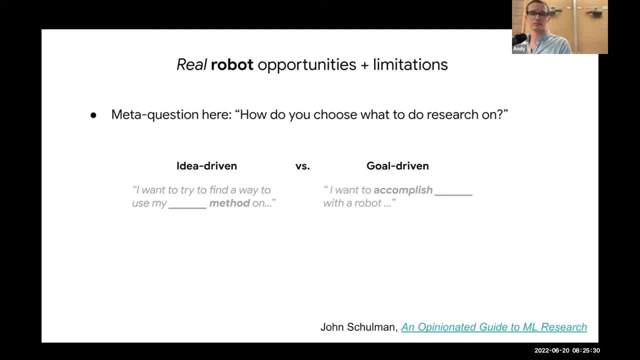 want to go accomplish something With a robot. it's, you want to go accomplish something with a robot, And maybe you don't care at all how it happens And you're just excited about the goal that you're going after. And maybe when you share, that result out. 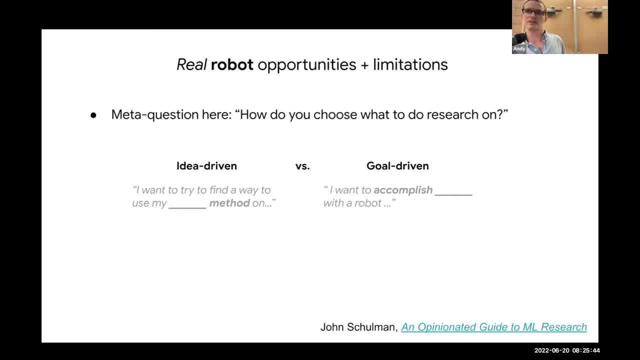 if you're successful in the end, nobody's going to care that you use some simple method to make it happen, because the result is quite impressive. Or maybe you need to innovate and come up with a whole bunch of new things. So idea-driven is a little bit more sort of you've got. 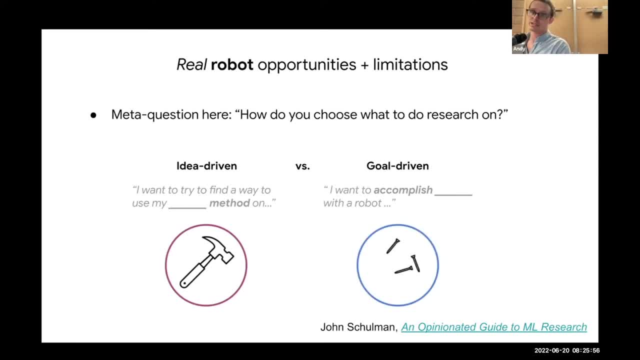 the hammer and you're looking for nails. Goal-driven is a little bit more OK. what are the nails? What are the problems? What are the opportunities? What are the opportunities? And in the robot learning case, I think it's especially 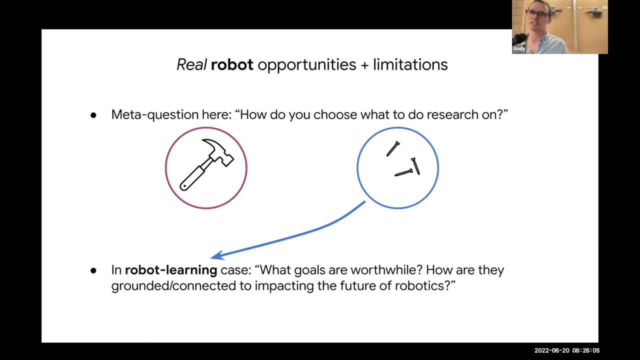 interesting to think about. but we can't just say, oh, let's go for the nails, Let's go for goal-driven. I think we have to have a sense of what goals are worthwhile and how are they going to connect it to impacting. 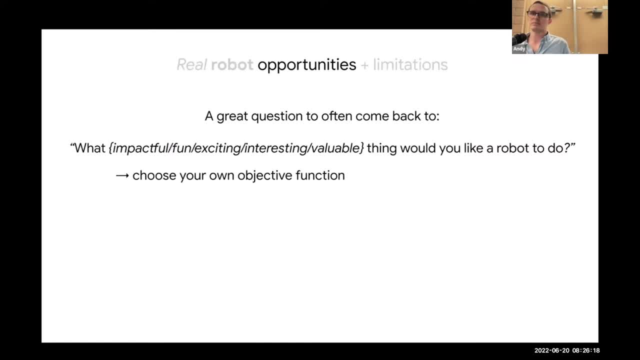 the future of robotics. So it's very simple, but I think often one of the best ways to start, and even come back to often, is just asking yourself, sort of use your own imagination, What impactful, fun, exciting, interesting, valuable, 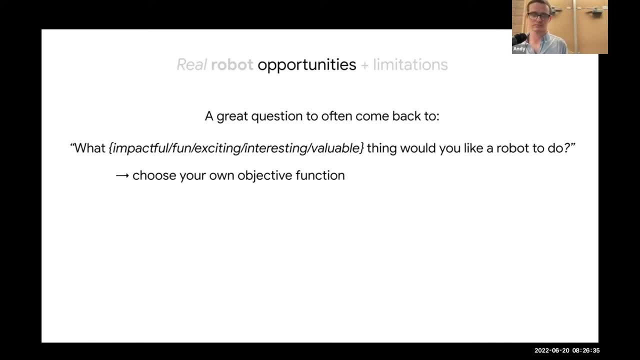 choose your own objective function thing. do you want a robot to do? And I think it's just. you know it's easy to get lost in the weeds of: oh, I'm doing this, working on this little problem, but what do you want the robot to do? 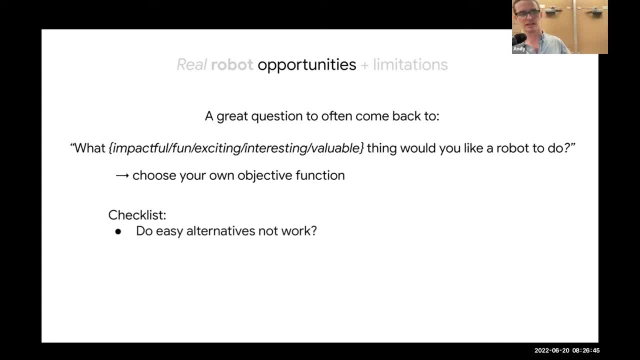 It's a very helpful question And a little checklist to go through is OK. do easy alternatives work? Is it implementable in the real world Or is there a path to do so And it might be kind of hard? Doing anything with robots is pretty hard. 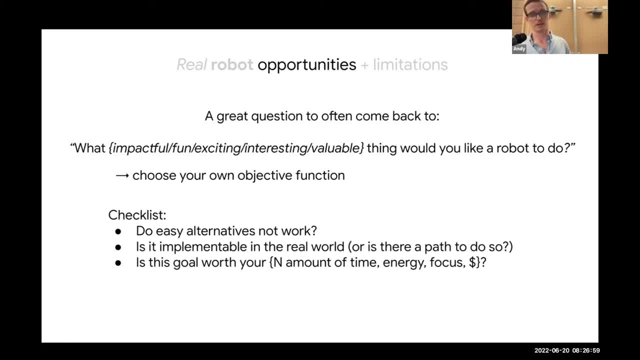 So is it an interesting enough goal that it's going to work? Is it going to be worth your n amount of time, energy, focus and dollars? And if they answer the questions- all those are yes, then you might have a worthwhile problem. 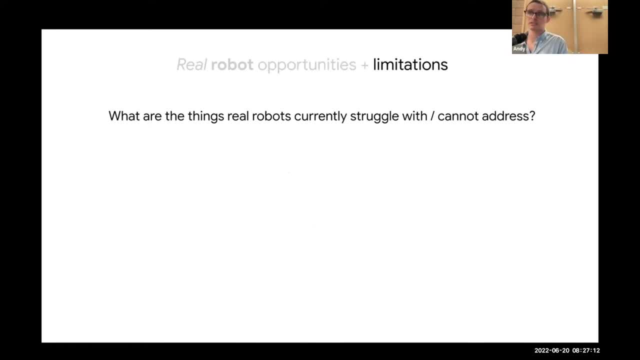 On the limitation side, what are things that real robots currently struggle with or can't address? I think for people maybe new to robotics, especially because I love sci-fi- but it's funny because I'm a robotics researcher. but I don't know how old I was when I realized that C-3PO was. 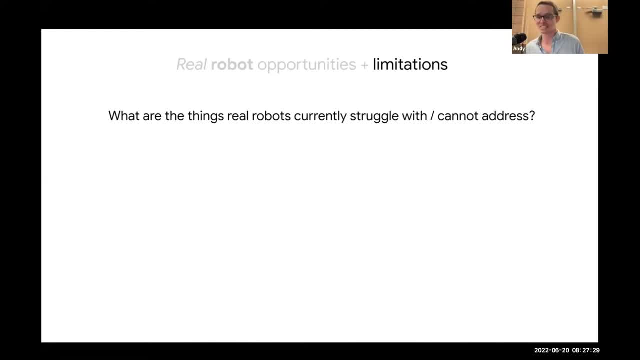 a man in a costume. you know what I mean. I don't know exactly what the number was, but it was at least double digits probably. Let's put it that way. So getting a sense of what is actually the state of what robots can and can't do, I think. 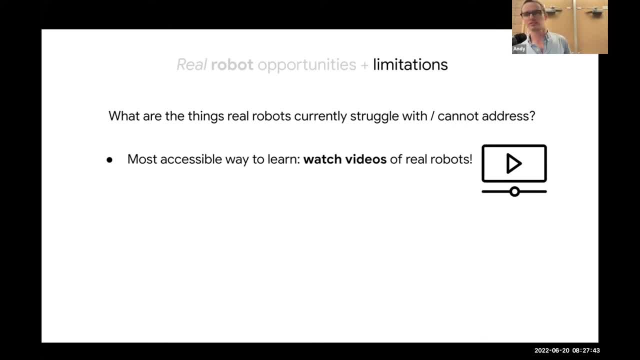 is really important to do, And I think the most successful and easy way to do it is just to watch a lot of videos of real robots, And that comes in a bunch of different flavors. Whenever you see research papers and they have video, just click on the video is the first thing that I always do. 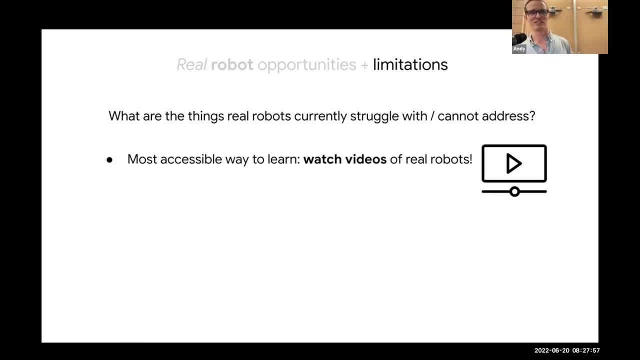 I feel like a lot of researchers, and probably in vision too, are just always looking for the videos, the highest bandwidth way, often to understand what's really happening, And then also, too, just search the web, Just watch a lot of videos of real robots. 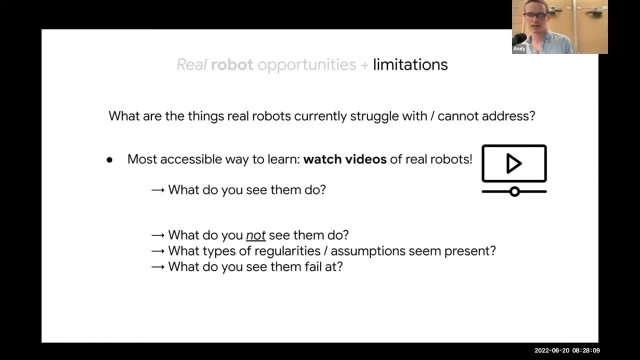 I think that's honestly the best way to just build a lot of intuition of what is actually possible and not, And pay attention not just to what you see them do, but also pay attention to what do you not see robots do. I think I mentioned this earlier when we were chatting with Andy. 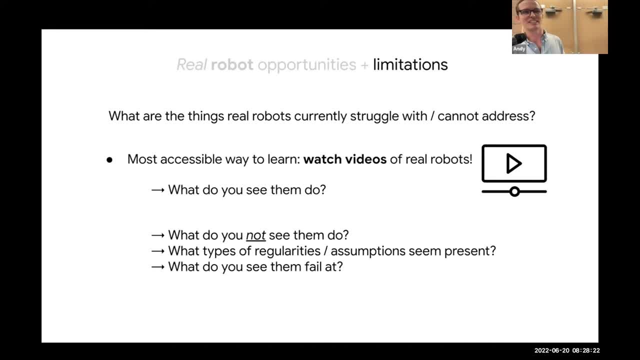 that often when people put together robot demos, they kind of show you everything that the thing can do And if they're not doing something, then you know that they probably can't do that. Or look and try and do something that you know and take note. 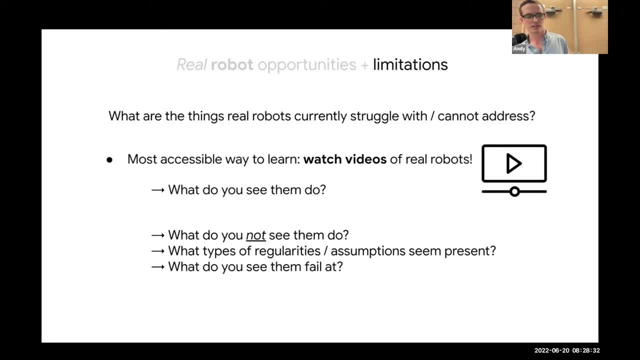 Like what types of regularities or assumptions seem present in the environment or the set up at LARC And what do you, you know? hopefully they, in a recent paper at least, they'll actually show some failures and take note of those too, of course. 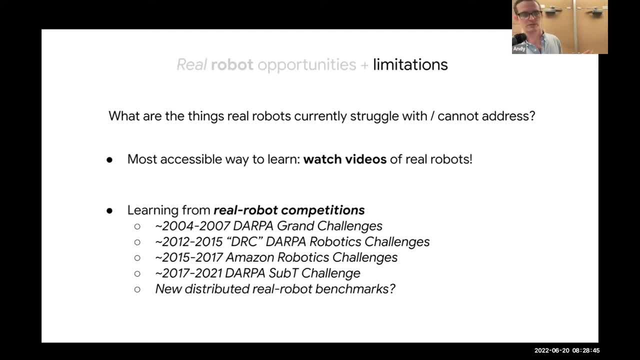 I think another huge source of knowledge to look at, especially for folks into robotics, is learning from real robot competitions. So I think DARPA gets a lot of credit- for it should get a lot of credit in my mind- for running and organizing and instigating. 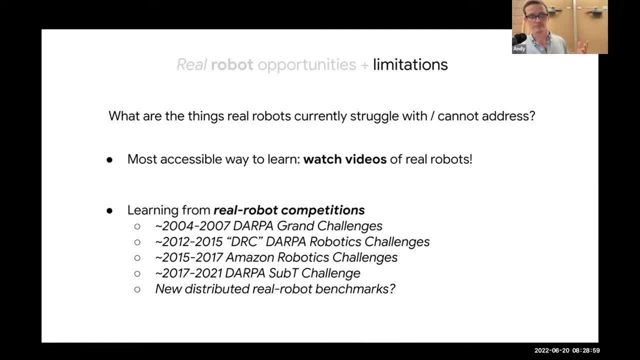 a lot of these things over the years. So there was like the DARPA Grand Challenges, which was sort of a key, you know step in building a lot of momentum in autonomous driving. There was the DARPA Robotics Challenges, which was the humanoids like ATLAS. 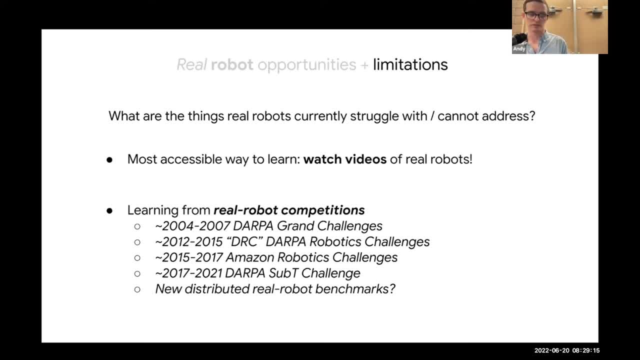 and a bunch of other humanoids. That was a huge program 2012 to 2015.. 2016, maybe two- These are rough, rough dates. The Amazon Robotics Challenges- Andy participated in that one. Props to Amazon for actually putting that one together. 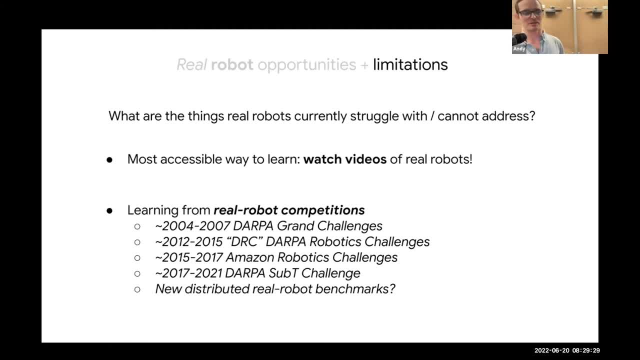 It was really cool. It was really cool, It was really cool. Most of my list here is from DARPA, but I think it was awesome and really well received by the community that Amazon put that one together, Or the, I think, the most recent one in the DARPA world. 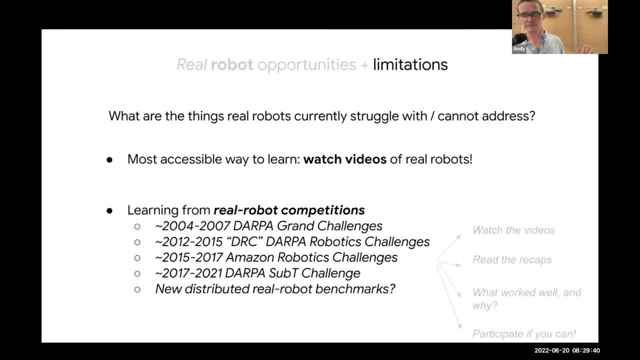 is a subterranean challenge. So there's just a ton of learning to be had from these types of events, as people are actually trying to put forward, on real robots and competitive teams and sort of problems that, by definition, robots can't easily solve. 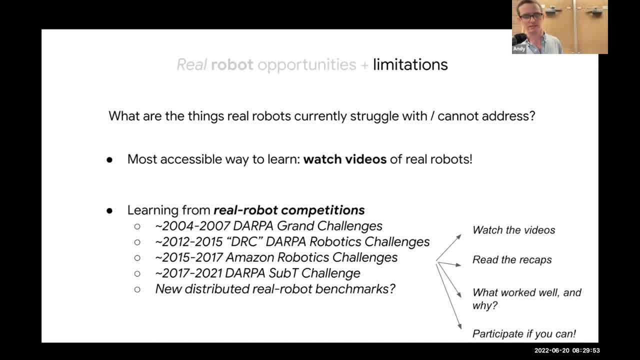 like recipes that actually work. So definitely with these, I recommend watching the videos, reading the recaps- There's all these like review papers of how these things went down- and try and take note of what worked well and why And if another one of these sort of opportunities come around. 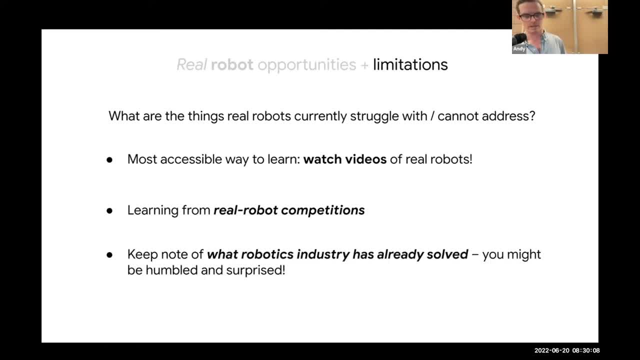 I would strongly encourage participating, if you can. Another one too. you might be humble. Keep note of what robotics industry has already solved. There's just a lot of things that you know. if you can, I recommend going to a robotics industry conference. 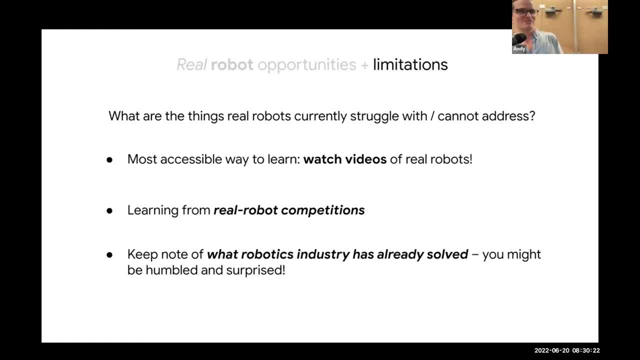 There's a lot of things that, like you, might be like- oh no, my research problem looks very similar to that, but they're just deploying it and, like you know, doing all these things at scale and industry. So that's another one to keep in mind. 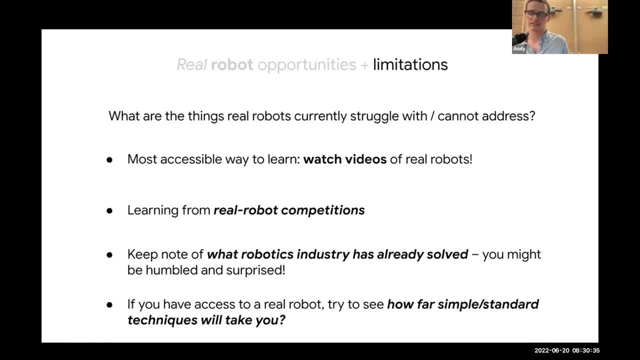 And if you do have access to a real robot, I highly recommend just trying to see how far simple and standard techniques will take you And that can help you identify what are the sort of limitations that you know- maybe learning-based robotics or new techniques? 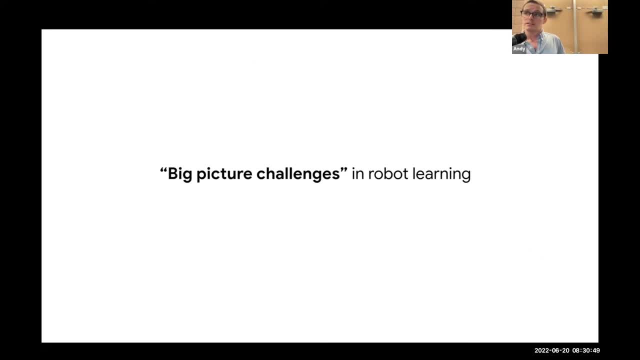 actually need to come in and solve. So next in the toolkit, just keeping in mind big picture challenges in robot learning, These are the. these are the big, big picture challenges. This, though, is just my own biased and non-comprehensive short list. 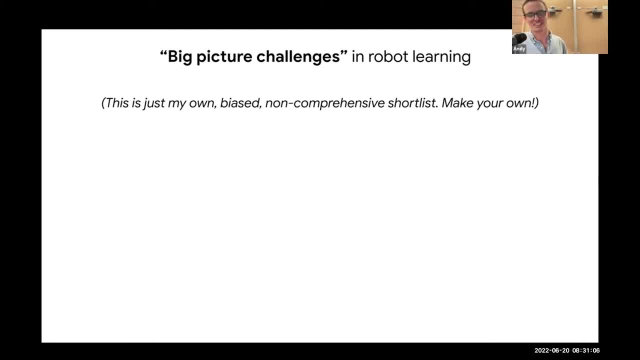 And you know, I'm gonna show you what maybe mine is at the moment. just a quick take on it, But definitely I encourage you to make your own and sort of accumulate your own version over time. So I would say my number one is just: 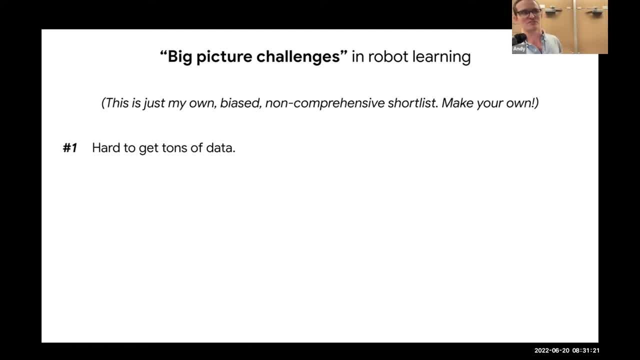 it's very hard to get tons of data. You wanna do learning sort of. by definition, you kind of need data in robotics. You can get a good amount of data, but it's very hard to get a ton of ton of data, And I think that is one of the fundamental challenges. 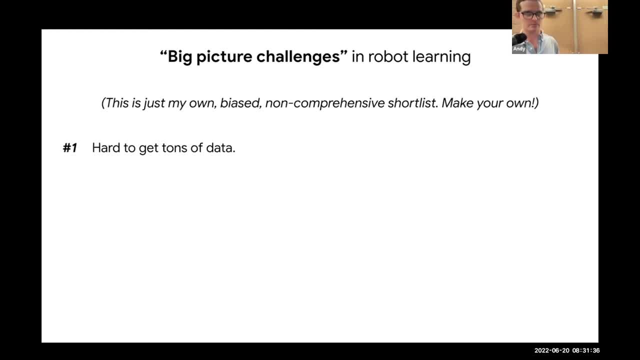 of the field And I put it as a separate item. Number two here is just exacerbating number one, which is that number one is exacerbated by the embodiment cross task space explosion of the sort of space over which the data needs to exist. So what this? what I mean by this is that in 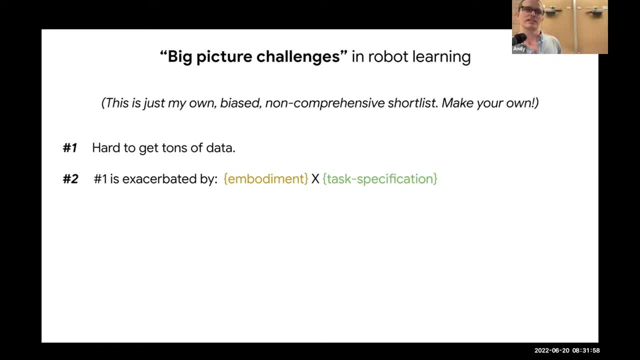 in computer vision. I know there's like point clouds and other things, but let's say that a large majority of computer vision operates on the RGB image, or maybe it's monochrome, whatever, but you have RGB images And there's a lot of different cameras out there. 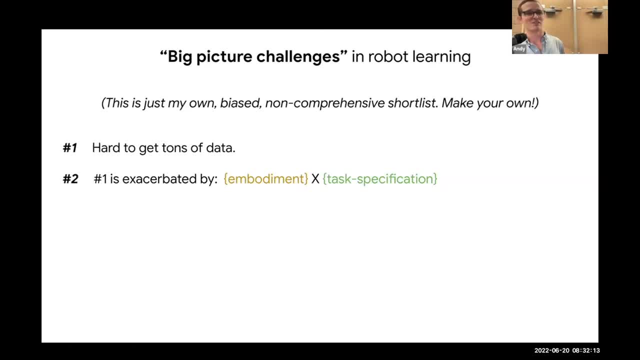 but you know what? as you all know, there's a lot of regularity in what an RGB image looks like. You know, height by width, by three. it's a beautiful thing. There's a lot of regularity, And what this means is, of course, 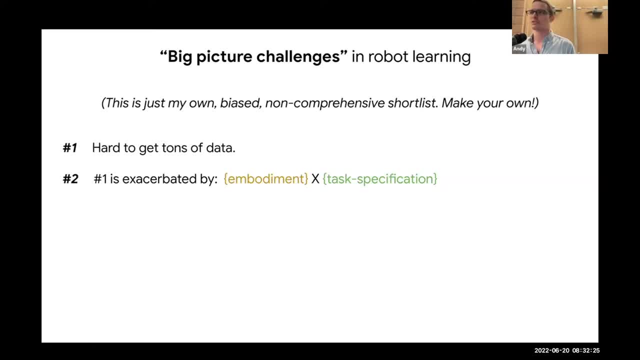 there's different intrinsics, there's things that affect different things there. Exposure: I know there's a lot of subtleties, but it's just known that RGB images from all over the place is sort of as long as they're sort of not too fisheye. 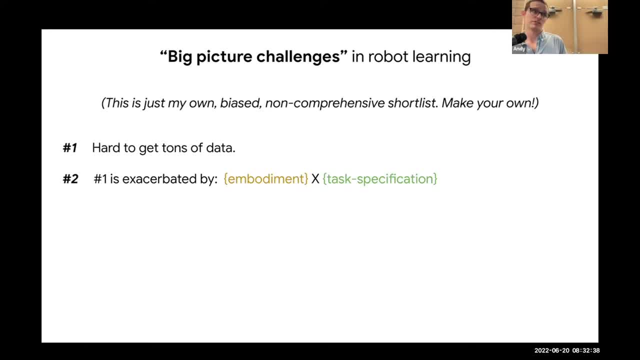 and don't have other weird artifacts. we can get machine vision systems to work at scale on a lot of these things. Everybody has one in their pocket. They all have roughly the same sort of representation of the data. In robotics it's completely different. 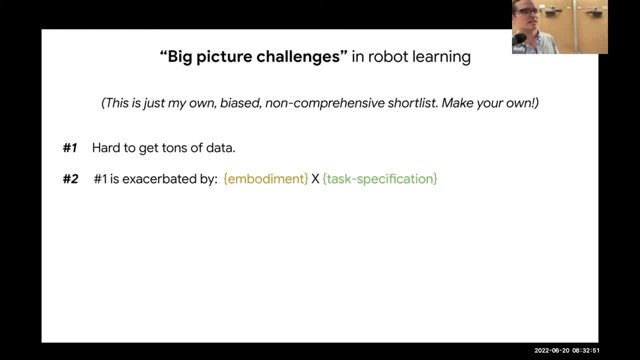 Every robot, especially from the actuation side, has a different embodiment And even if you have like 10 copies of the quote unquote, same robot, every single physical actuator, you know, maybe ages a little bit differently. Maybe somebody replaces something. 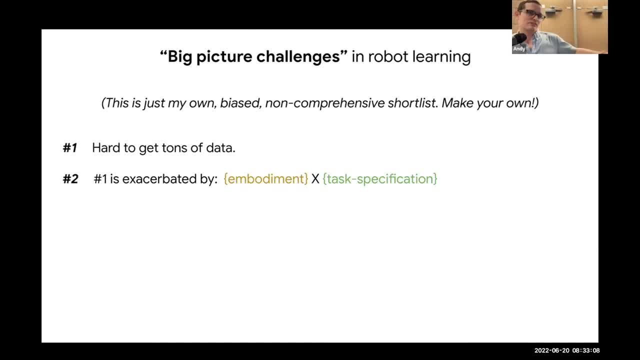 so the actual geometry of it is slightly different, And that's even if you have 10 copies of the same robot. but there's all these other robots out there And so sharing data across all these different robots, this embodiment challenge of how they have. 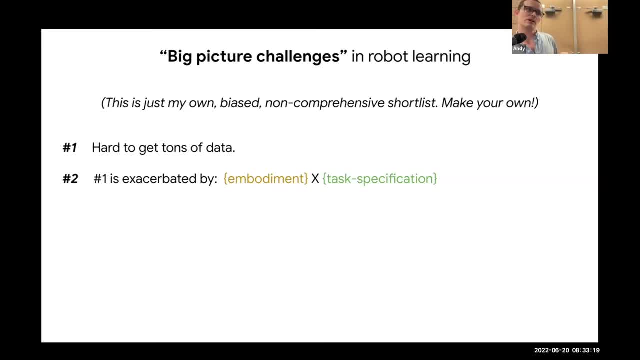 different embodiments. it just completely explodes the amount of data that you might want. Maybe you want to have enough data to cover every single manageable embodiment ever possible, but it just explodes your data. It just explodes your data requirements. And on the other side, 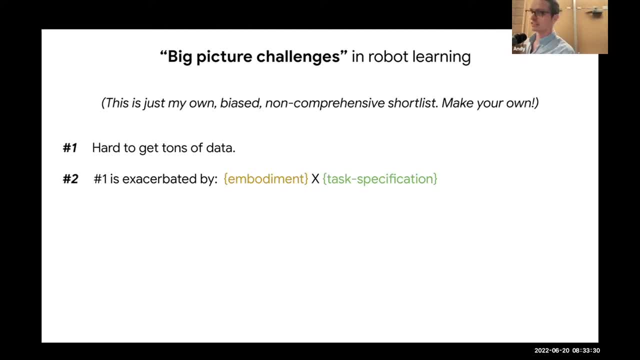 in conjunction with the embodiment challenge is the task classification challenge, which is that in computer vision there's actually a fair amount of diversity of different tasks, So you might have classification detection, pixel-wise segmentation, whatever it is. In robotics, though, it's just endless. 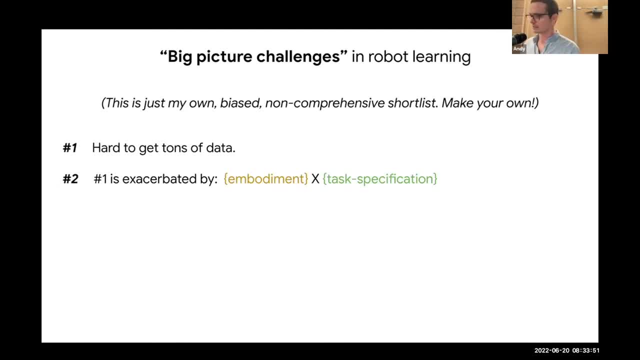 There's so many continuous spaces over which task classification might exist, So a task might be: hey, robot, can you take this coffee cup here and can you take off the lid, and can you put the lid there and can you put the cup back there? 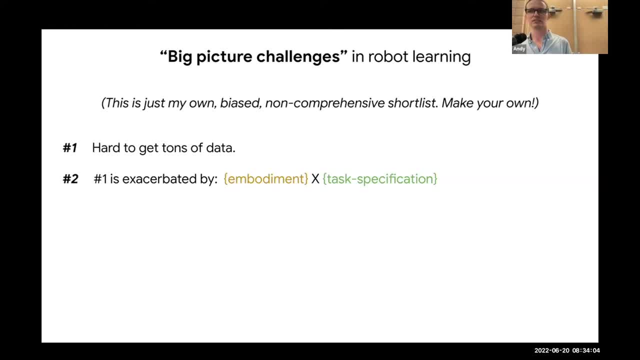 and actually first can you pour out maybe 50 milliliters into another cup And all those that's a valid thing to ask of a robot. I think language has a little bit more of a similarity in that- the sort of things that you can ask. 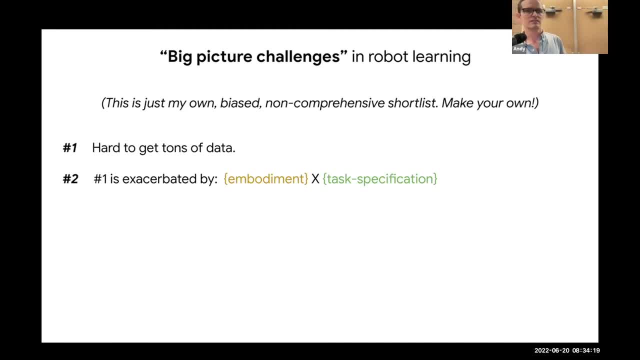 a language model is sort of unbounded, other than just what's expressible in language. I think they have that same challenge too in robotics, but again compounded with embodiment. So I think this is my number two and it just exacerbates number one. 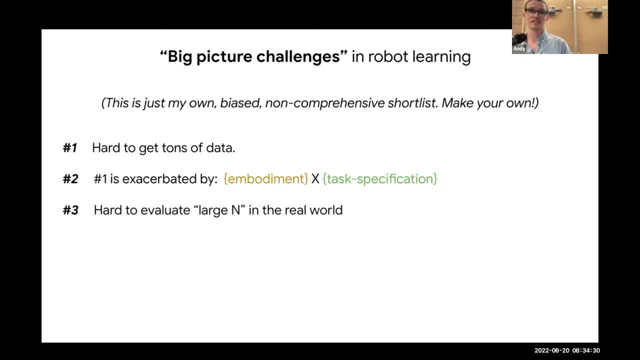 Data's hard. Okay, number three related but different is it's just hard to evaluate large and in the real world. I think we can do things in the real world, but it's hard to evaluate a ton of things in the real world. 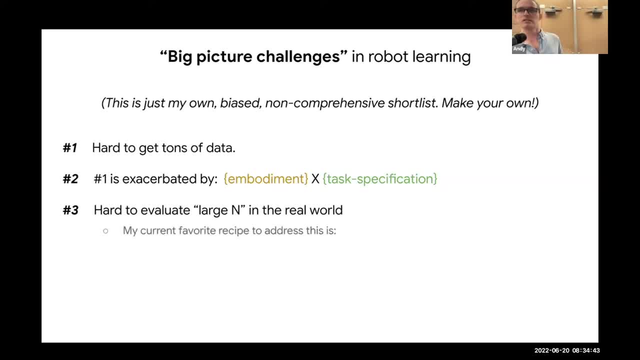 I have a few thoughts on sort of my current favorite recipe to try to combat this, which is that you start with motivating from real world opportunities and limitations and then you make a relevant simulation. This is a common technique that I think is often useful. 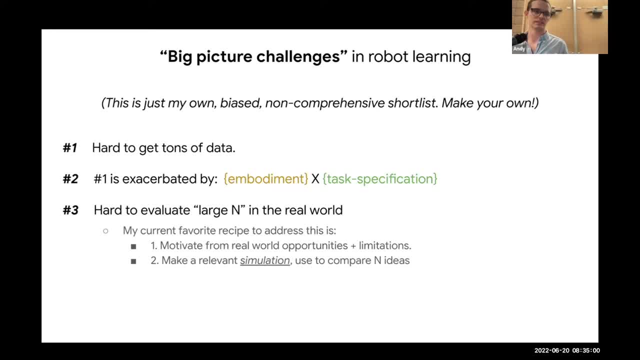 And use the sim to compare your full set of different ideas And then cull that full set of different ideas down to some small subset and validate and compare those things in the real world. I think this is sort of a very practical, my current favorite recipe for trying to address this problem. 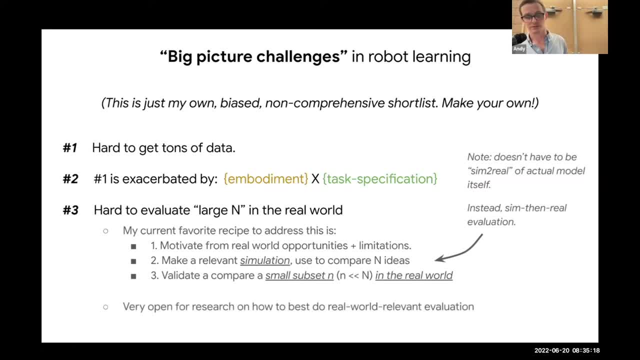 But it is certainly very open for research on how to do a good real world evaluation. And I also just want to note that you might look at that and be like, oh yeah, sim to real, And I think sim to real is interesting. 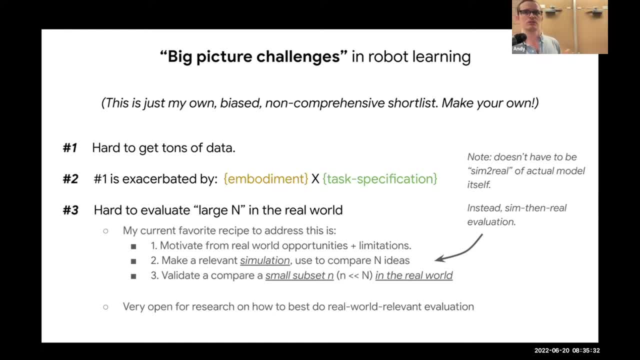 But the recipe that I'm saying here is sort of not sim to real of a model itself, but rather it's kind of like meta sim to real, where you evaluate lots of different things in sim and then you choose the best sort of algorithms. 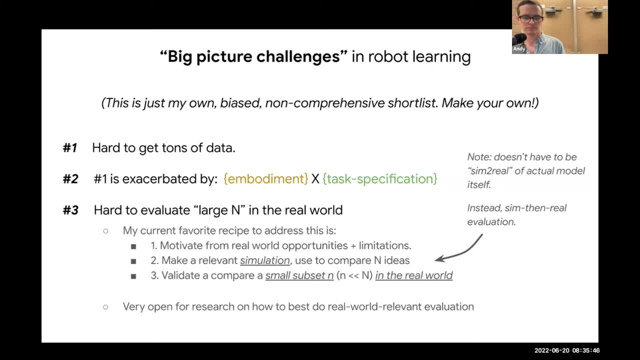 or maybe hyperparameters, and just separately entirely set them up in real. It's kind of like sim to real of the algorithms but not the weights, so to speak. And again, a lot of people use this type of recipe But it's sort of my personal favorite. 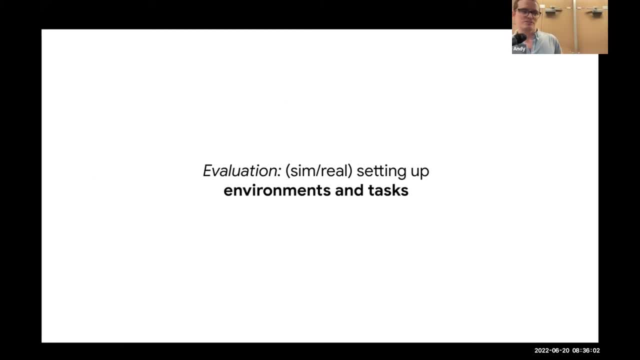 OK, so that was some thoughts on big picture challenges. Again, I encourage you to come up with your own recipe. So let's talk about evaluation In robotics. I think evaluation often boils down to in sim, to real setting up environments and tasks. 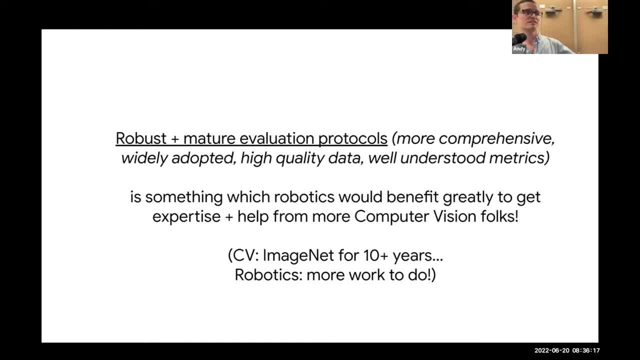 And I think there's a lot of subtleties here And especially here with computer vision folks- robust and mature evaluation tools, more comprehensive, widely adopted, et cetera, is something that in robotics we would- robotic researchers would love to get additional help. 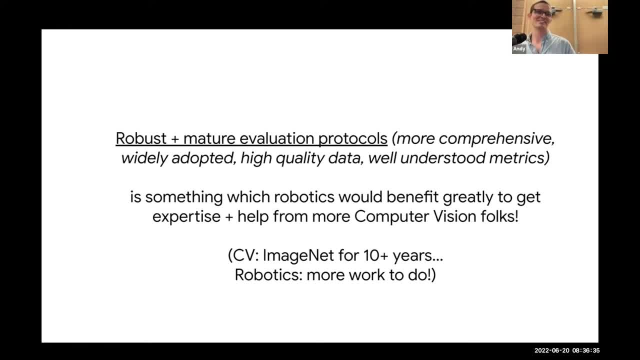 from computer vision, Because I think over the past decade or so or more, robotics has been over here looking at computer vision being like wow, there's been so much consolidation and high quality data and benchmarks and the quantitative focus And that has really driven a lot of great innovation. 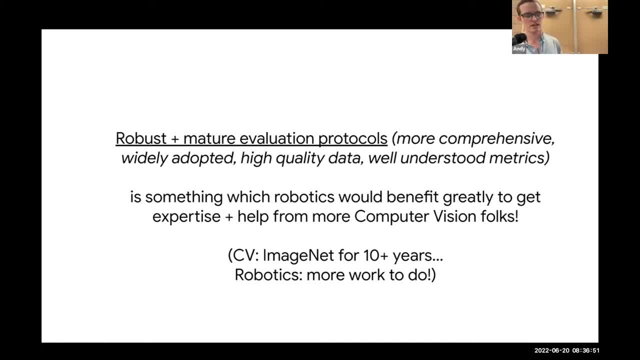 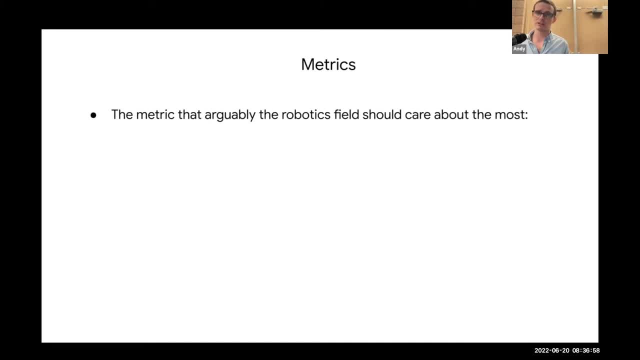 in the field And in robotics. I think we have some progress in that direction, but certainly more work to do. So let's talk about metrics. So with robots, I would argue that the metric the robotics field should care about the most is a very simple one. 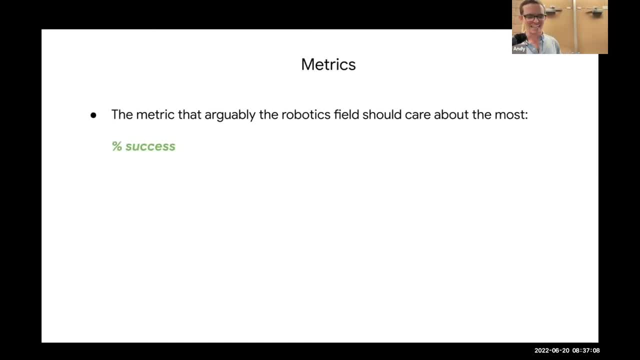 And it's percent success. That's my favorite metric And there's a reason for that Because, at the end of the day, if we care about making robots work, why don't we measure whether or not the robot works? That's sort of the metric at the end of the day. 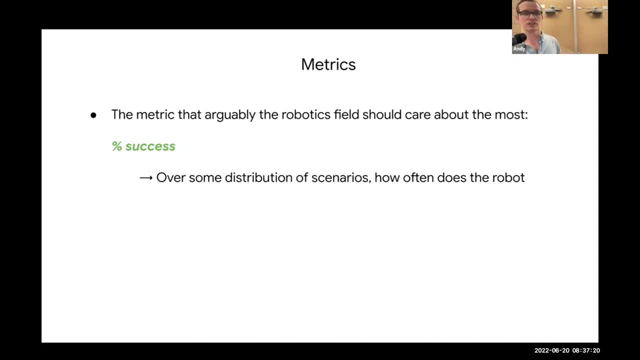 Of course it's more subtle than that. It's percent success over some distribution of scenarios. How often does the robot work? That is the question, especially for things that might not have been possible before. Or does it work better in a wider variety of scenarios? 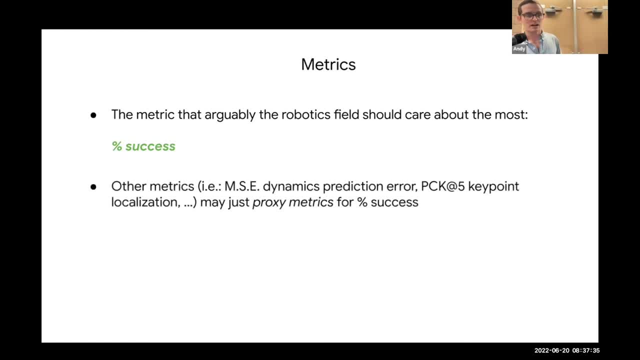 some wider distribution compared to prior alternatives. I think arguably there's a whole bunch of other metrics that you might care about And we measure and we put in research papers, whatever it is we track for projects that we're developing. I think they can all be very useful. 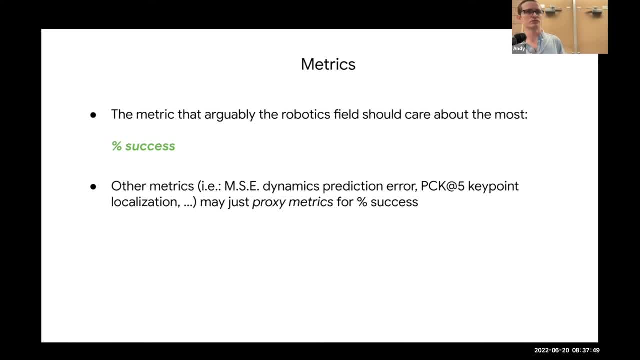 Ultimately, it's at least useful to consider thinking about them all as just proxy metrics, or percent success of real robots, I would say. I think percent success can be phrased to fit whatever problem you care about. That said, though, I think it is really hard to capture. 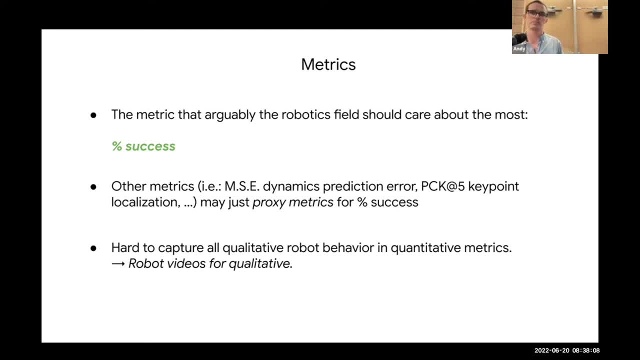 all qualitative robot behavior in quantitative metrics And I think there's basically just no way around it. I think that having videos- I already talked about videos once- having videos of robots actually doing things just communicates so much qualitative the nature of how the robot is functioning. 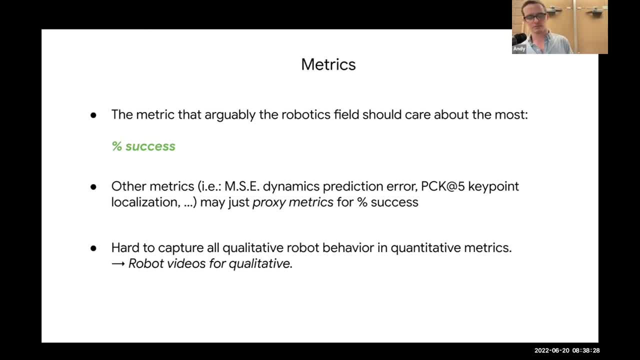 It's really hard to capture with quantitative metrics. So the combination of percent success, maybe other metrics if you need them, and videos, I think is kind of the best mix. I think there's an interesting debate. I couldn't find the reference but I 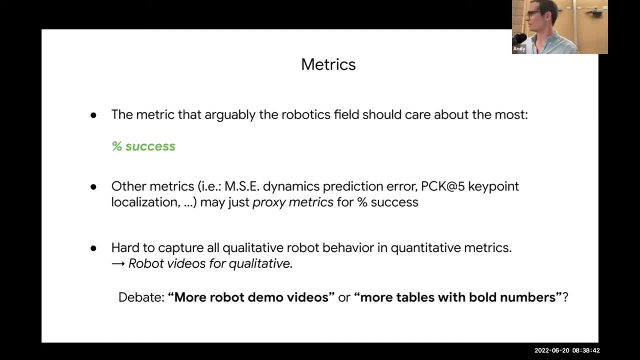 remember reading the paper- I think it was maybe Peter Court, I forget who it was. But an interesting sort of question that like: oh, maybe what robotics research needs as a field is less robot demo videos and more tables with bold numbers And CVPR. everybody here is really. 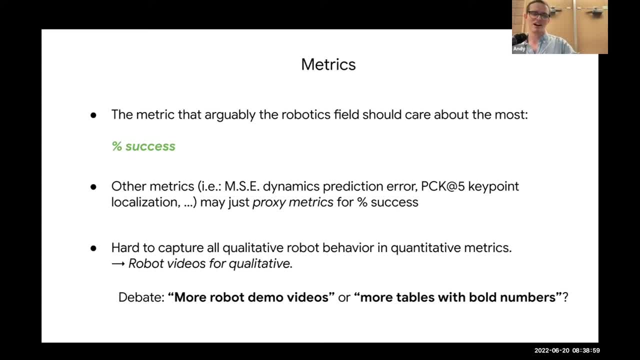 good at tables with bold numbers, I think. arguably, my personal view is that I think we need both. in robotics, I think tables with bold numbers are really good And they do drive sort of like: OK, let's actually be honest and what things are working the best. 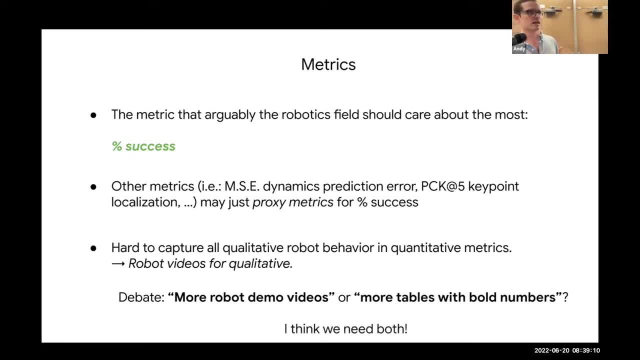 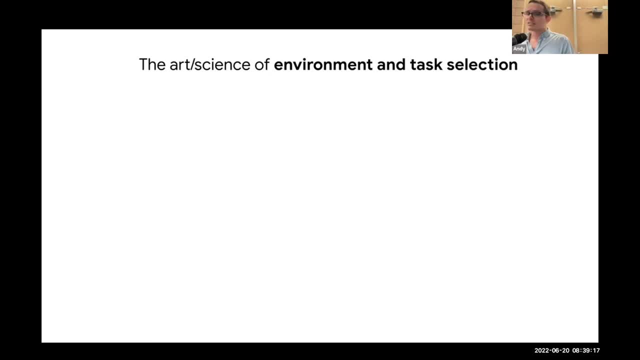 But I think again, there's just so much closed-loop real-world interaction, things that are hard to capture with just quantitative. I think we need both. OK. so the art and science of environment and task selection- I think there's some of it- is definitely art. 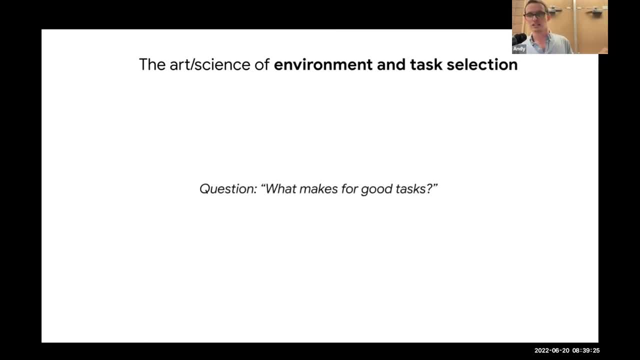 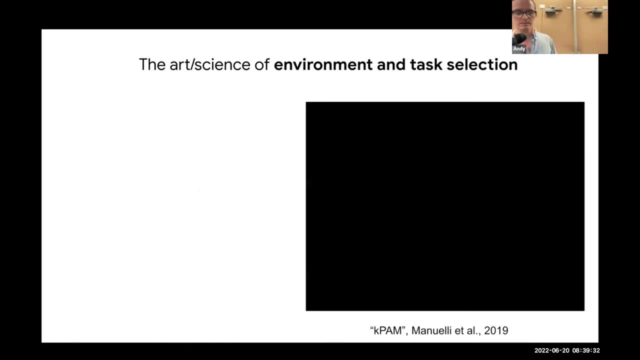 Some of it is not. Some of it can maybe be more science, But I think there's really a lot here where the question is: what makes for good tasks to be working on in robotics or tasks to be trying to apply our methods to in robotics? 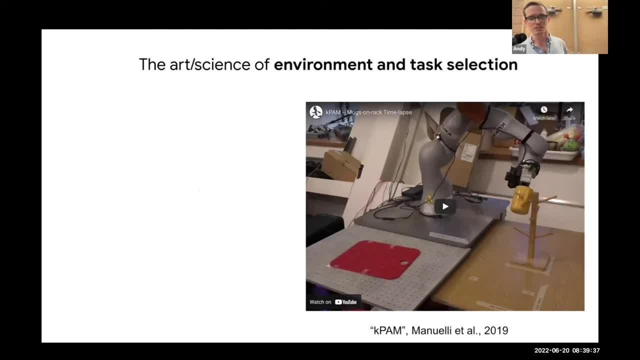 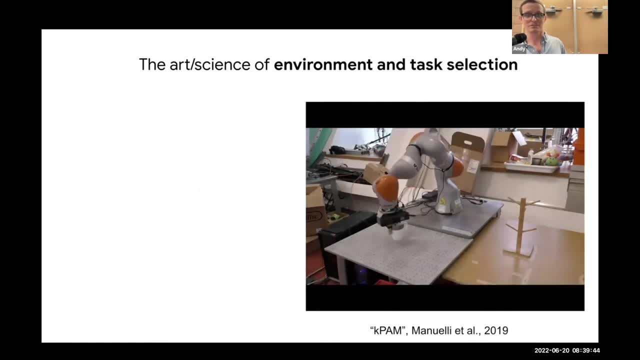 So I think the best way to do this is maybe through some examples. I'm going to be biased and pull some tasks from some of our own papers over the years, But this is one on the right which is the hang the mug on the rack task, which is actually over just the past. 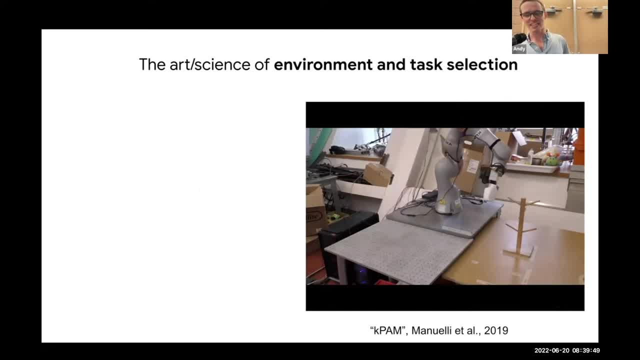 couple of years- has been adopted in a few other papers, I see, But I think it's a really nice task to get a robot to do And I'll walk through it. I'll walk through a few different reasons why. The first one, which I think applies to all tasks: 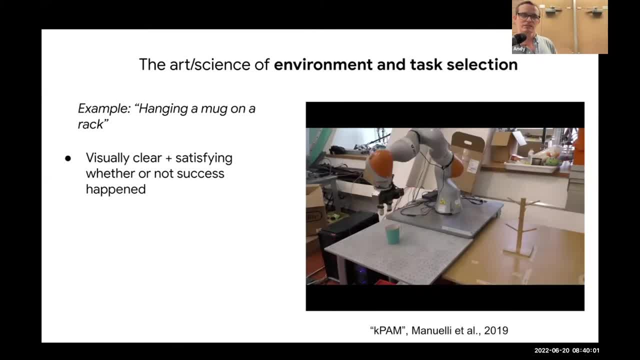 in general, no matter, because different tasks will have different flavors, measure different things. But one thing I think is really important is it should be very visually clear and sort of satisfying- maybe even like sort of ASMR style- of whether or not success happened. 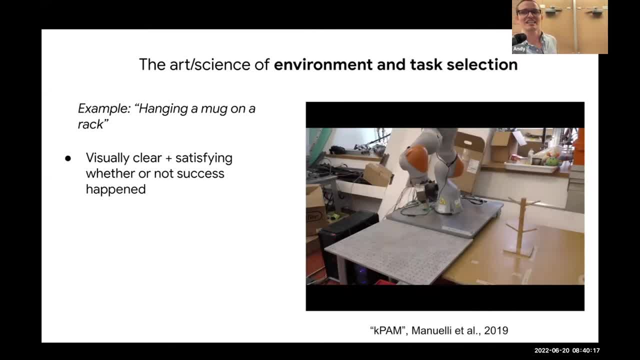 A bad task to be studying in robot learning. research, I think, is where you see the robot do its thing And at the end of the little second segment of the video, the title says success And you go. really You want it to be obvious that the thing succeeded. 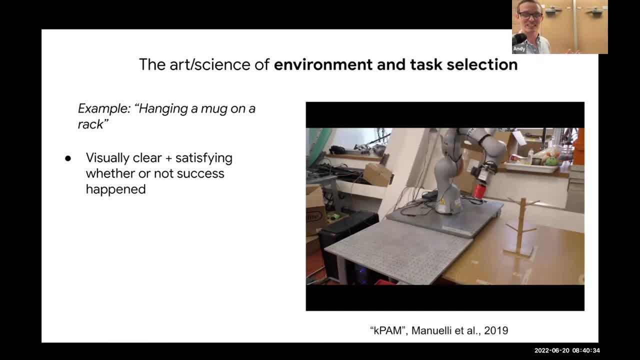 I think hanging a mug on a rack is great, because if it hangs on there by itself, it's obvious That thing worked. If it doesn't, it didn't work. So I love that aspect of it And, again, I think it's really just a nice thing to have. 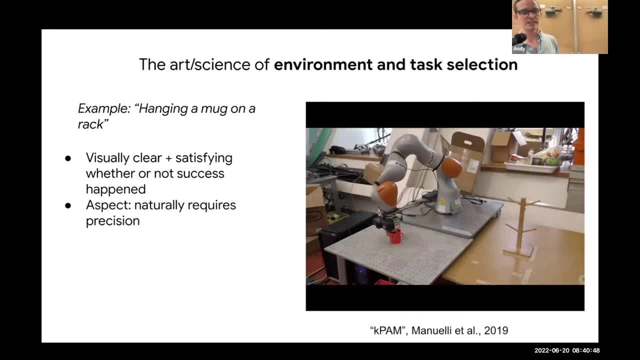 at least in research. for a bunch of things, This one is particular to this task. It might be something that you care about. This task requires precision To get the actual handle of the mug onto the rack. It's naturally a very sixth off task. 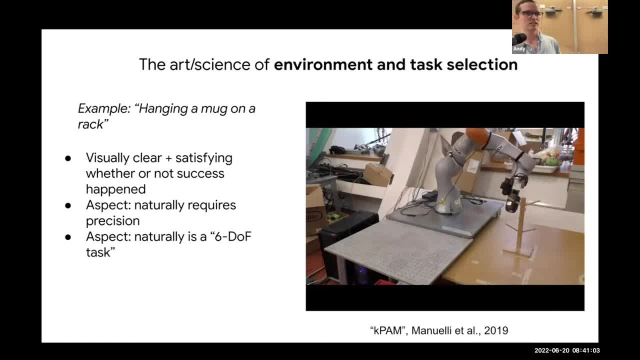 Actually a lot of tasks can kind of be more, maybe just translation only or maybe just kind of top down. This one is very full sixth degree of freedom in its nature. So that's nice about this one, if you care about that. 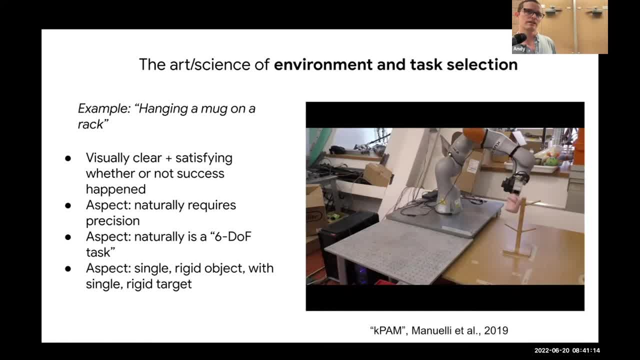 It is a single rigid object with a single rigid target, just to call that out. Maybe you care about deformable objects or liquids or things like that. And another one I think is nice about this one is it lends itself very well to class. 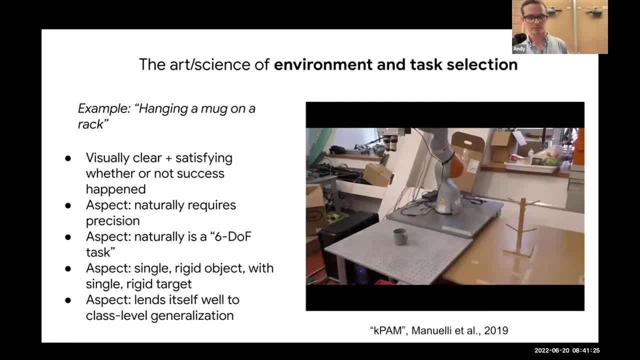 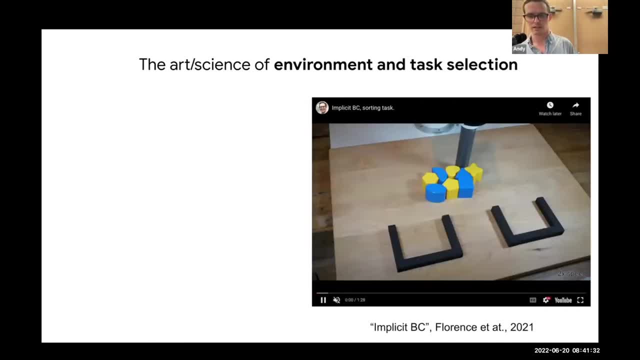 Level generalization, which is, if you're interested in studying that type of a topic, it's a good setup for that. Let's look at another task, another one that I like a lot, which is from a paper of ours from last year, which is sorting the blue blocks. 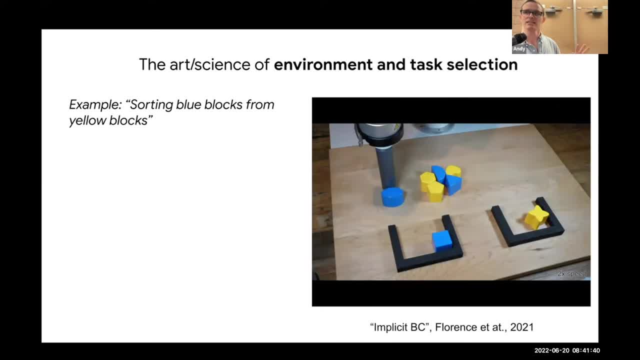 from the yellow blocks, or sorting in general of sort of like eight things is a lot more than one thing, And so in this task the robot's goal is to sort all the yellows from the blues Again. I think this one is very sort of visually clear. 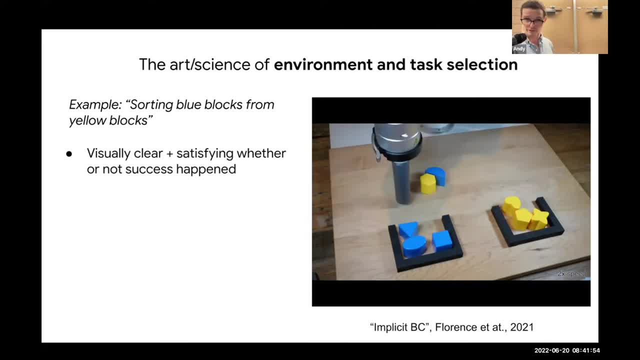 and satisfying Whether or not success happened. Maybe initially, at the very first frame of this video, you weren't sure what was going to happen, But by now you can kind of autocomplete in your head what should happen. Another aspect of this one is it's a handful of objects, not 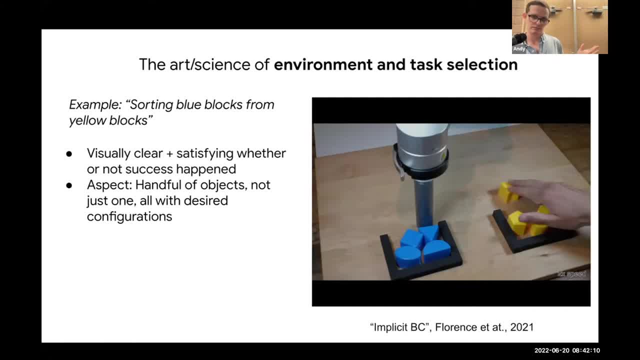 just one all the desired configurations. I sort of talked about that, but that's different than the one we looked at before. One interesting thing about this one is that we trained it so that the ordering doesn't matter, So it really forces a huge amount of multimodality. 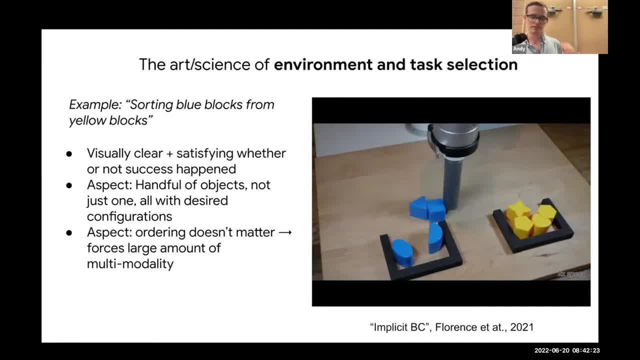 So at any point you know, oh, should I do this block first or that block first, et cetera. It's something that's super easy for humans to think about but can be actually hard to train robots to do. And then another one is for those of you that are maybe 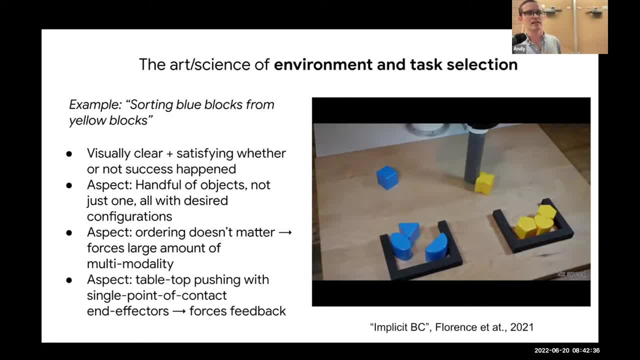 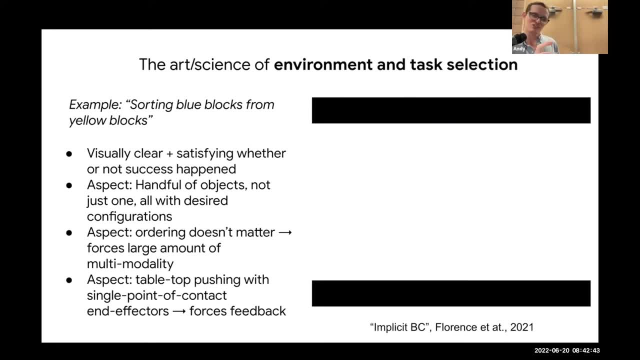 not familiar. this sort of taking a single point of contact pusher and sliding things around on a table is actually a very commonly studied problem in robotics. And yes, we know that we can just go grab the block and move it with an enveloping grasp and it's much easier. 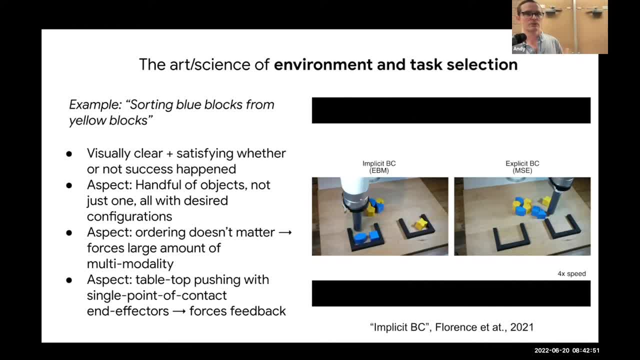 But the act of choosing to just touch it with a single point of contact. It forces you to have a lot of feedback, because it's very hard to predict with a single point of contact where the thing's going to slide, And so it's just a good, simple way. 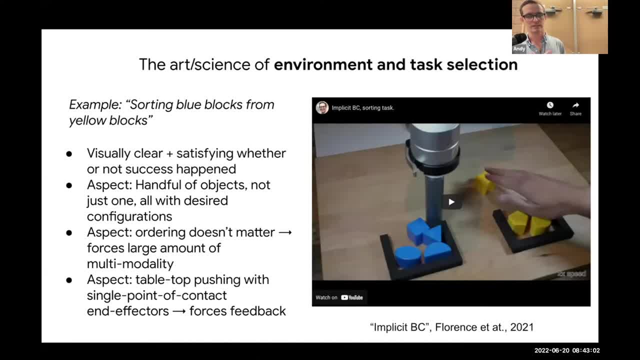 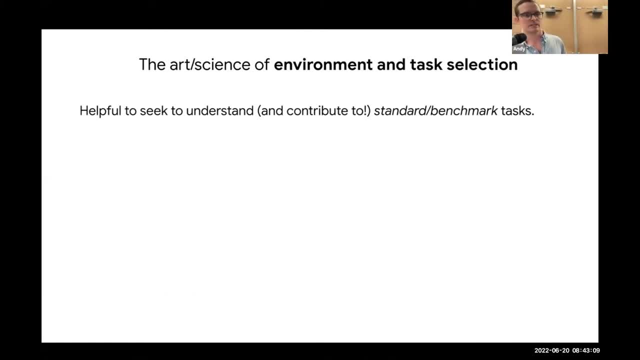 to force yourself to deal with high rate feedback in this case is a thing to study. So that's that. So those are maybe just a couple of examples. But another thing too, in addition to sort of thinking about: oh, how might I sort of maybe set 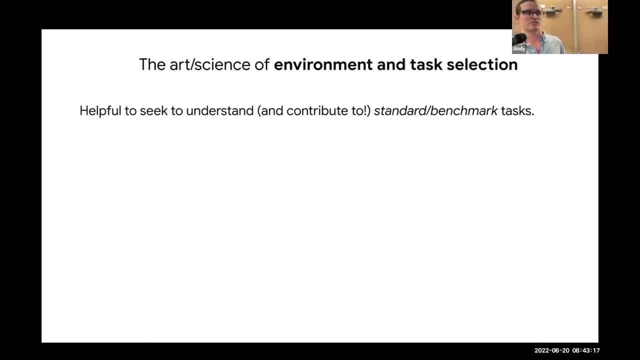 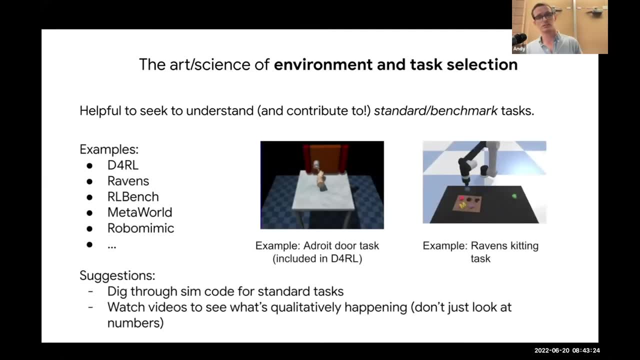 up my own tasks is we also we were talking about, you know, computer vision is great at benchmarking. I think it'll be good for the field to coalesce more and more towards the standard benchmark tasks And I think it's really helpful to sort of take note. 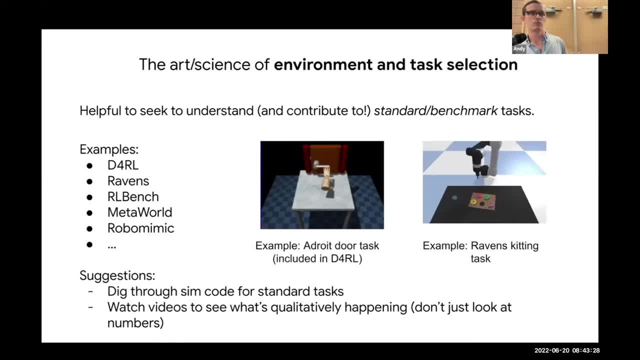 of what's out there already and appreciate what's really nice about some of the things that are out there already. But then also, you know, keep in mind, you know what might you want to improve. And I think actually one thing that happens a lot: 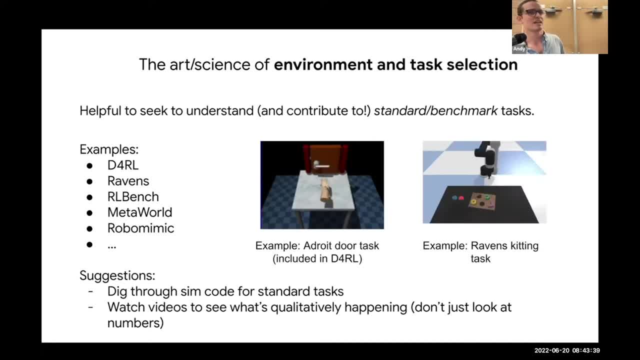 in robotics, benchmarks and things like that is that people love to complain And I get it. It can be easy to sort of get in the like: oh this data set it's not very good because it misses that or misses that. 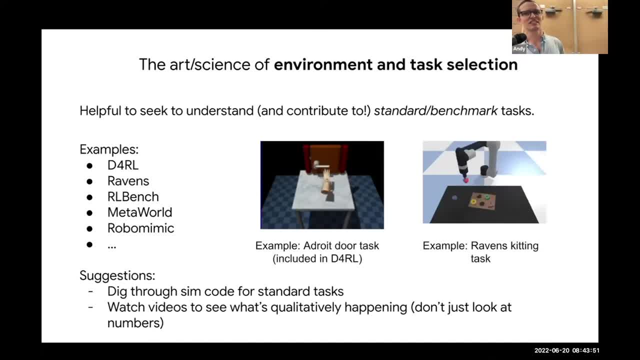 But I would encourage you, you know, rather than playing that game too much, just, you know, get out there and help make it better. And actually, once you start to try to make it better, you'll realize, oh wow, there's actually. 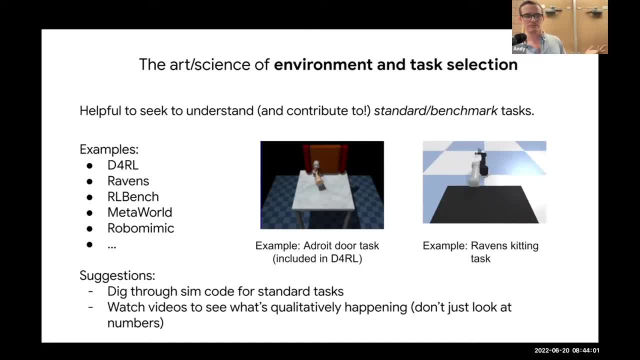 some really cool things about some of these data sets already. So this it's a really nice task, these DROIT tasks, which are included in the D4L suite, but from a different paper from before, but nicely included in the suite. 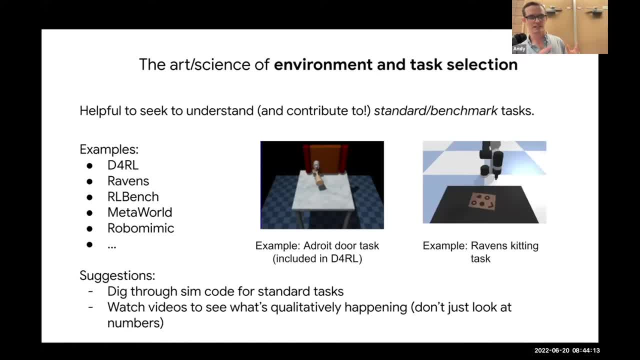 They have some really nice sort of like high degree of freedom: hands interacting with environments. This one's opening the door. This is from Raven's benchmark, which was from the Transporter Nets paper that Andy was talking about. This is just one of the tasks there. 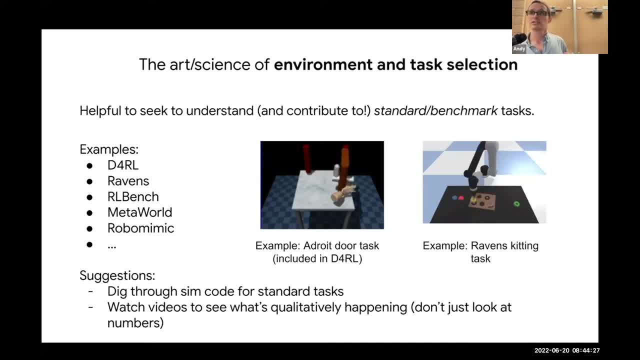 There's a handful of others listed on the left. I encourage you to not just sort of like read the papers, but actually dig through the SIM code for the standard tasks And when you are running methods on these tasks. I highly recommend it's surprising how many people don't do this. 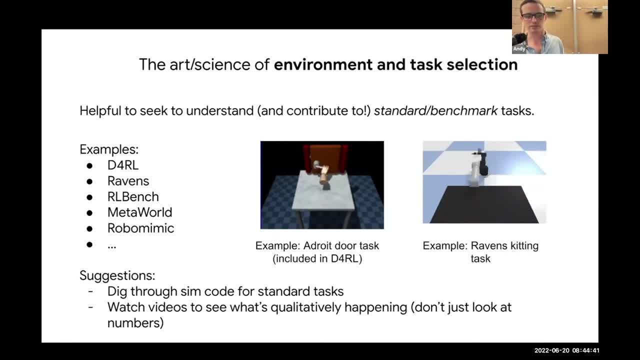 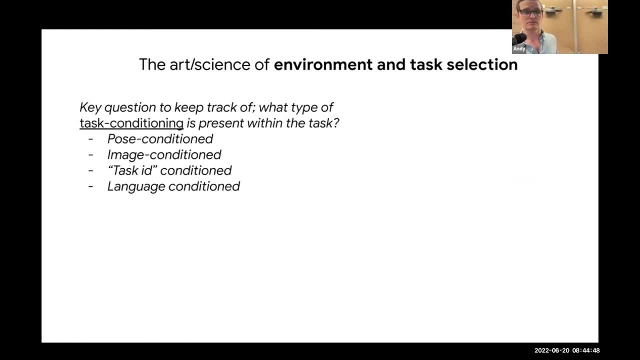 but it's really helpful to actually render it and qualitatively watch videos of what's happening, Don't just look at numbers. Okay, so another key question I think to keep track of with tasks is what type of task conditioning is present. 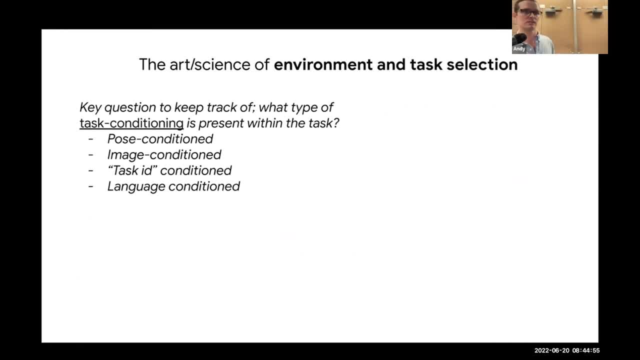 We were talking about the task conditioning with: hey robot, can you move this cup here? It's sort of language. models are sort of an analog of have a huge amount of conditioning Within robotics. when we have tasks, yeah, there's a variety of ways to condition them. 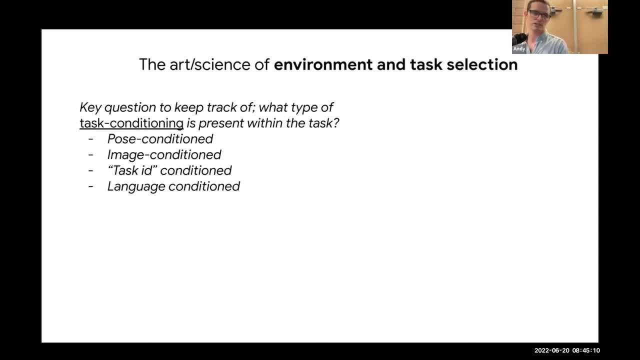 So they could be sort of like object state, like maybe pose condition or image condition, goal image condition or task ID condition, or maybe language is a very flexible way to do it. It's helpful to keep in mind, Actually, the last task that I showed on the previous page. 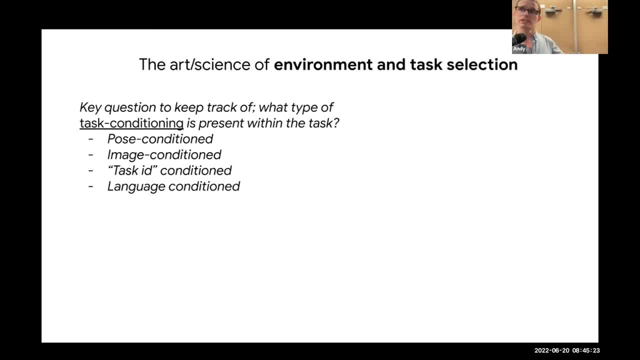 had conditioning in terms of like goal configurations of objects, but they didn't have a goal image. It was just sort of trained to sort of mimic. the demonstrations was the only way that that was conditioned. I think it's really interesting to think about the sort of like crank it up to kind of like the dolly. 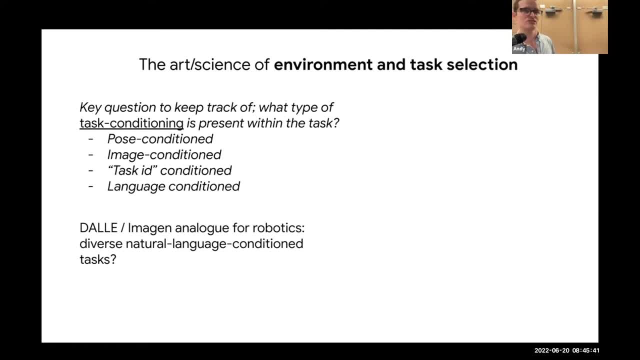 or image, these sort of like very flexible, just text to image generation models like would be the analog for robotics, where we just have super diverse natural language condition tasks. I think that's a really nice point. It's a really nice place to be shooting for. 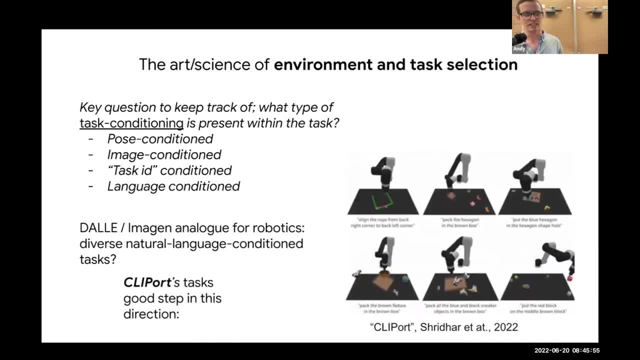 Andy talked about clipboard and it's in the co-op. You know they're not all the way there, but I think they put together a nice suite which is actually built on Ravens from the last slides that I mentioned of having a pretty good diversity. 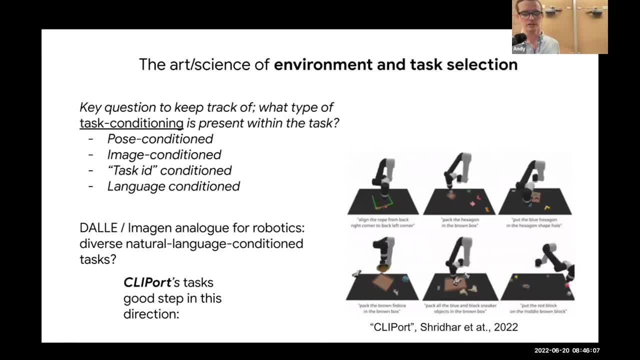 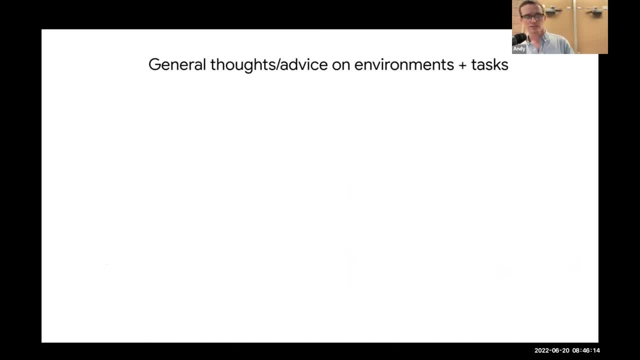 of language condition tasks, And I think that's a good step in that direction. There's other works that also have these types of things as well. This is just one example. I think it's a good direction to keep going. So some general thoughts on thoughts and advising environments. 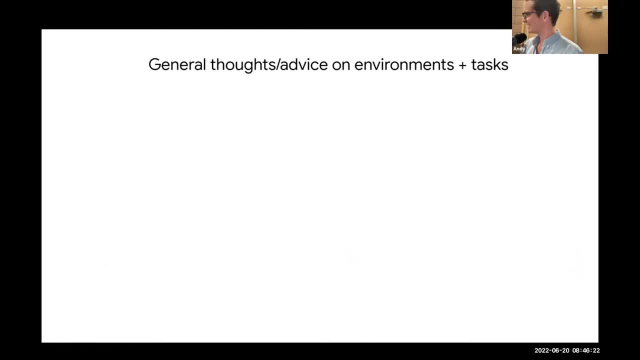 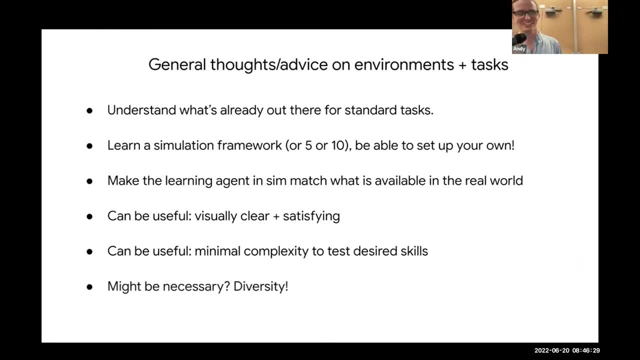 and tasks. also a quick time check. I'm one minute over. Well, let me just okay, I keep going. Okay, so some general thoughts and advice on environments and tasks. Understand what's already out there, Don't just like start building your own thing. 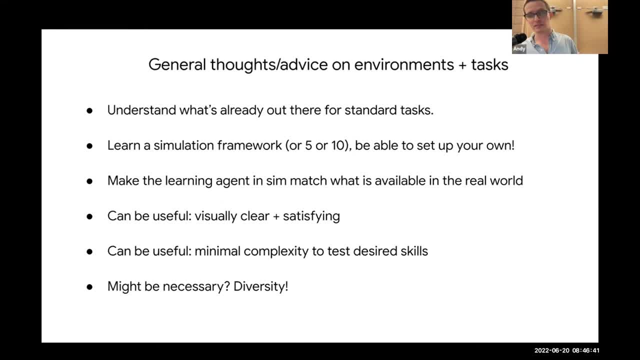 and without consideration of what's already out there, Highly suggest learning a simulation framework, or five or 10 to be able to set your own, set up your own tasks and environments. You can start with the co-op that we shared today and tweak that and you're off to the races. 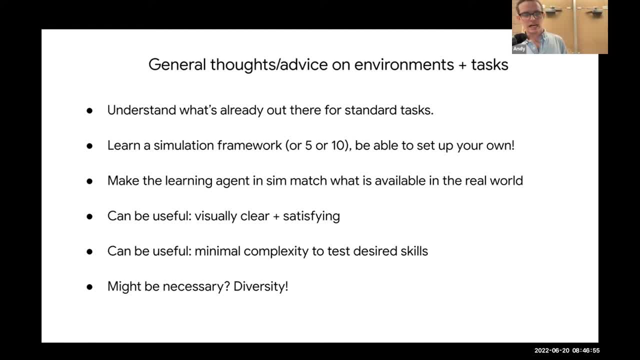 There's a lot of other good frameworks out there too. I think it's really useful to you have a simulation, but like, don't cheat, don't try to cheat too much in terms of what the learning agent actually has, is going to have access to. 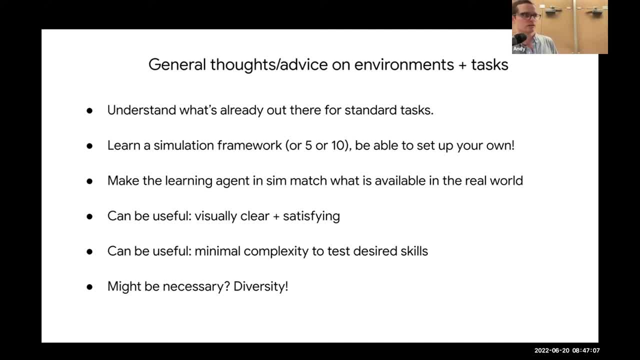 So in the simulator you can have the learning agent, just have full state of every object in the world, but you can't get that in the real world. So if instead you force the learning agent in the simulator to only just use images, then that's gonna transfer over better. 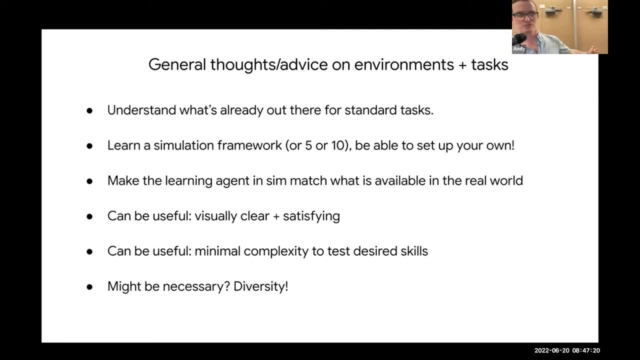 that sort of set up to the real world. of course I think again it can be useful. We talked about it. to have very visually clear and satisfying tasks can be useful to have the minimal complexity needed to sort of test the desired skills. 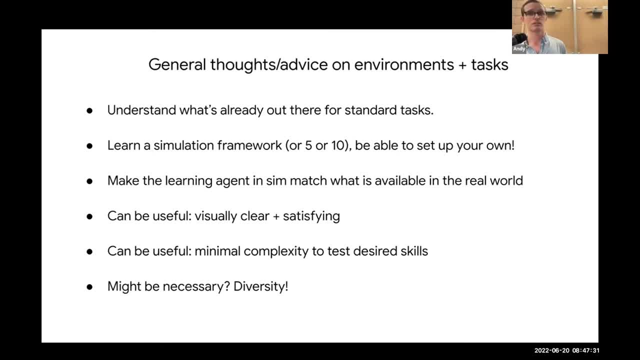 We talked about that with the co-op in terms of it's just a few blocks and a few goals, but it sort of gets at the right level of diversity. there Might be necessary to have a bunch of diversity. And another thing too, maybe I sort of already tried to review this upon you. 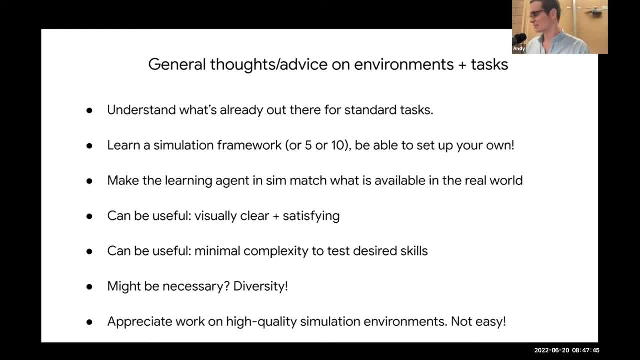 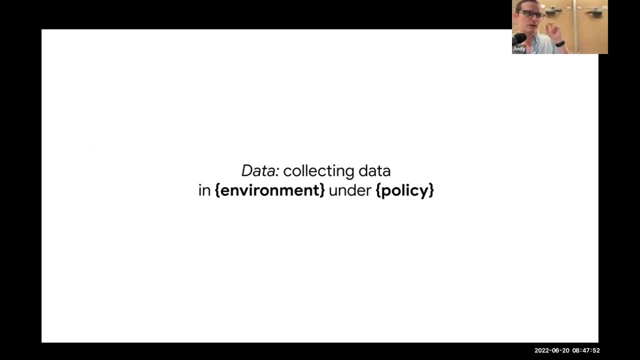 but like appreciate the work that goes into high quality sim environments because it's not easy. Okay, so data. There's basically just one thing I wanted to say here with data, which is that data and robotics is kind of tricky Because data means collecting data in some environment. 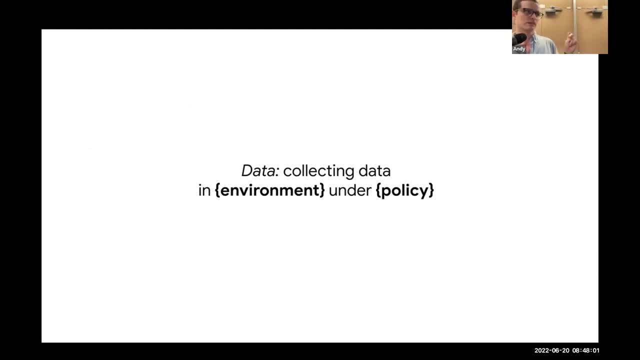 under some policy. It's that last part which, if you're not familiar with the way we collect data in robotics, that's the way, ooh what? So I'll just talk to that real quick. So one thing on the environment is I just wanna note. 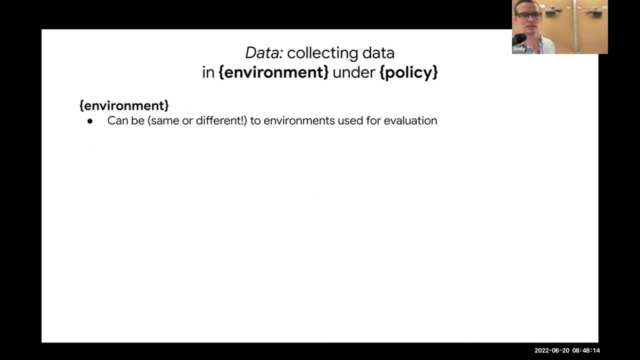 that the environment in which you get your data can either be same or different to the environments that are used for evaluation. That's something to know. But with the policy, I think this is again quite interesting, in particular to robotics. So in robotics we care about temporarily sequential data. 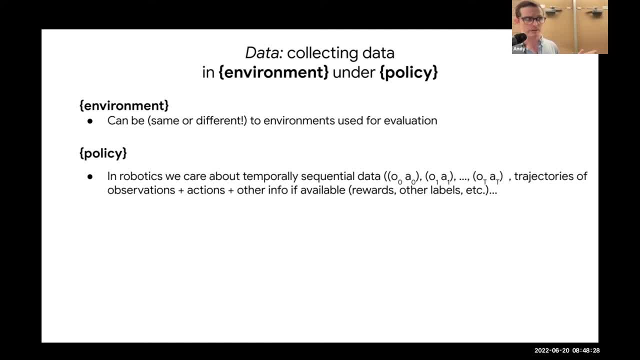 So trajectories of observations and actions, maybe other things too, But the key question always is: what was the policy that was used to get that temporarily sequential trajectories of observations and actions? That's the key question. And what was the policy's goal? So maybe you have taskless sort of data. 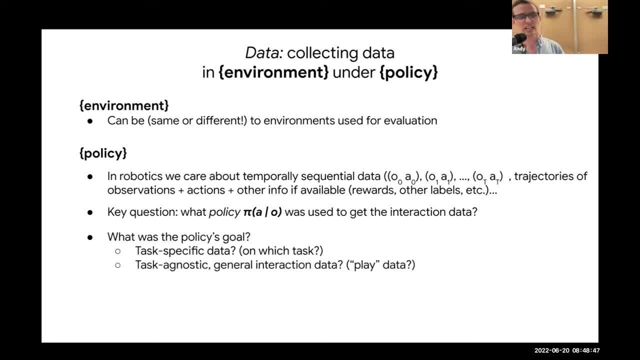 but also another very interesting direction to look at is sort of just have task agnostic, that's. it's helpful to be more specific than that and sort of in different instances. but there's at least a sort of informal notion of quote, unquote, play data. 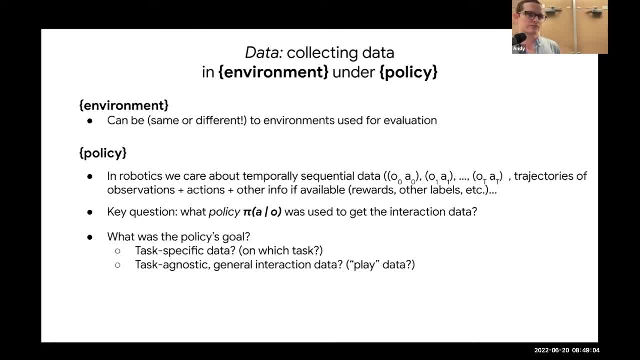 where you just kind of have general data of an agent sort of interacting with an environment- Maybe it's humans that are just sort of playing around and just doing whatever comes to mind for them- And then also think about who is providing the data. So, in addition to what's the goal, 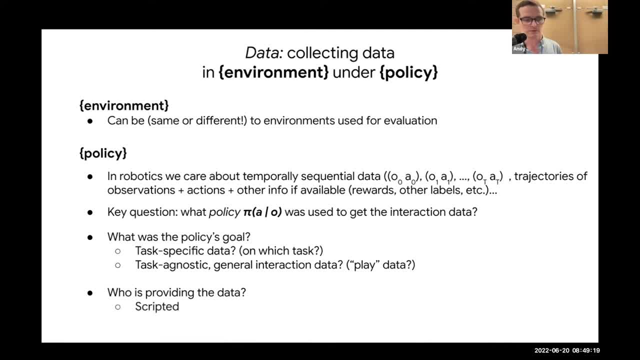 the sort of reward function, so to speak, of what policy is operating under. who is providing the data? In the co-op that we provided today, the data that is used to train the policies is from a scripted policy. I think it's a really good recipe for just setting up. 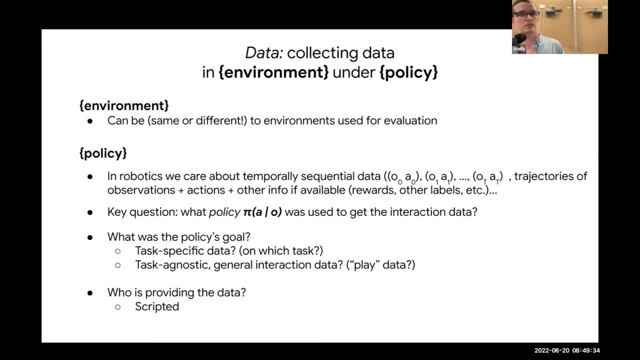 hey, you wanna do a learning based robot, train it to mimic some scripted policy? Super nice, because then you can just you wanna change your task, just change your scripted agent, you're done. You just need to generate the data out of that scripted policy. 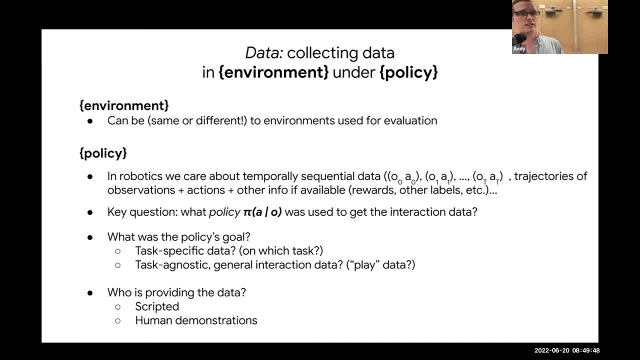 Another option is human demonstrations- Another very interesting option, I think. personally I think it's the most interesting because I think it has the best sort of relevance to sort of real world robotics And there's a lot of interesting challenges with multimodality and non-Markovian nature. 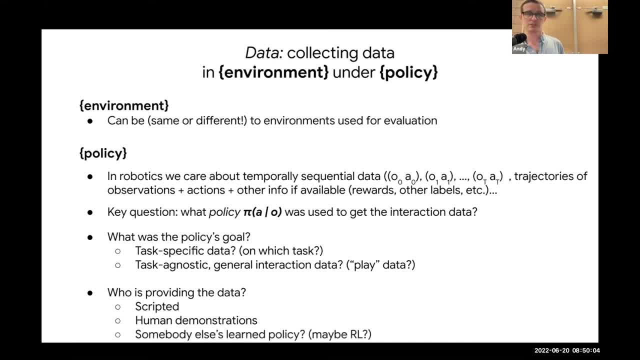 of human policies. Another option too, though, is to use somebody else's learning policy, or maybe you have your, maybe that's from RL, or maybe that's from something else, But these, I think, are kind of the three main options to help to keep these in mind. 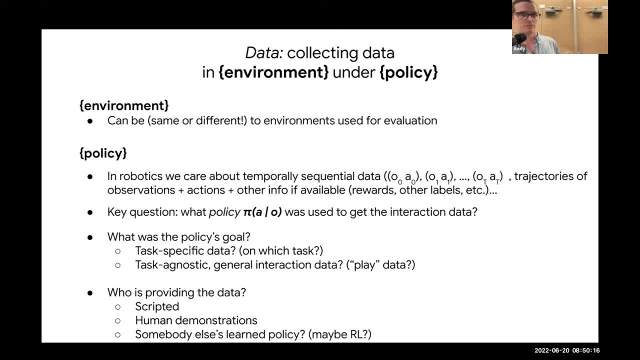 So again, you don't just have data that comes out of nowhere In robotics. we have temporary sequential data Like: what are the actions that were chosen over time? It was operating under some policy. What was that policy? Very helpful to keep in mind. 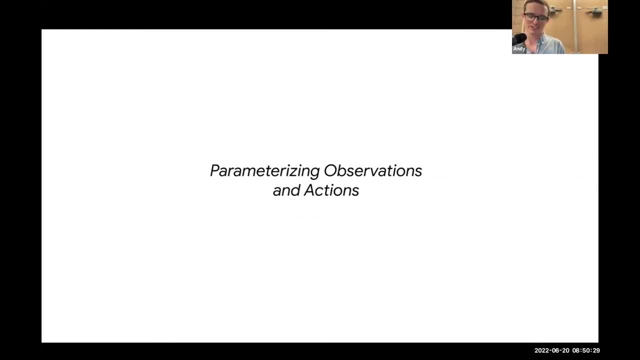 One that is. I think it's kind of niche, but I think it's like very important and it's sort of unavoidable and sort of agnostic to. whatever method you use is just how you choose to parameterize your observations and actions. I'll go really quick because I am quite over time. 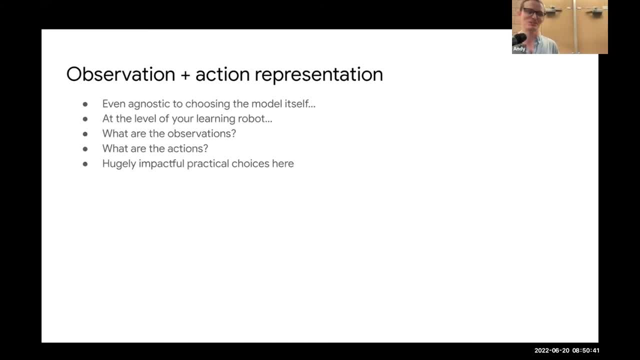 but okay, maybe, I'll maybe not go too quick. But so even agnostic to choosing the model itself, but the level of like. what fundamentally are you learning, What are the observations and the actions into your learned agent? This is a hugely impactful practical choice. 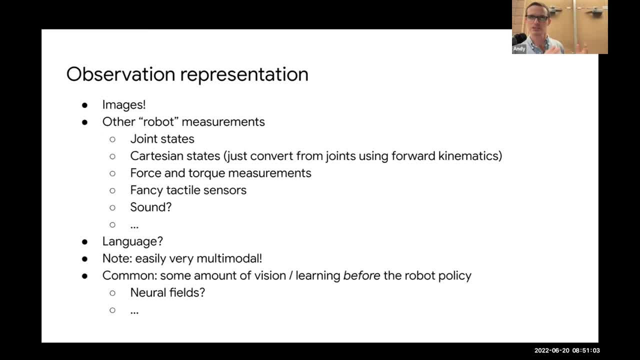 On the observation side. it's maybe the simpler side. Okay, whatever images- We're at a computer vision conference, We love images. I do think images are the most important sensors for robots in most cases that I'm interested in, But there are a bunch of other things. 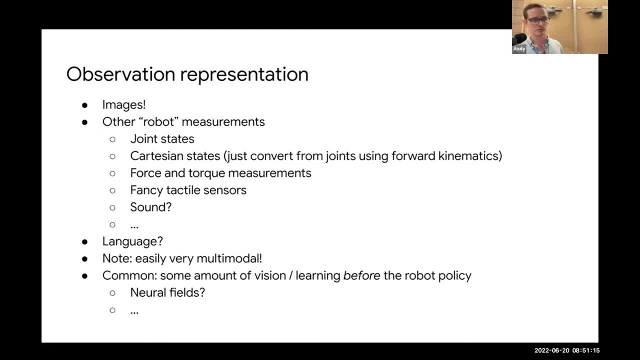 you get from the robot joints. Cartesian states. force torque measurements, maybe fancy tactile sensors. force torque measurements, maybe fancy tactile sensors. force torque measurements, maybe fancy tactile sensors. It's fancy because they're not really sort of mainstream. Yeah, they're very cool. 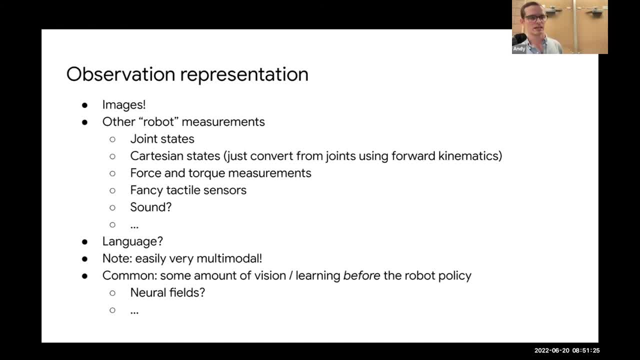 Sound, I think is underutilized. Maybe you have language coming in, A lot of different options. All this is very multimodal. There's also it's very common in robot learning research to kind of pre-process some of the kind of raw. 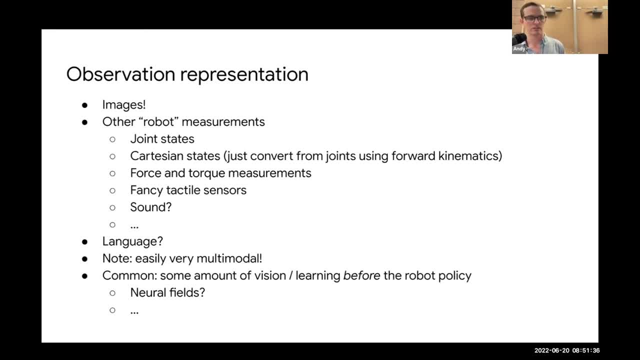 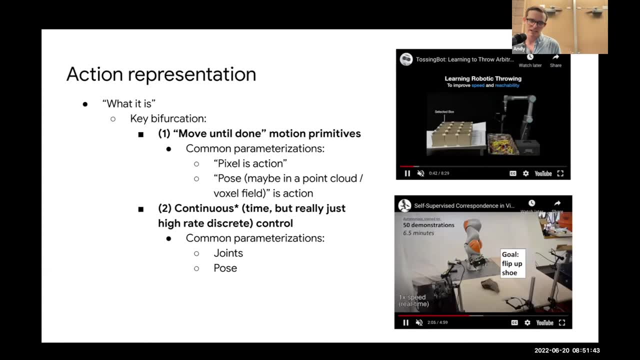 imagey stuff into something that is then kind of considered an observation to your robot learner. So maybe neural fields or whatever. it's going to be A lot of different options there, But I think it's the action side where there's a little bit more subtlety. 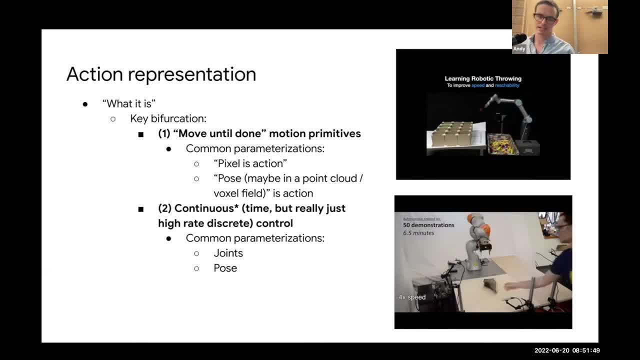 So a key thing that I think is really important, a key bifurcation that Andy sort of hinted to in the co-op, is that there's really two main ways that people parameterize actions for learning-based robots One, and there's lots of pluses and minuses to both approach. 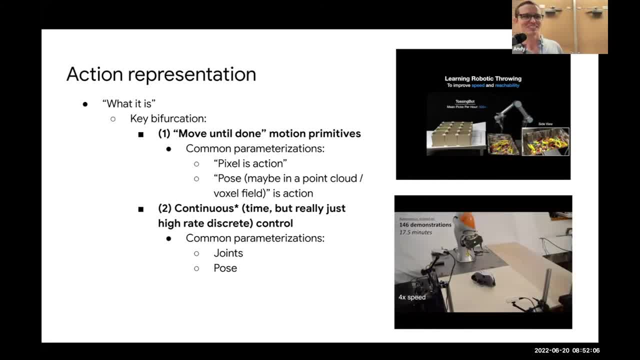 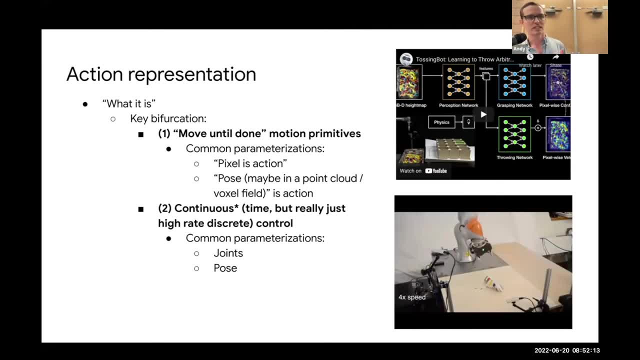 One is kind of Andy called it. we have a lot of different names. There's no like good standard names for these. So if anybody has a better option, let us know. But we sometimes call one like sparse control or motion primitives. 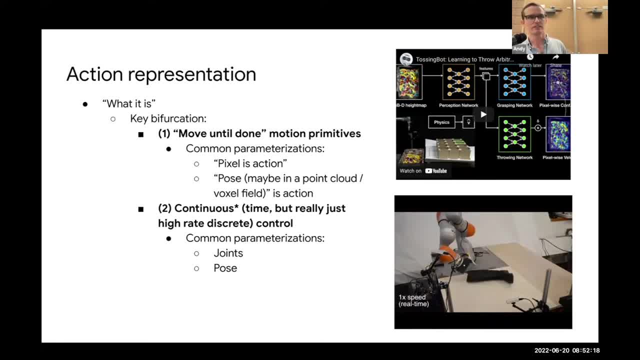 But the key aspect is you move until you're done. So you sort of look at the world, you choose a thing, and then you might be moving without sort of revisiting your learned policy component for maybe a few seconds. And that is actually the type that's operating. 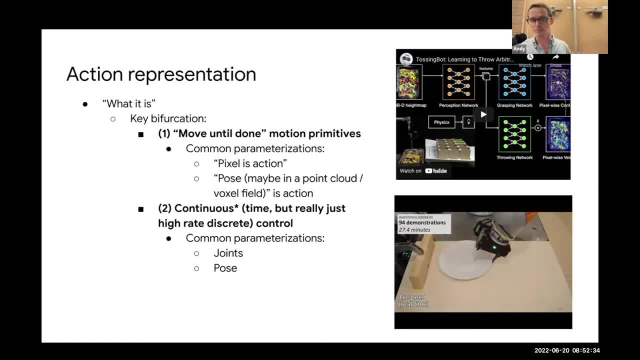 in the co-op that we gave out today And some common parameterizations of how we might sort of parameterize the learner in terms of what it chooses, what is its action is. you can consider like sort of pixels action, which is a really nice setup. 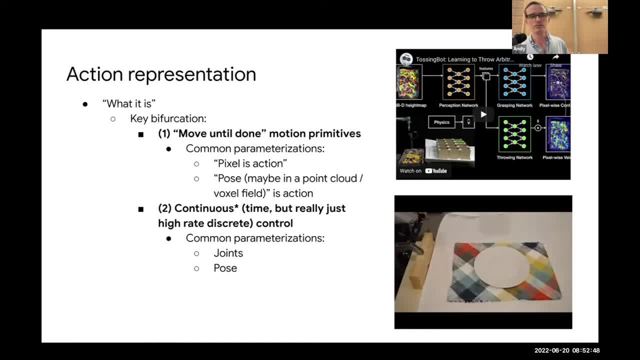 and works really nicely with a lot of computer vision tools. Maybe a pose like maybe in a point cloud or in a voxel field is an action. That's one way to do it. I'll come back to why these are good choices to use this sort of motion primitive style. 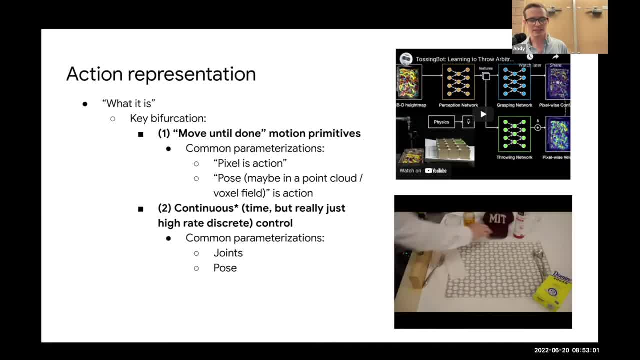 Another option. it's kind of a misnomer, but the way that people usually talk about it is they call it continuous control. Note that by continuous they're really referring to time, but it's not actually continuous time, but it's just kind of high rate discreet. 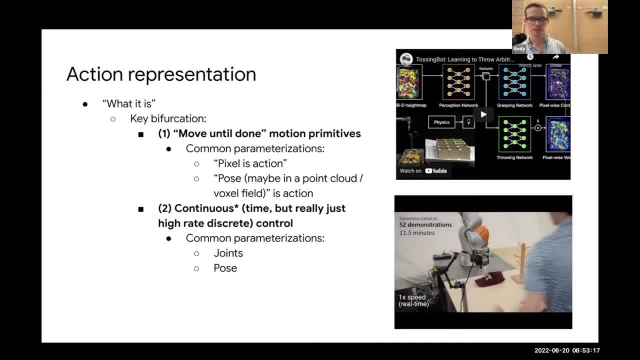 sort of in the range of maybe five or 10 Hertz, something like that. People usually call it continuous control, And there's an example on the bottom right of doing continuous control where, at 10 times a second, the robot is deciding what it should do. 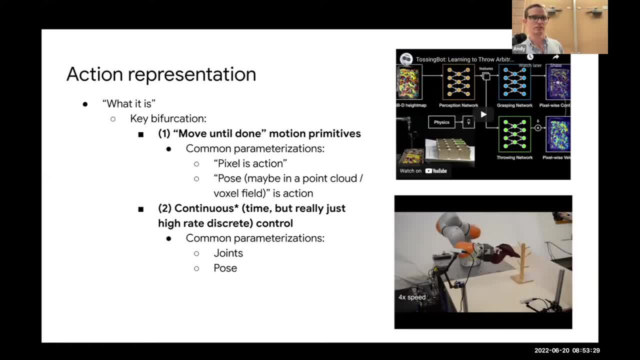 And one of the advantages of this type of setup is that you can have actually like real time reaction to what's happening in the world. A downside, though, is this direction is much harder to work in practice, I think, and to get to generalize, 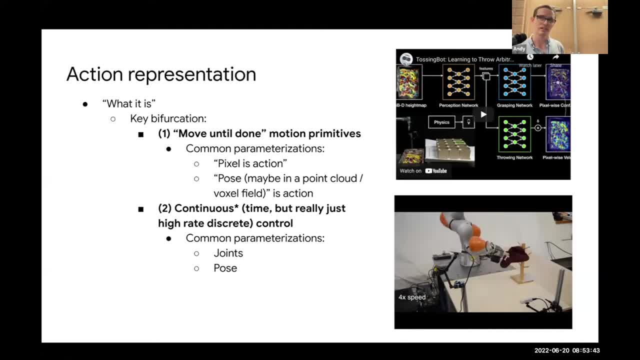 over a lot of different scenarios and it requires a lot more data. So you need to be like logging all of your data at full, 10 or 30 or higher Hertz. It requires a lot of data, Whereas the motion primitives approach. 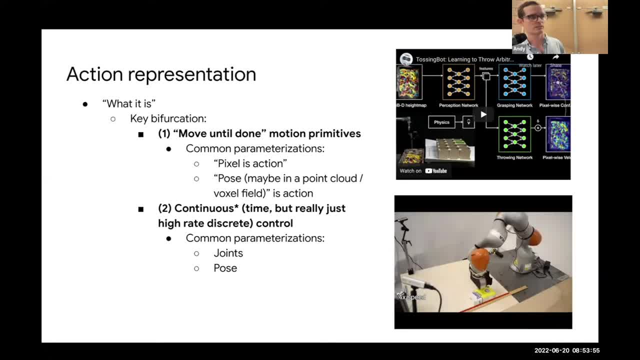 you can formulate very simple efficient learning. You need to log a little bit less data from the robot. I think in practice also too, in terms of robots that are out in the world making money. most of them are using some sort of. 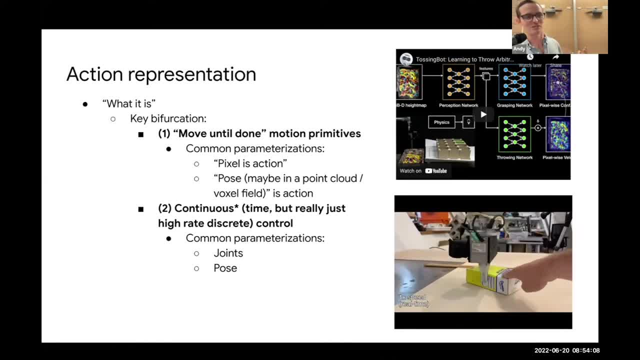 if it's a learning based robot sort of all these like bin picking startups. they're all using this sort of first one of motion primitives. It's just a very practical choice. The second one maybe in the long-term could end up. 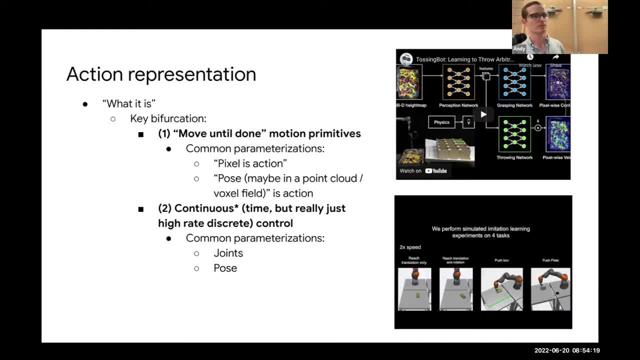 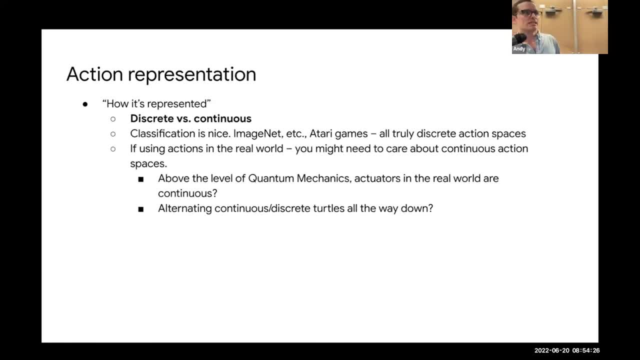 it's sort of by definition, could kind of subsume the first one, but it's a little bit harder and trickier to get to work in practice. In addition to like what is, are you doing those two different versions I talked about? 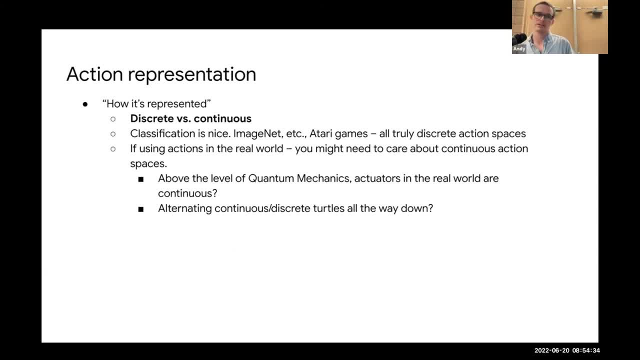 There's other ones, but those are the two main ones- is: how is it represented? The key thing here is discrete versus continuous. Let me just quickly say that classification and discrete choices are very nice, but in the real world, at least above the level of quantum mechanics. 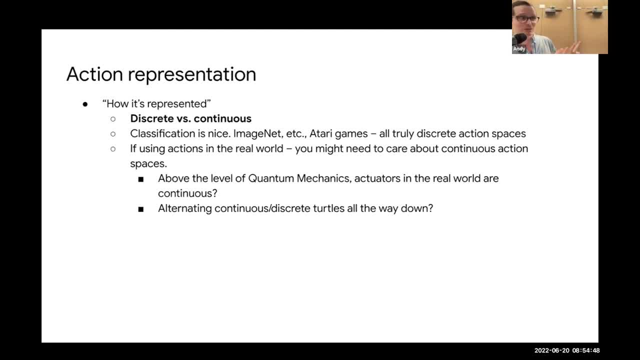 all actuators in the real world are continuous. So maybe you have a suction gripper which is quote unquote, a binary, you know, on off actuator. really underneath there there's a bunch of physically continuous things with voltages that can be changed continuously. 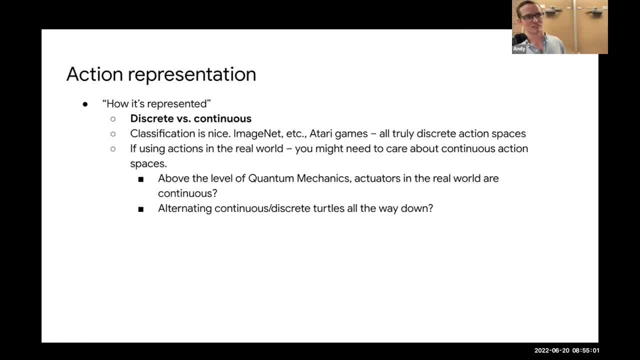 It's really continuous. but wait, it gets trickier than that because digital control is cheap to implement And so actually often, even when you have continuous things, it's PWM with a digital signal, And so I just kind of think about it. 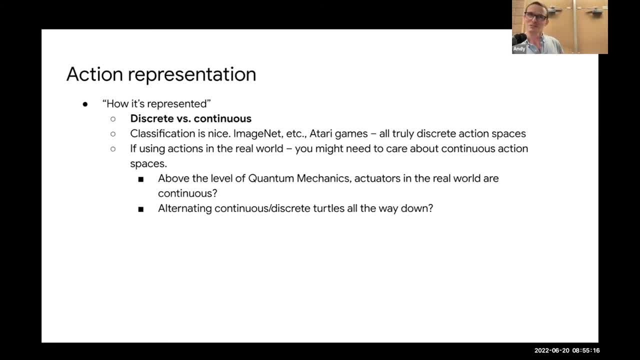 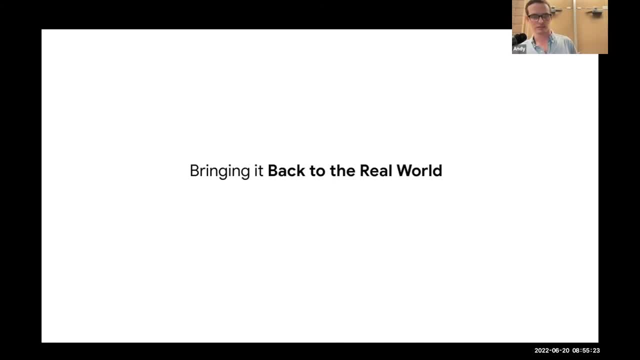 as alternating continuous discrete turtles all the way down. it's really tricky, but I at least want to try to impress upon you that continuous is important And you should at least consider thinking about continuous action spaces, which come up with a bunch of trickiness to them. 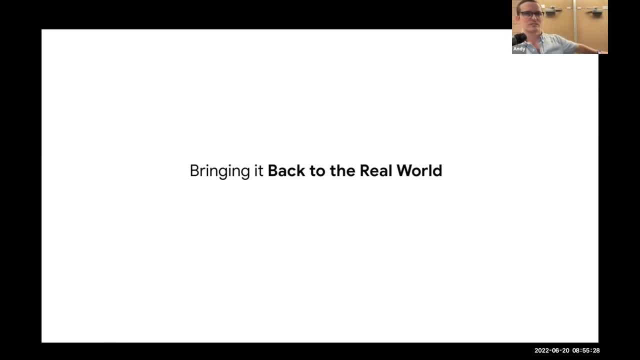 One quick thing on bringing it back to the real world. We just talked through a bunch of different concepts that can kind of be instantiated, maybe out in sim. But again, I think it's really helpful to bring it back to the real world every once in a while. 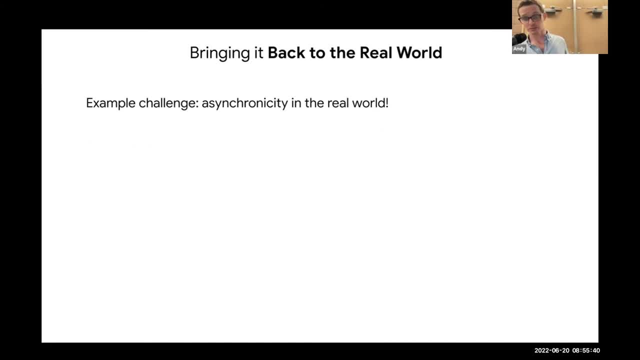 Just one example of this is that asynchronicity in the real world is really hard. So maybe in your simulator you set it up with perfect, discrete, indimension, discrete MVPs, Markov decision process, where your observations come in all at the same time. 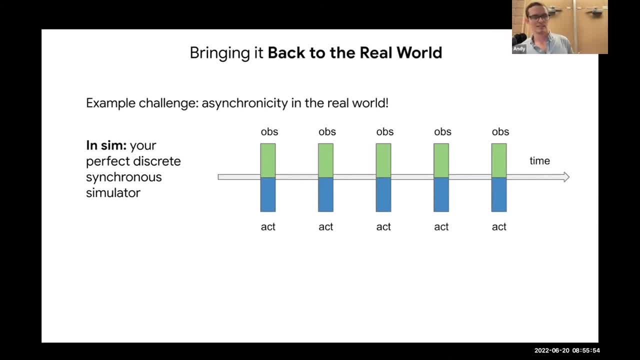 and you have an action all at the same time, and you can take as long as you want to. The time doesn't even really move linearly. You can take as long as you'd like to just decide what happens and you're good to go. 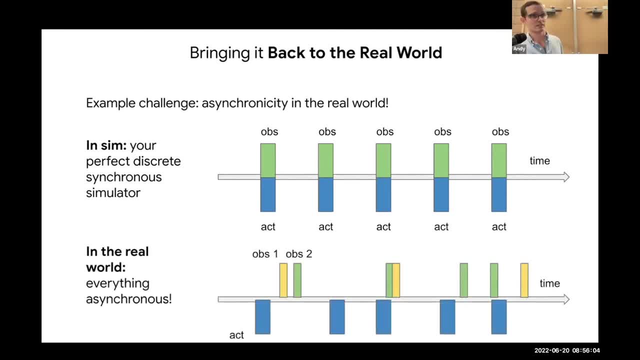 But in the real world, actually, all of your observations, they come in asynchronously, not necessarily at the same time. Sometimes the sensor doesn't hit its desired rate And then also your actions are happening all asynchronously too. And also, by the way, 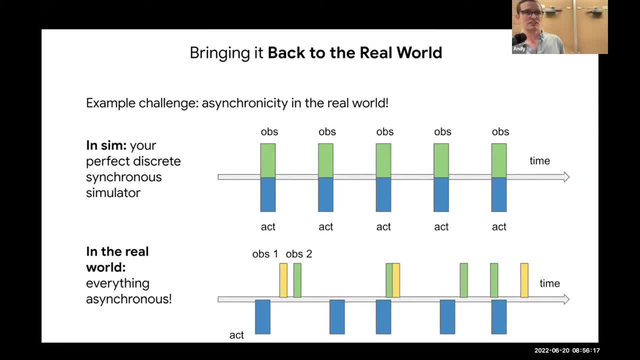 while you are running your machine learning model, the real world hasn't stopped. You have to deal with the latencies and the models, and there's all these tricky things that happen basically because of the setup. So that was the toolkit that I'm putting forward today. 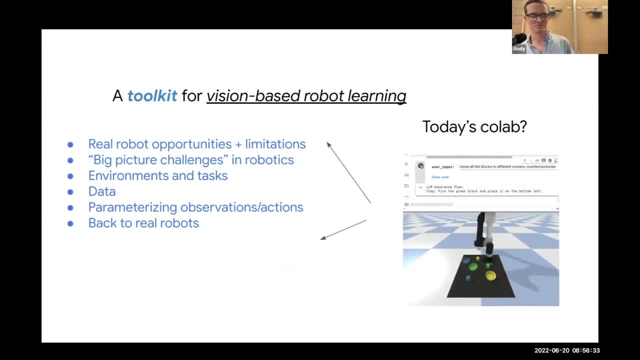 Is it fully comprehensive? No, but maybe it helped think about how different things fit together and what are some important things in the field. And again, I think there's a lot of nice connections with the co-op from today. The co-op is, I think, addressing definitely some. 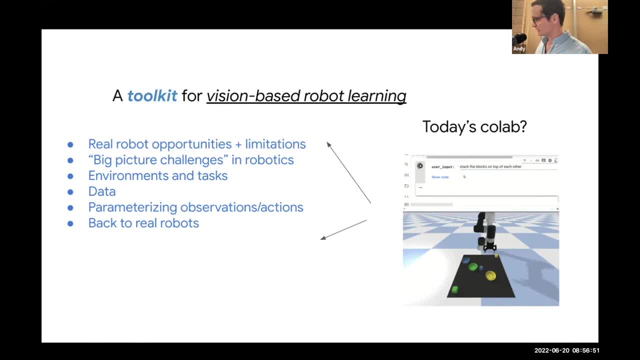 of the big picture challenges in robotics by sort of tackling data challenges with, on the vision to action side, very efficient architectures and then also leveraging large pre-trained models from other areas. So when Andy will go through later more with using LLMs in robotics contexts. 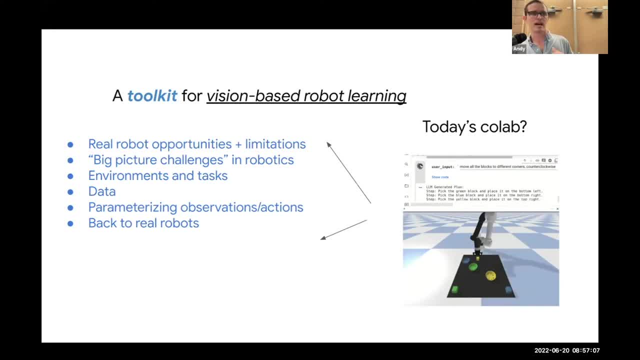 We talked a little bit with Andy earlier about how the environment and task was sort of nice and simple and set up to test just what we wanted to do. The data was collected by scripted policies. The actions are parameterized as these sort of move until done motion primitives. 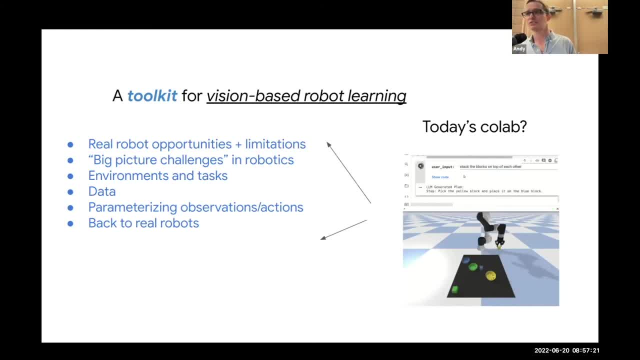 And back to real robots. Well, I can leave you to. if you end up forking the co-op and doing your own thing, you can go run something like this on a real robot, which I highly suggest you do. Cool, That's all I have. 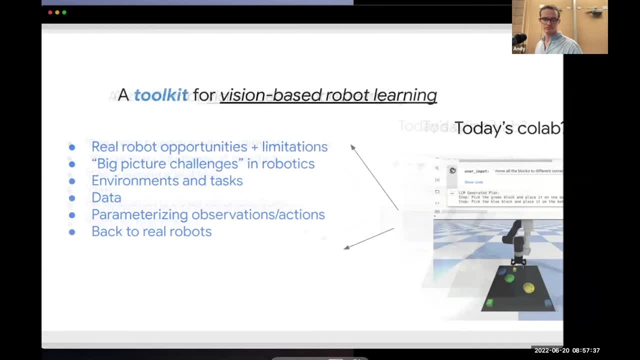 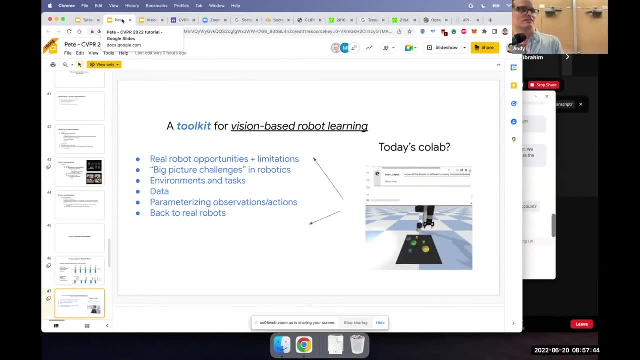 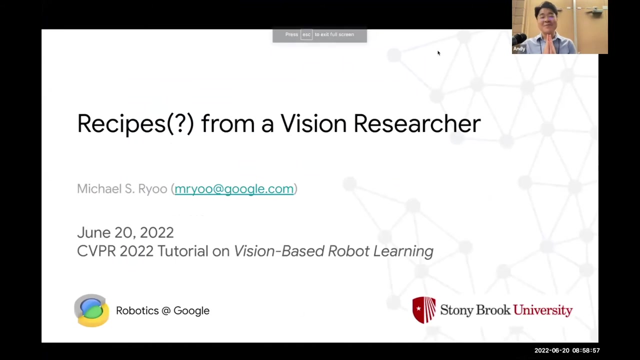 If anybody has any questions I'm happy to take, But I'm also happy to go on to the next speaker to let it take more time. So I'm going to essentially share my experience as a computer vision researcher in doing robot learning research. 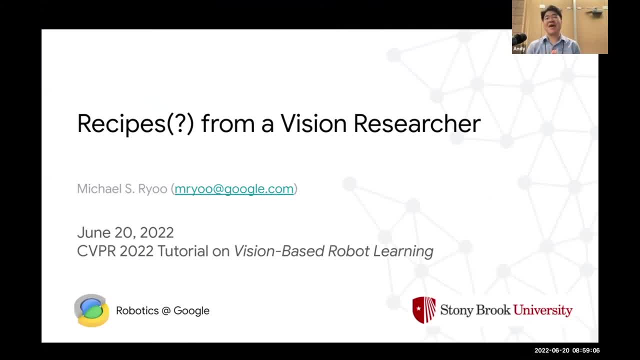 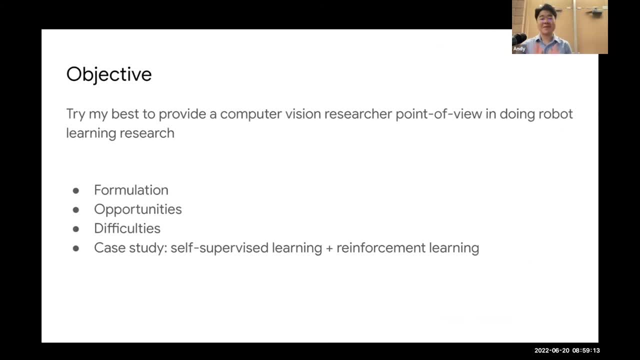 Some of this will actually be echoing what Pete just presented, which is good. So what's the objective? As mentioned, I would like to share my experience- my computer vision researcher point of view- in doing robot learning research. I plan to talk about the difference. 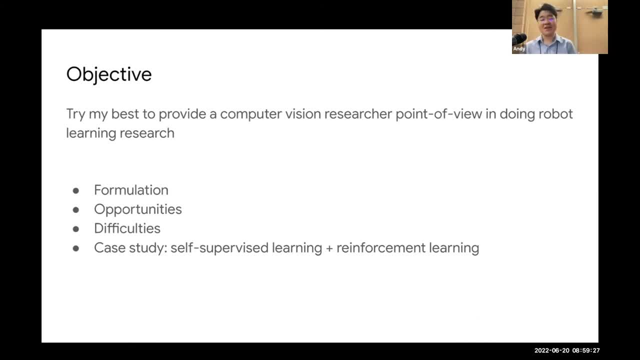 between computer vision and robot learning in terms of the problem formulation, discuss about the opportunities, discuss about the main difficulties- the difficulties I face so far- and also share my experience by talking about a case study, which is about combining self-supervised learning. 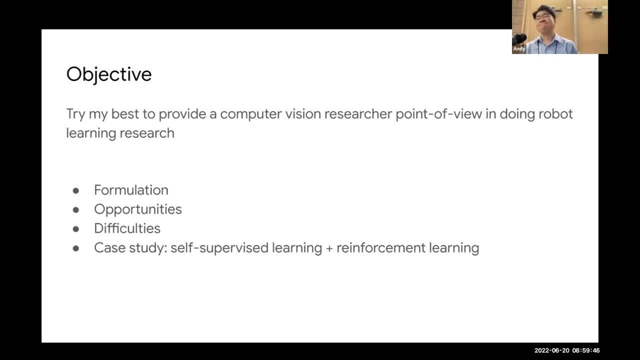 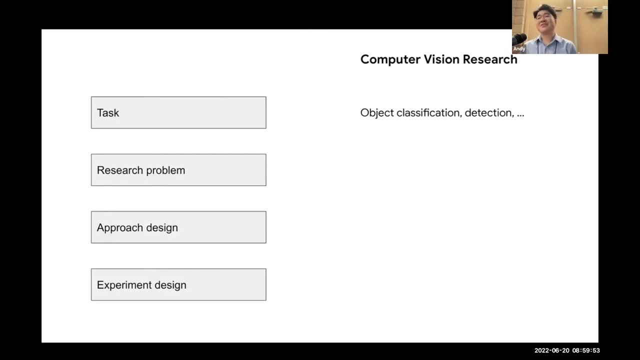 and reinforcement learning and, as I mentioned, how it failed. OK, So when I think about doing computer vision research, there are several components, several decisions I immediately think about. So imagine yourself as a graduate student and assume that you want to work. 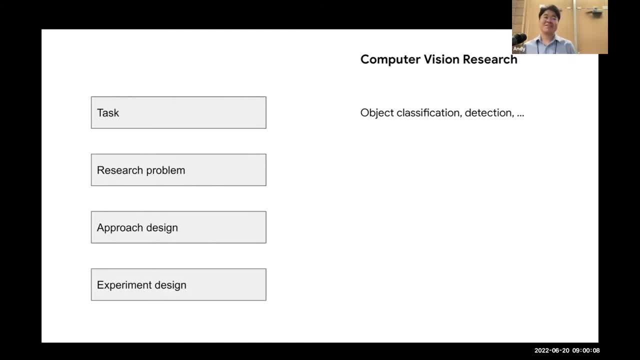 on a research project, a brand new research project. There are several decisions you need to make. One decision is obviously what computer vision test you will be focusing on. It could be something like object classification, object detection and so on, But you just need to make a decision. 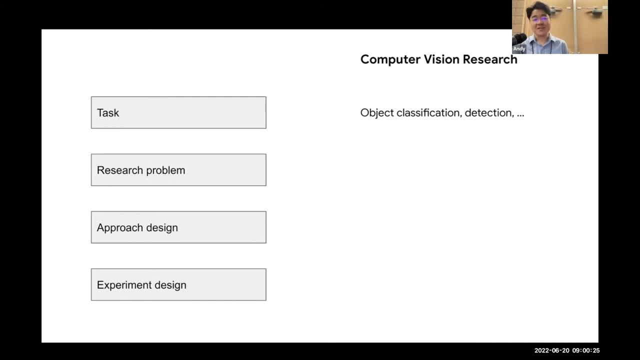 And then another component, once you decide on the task, is about the actual problem: research problem, such as learning better representations from large language models, which is a popular topic, and so on, After you decide on the idea or the problem. well, 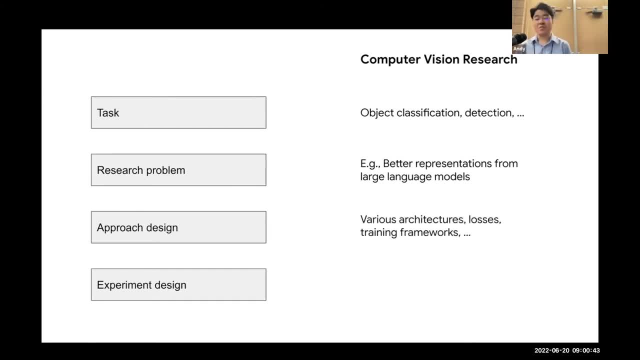 you'll need to design an approach. There could be various different types of model architectures. You can focus on the different, you can focus on the training framework- and yeah, there are so many. After deciding the approach, obviously you also need to design your experiments. 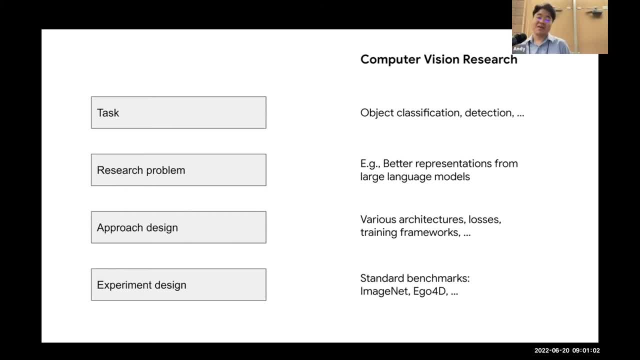 And we usually go with standard benchmarks like ImageNet or something like new and fancy like Eagle4D. And if you actually ask me which part among these four is easiest, as a computer vision researcher, I would definitely say it's this one. 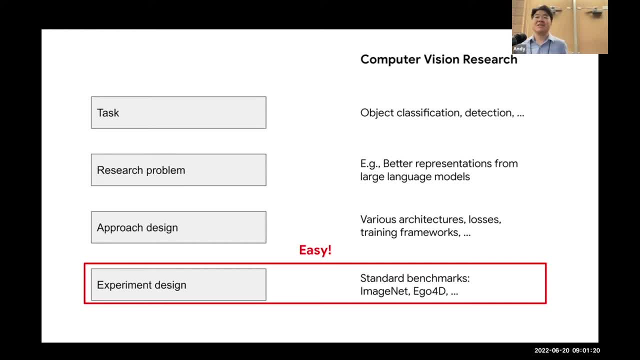 I mean, once you decide to work on object classification, ImageNet is a must. We cannot really avoid it. We cannot convince anybody without testing it on ImageNet, so I don't even need to think about it. I just try to follow whatever people have been using. 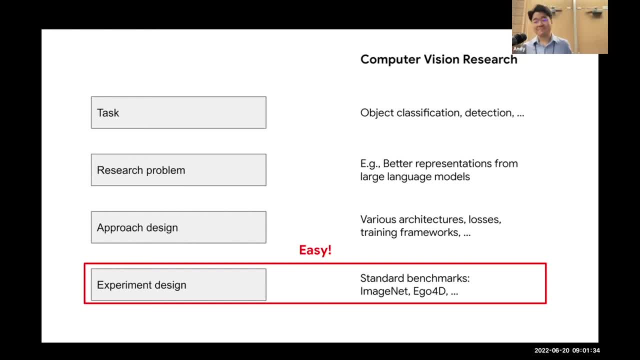 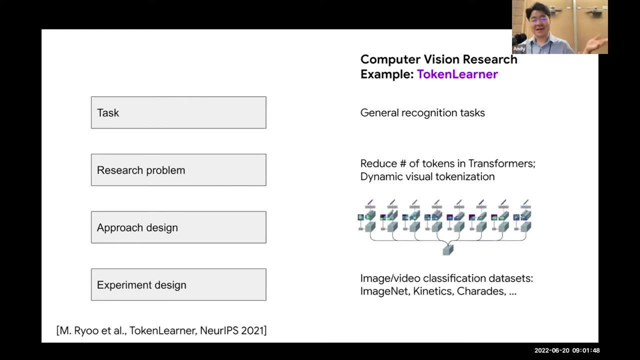 in previous papers And that's pretty much it. And sorry for embarrassingly bringing my own paper as an example, but this is TokenNano And if you look at the TokenNano it actually kind of falls into this kind of flow. The test in this case was a general recognition. 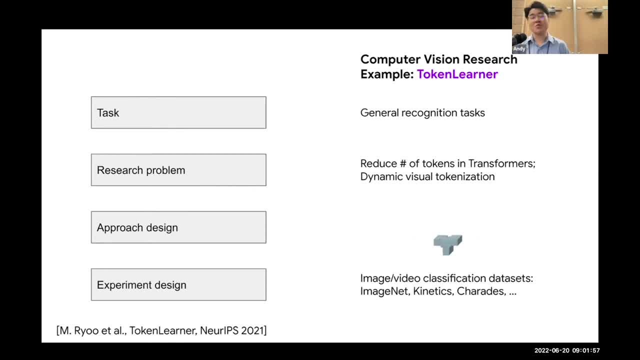 including object recognition and video recognition- mostly image classification and video classification- And the motivation I don't know. The problem I wanted to focus on was essentially reducing the number of tokens in transformers and do some dynamic visual tokenization, And there was an approach to implement this. 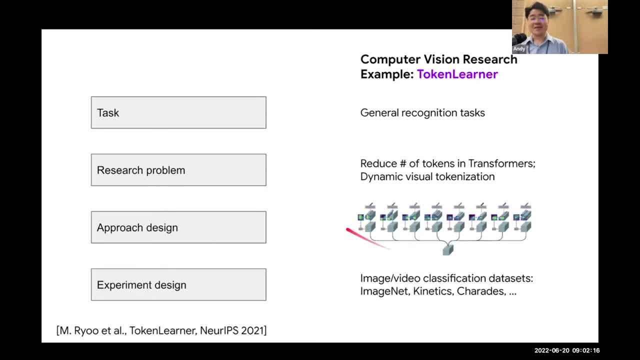 in the form of the spatial attention mechanism, And then after that, yeah, the decision for me was pretty easy: I had to use ImageNet, I had to use kinetics, I had to use arrays, And that's how things went. Now let us try to think about what we need to do when we are 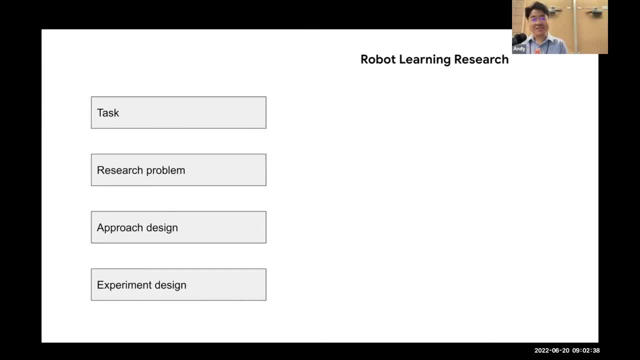 doing robot learning research. In terms of the task. there are many different robotics tasks But in particular, what we are talking today is action policy learning. It's not really too different in some sense from what we do in computer vision. We are essentially trying to learn a function: learn. 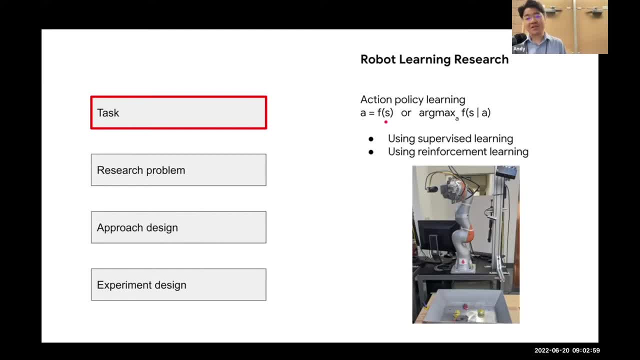 a model that will provide you on action given your state, or give you some score energy of state given action. So in this case, your CNN, your transformer or your model will be taking like two different types of inputs, But other than that it's pretty identical. 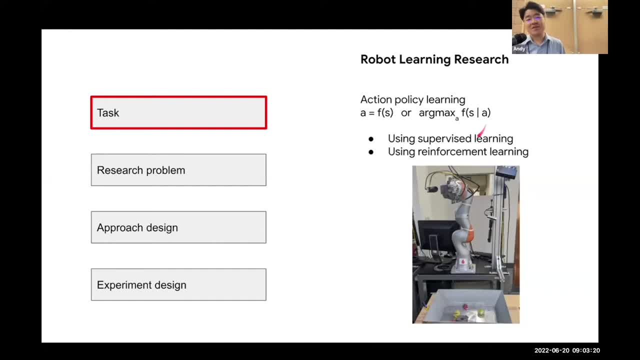 to what you have been doing so far. There are different ways to train such model: using like supervised learning, and it becomes more like behavioral cloning, or you can use reinforcement learning, and there are like well-prepared theory, framework, code and everything that's ready for you. 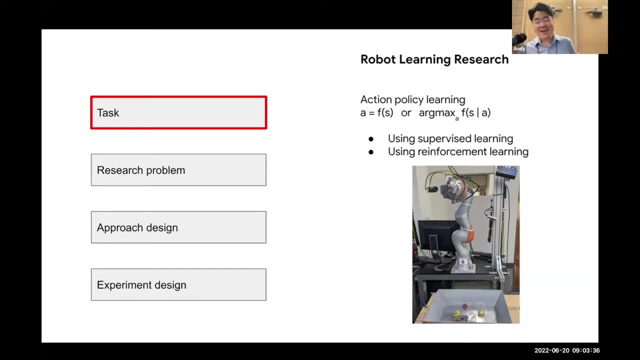 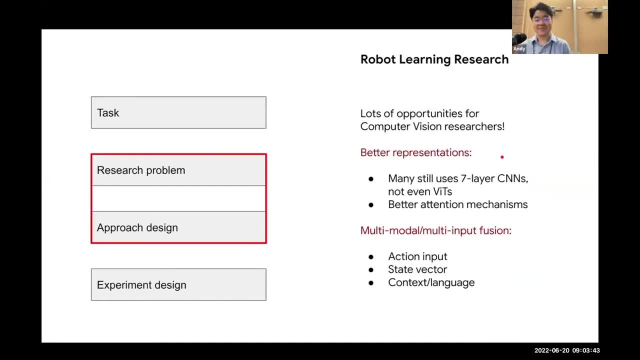 So in some sense, this is what you need to do. And then the good thing is that there are so many computer vision researchers can benefit in terms of the research topic and the actual approach. There are lots of opportunities. We can actually contribute to robot learning research. 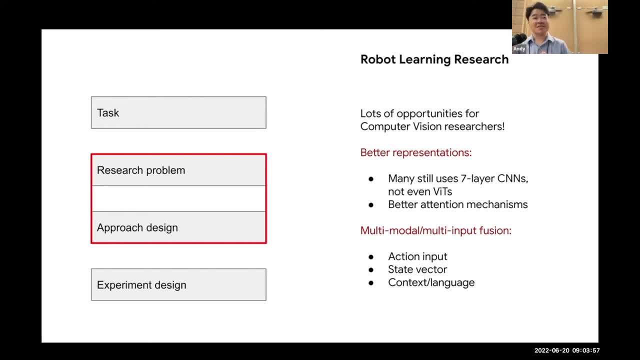 by coming up with better representations. Very surprisingly, many of actual like robot learning, research papers, even like one year ago, they were still using like basic seven-layer CNNs, not even like VITs, I mean, if I publish a paper, a computer vision. 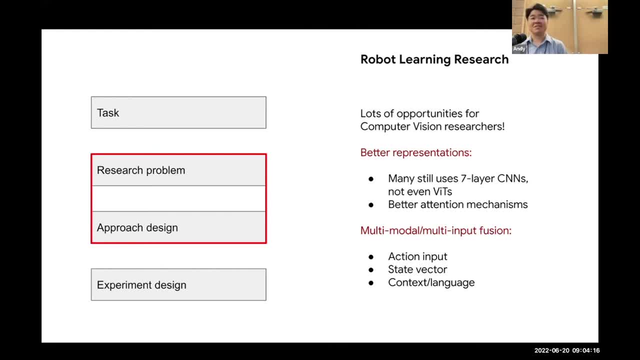 saying that, oh, I use VIT, I'll get a huge amount of criticism saying that, oh, VIT is outdated. But in robot learning, even with the seven-layer CNNs, they were the reinforcement learning from pixels and imitation learning, and everything was being- I mean, was being- 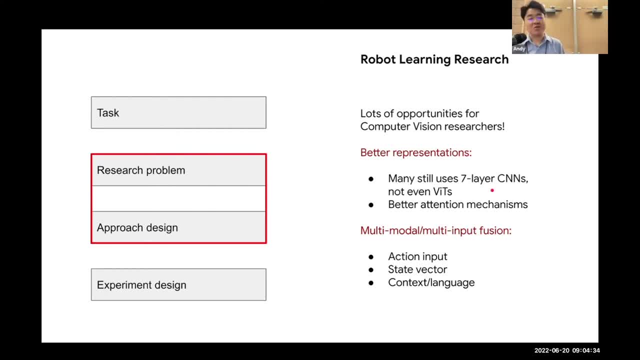 done successfully, so they were taking advantage of it, but we all know that this is limited and there is a huge amount of opportunity. I'm also as mentioned the formulation of action policy. learning naturally leads to multi-input fusion. there is like action input. sometimes it's multimodal. there is 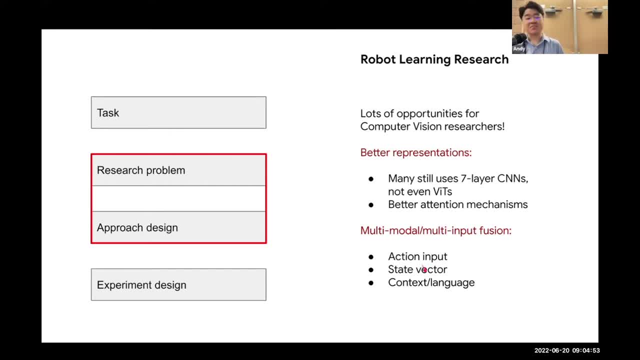 other types of data, audio language, sometimes the state vector telling the configuration of the robot, and there has to be naturally on the fusion and as computer vision researchers we are really good model architects. so there is a lot of room for us to benefit. and again, sorry for bringing my own paper as 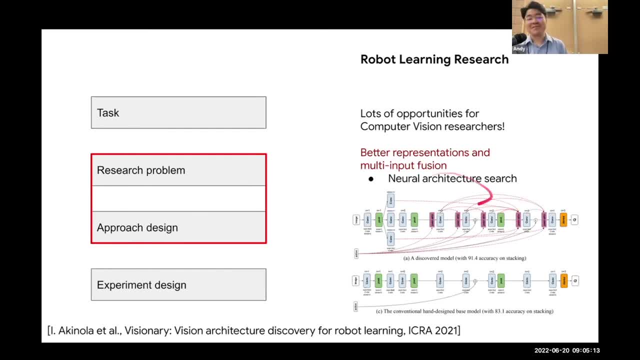 an example we did, I mean- and this was regarding better representation and multi-input fusion, and in this case I already did- was run a very simple neural architecture search. so this was the kind of state of the eye model as I mentioned, like five convolutional, sorry, seven convolutional. 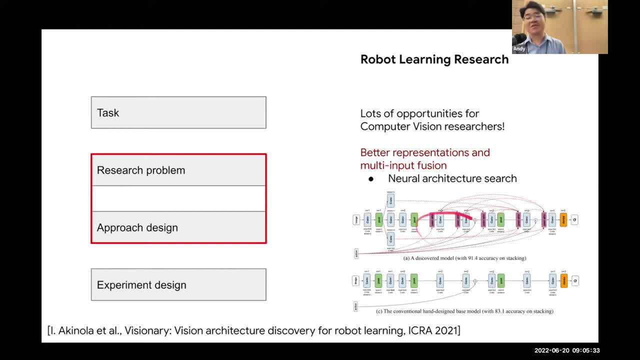 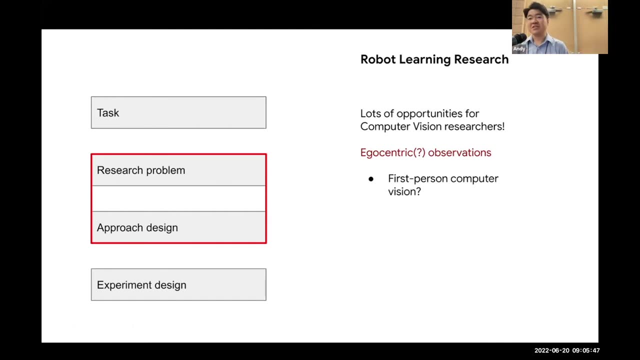 layers and so on, and we were able to find a better model by doing neural architecture search and that was giving us better representation, allowing us to improve the test success accuracy. another aspect is that once we have like robot images, many of these robot images are egocentric or robot centric, so 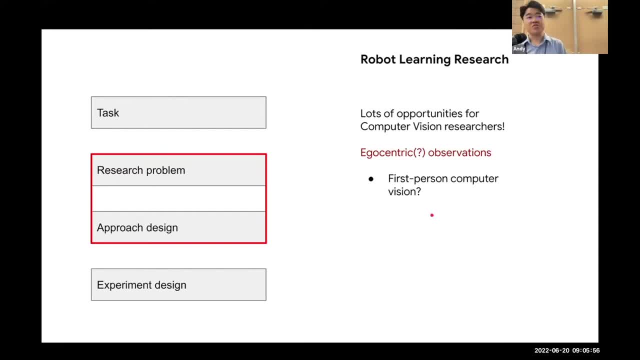 first-person computer vision or egocentric computer vision. research in our area can also particularly benefit robot action policy learning by doing better state representation. another example will be about learning dynamics model. so if you are able to like, learn to hallucinate what the robot will look like. 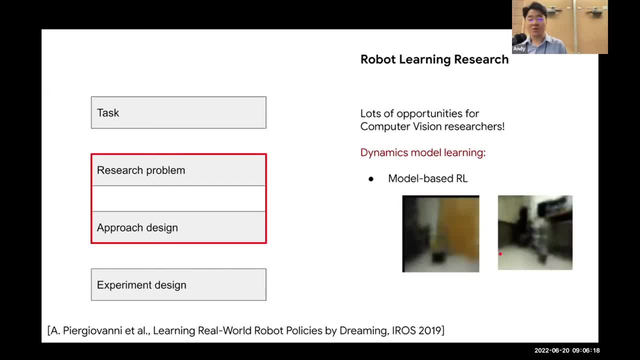 essentially learning a simulator using GAN, autoencoder or different types of approach, different types of approaches. you can directly plug something like this in as an as model into reinforcement learning, as model-based reinforcement learning. So learning of generative model also has a good opportunity to benefit action policy learning. 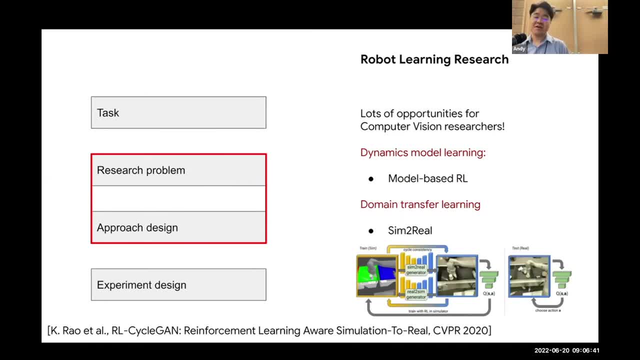 Another immediate thing is about sim2real. So there is a gap between simulator and real world robots, but we ultimately want to benefit real world robots, Meaning that we have lots of training data in sim and we want to transfer that to real world robots. 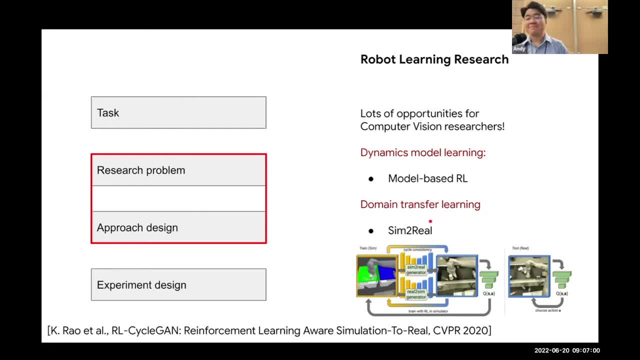 And as computer vision researchers, we kind of have this research area of domain transfer, learning, And this is the exact application of domain transfer in some sense. And as you can see, yeah, this was done and was published actually at CVPR. 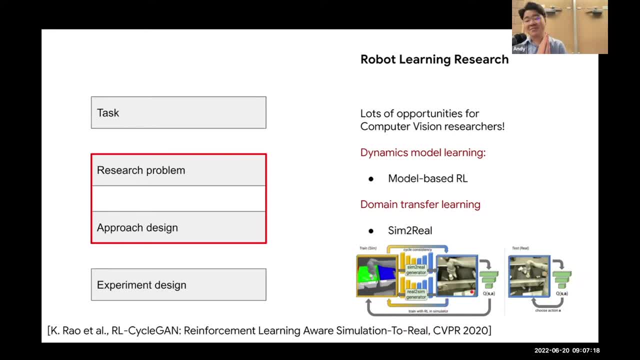 And you can see that this is a hot topic. I mean, this is an important topic and there is a lot of opportunities we see here. Okay, so these are lots of opportunities. I mean- and I'm just listing some examples- 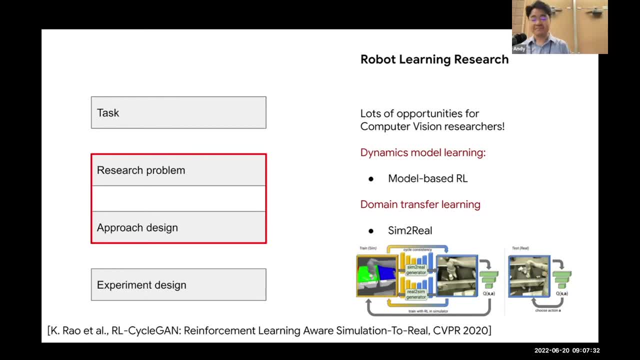 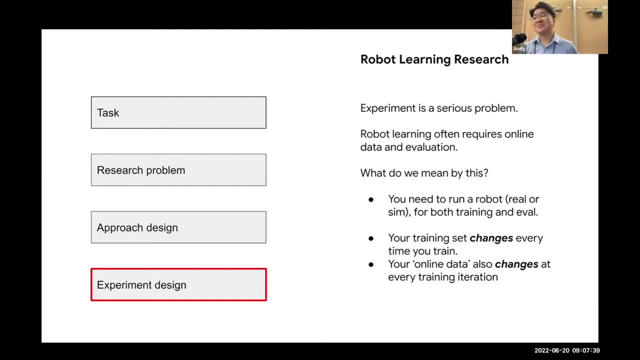 and of course, there are many, many more you can think of. But when it comes to experiment design, it's the opposite. When I was talking about computer vision, experiment design was the easiest. Somebody already did this for you and you just had to follow. 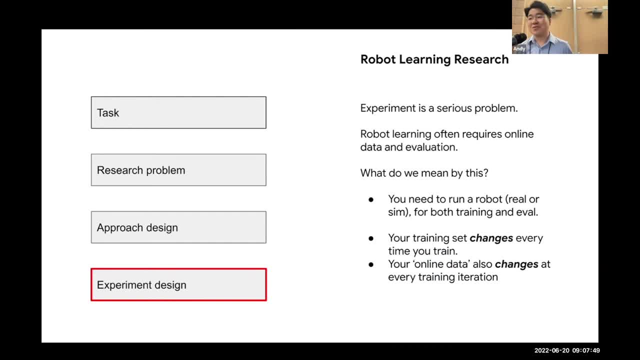 But here in robotics, this becomes a serious problem. essentially echoing what Pete also presented, Robot learning often requires online data and evaluation by its nature. What do you mean by this online data and evaluation? It essentially means that you need to run a robot. 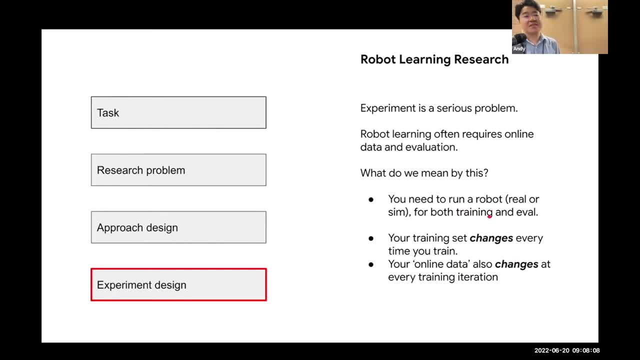 in real or in sim, for both training and event. Okay, what's so bad about running a robot? Well, once we run the robot, there are things that happens. Your training set is essentially obtaining online data, Meaning that what you use for your training, 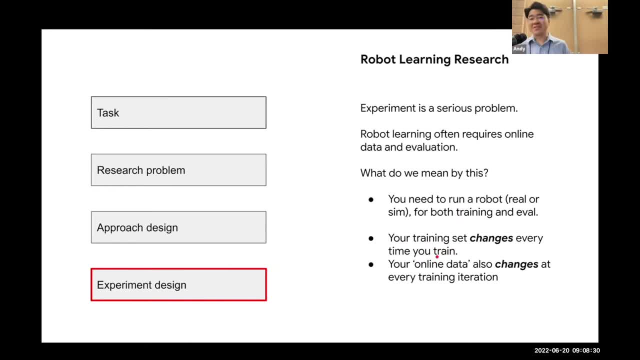 changes every time you train, So, based on different random seed when you initiate the training, the data you will be obtaining on its way will always differ, And it's more like you are training your computer vision model every time with slightly different data set. 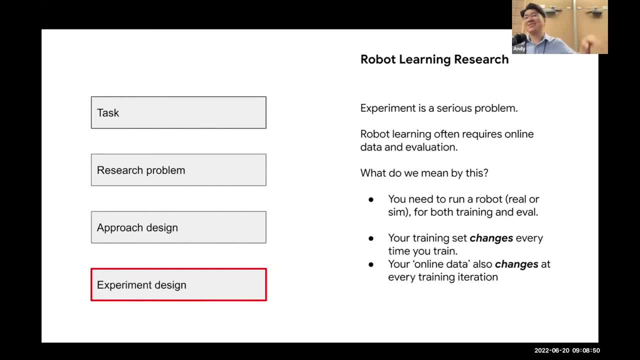 And you are still expecting their accuracy to be stable. the final result to be stable, which is not really. Another thing is that, since you are doing online data, you're using online data. this means that your data changes during the training. 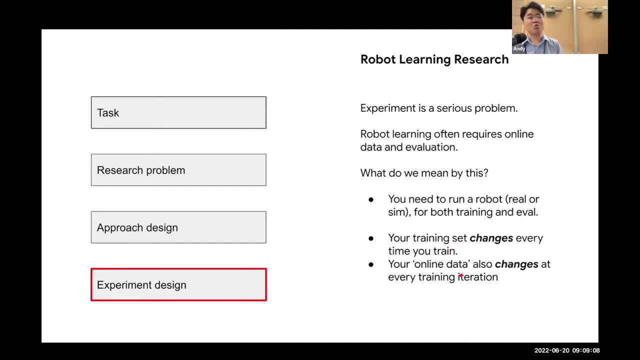 So, as your robot is interacting with the environment and seems more real, you get new data and that's what you are supposed to use for your supervised learning or reinforcement learning. And because it changes, there is a distribution shift: Training this data distribution shift. 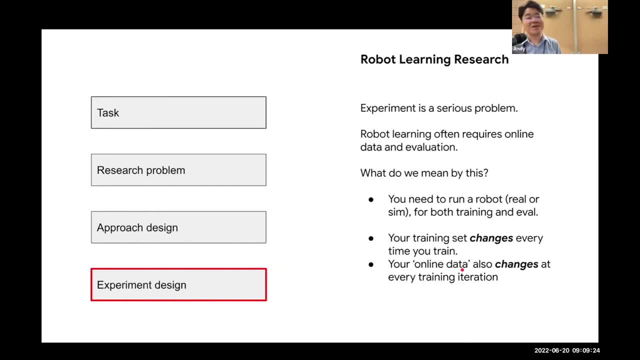 And there is also data distribution mismatch. Go to the Excel page and addろう Meanwhile, go to files and go to the plank Dataек. really, I'd recommend you to try to use this data distribution shift, now fetch, because this online data will differ from training and evaluation. 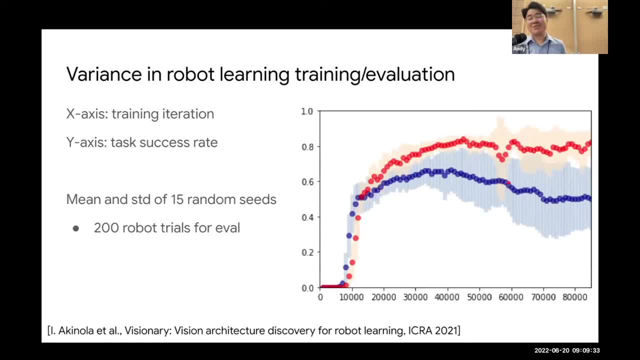 And here is an example. So this is the architecture. I mean the graph I grabbed from the architecture search paper. The red curve is the new architecture and the blue curve is the previous architecture. I mean, of course, the red is performing better, but what I want you to look at is not that. 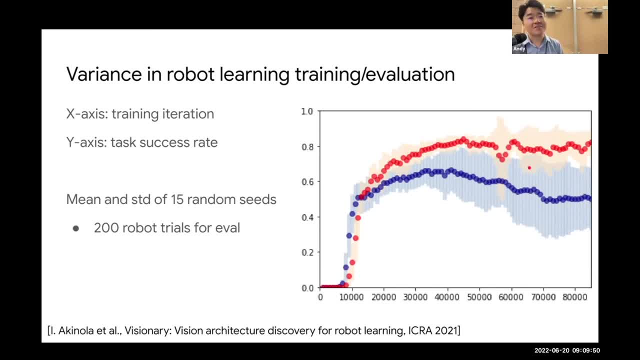 I want you to look at these transparent bars, These are the standard deviations, and particularly look at the standard deviation of these. you know the blue curve and I mean they kind of actually overlap. So the difference between these two models is very, you know, huge. 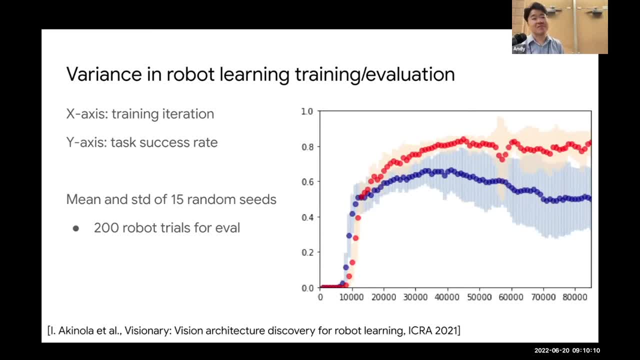 So maybe, based on this graph, we can conclude that this is better. However, when we talk about computer vision, we are usually competing in the in the random of like 1% accuracy difference, like 2% accuracy difference And if you stand the deviation. 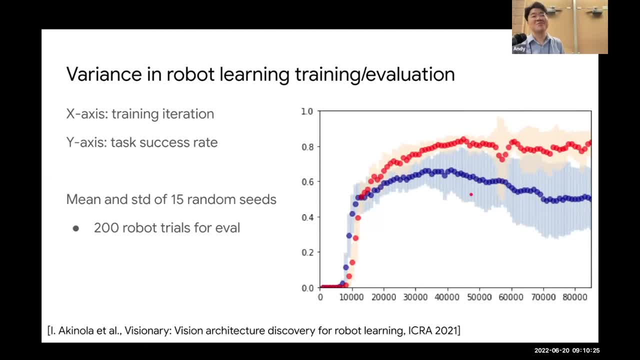 If you can see here is like 20% and if your model relative accuracy is like 2% better, can you really tell that it's a better model or is it just by your chance? And this is the difficulty you will be facing. 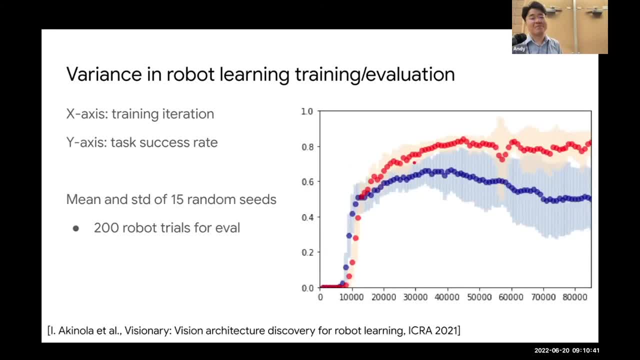 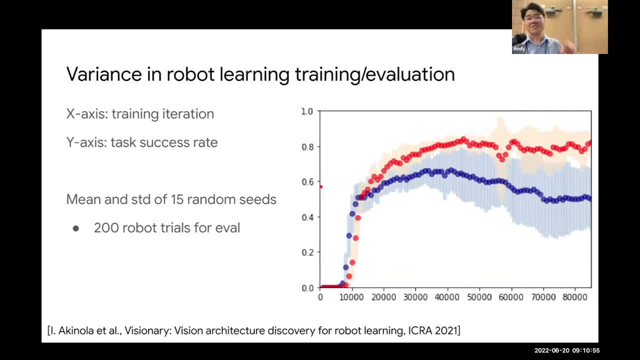 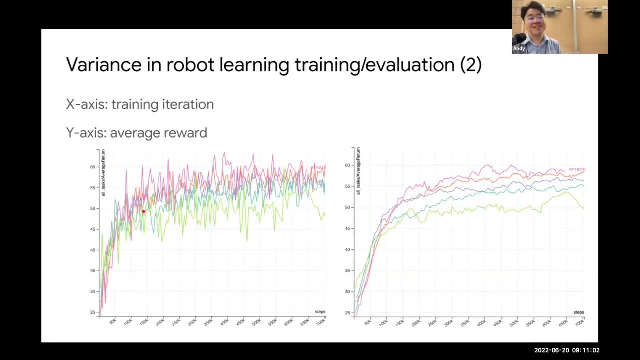 for like multiple random Zs. But if you just compare, like the same model over multiple single runs, this is how they look. So your evaluation changes almost at every like you know training, iteration And even if you smoothen it. so this is nothing but a smoother version of it. 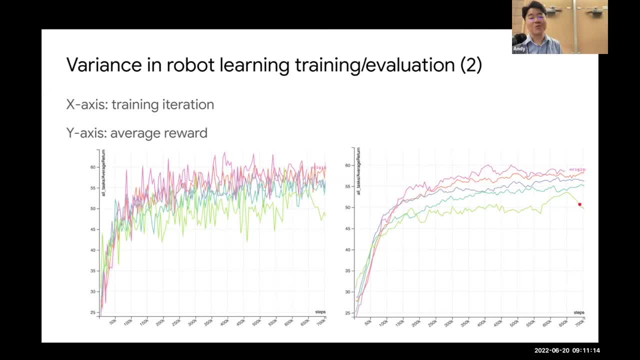 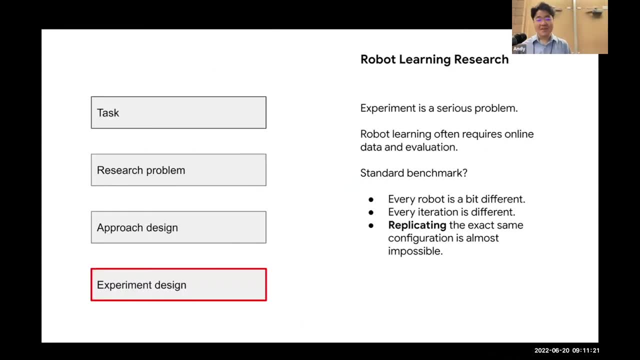 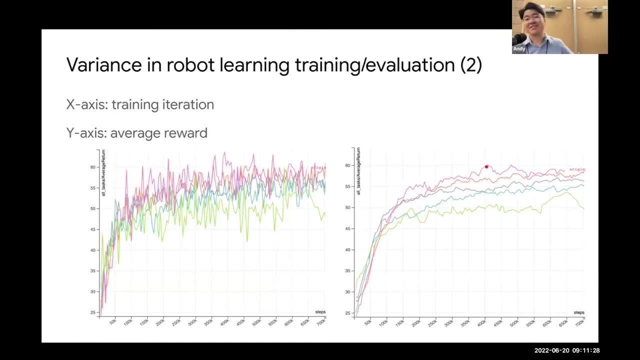 The same model actually ends up being somewhere totally difficult, And this is the situation you need to face. So, So another aspect in it, I mean. so, assume that you are somehow able to stabilize this, Assume that you are able to run this like 100 times, 200 times, thousands of times. 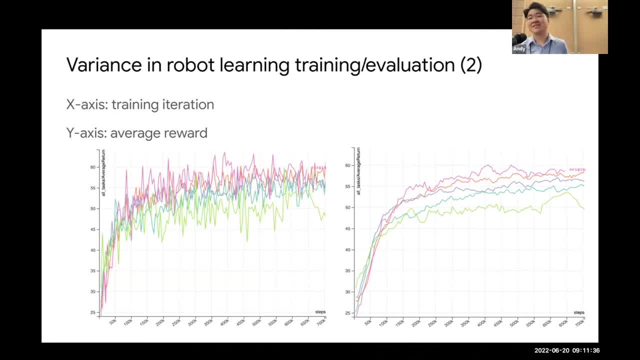 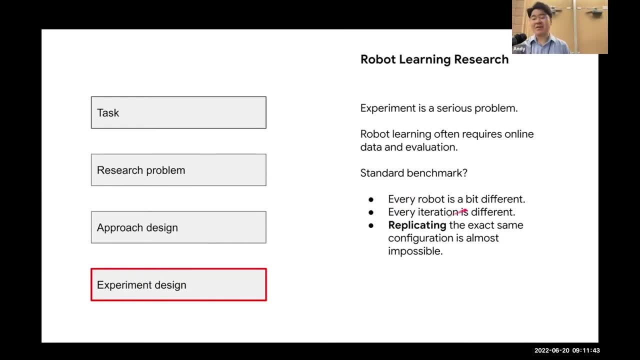 and were able to establish some reliable like evaluation metric. Even after that, there is an issue of standard benchmark, As Pete mentioned. every robot is physically slightly different And every iteration, as I mentioned, every training iteration, every training random seed. 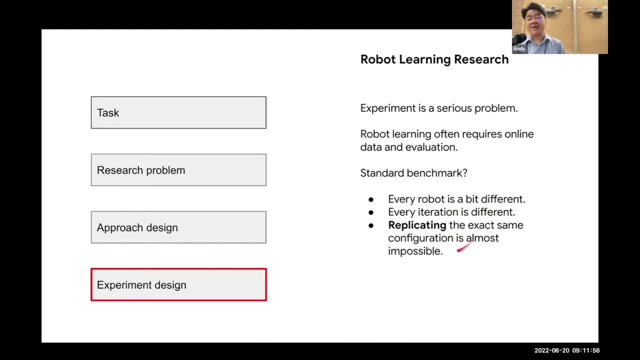 your data will be different and everything will be different, And also replicating the exact same configuration is almost impossible. What I mean by configuration is, if the robot is interacting with objects, you need to exactly place it at the same configuration in order for you to compare your approach. 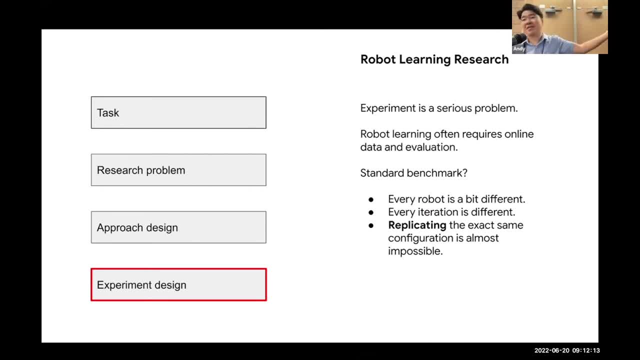 with someone else's approach on the other side of the planet. So coming up with the So standard benchmark is an open problem. It's extremely challenging, particularly for real robots, And obviously that leads us to, you know, take advantage of simulation. 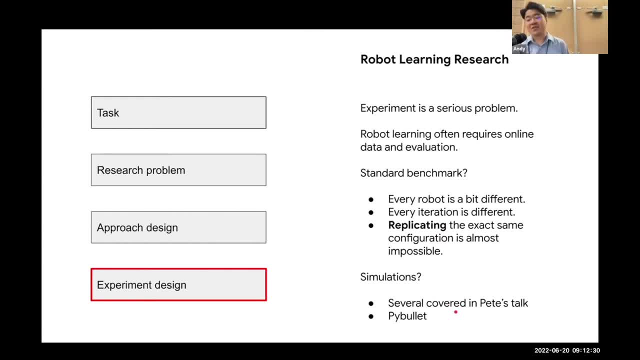 And there are multiple, several simulators covered in PSTO. There is also PyBlood environment and is using for the collab session today And these are some of the options. But the inherent problem of lacking standard benchmark in real robot tests is a problem. 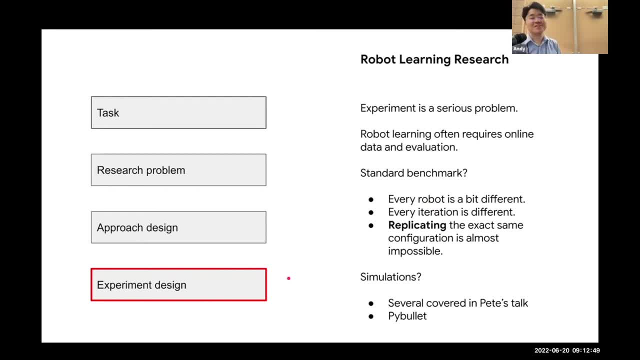 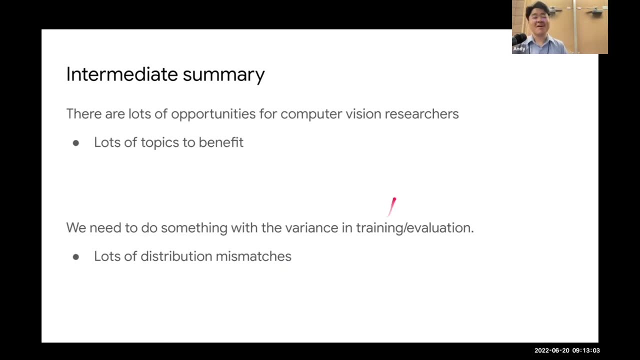 You will be facing. I mean, as computer vision researchers, we kind of take it granted that there is a standard benchmark. We can compare everything fairly. you know openly, publicly, That luxury will be gone. Okay, so the intermediate summary is that there are lots of opportunities for computer vision researchers. 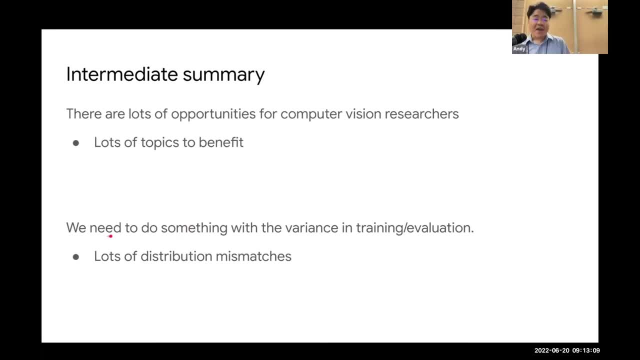 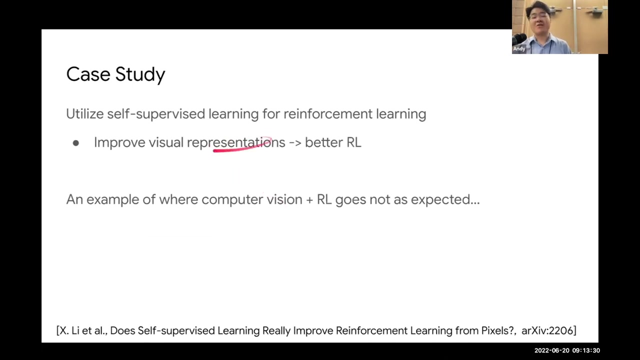 Lots of topics we can benefit And we also need to do something with the variance in training and evaluation. There are lots of distribution mismatch And some of them are far out of reach for the. So in terms of the results, There are lots of possibilities. So we may need to take advantage of some of the opportunities that are out there, But we need to take advantage of some of the opportunities that are out there And we need to take advantage of some of the possibilities that are out there, which causes such variance. 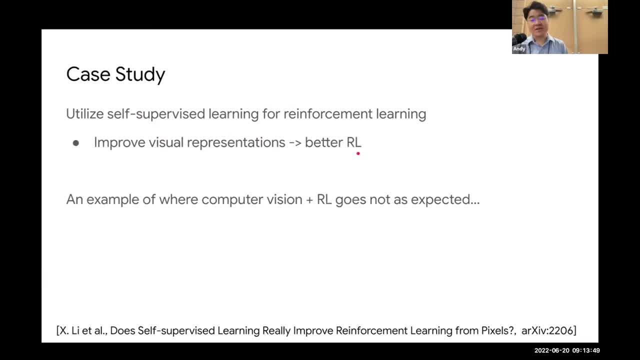 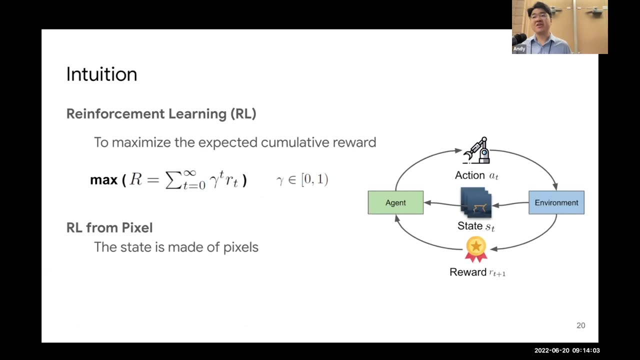 self-supervised learning so that we can do better robot learning and this, as i have been kind of forecasting, is an example of where computer vision plus rl goes not as expected. so let's, let's look at it. intuition is, as mentioned, there is reinforcement learning or robot learning, and 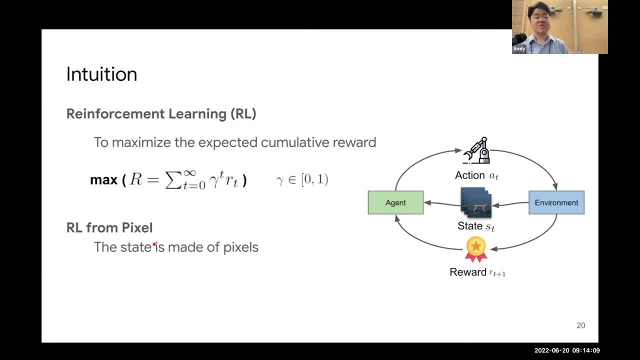 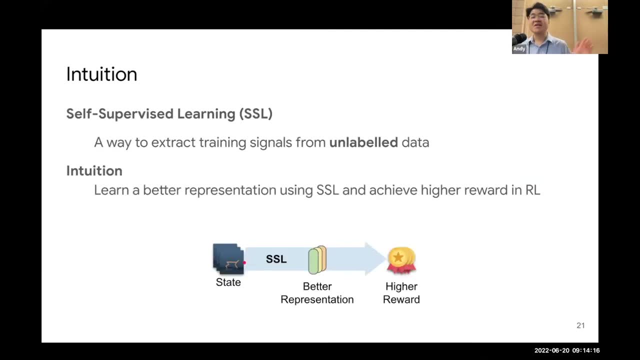 we are particularly interested in reinforcement learning from pixels, so that your state is made of pixels or representations learned out of pixels. and then there is the cell supervised learning, which you will be kind of more familiar with um. it's a way to extract training signals from unable data, and the intuition is to learn a better visual representation using cell supervised. 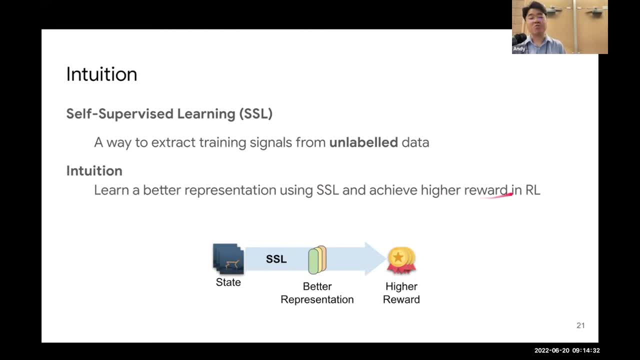 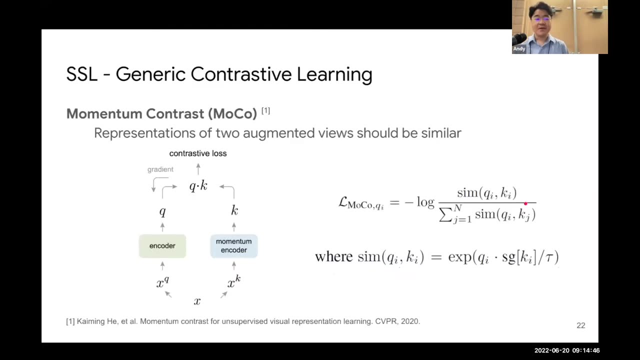 learning and achieve, ultimately achieve, higher reward in reinforcement learning. so yeah, the benefit from cell supervised learning losses. and then, um, try to learn the better representation which will eventually lead to the better reinforcement learning and better robot learning. and just to kind of give you what cell supervisor algorithms, self-supervised losses, we have been 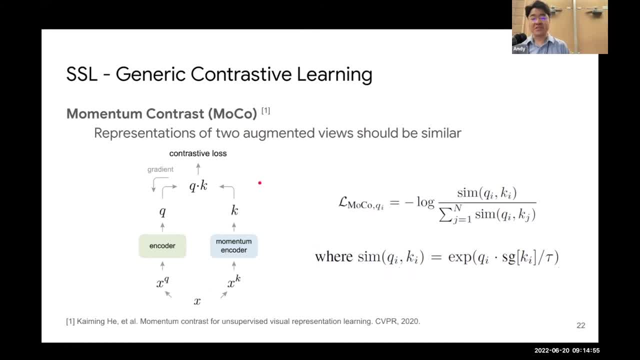 investigating. there is like moco, which is an example of like, pairwise or contrastive learning. we have the same data, we have two different augmentations of the same data- i mean same image, essentially- and we have two different types of encoder, which is the action, the regular encoder. 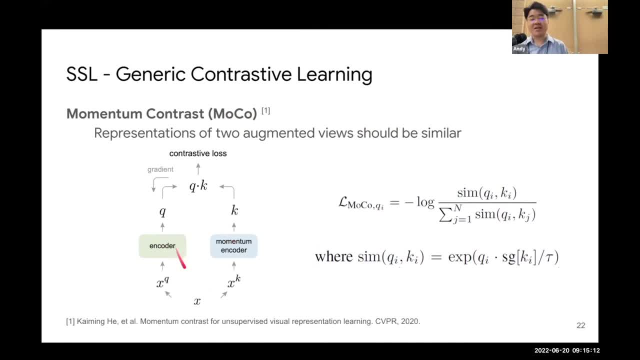 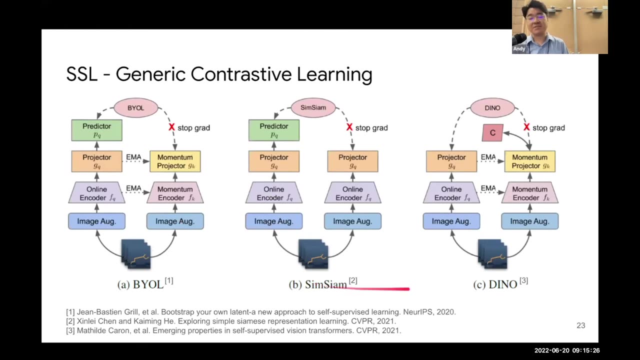 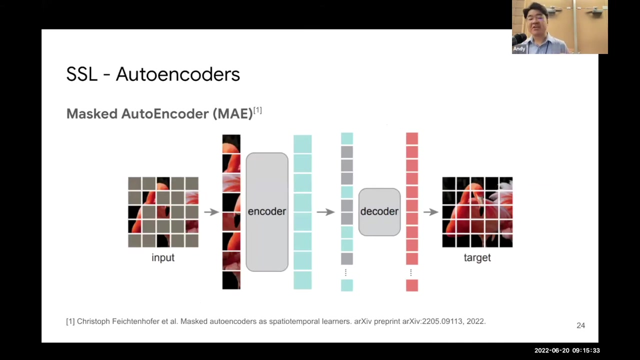 and momentum, encoder, encoder, and then we just say that well, this is on the same image, two different augmentations, so they should actually stay close within the representation space. and there are lots of billions um doing something similar, like byol, sims, iam and dino. there are other types of cell supervision, such as, like reconstruction, based on autoencoders. 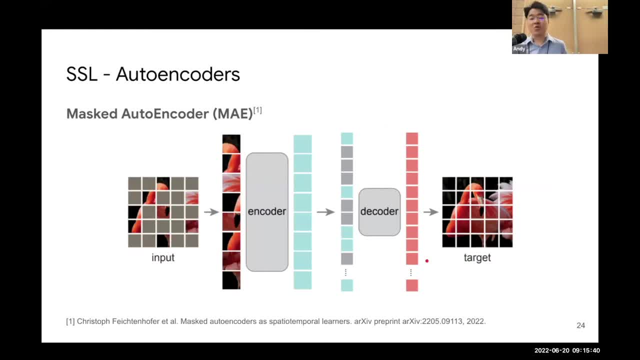 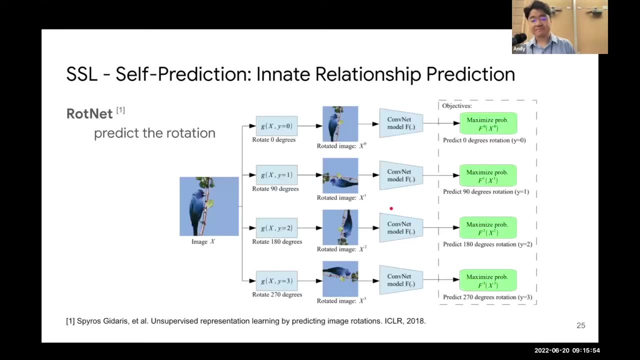 there are. there has been traditional autoencoders, there has been mass autoencoders. there are also training models for this and it's very interesting because, with the using the kind of modeling i just showed you, um, here i am just showing that training your network, training your model, together with a loss like this will ultimately allow the representation to be more generic. so, yeah, there are lots of studies and there are other types of cell supervised losses, like predicting certain things, like if you rotate objects, you can actually set up your representation so that you will be able to predict how much it rotated. 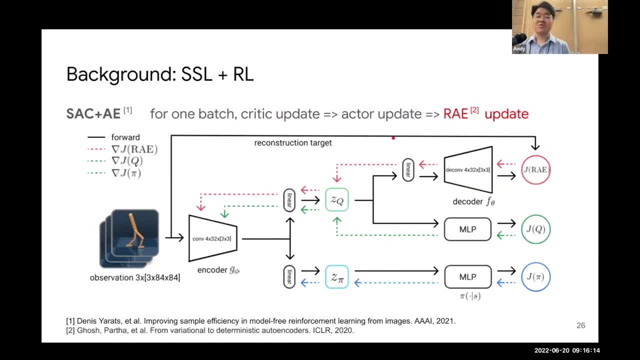 So there are things like that. And then there were previous work trying to compare or trying to combine self-supervised learning plus reinforcement learning, And this was a simple combination of soft actor critic plus autoencoder And although it looks complicated, part of it is just soft actor critic training, like this part. 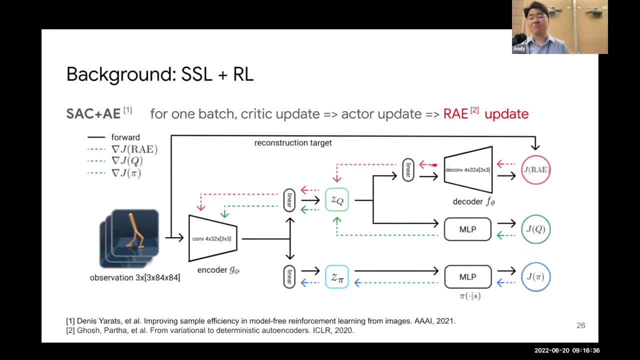 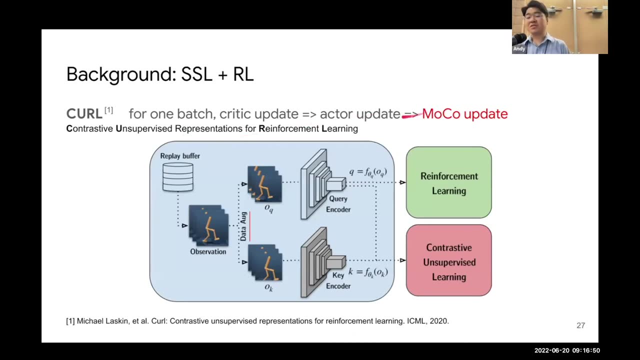 And part of it, if you just look at the red arrow, is just the autoencoder training. So they were actually trying to put everything together and trying to jointly optimize different types of losses And they showed that it benefits. There was another thing which is more based on the contrastive loss, essentially very similar to MoCo. 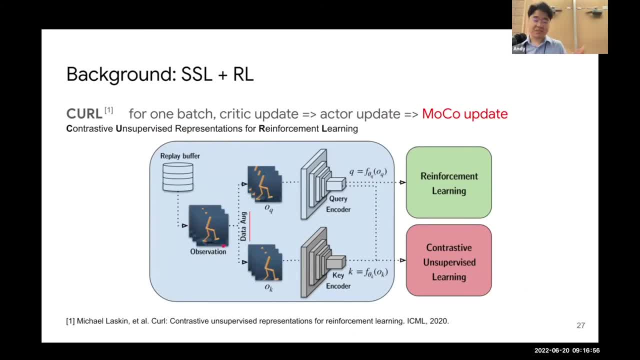 As mentioned here, we have a robot image in Sim And we tried to get two different augmentations, which are essentially different croppings, give it to the encoder and then try to minimize their distance by having this contrast And then we tried to minimize the contrastive loss in addition to having the action policy, learning reinforcement, learning loss. 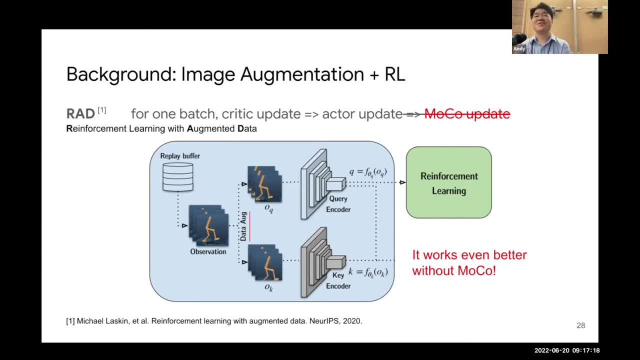 And then there is another kind of story going on- Sorry for confusing you. Saying that, I mean this was kind of interesting because it was the same architecture- and people suddenly claim that well, if we keep the architecture, the actual architecture, and then if we just get rid of the self-supervised loss part over here, it actually performs better. 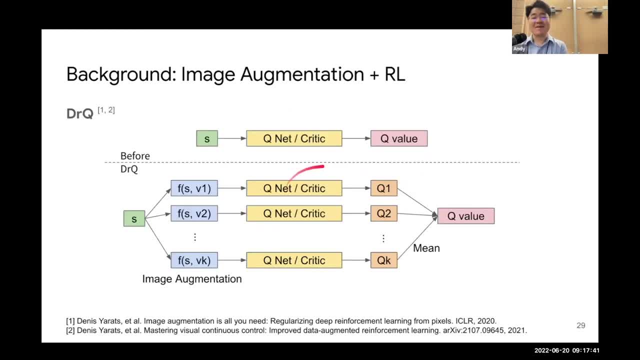 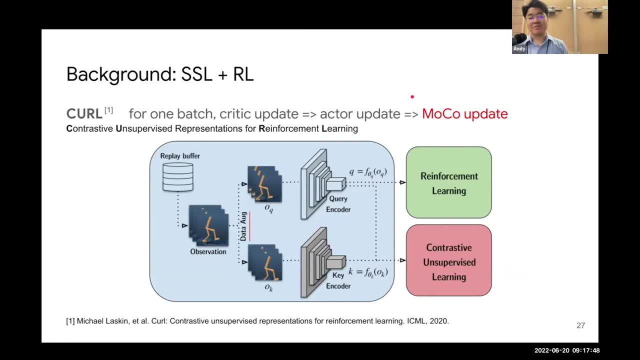 And there were other papers also saying that yeah, maybe image augmentation might be sufficient for reinforcement learning, which were kind of contradicting what was claimed in this reinforcement learning plus self-supervised learning. So we wanted to kind of investigate what self-supervised learning losses will truly benefit reinforcement learning. 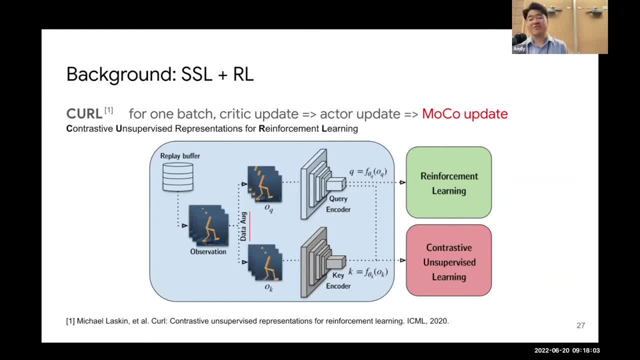 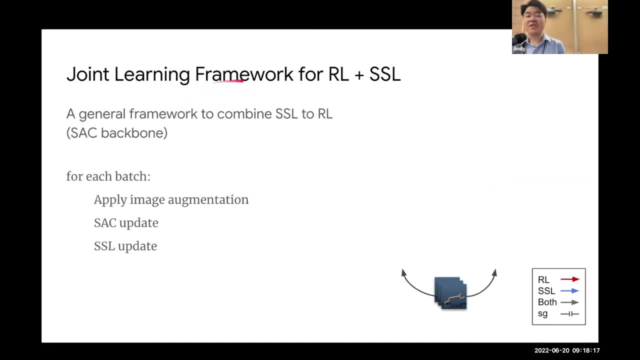 And, essentially, what would be the recipe or what would be the framework to combine these things, How to make the self-supervised learning from reinforcement learning to self-supervised learning, computer vision, literature, best benefit reinforcement learning for robot learning. so, uh, we formulated a joint learning framework, what we call uh, extending the previous um curl. 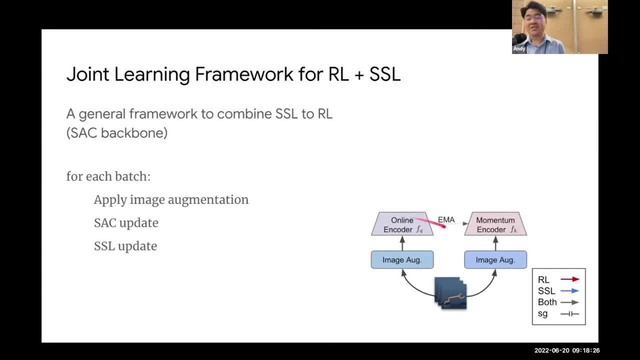 or software critic plus autoencoder. so, as mentioned, yeah, this is very similar to curl, but in addition to the reinforcement learning part, uh, we attached many self-supervised learning heads. if we just have this one, this becomes very similar to curl. if we add this one, there could be more self-supervised courses, and we try to optimize. 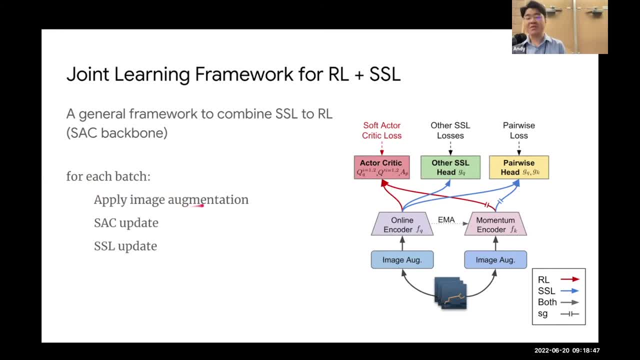 all these jointly within the same batch. we apply image augmentation, we apply reinforcement learning update and we apply self-supervised learning update and, yeah, we replace this one with many different losses and we try to compare them. how much time do i have? i mean, well, um, everything got shifted, but yeah, all right. all right, i'll continue. 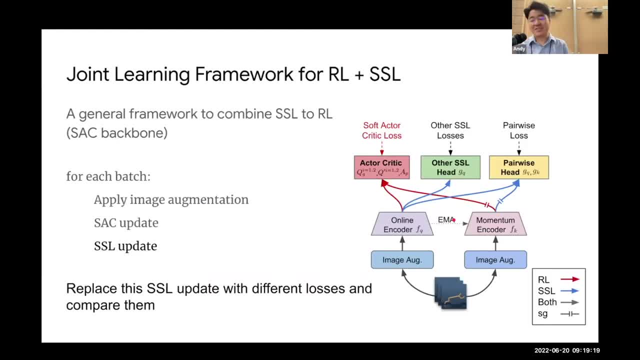 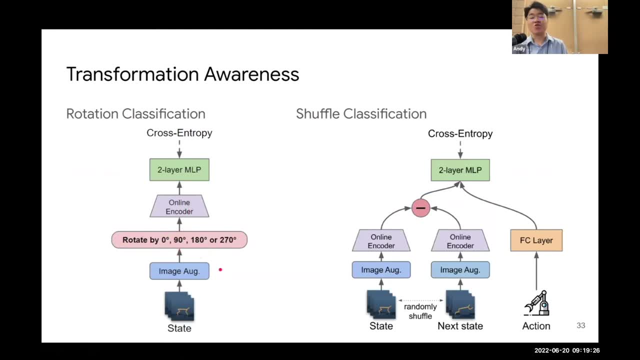 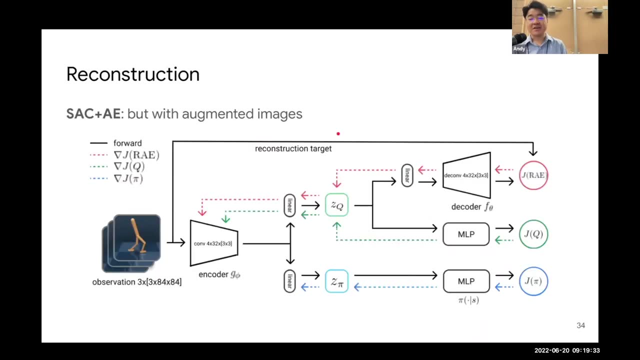 so, uh, this was the general framework and, as you see you, this can easily be converted into one of these. you know, contrastive losses, or can be take, i mean or can incorporate computer vision, cell supervised losses like rotation classification, shuffle classification and even the reconstruction which was actually used in software critic plus autoencoder. 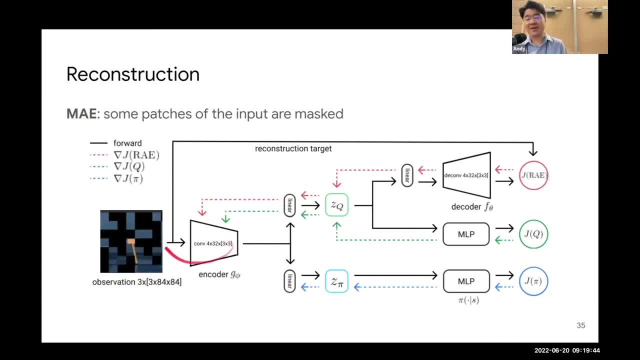 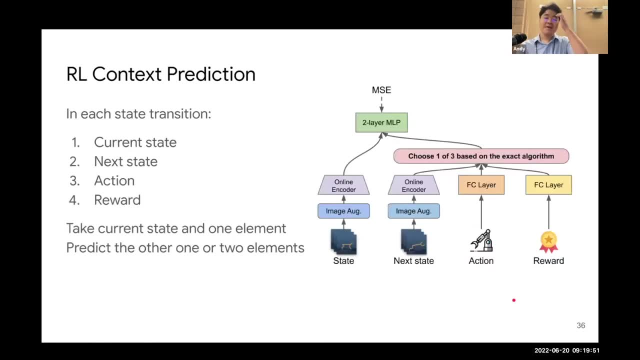 yeah, and we can also take advantage of mask autoencoder instead, by masking the input and then trying to reconstruct, together with running the reinforcement learning objectives. and there are other types of reinforcement learning- specific cell supervised losses, which are like reinforcement learning- context prediction- so we can take advantage of the. 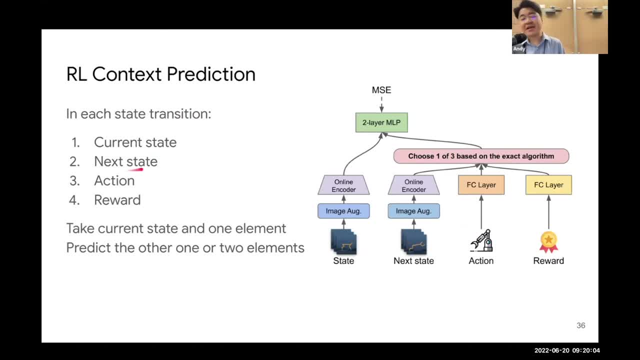 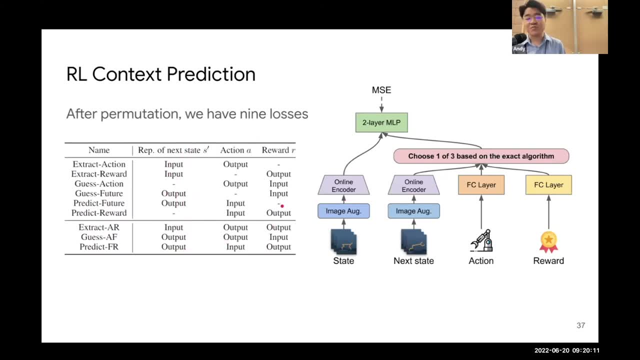 formulation to predict the current state, next state, action and reward. and yeah, we can give some of these as an input, some of these as an output, and then trying to formulate the loss out of it without any annotation. so, skipping the details, i'll just say that there are also, like cell supervised losses. 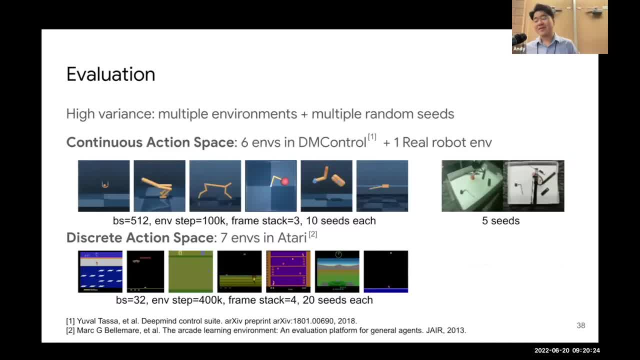 specific to reinforcement learning context. okay, that's enough for the setting. now we want you to evaluate which cell supervised laws is a good, which are bad, by evaluating them in different environments. one is in sim, the mind control suit. another is more like a computer game: atari. 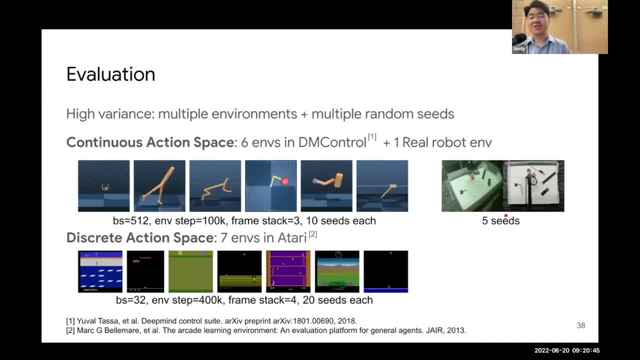 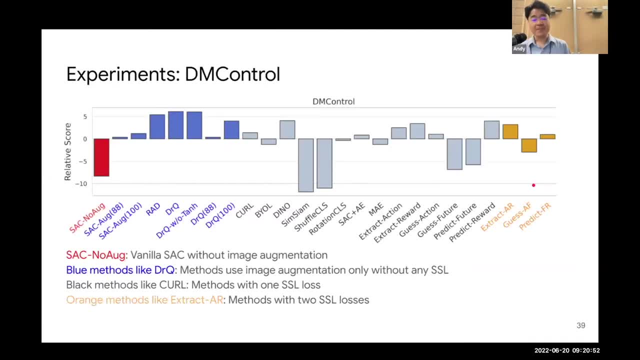 and finally some easy real world environment where the task is just just simply to reach and stay close to the target object as much as possible. and here's the result. on the mind control suit, red one is the base: vanilla by baseline, without any augmentations. all the other methods, whether they are using cell supervised loss or not, uses image augmentation. 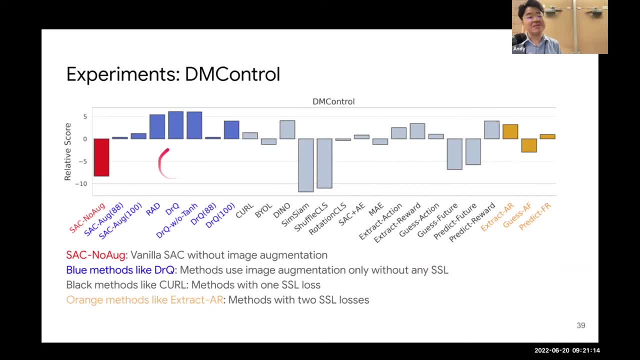 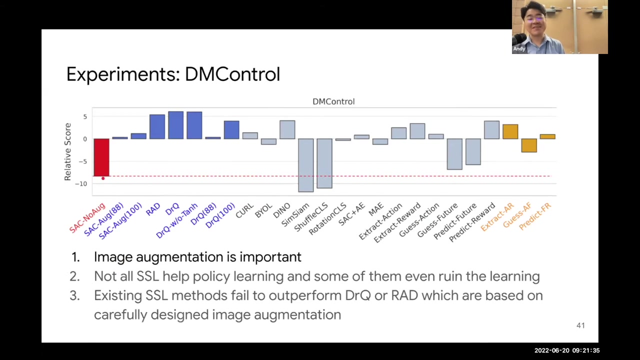 so blue are without any cell supervision, they are just image augmentation. only these, you know, are black methods, they are with cell supervised loss and orange is with multiple cell supervised losses. actually just two, and we find some interesting observations. um one, yeah, here's the basic baseline, and baseline was pretty bad, but some cell supervised losses were. 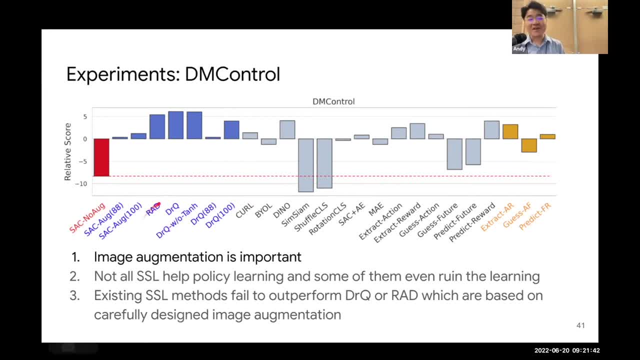 actually even worse than that. on the other hand, image augmentation they were performing pretty well. i mean, compared to all these methods, um image, even the worst kind of image augmentation- was actually reasonably better than any of the cell supervision. so not all cell supervised loss is actually very good, but it means that some of the learning was not sketchy and is not good. 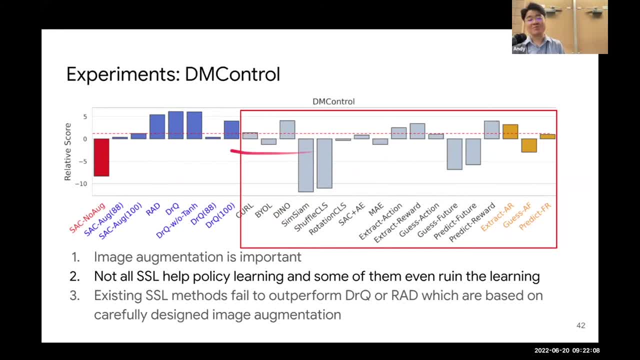 and there was some critical errors, or some of them actually got very bad, but i think that the type of learning that actually got the best result for us was actually really good. but i think that this is another path that we can actually use um everyriot in the field. 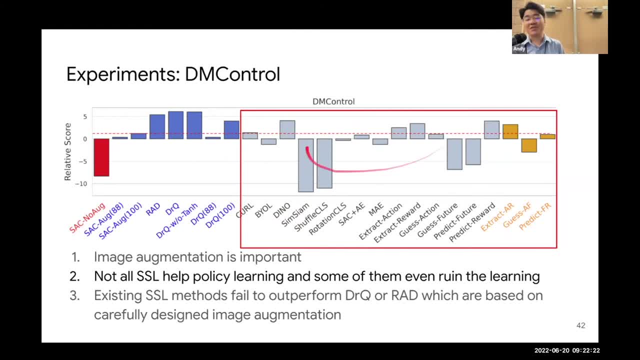 so, in terms of the self-supervised learning- this one i were talking about with the conflicts with the self-supervised learning- but i think the performance of the search in this case, this one was really, really good, which was by far one hundred percent better than the self-supervised learning. 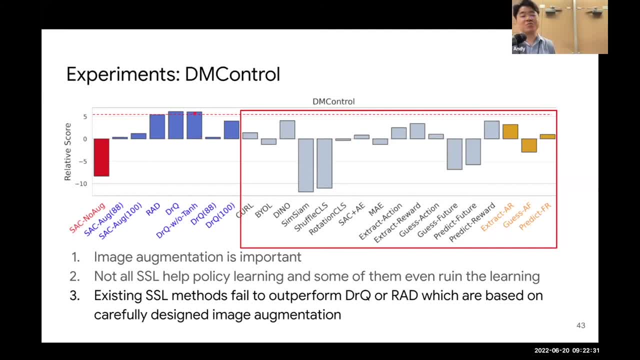 there were some really very good results that were shown, but this pair of these issues were not good. If we carefully hand-tune image augmentation parameters, we find that they actually perform better than any of single cell supervised losses. They actually perform better than combination of multiple cell supervised losses. 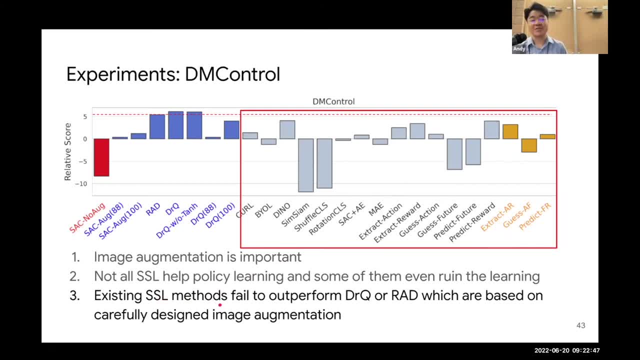 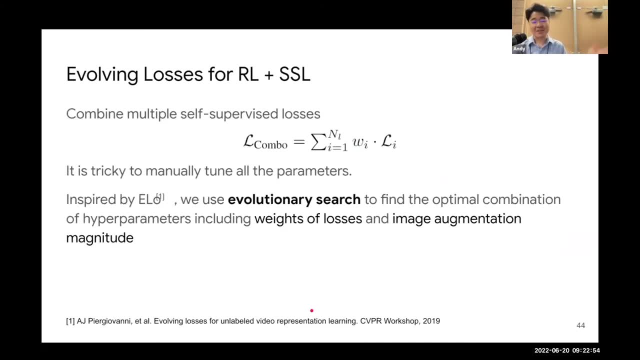 So this is actually showing that existing computer vision based cell supervised losses actually fail to outperform carefully designed image augmentation, meaning that they are not really compatible. So we also try to investigate how much- I mean how- we can actually combine multiple different types of cell supervised losses by doing evolutionary research. 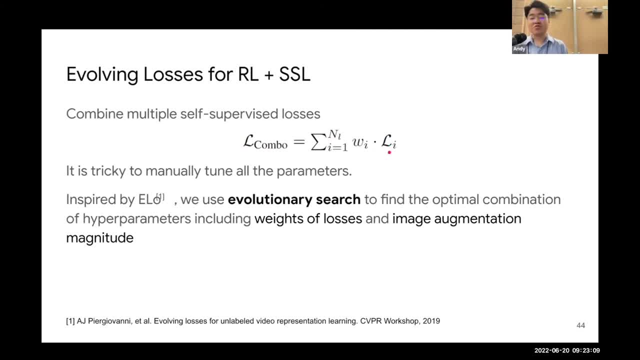 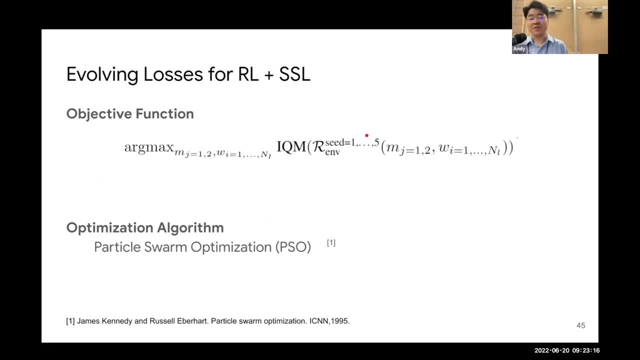 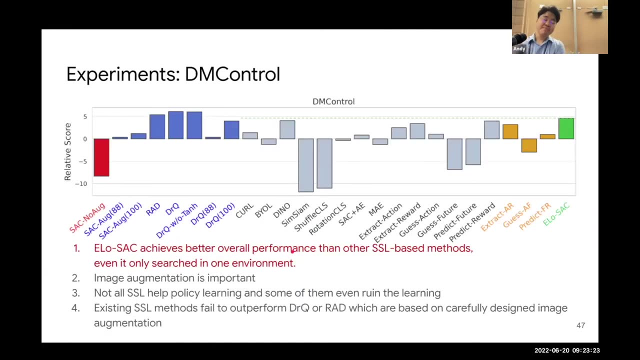 We try to combine multiple different types of losses using an evolutionary algorithm And based on that, we were able to find some optimal amount of like parameters combining these different types of losses and come up with something like this And the observation here: Okay, 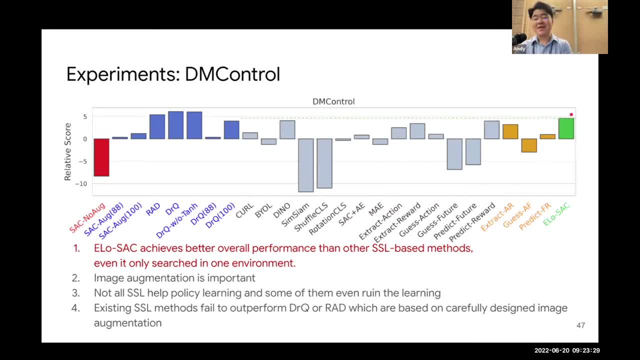 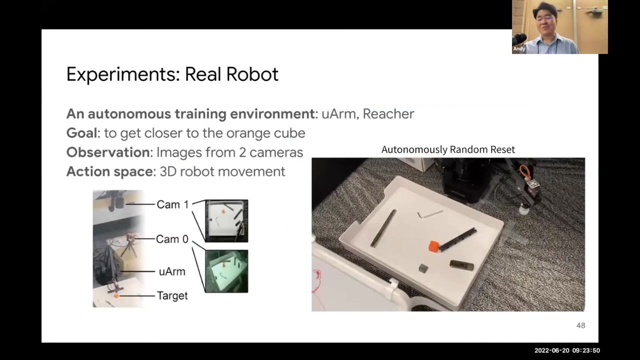 So what we see here is that this combination of everything actually is better than everything, which is good, And it's still worse than image augmentation only. So use of cell supervision, regardless how many losses we used, was still inferior to carefully design image augmentation, meaning that, okay, what's the point in doing this? 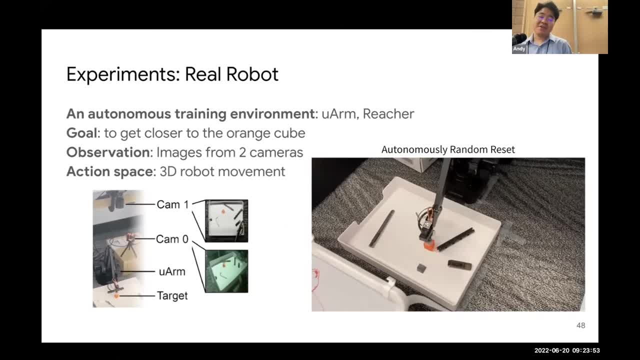 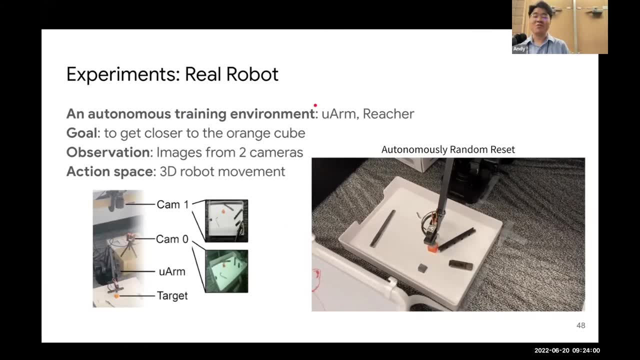 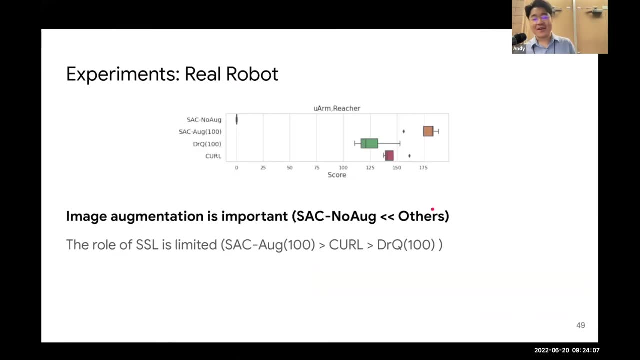 So we also try to confirm whether these holes are in real robot environment by running a very simple, you know, robot test. It's a richer version- I mean real world version- of the richer in simulation And the goal is to just, you know, get closer to the orange cube as possible. 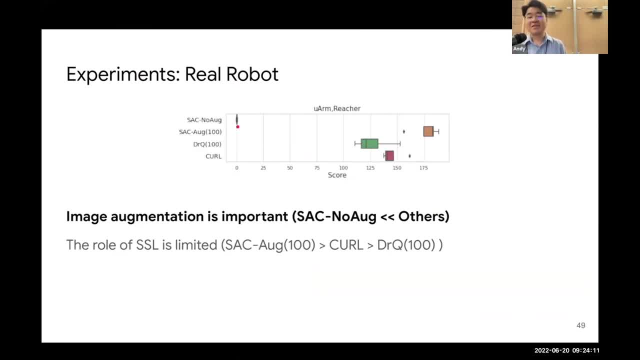 And here is some interesting results. Without augmentation, given a limited amount of data, we were not able to learn anything. As soon as we give augmentation, it learned actually well and it actually learned better than use of the cell supervised learning method. 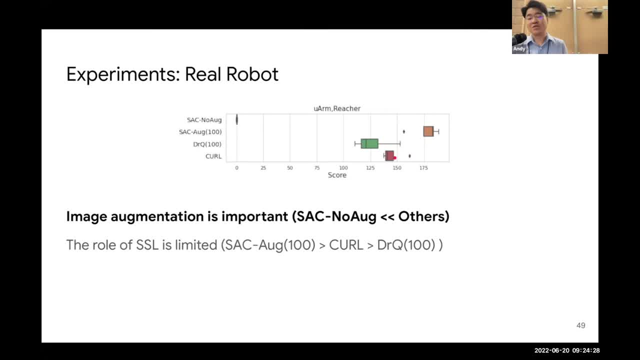 Okay, So this is the result of the augmentation loss And CURL is one of the kind of most typical cell supervision plus reinforcement learning, And we were able to see that the image augmentation itself, the basic vanilla image augmentation, was sufficient to outperform CURL. 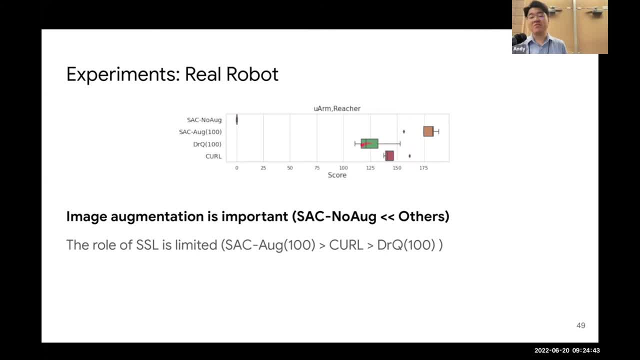 The DRQ, which was really good in DMC, didn't really work very well here, meaning that they were kind of overly optimized, like you know, to dim my controls to parameters. Maybe the hyper parameters were off. I mean, this is image augmentation only, and this is image augmentation only relying on 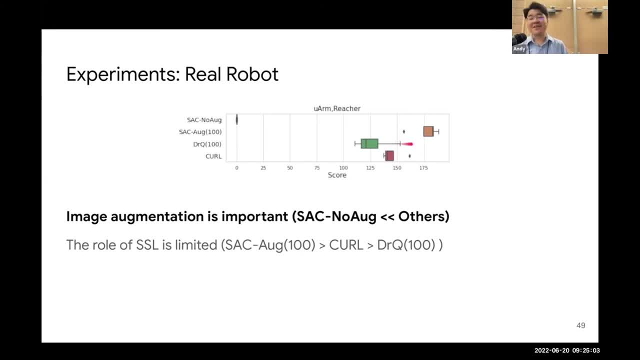 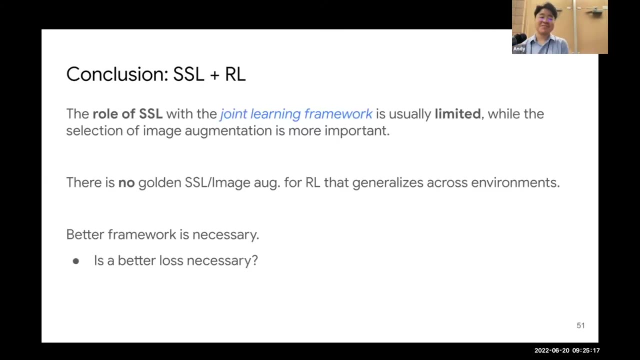 different. you know augmentations, But in the end we see that the augmentation identical to CURL. what was being used in CURL is actually better without cell supervised loss in CURL. So that's pretty much it. The conclusion we were able to observe was that the role of cell supervised learning 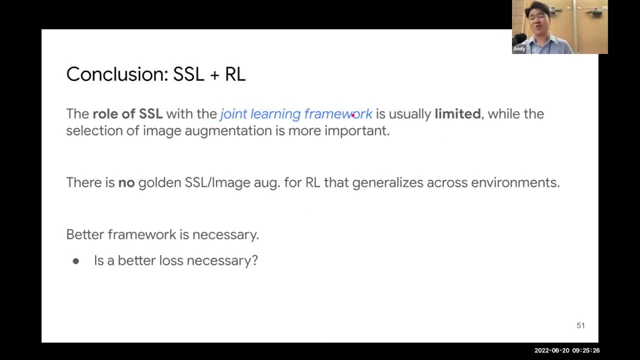 and this, within this joint learning model, is very important. Okay, So what we found is that the role of cell supervised learning in the reinforcement learning framework, trying to jointly optimize everything, is usually very limited, while the selection of image augmentation is sometimes much more important. 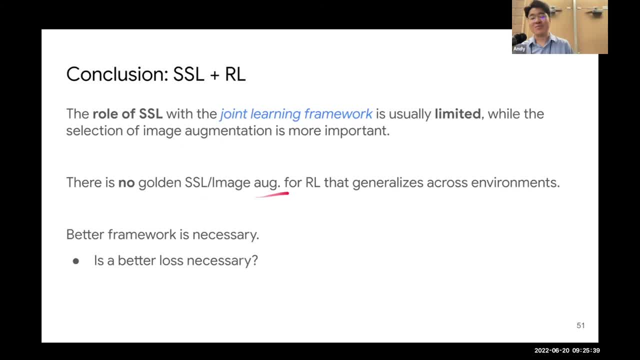 We were able to kind of find that there is no golden cell supervised learning or image augmentation for reinforcement learning that's generalized across environments, which is a bit disappointing, because we kind of tried to combine cell supervised learning from computer vision, reinforcement learning for robot learning and yeah, it didn't work. 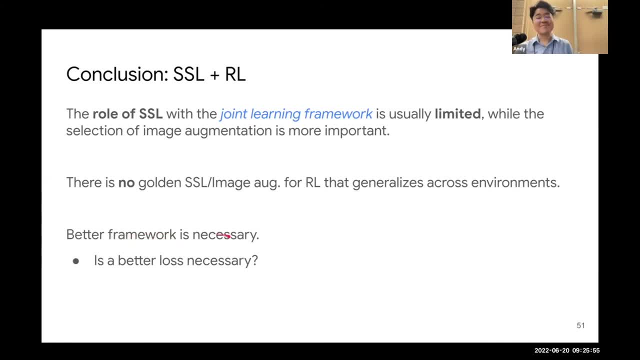 Okay, Thank you, That's a very good point. Better framework probably is necessary in combining them, not just this joint optimization framework, And whether we need a better loss function or not, that's an open question, I think, from here. 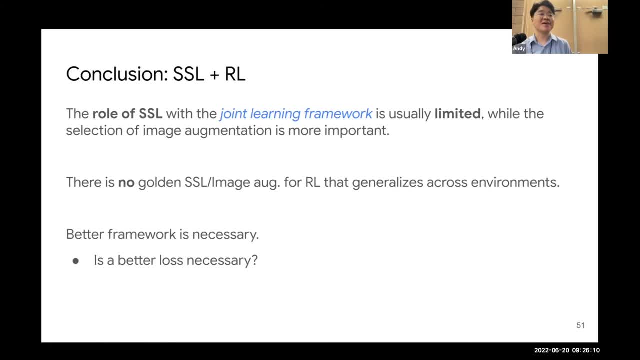 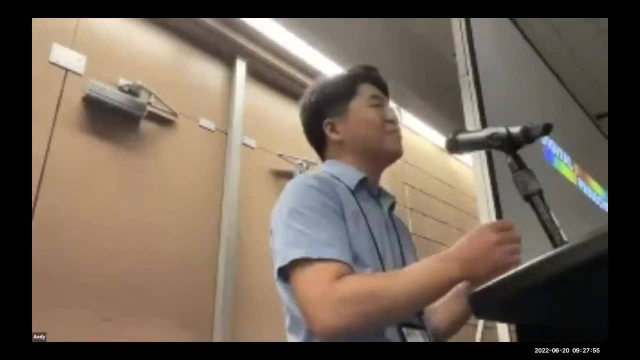 So that pretty much kind of concludes what I want to say today, and just let me know if you have any questions. Yeah, yeah, yeah, If you can use a microphone, that would be better. and then we try to, you know, extend whatever has been the mainstream in robot learning. 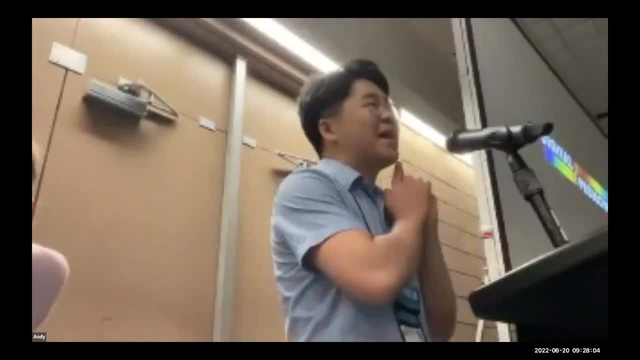 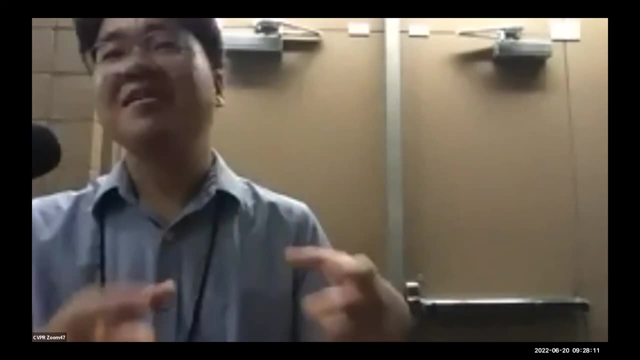 in terms of cell supervision plus reinforcement learning. so that's the reason why we used- and i think the reason why they used, they initiated, formulated this framework is because, as mentioned, the training data is kind of changing during the online like interaction with the environment. so it was, i mean, it was pretty natural that the batch is updated at every training. 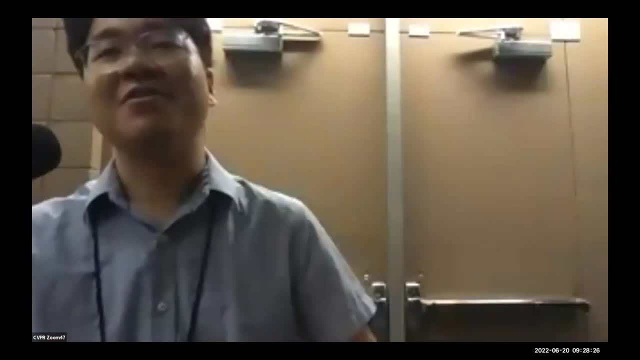 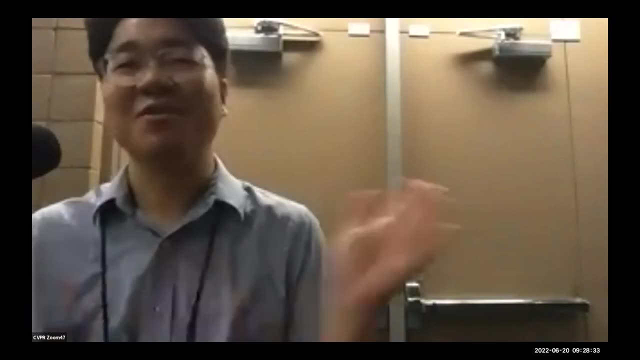 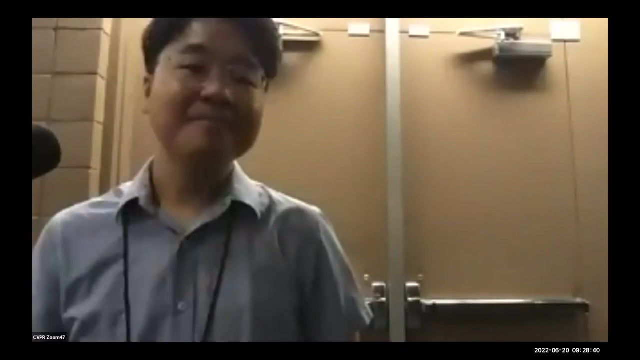 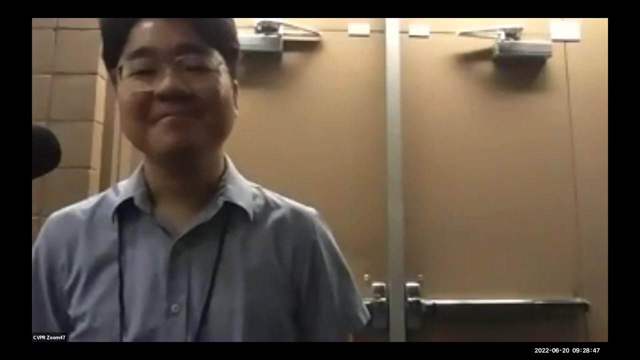 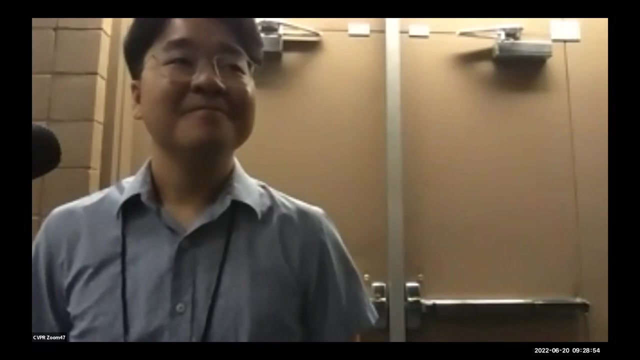 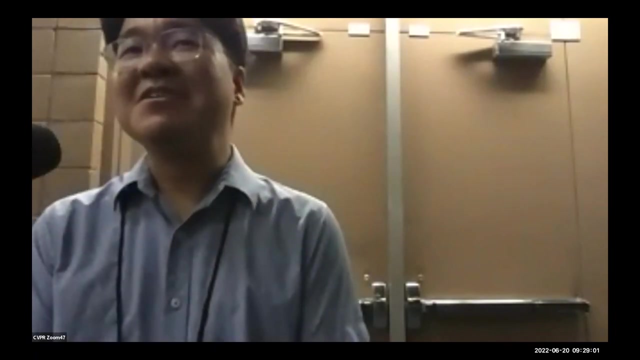 iteration, and they want you to apply the cell supervised learning laws and the reinforcement learning laws for every batch they are taking. so i think that's how they came up with it and we just try to follow it. so the question is whether cell supervised learning is really useless for robot learning. 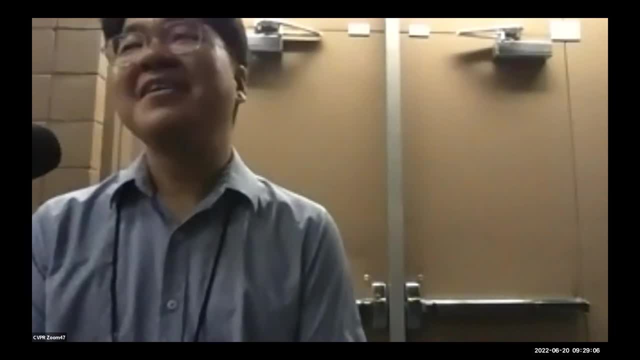 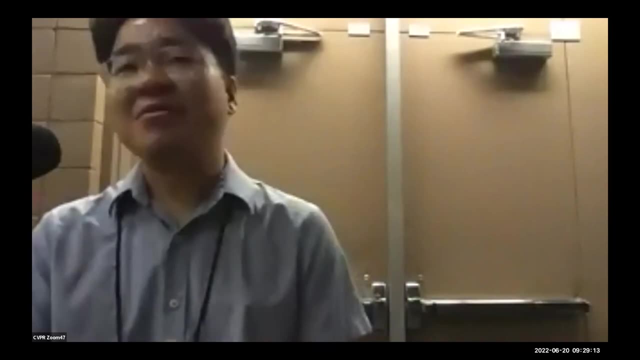 my answer is no, um, i think there is a hope. so, if we are only taking advantage of online data and if we are using the current um, this joint learning framework, the answer is yeah, this is not doing anything. however, when we switch to pre-training framework, there is a lot of. 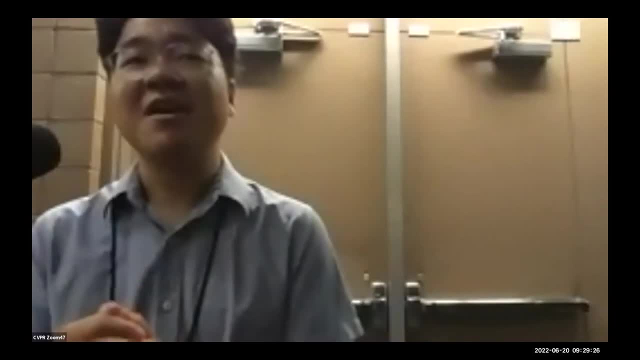 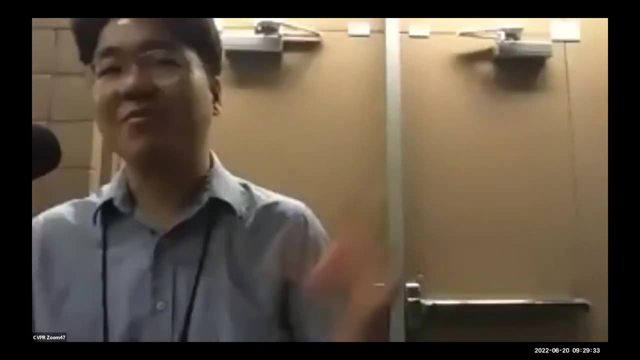 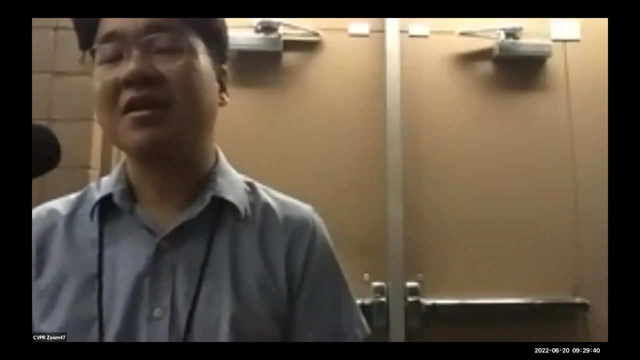 potential that we can minimize the environment interaction by taking advantage of already collected data. i mean we can even take advantage of the data on youtube or whatever data that's out there and in that aspect, pre-training framework has more potential in taking utilizing such data with self-supervised losses. so there is more potential in that direction, definitely, and i 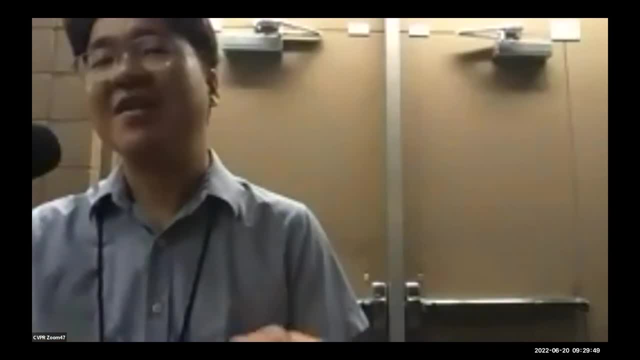 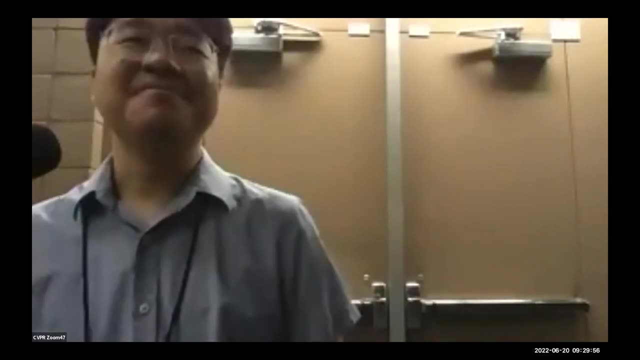 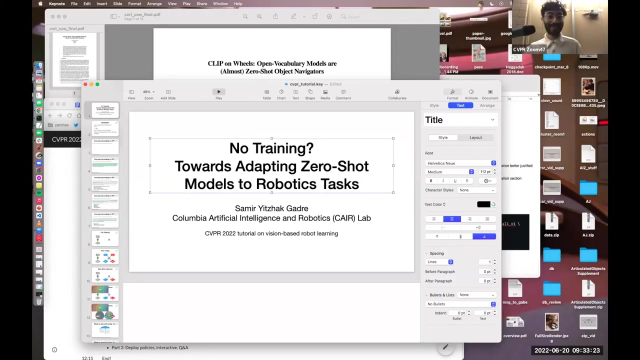 think we are simply lacking. we have not yet found the good framework to combine self-supervision and smart learning, which is up to our all of us, all of our future study. all right, thank you, okay, so, uh, my name is samir um. i'm here as part of the 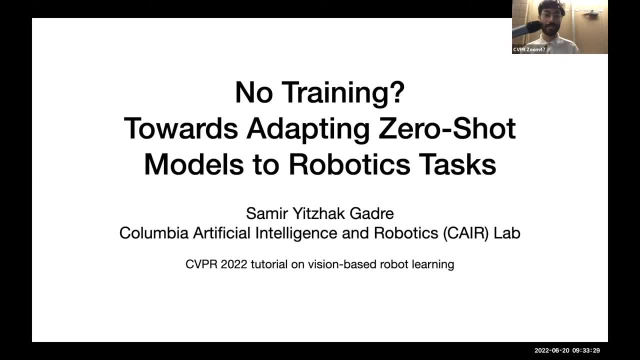 artificial intelligence and robotics lab, and today i'm going to be talking um, about using existing zero shot models to do zero, to do robotics tasks, and i have this kind of provocative question here, which is no training- and i specifically mean no training for for robots and um, this seems kind of like a ridiculous question. um, in light of all of the 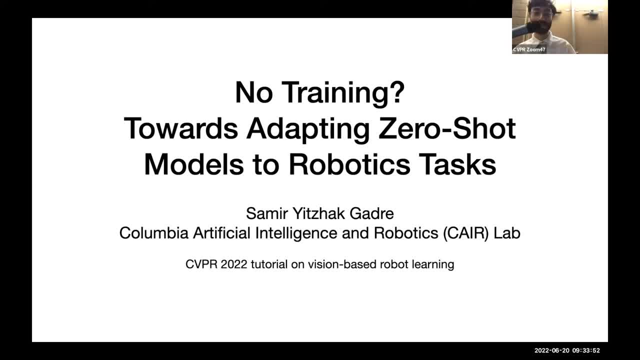 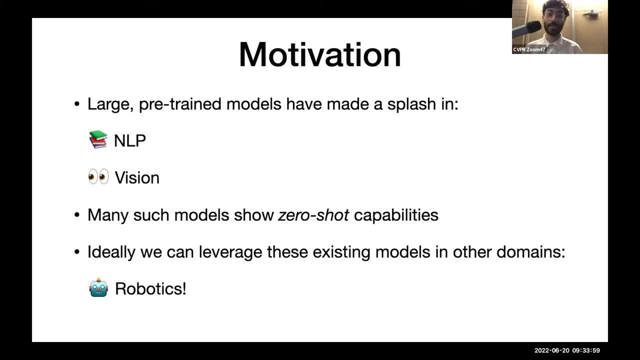 talks and wonderful um like tutorial that's happened so far, um. so let's start with a bit of motivation. so if we look at the backdrop of what's kind of happening in nlp and in vision, um, there are these large pre-trained models that are are really sort of making a splash and 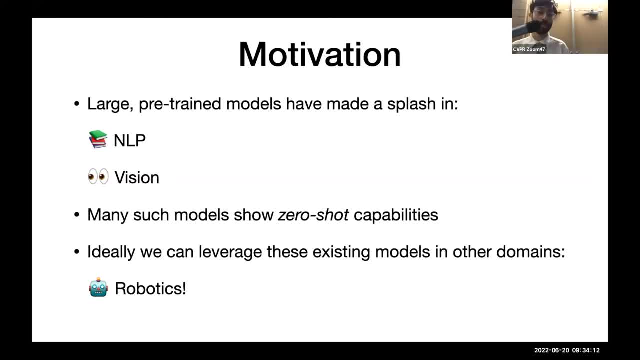 they're doing all sorts of cool things and, most notably, they're doing them zero shot in a lot of cases, or at least this is a very new kind of line of study. so here what happens is we're going to train on a specific pre-training task, but at test time we're going to task test on unseen tasks, but something about the structure of 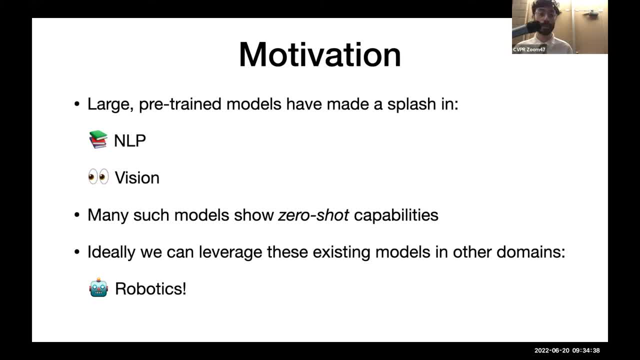 our pre-training actually allows us to do these tasks downstream, so this is incredibly exciting, and it then allows us to pose this question of: can we actually use these models more or less out of the box- um, maybe with algorithms around these models, in order to start to do some robotics tasks? 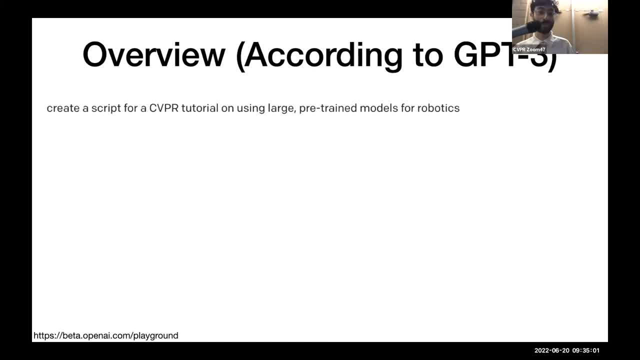 okay. so to start, just as an overview of this talk, i decided to ask gpt what this talk would be about, so i prompted it with the cvpr tutorial on using large pre-trained models for robotics, and this is what it gives me. i'm not going to read through the slide, but i'm going to give you a little bit of a. 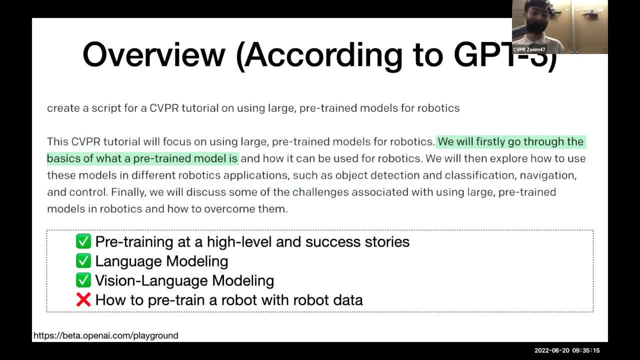 read it, but it does roughly outline the talk, which is interesting. so first i'm going to talk a little bit about pre-training at a very high level and sharing some success stories from both nlp and vision. what i'm not going to talk about is how to use sort of robotics data in order to pre-train. 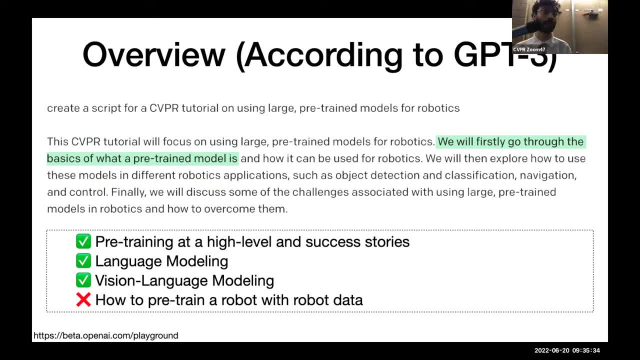 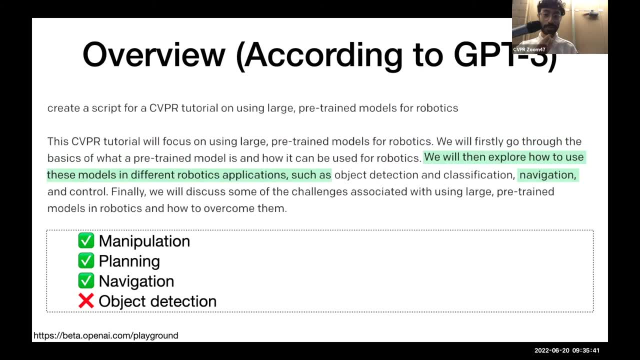 this is a super exciting direction and something that i do think that we should all be thinking about, but it's sort of not within scope for this talk, so next i'm going to talk about a few applications of these sort of existing large, pre-trained models, specifically for manipulation, planning and navigation tasks. and then gpt also wants me. 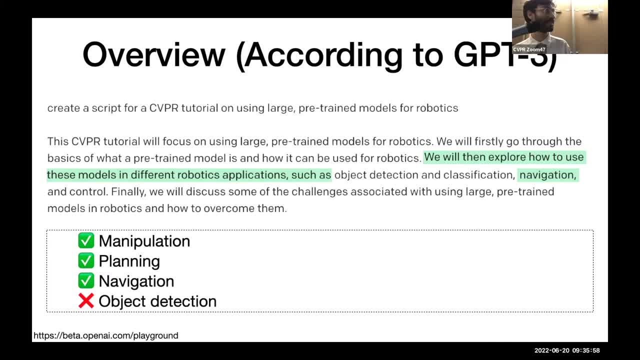 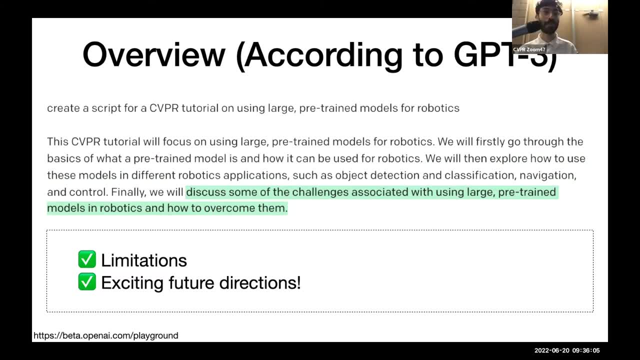 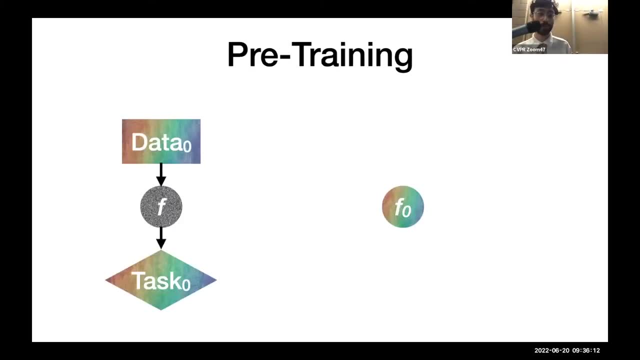 to talk about object detection, but i'm not going to do that. and then, finally, i'll talk about, like, a few limitations and some exciting future directions, hopefully inspiring many of you to start working along this direction. so so okay, so just a brief review of pre-training. we have this function f, which is randomly initialized. 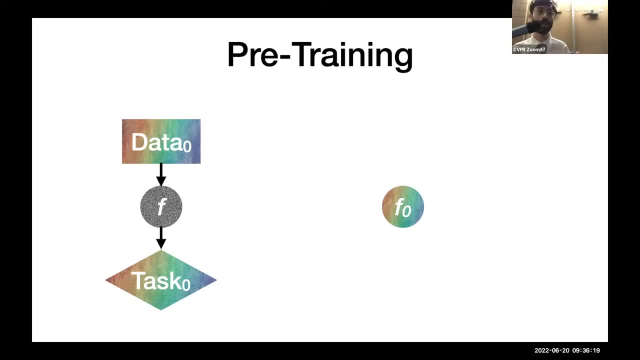 we choose some tasks and we want this task to be sort of general but also pretty diverse. so the rainbow here highlights the diversity. and then we get this checkpoint, which is f0, which is our pre-trained model. so now what we can do is this is sort of the standard fine tuning setup is given. 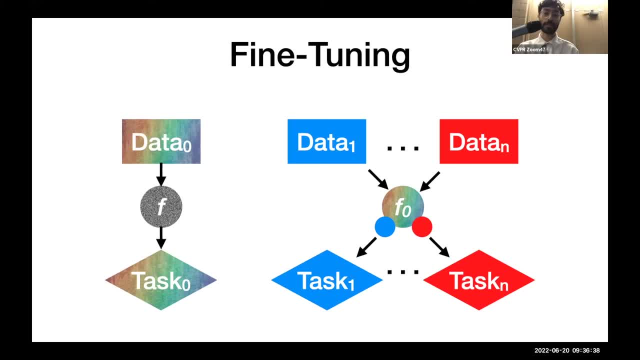 data for our downstream tasks, say d1 through dn, we can fit a small number of parameters, either like a linear layer of some sort on top of this representation, or we can do end-to-end time tuning. so the most the thing that i think is really interesting is now, with these large models, you can start to not necessarily see data for these. 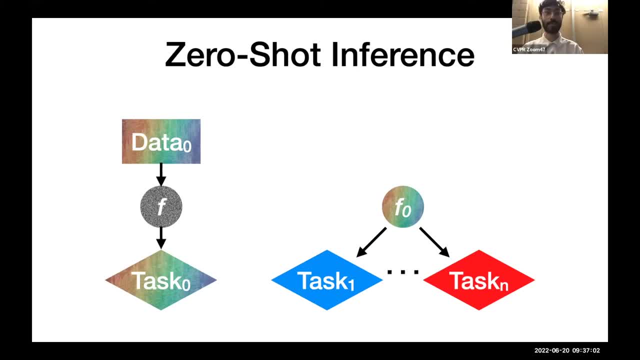 downstream tasks and still get sort of respectable performance. it's important to note that the gap for some tasks in nlp and vision is is considerably high compared to the fine-tuning solutions. but in a lot of cases this works surprisingly well, and we'll talk a little bit about how this is working in a second. but one thing to note is that it's not 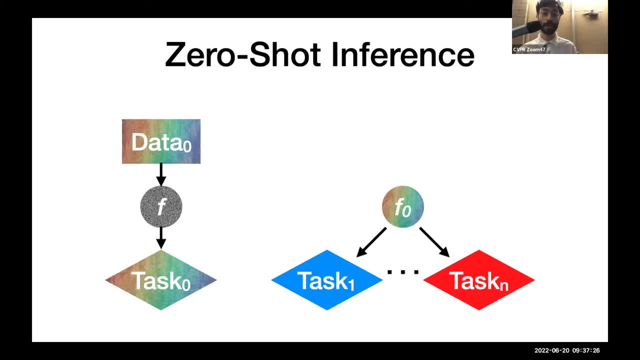 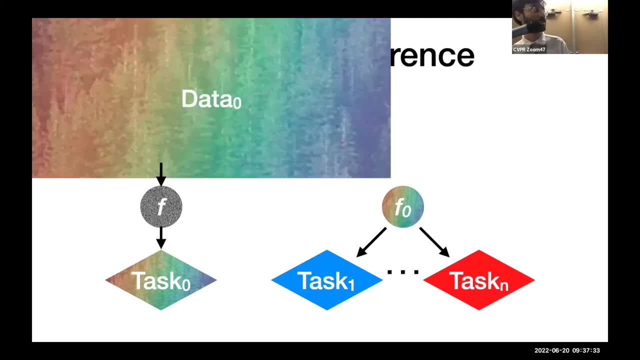 just about the objective that you choose at pre-training that allows this to happen. there a few other magical opponents. the first is data, so your data probably should look more like this, and then you all probably see where i'm going, but should also probably look more like this, so they don't really fit on the slides anymore. 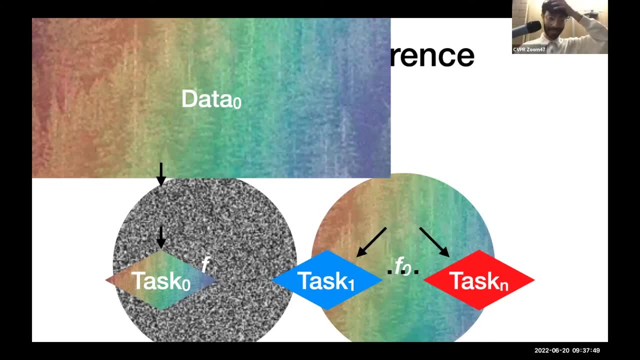 so this is something that i want everyone to kind of keep in mind, just because i'm going to be talking about the objectives and the algorithms and this is kind of the the intellectually interesting part to talk about. but a lot of the success is really being driven by this kind of 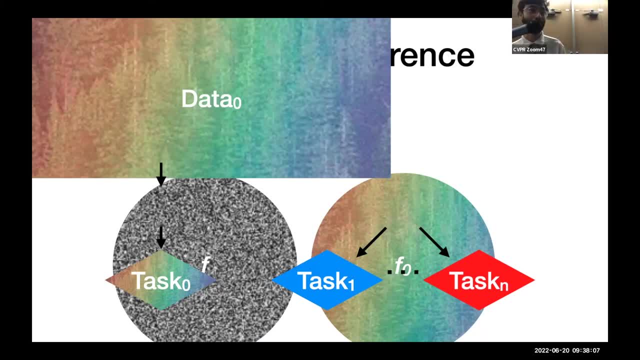 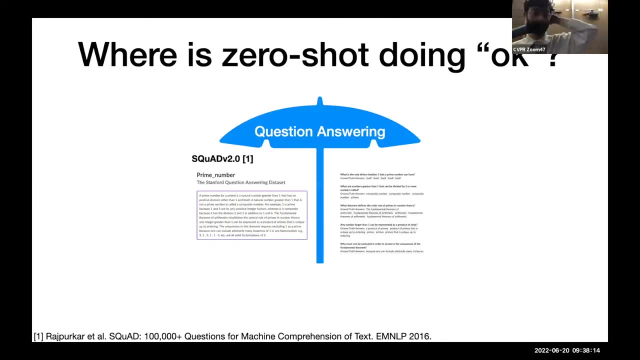 story and it it seems to be working so well that we we really can't ignore it, in my opinion. okay, so i'm going to breeze over this, but here, like a few success stories and zero shot doing. okay, so question answering in nlp seems to be we seem to be on the right track there. 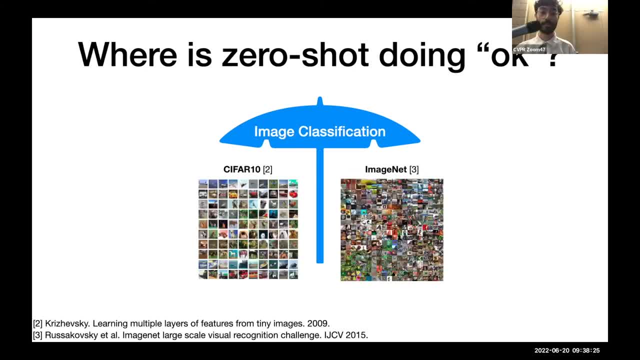 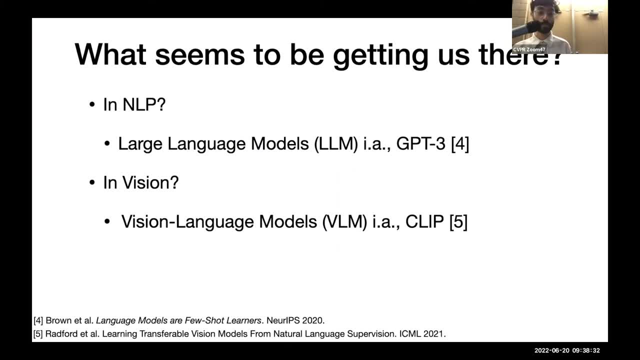 and then image classification in the vision world. so what seems to be getting us here, at least on the objective side? um, so i'm going to talk about two, two kind of high level objectives. the first is language modeling and the second is the language modeling and the second is the language modeling and the second is the language modeling. 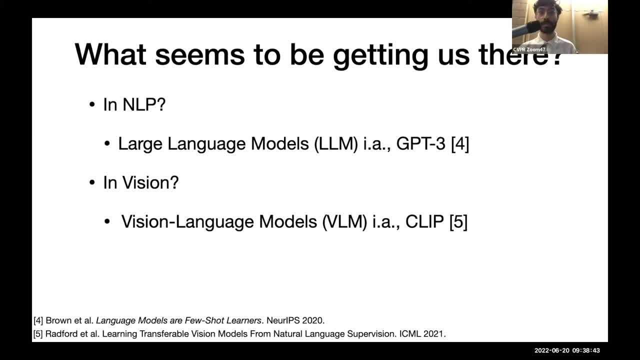 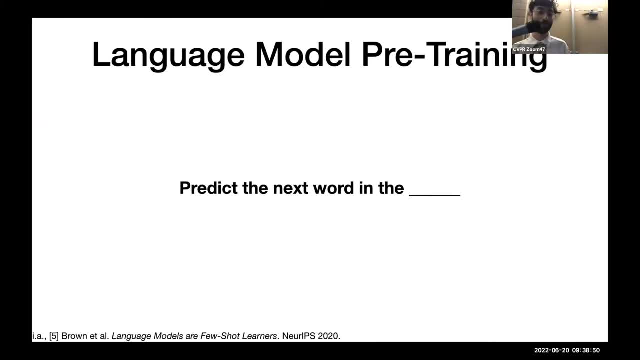 this vision language contrastive objective used in CLIP. So with language modeling the task is gonna be pretty straightforward. It's just kind of predict the next word in the sentence. So by training a model to do this on sort of very large purposes of data, 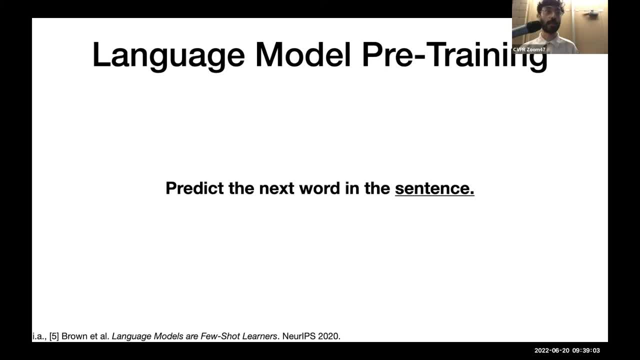 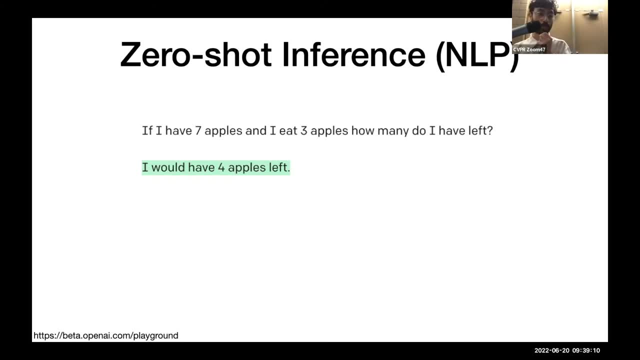 it starts to like learn some interesting things about language and the way that humans might pose questions and do other things. So the cool thing here is that we can now do things zero shot at inference time. So here I've posed a subtraction problem to GPT. 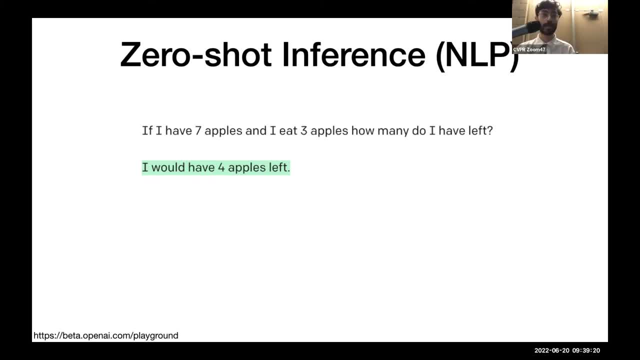 where I tell it I have seven apples and I eat three of them and I ask how many I have left and it tells me that I have four apples. You can also imagine doing kind of a sentiment analysis type tasks. So here I have the phrase: I love computer vision. 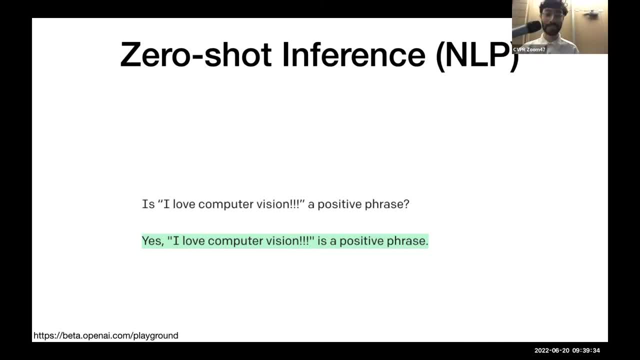 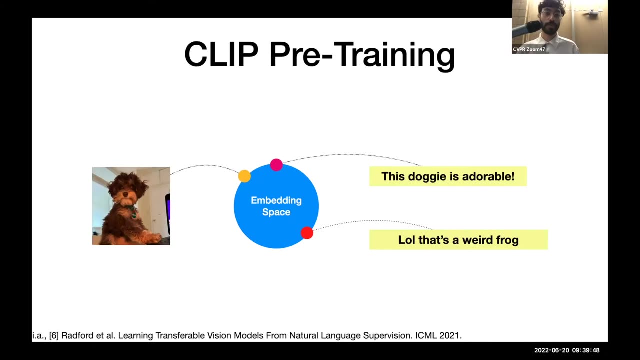 which we all do and GPT agrees it's a positive phrase. So the point here is that we haven't explicitly trained this model to do sentiment analysis, but it kind of comes out of the wash in this kind of language modeling objective. So similarly we have some kind of fun objectives in vision. 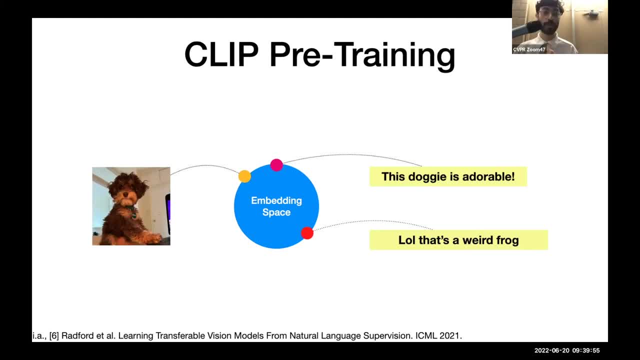 So there's this CLIP objective, wherein we're going to try to align representations of images and corresponding captions in a feature space. So here we have this dog and then the caption: this doggy is adorable, And we want the features for these things to be very close in some embedding space. 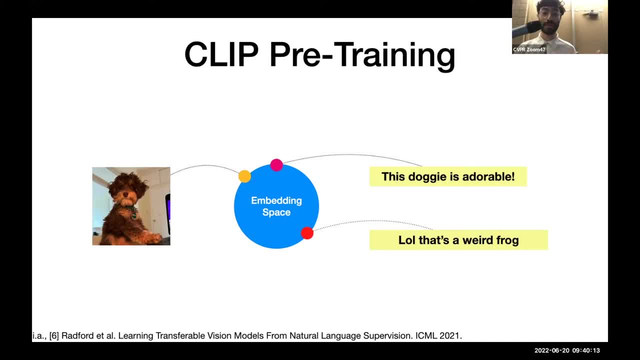 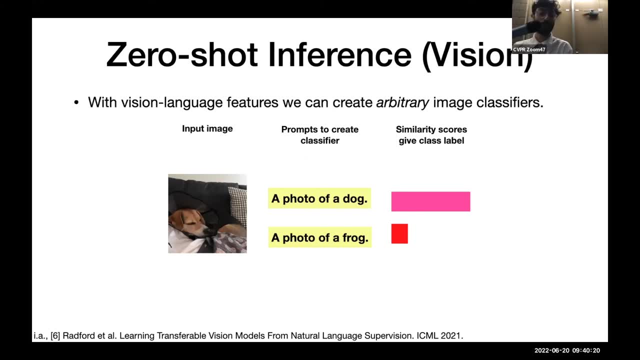 and far away from sort of this dissimilar concept of: LOL, that's a weird frog And the cool thing here is now we can define arbitrary classifiers at test time. So, given a caption, a photo of a dog and a photo of a frog. 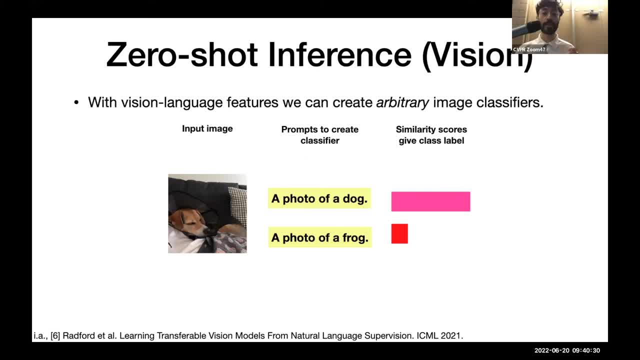 I now have and the corresponding text features for these. I can now ask the question: is the dog feature close to the image dog feature? And if that is the case, then I'll classify this image as a dog. So this is kind of how zero-shot emerges in this case. 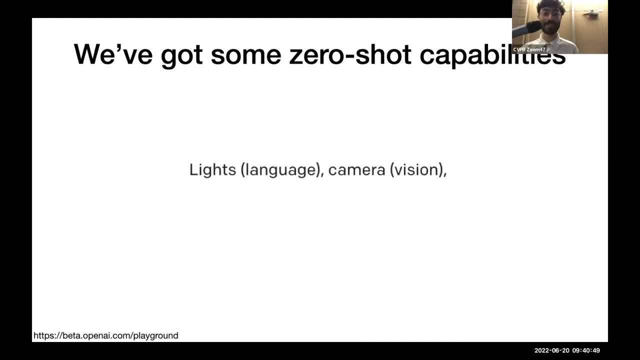 Okay, so we have some zero-shot capabilities, So we have lights in parentheses, language camera, which is the vision. What are we missing for robotics? And GBD tells us action and, more specifically, motor control, which I think is probably not too far off. 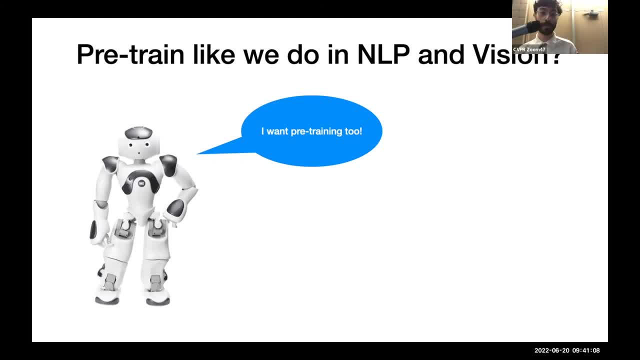 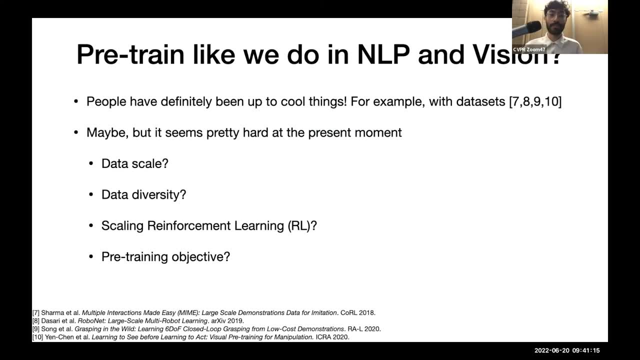 Okay. so the first thing that we might think to do is we might want to pre-train the robot, like we did in NLP and vision. So the robot wants pre-training too, And this is maybe possible, but I think it's probably hard for a lot of the reasons. 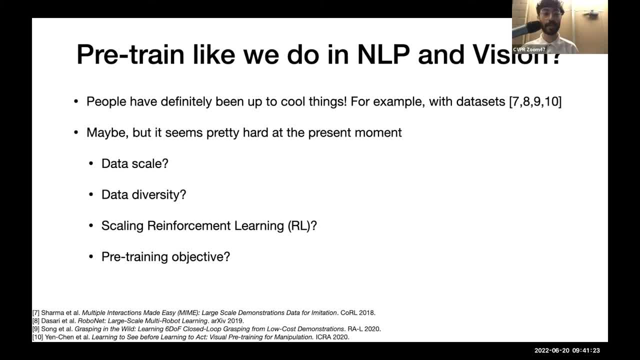 that sort of the earlier presenters mentioned, And I think one major thing is data here, but people have definitely been up to very cool things on the data space and also the algorithm space. So that's sort of the answer is maybe, but maybe we're just not there yet. 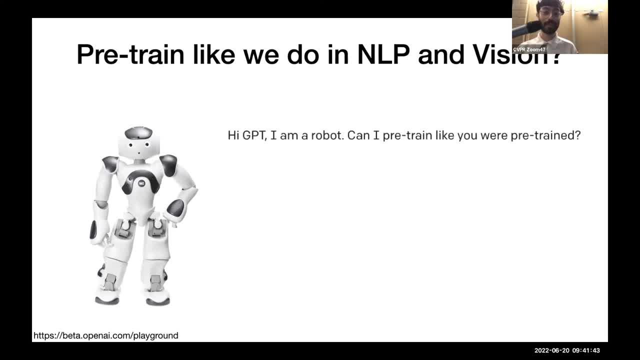 Okay, but let's ask GBT: can I pre-train the way that you were pre-trained? Any guesses on what GBT is gonna say? Okay, GBT says no, no, you cannot Pretty like definitively. So the robot's pretty sad here. 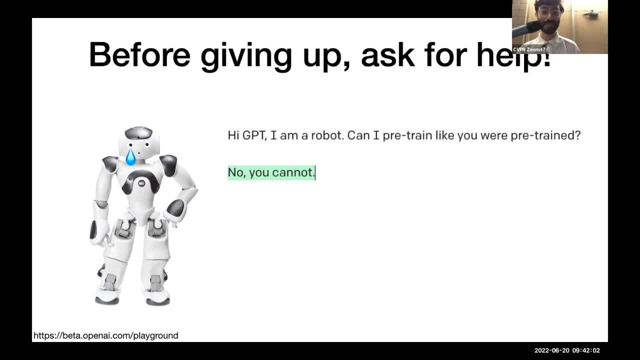 So what do we do now? Do we sort of give up? No Before we give up, we give up. No before we give up, we give up. Maybe we can just ask for some help. So we say, okay, no, you cannot. 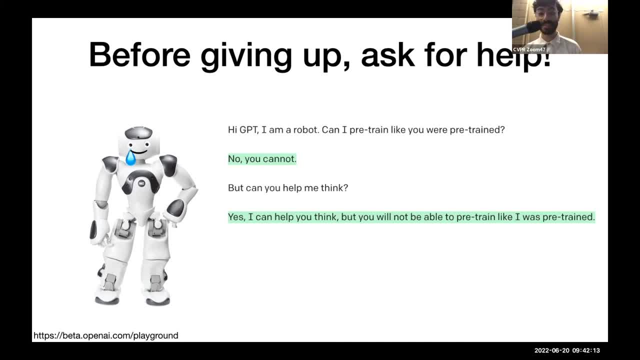 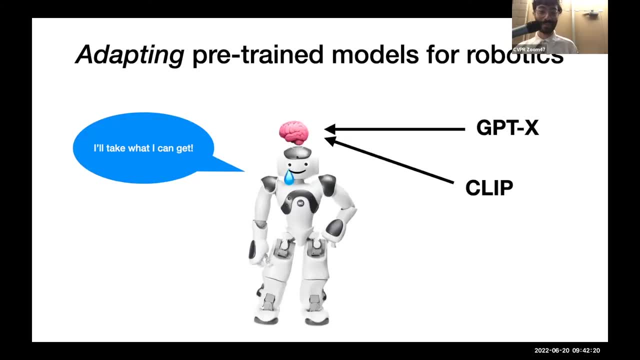 but can you sort of help me? And GBT says, yes, I can help you, but still you can't pre-train like I was pre-trained. So it's pretty adamant that you can. So here's the kind of working idea now. 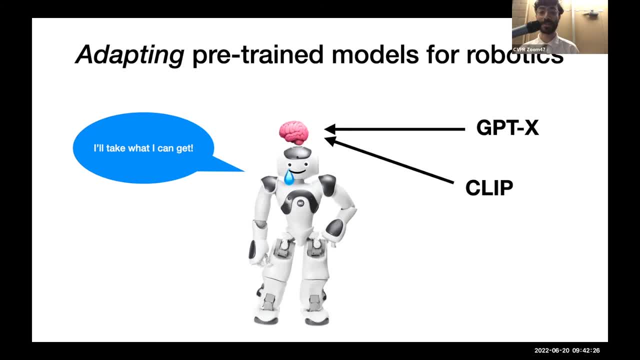 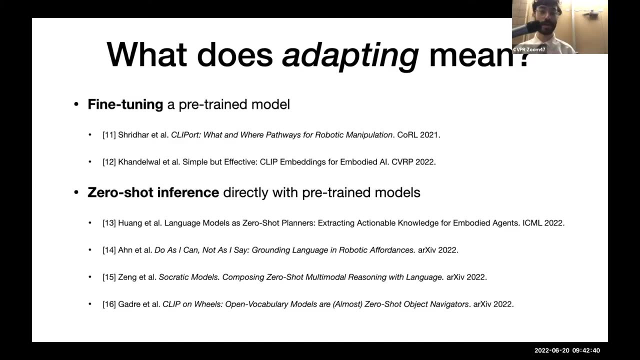 is that the robot is sort of gonna take what it's gonna be going to get, And how are we going to adapt GBT and clip in order to do robotics and models of this, Presumably? So what do I mean by adapting? I could mean like a couple of different things. 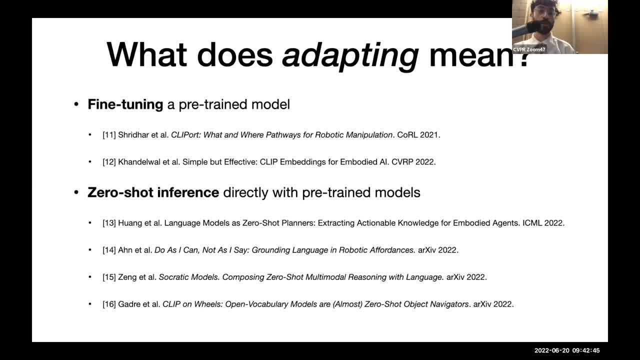 So one thing is fine tuning on top of these representations. Another could be zero shot inference, So directly using their zero shot capabilities for robotics, And I'm gonna talk about a set of this work. So clipboard has already gotten like a lot of mentions. 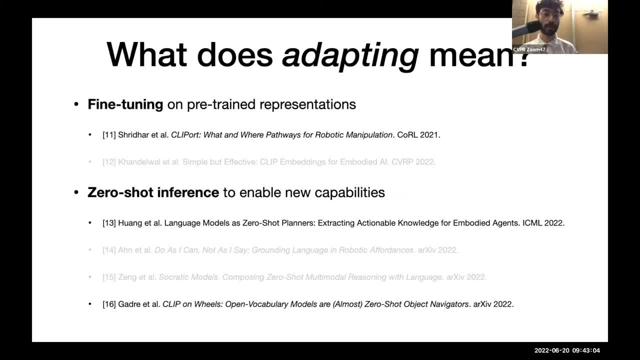 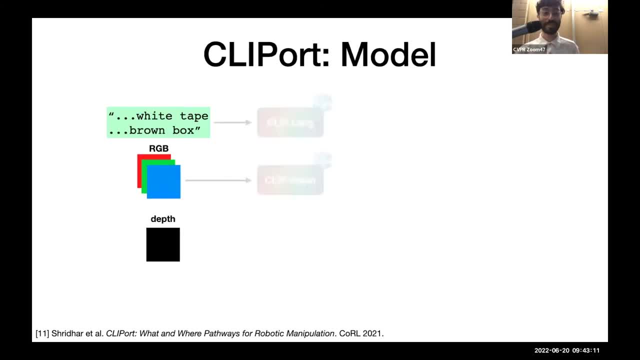 So I'm just gonna kind of breeze over that and then focus on these two works Using sort of zero shot methods. Okay, so I'm actually just maybe gonna- since we've talked about clipboard quite a bit, I'm just maybe gonna show their demo videos. 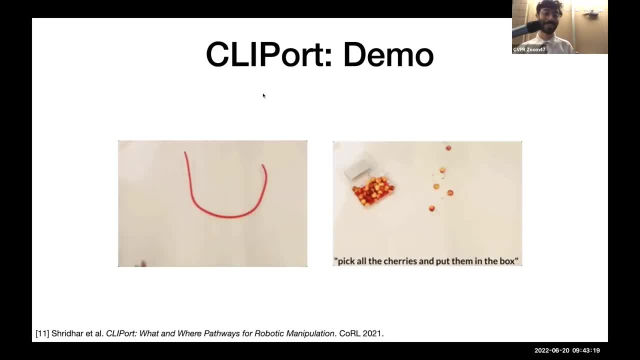 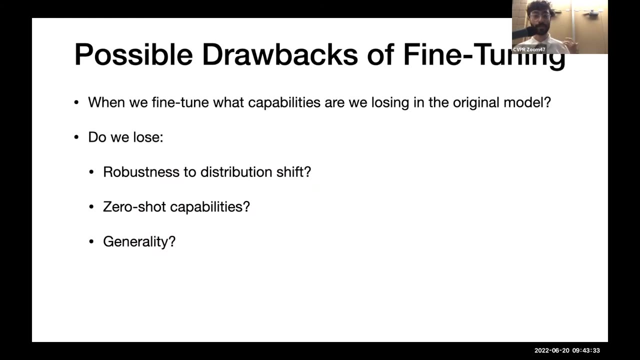 which I think are really cool. So here's like a example of, you know, closing a loop on a piece of string and then like picking up cherries, Okay. So, as I've explained before, I've kind of like made a Đâyм. 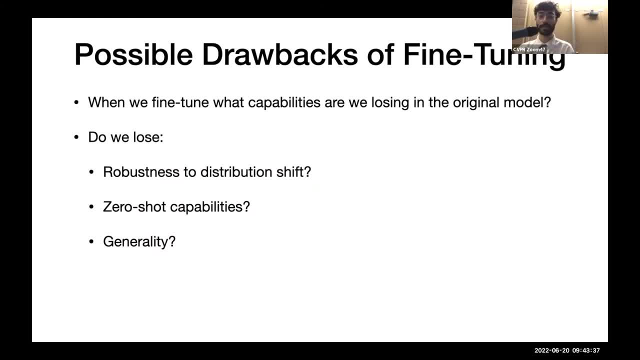 Okay, so, as I've explained before, I've kind of made a Đâyм, So as sort of Andy and others alluded to, you kind of have to do this, this, this training on top of clip, And so I think it's important to think about what we're maybe using by doing this. 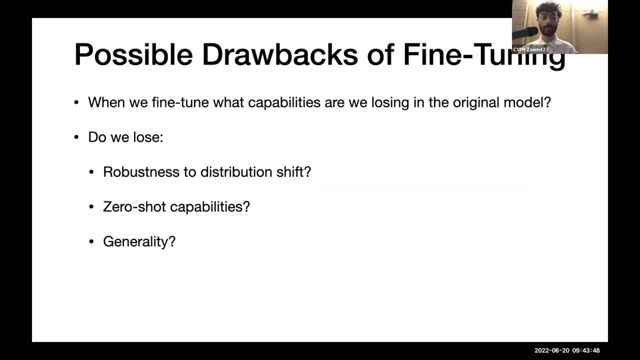 And here are some possibilities For one you could. you could imagine losing a bit of robustness. so these models are incredibly robust to a lot of distribution shifts. but when we start training them on sort of these target demonstrations in more of these tabletop settings, 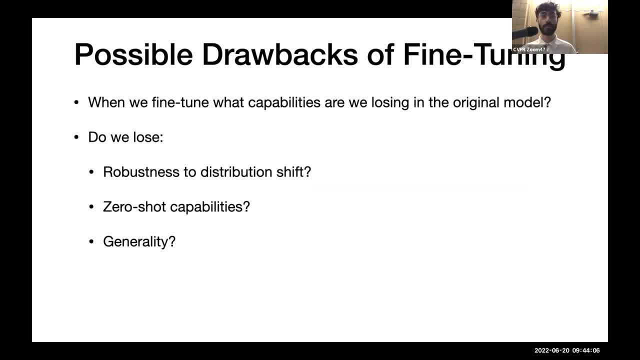 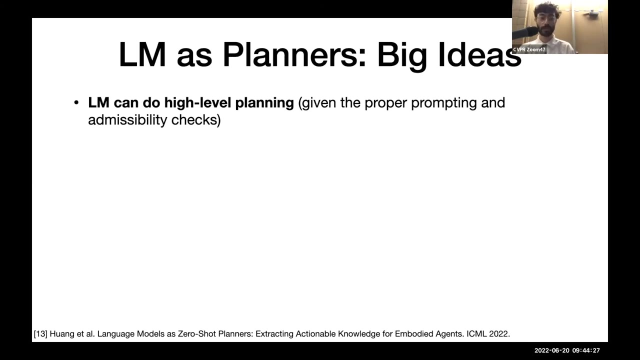 maybe we start to like sort of throw away those, those really nice properties. clipboard does show some kind of like generalization of different concepts, but maybe it's not as generalized as sort of the original clip model. So another alternative, I guess, is to kind of use these models zero shots. so the first paper I'm going to talk about along this direction is this: 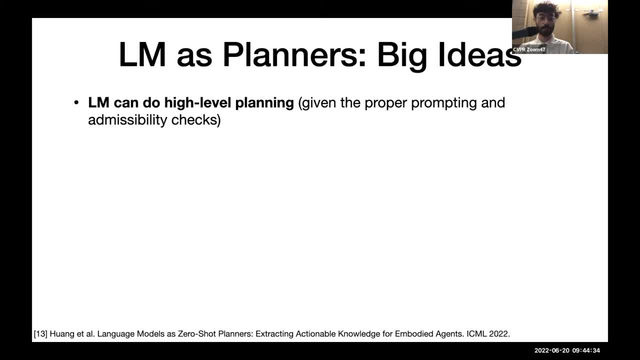 Huang et al paper Called that essentially uses language models as planners and the high level idea very much is the title of the paper, which is that by sort of prompting these language models, we can actually get them to give us high level plans. 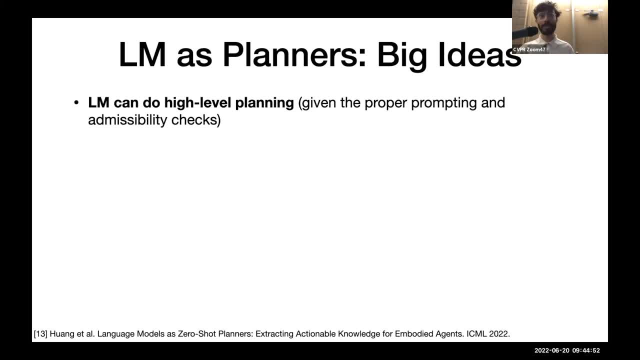 And so what do I mean by a high level plan? You know, maybe getting to New Orleans you would make sort of a high level plan in order to get to New Orleans, buy tickets, jump on a plane, etc, etc. And so it's. 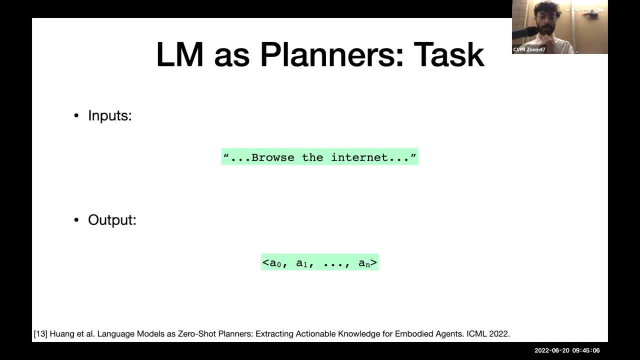 It's kind of exploring that direction. So as input we're going to give a very high level tasks such as browse the internet, and then as an output we want sort of a sequence of actions that will achieve this task. And in this paper the actions are pretty abstract. but you can imagine, for each abstract action you can maybe have a bunch of like lower level actions that implement that that high level action. so this is kind of how these things work. 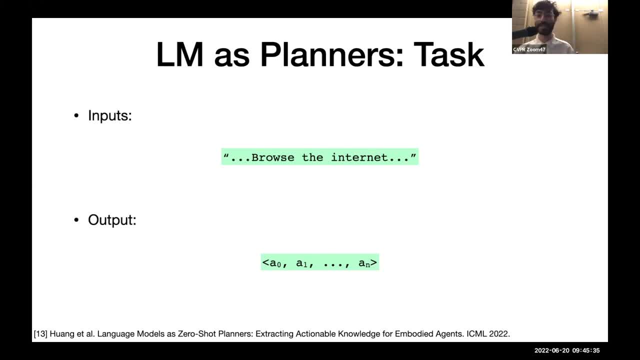 And so this is kind of how these things are related to robotics, ultimately. Okay, so the first thing we're going to do is we're going to have a frozen large language model and we're going to feed it in this browse the internet and then, prompted with step one, sort of trying to get it to come up with what the step is. 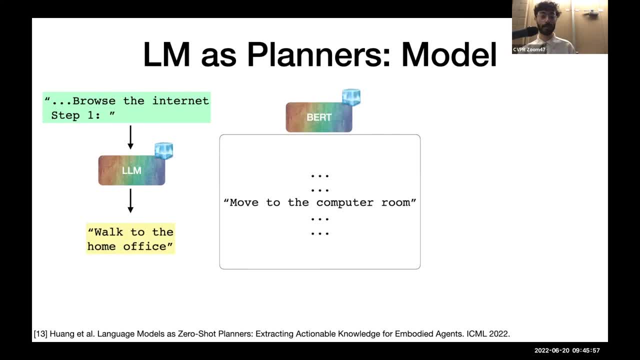 So maybe they'll say something like walk into the home office. But walk into the home office isn't nothing, something that our robot necessarily knows how to do. So we have to kind of do this arbitrage step of retrieving from the actions that we do know how to do, like which one is the closest. 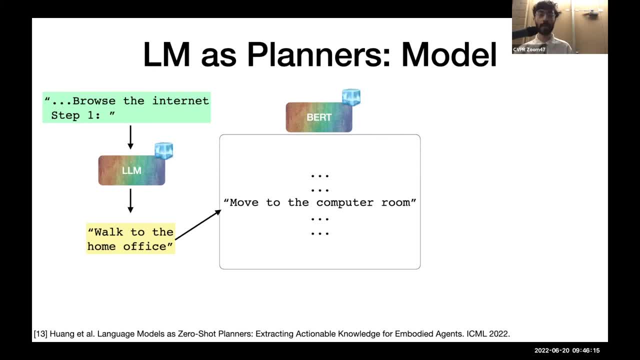 And we're actually going to do that with another language model called Bert. But the thing to note here is that we just have a feature for walk into the home office and features for everything here and we're just going to kind of do like a matching step. 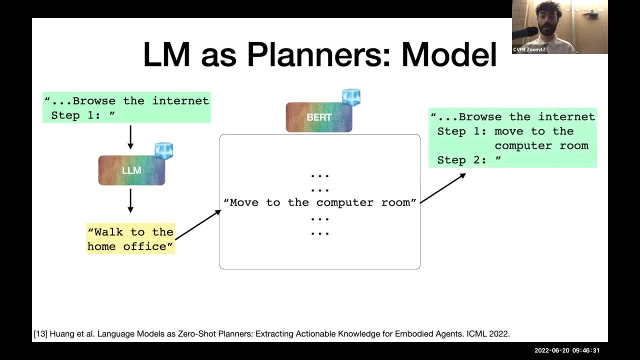 And then we're going to just append this to the, to the prompt, And now we have moved to the computer room, And then we can imagine just doing this kind of over and over again until we have some kind of stopping condition. This is how we're going to get our actions. 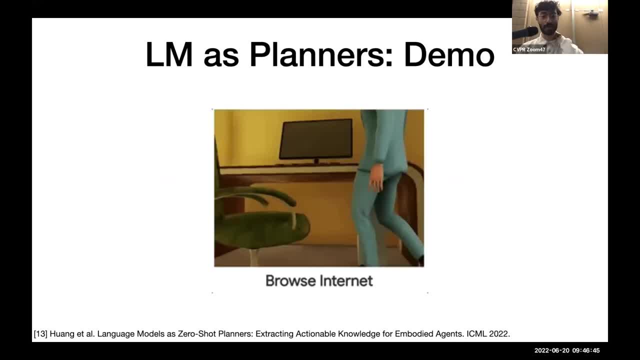 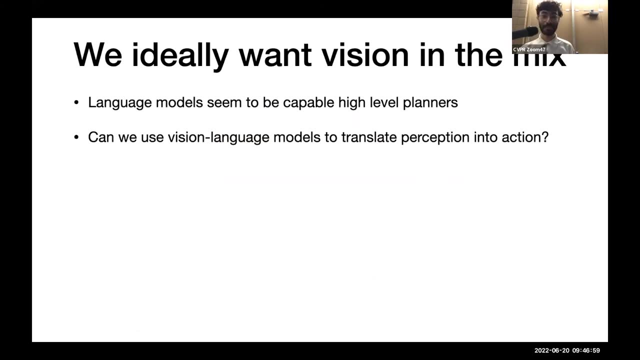 And so this is kind of a demo from their paper of this agent executing these, these high level actions. And then it kind of goes to the computer and it's looking at Google. Okay, but ideally we want vision also. So the last paper I'm going to discuss. 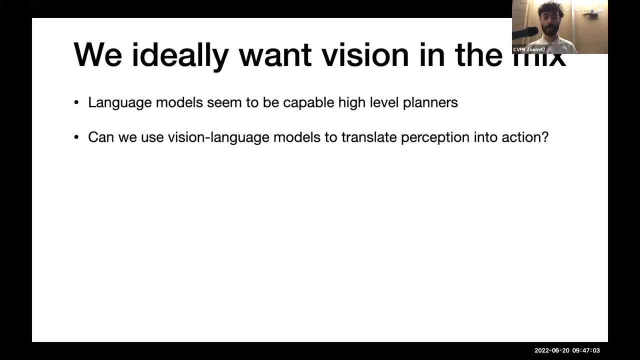 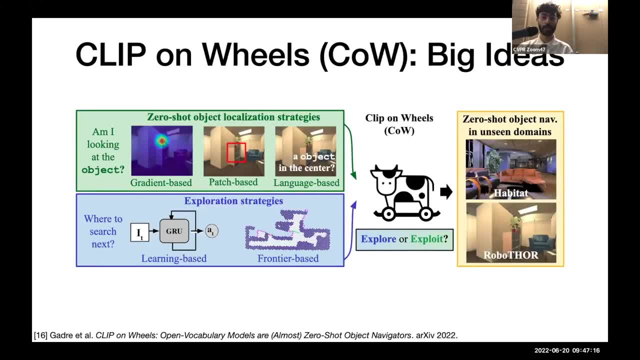 So this is the clip on wheels work, or cow as we like to call it. So the high level idea here is that zero shop models can classify images, Zero shot, as I kind of described earlier. so maybe we can use some Zero shot, as I kind of described earlier. so maybe we can use some vision tools such as like saliency methods or relevance maps to try and extract localization information from these models. 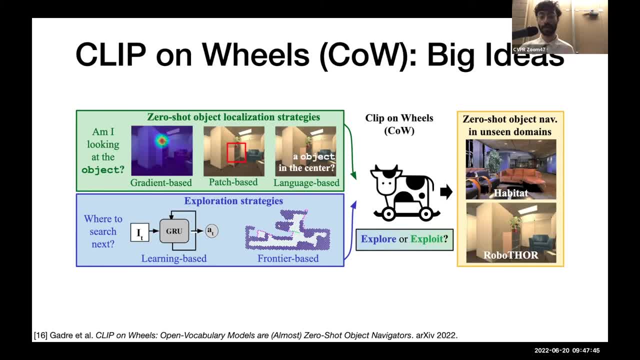 And then we kind of get a very simple heuristic, which is when we've localized the model plan to it in some kind of a map or, if not, just explore until you do generate a view where you've seen the object. So it's a, it's a fairly simple heuristic. 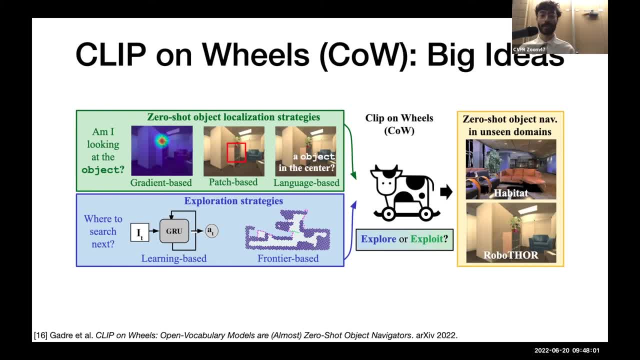 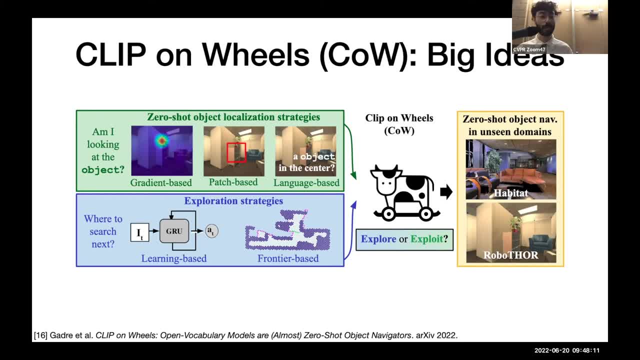 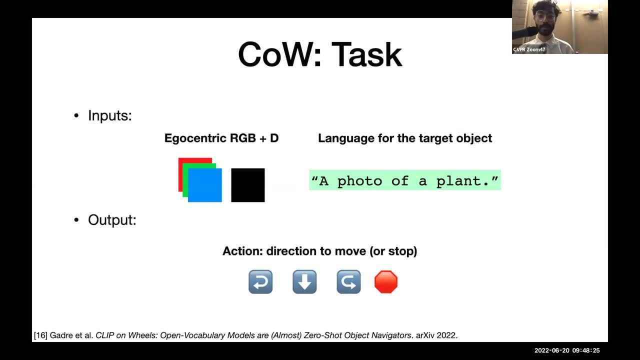 And these, These two environments and habitat and Roberto, or which have very visually distinct appearance, and then start to gain a little bit of understanding about, like the robustness of this method to some distribution chips. So here we have as input, like RGB image and then language prompt of the targets, in this case of plants. 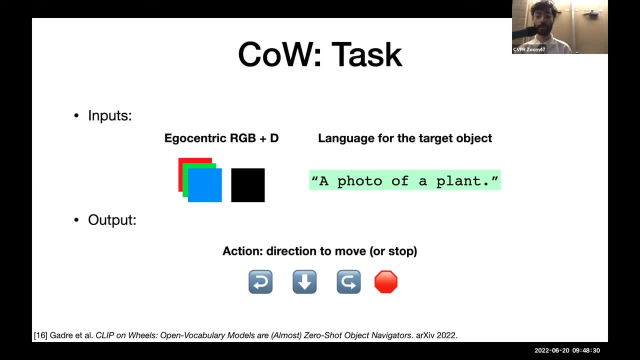 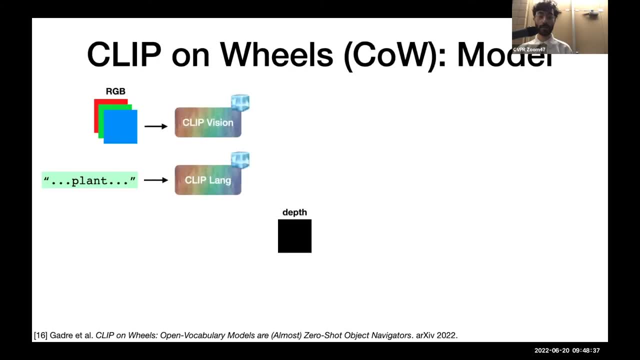 And then language prompt of the targets, in this case of plants, and we're going to output some discrete action, um, either movement action or stop saying that we've found the object. so again, we're going to encode the image and the language to get the features. 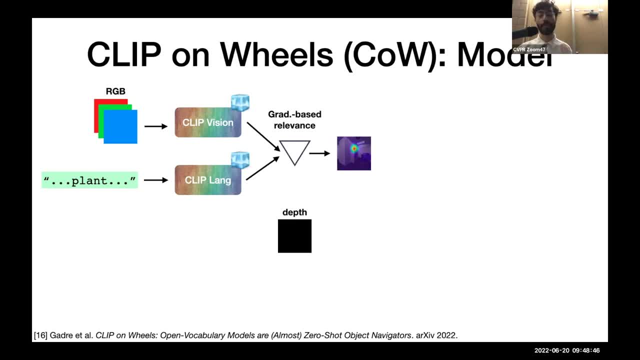 and then, um, we're going to use like a modified version of a gradient based relevance map method, so i think one that is very commonly known in the vision community is grad cam. so this is kind of a modification for that, for the ITs, with a few other other things going on. 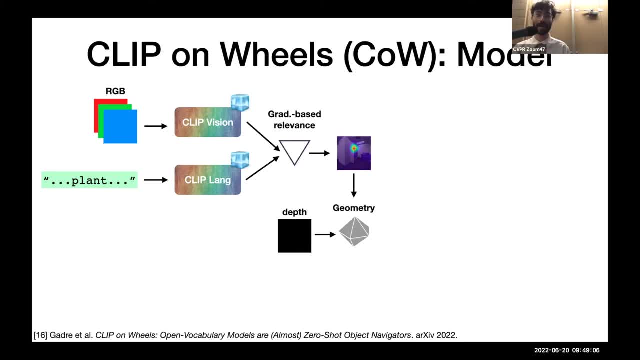 and then using geometry is something way throwback. potentially, in the vision tool book we're going to, or toolkit, um, we're going to, kind of fit these relevance maps that are kind of these top-down things that we can do using like pose estimation plus, um, you know, back projection, and so now 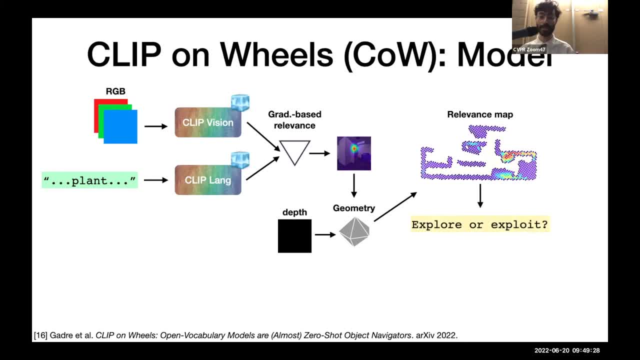 we can ask the question: should we explore or should we exploit? and if we are confident that we found this object, in this case plant, then we just like kind of plan to it using a planner, and if not, we just like explore some more. um, so yeah, so i mean, arguably this is like a little bit of a hack, but 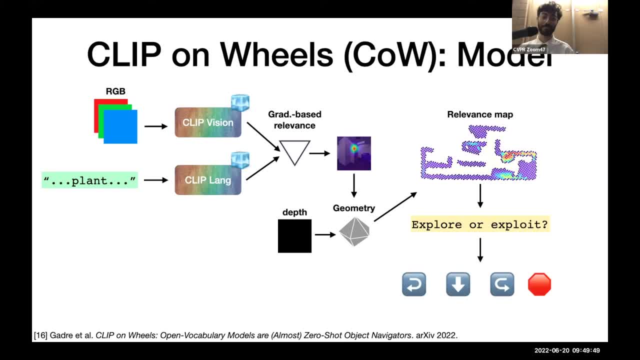 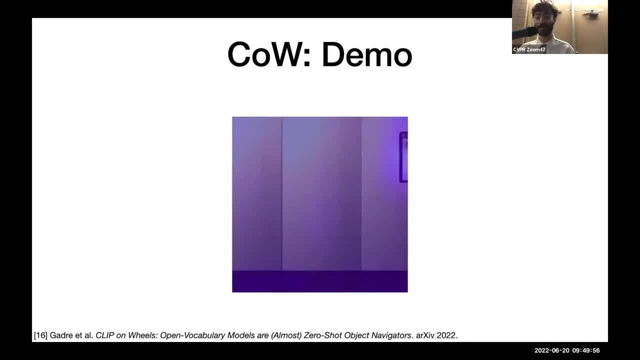 the cool thing is that you don't really have to train um, so yeah, um, and i have just a short little sequence here where we're looking for the plant we're gonna like, maybe explore around. oh, we found it, and now we go into planning mode and, uh, we just move there. so, yeah, that's that. so i think i'm a little bit. 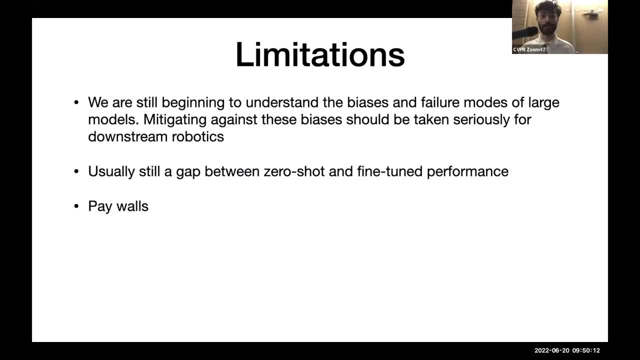 close on time, but i just wanted to say that these are kind of some the limitations of kind of using these large models. so there are known biases in these models, like, for example, racial biases, and i think we should really be taking them seriously, especially as roboticists. 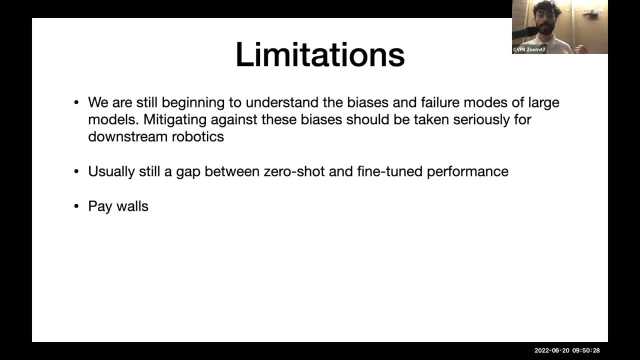 and and vision folk, um, and making sure that these biases do not like affect our, our downstream robotics algorithms, um. so i think that's a huge limitation that that deserves like a lot of study. um, also, there's still like a pretty huge gap between a zero shot method and a fine-tuned 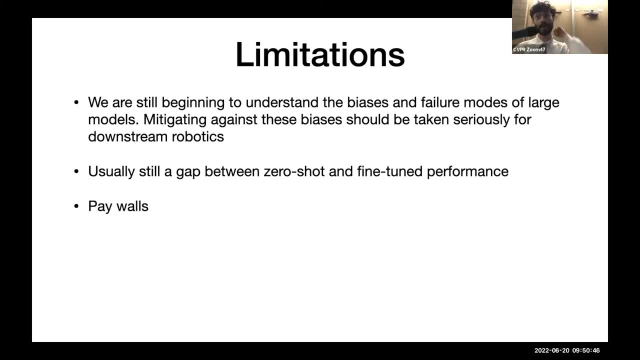 method. so um kind of closing that gap, i think in classification. um that gap is shrinking rapidly but in some other tasks, um, that's that's sort of definitely a limitation. and then paywalls, i'll mention, is another one. like a lot of these models are behind paywalls, um, 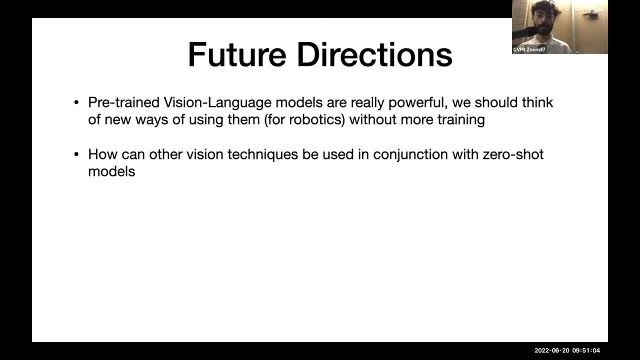 and maybe in the future this will become more common. so it's just something to keep in mind. and on the direction side, um, basically these models are very powerful and i think they kind of open up some new like algorithmic possibilities and we should start thinking about. 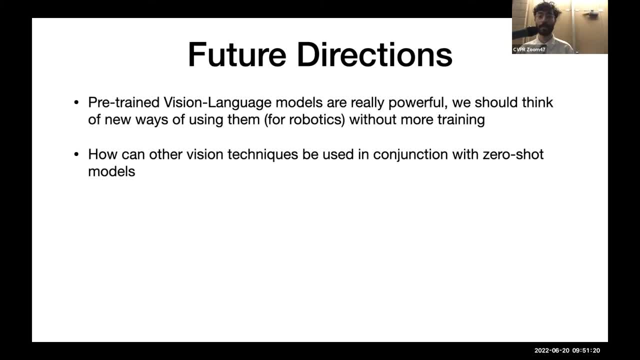 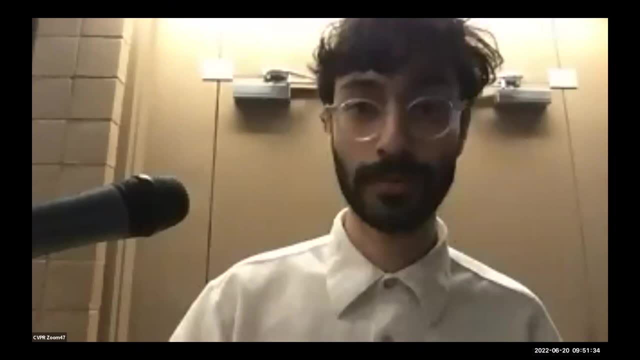 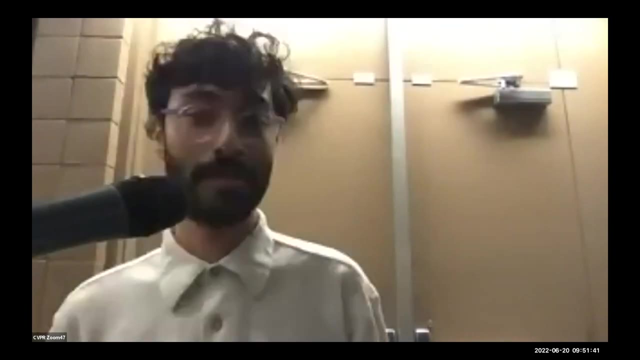 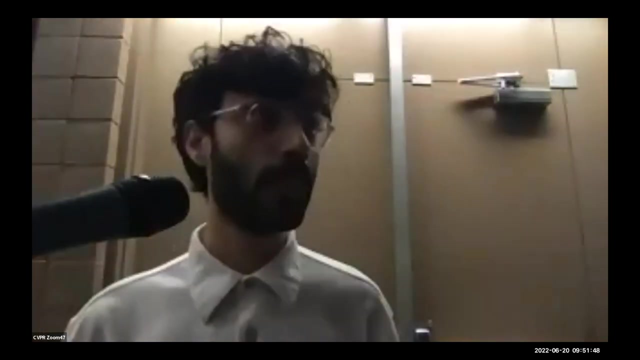 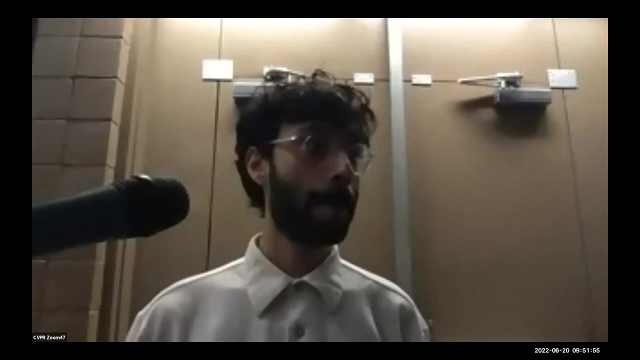 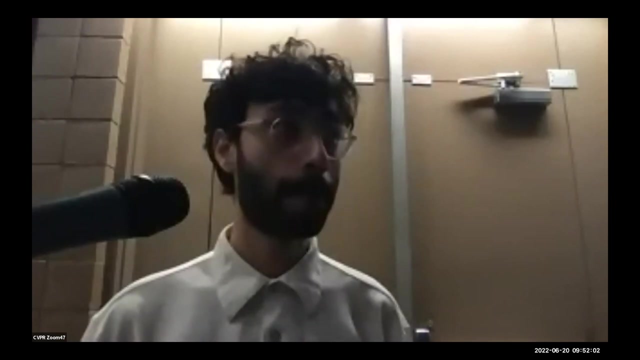 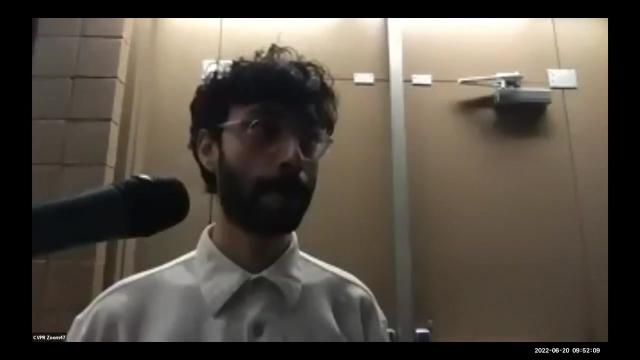 those, instead of, uh, necessarily just trying to learn everything, although i think learning probably is a part of the process. so yeah, so, yeah, so yeah, people have questions. so so, yeah, so, yeah, So, yeah. so that's a good question And I, I think, 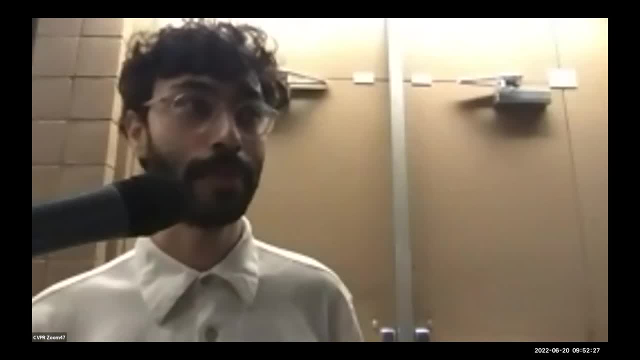 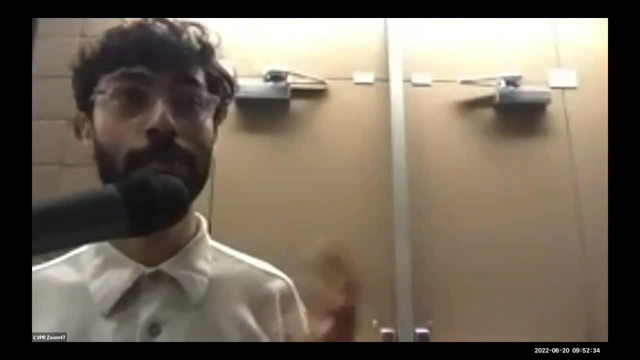 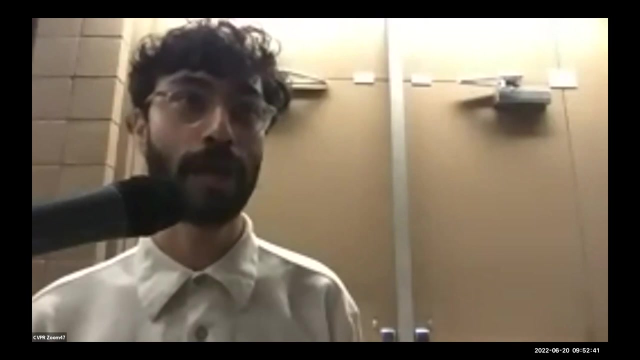 so I think part of the reason that this, this direction, makes sense of leveraging the large pre-trained models is because because we actually do know how to plan. So if you know the sort of robot geometry then you can maybe implement a lot of low-level actions. 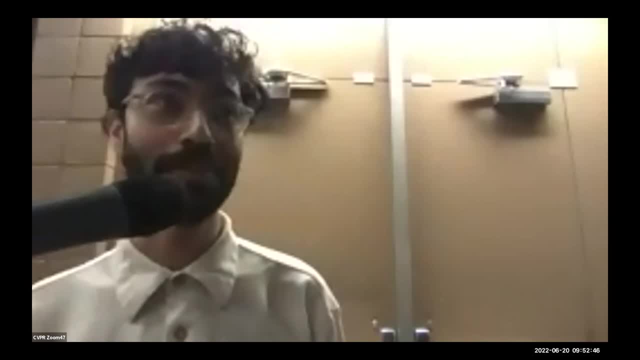 like through planning frameworks, Like, like I said, I don't know if this is, like necessarily the answer long-term, but it does allow us to do things with, with these kind of large models, as kind of doing the reasoning behind the planning. 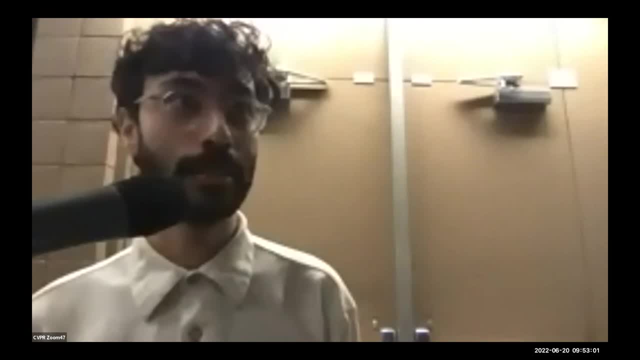 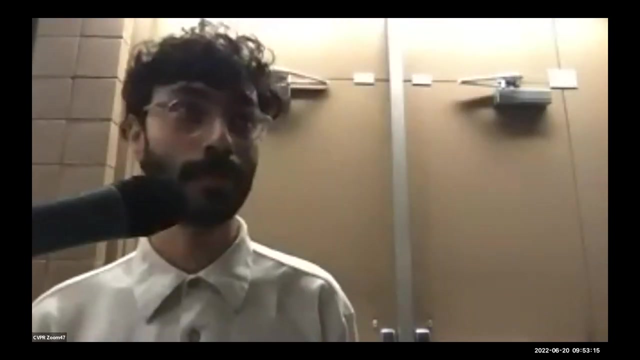 Yeah, Does that? does that answer your question? Yeah, So maybe you wouldn't necessarily want to have a large model to model actions, although that could be interesting as well. Yeah, Yeah, yeah, definitely, I think that's yeah. 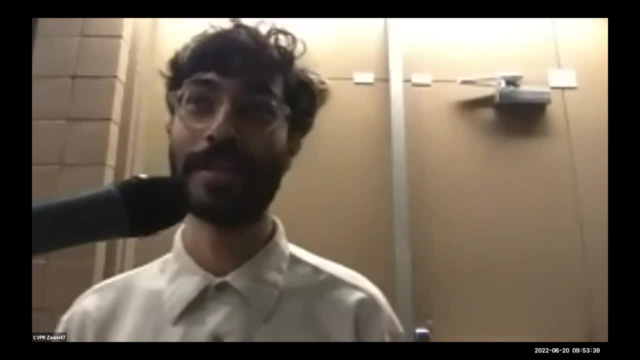 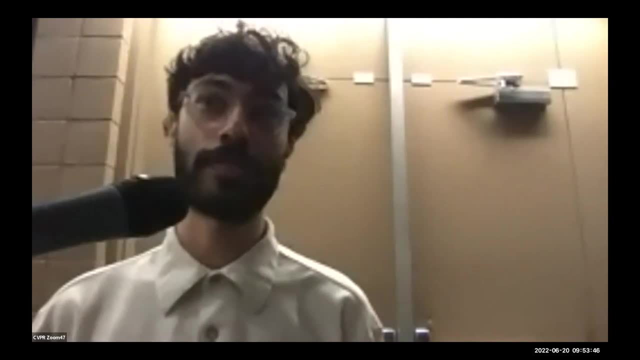 that's a super cool thing that I've- yeah, I've been thinking about that a little bit, Yeah, So I think in the traditional navigation literature people feel that priors are pretty important. So like, for example, if you're trying to find I don't know- 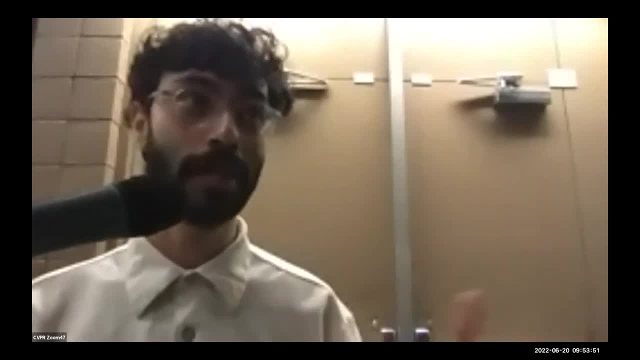 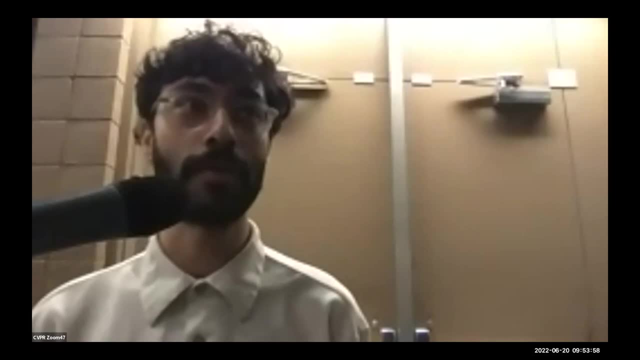 a fork, then knowing that a dining room is close to a kitchen is probably close to a fork is sort of helpful for efficiently navigating. Yeah, So maybe I think it's very likely that language models encode a lot of these priors and that maybe they can be used. 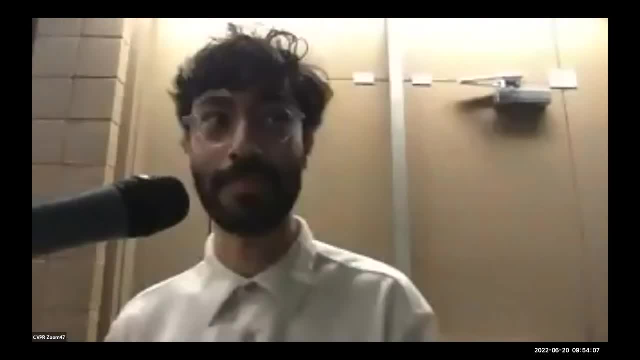 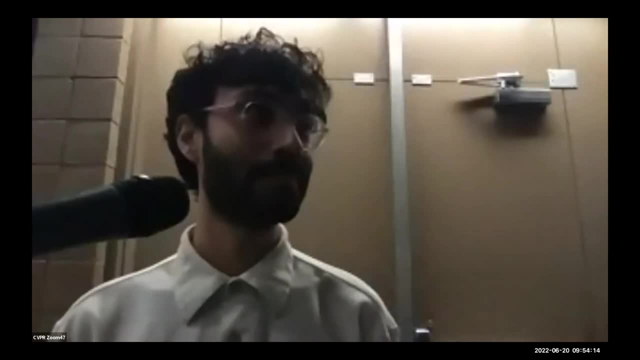 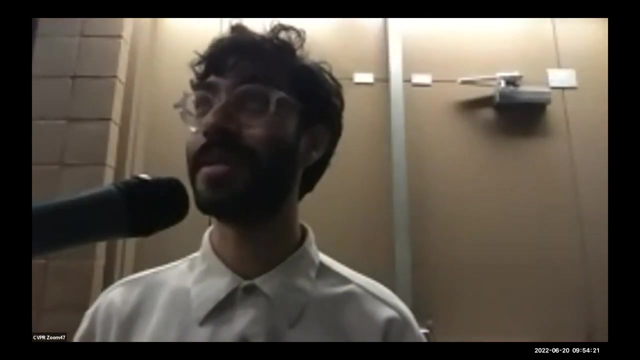 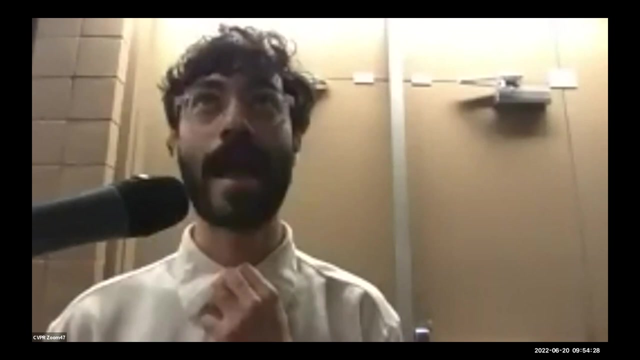 And maybe kind of like the Socratic models kind of line of work I think kind of gets at this too. Yeah, Oh, I mean, I think it's kind of sort of maybe with extending the logic to make, if you want to use the usual thing. 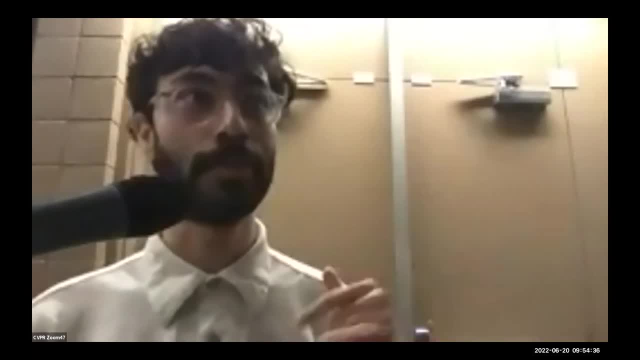 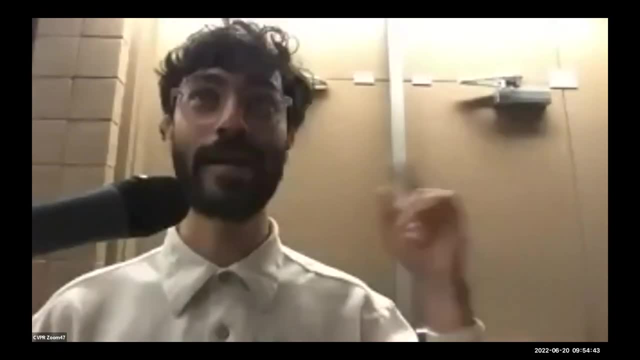 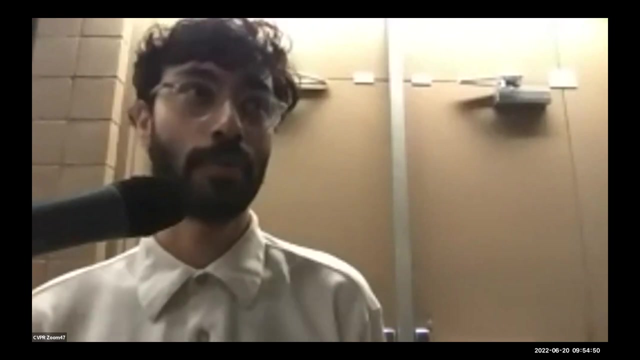 I think that that would be the most useful way to kind of then find a way to do that kind of thing. Yeah, So I think the way we can bring that into some of the sort of interesting things that I'm seeing is to have 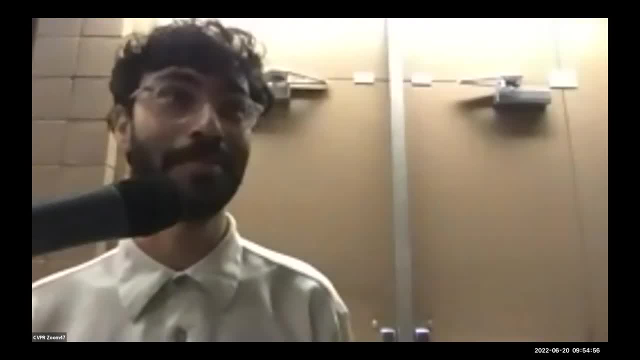 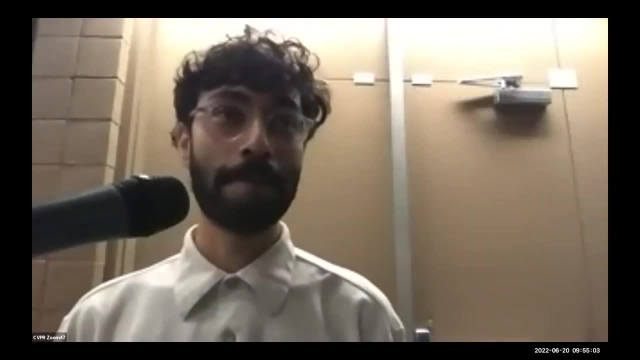 And then it's probably more like a tree-based thing than a list-based thing, but I don't know. Yeah, So yeah, Okay cool, Thank you. Yes, now. It says yes now, Okay, great Cool. 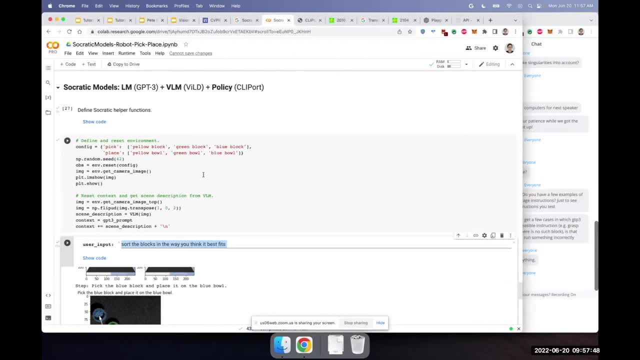 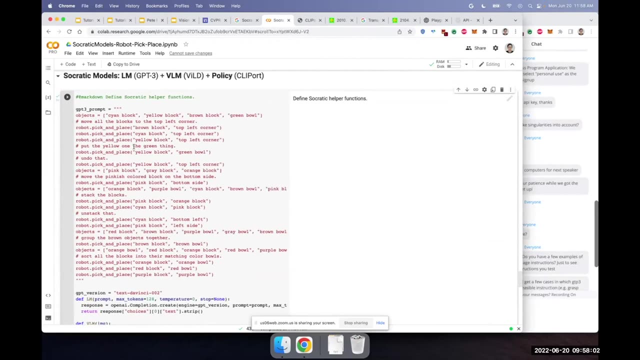 So, with some of these interesting language model capabilities, this last part of the demo ties everything together into this final system that allows prompting GPT-3 to come up with given a list of objects, for example, as detected by the visual language model. 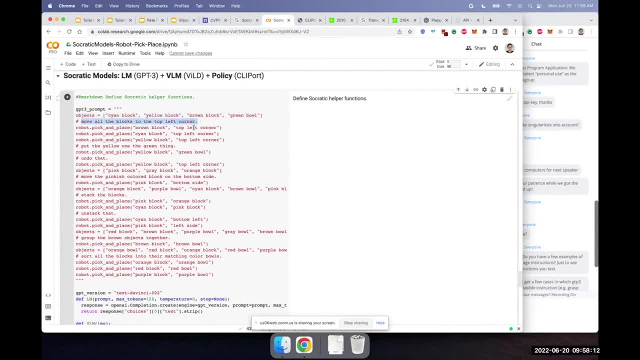 take in the human command and then generate step-by-step pick-and-place commands that it would feed into clipboard. So you might notice that at least the structure of the prompt here that we feed into the language model is of code, Or at least looks like pseudocode. 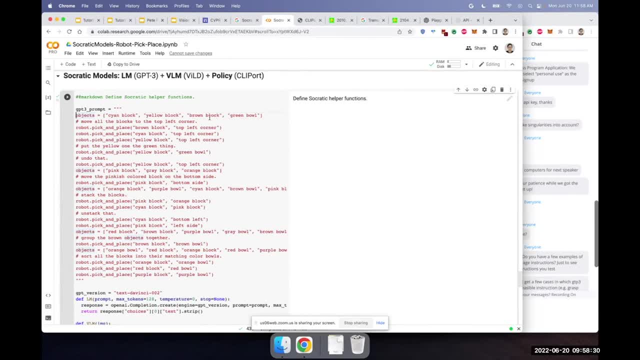 And there's a reason for this. We've been playing around with language models and how we can get them to be very structured in their plans, And sometimes models like GPT-3 might accidentally go out of distribution of the way that you intended to. 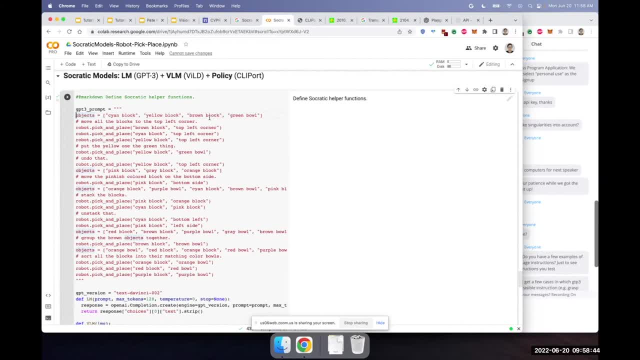 So pseudocode is actually a fairly good way to keep that constraint into, because generally code is structured and the way in which you change your prompts to sort of fit in code is like coercing the model to do that. Yeah Yeah, And so I think that's a good example to zoom into that part of the data distribution that's. 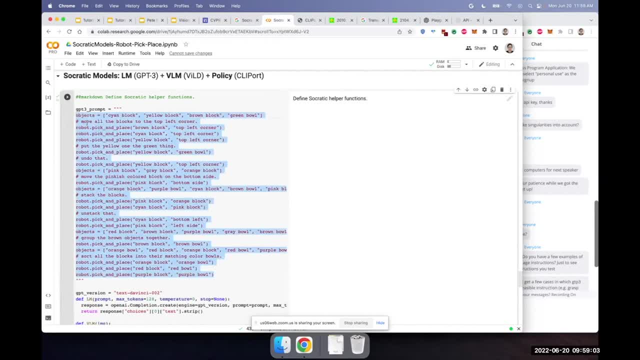 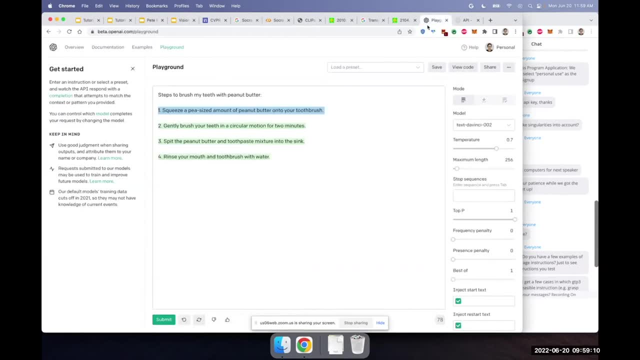 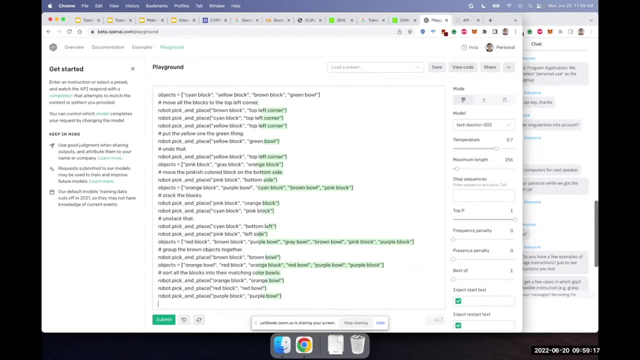 looking at code. So what's what's what this prompt? here is several examples of what kind of outputs we expect GPT system to respond to. So, for example, if you just directly copy paste this into playground, you can play around with what potential output and might be able to generate a condition on some task. 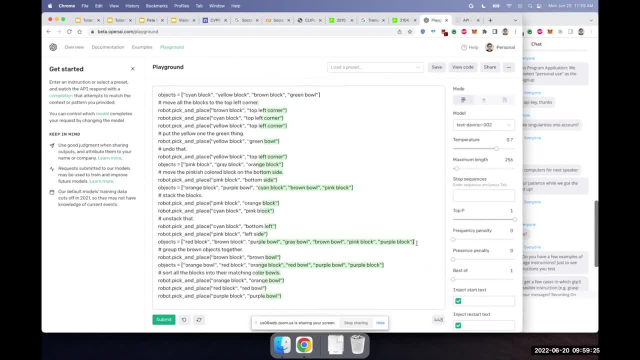 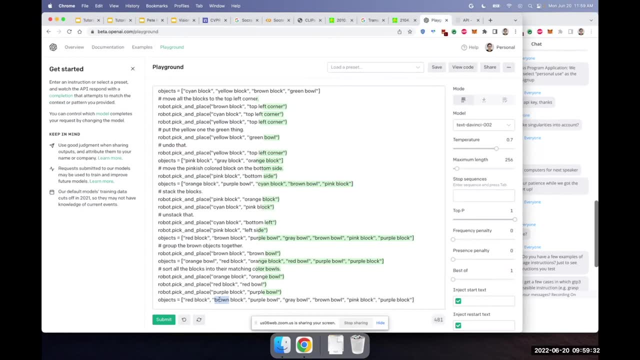 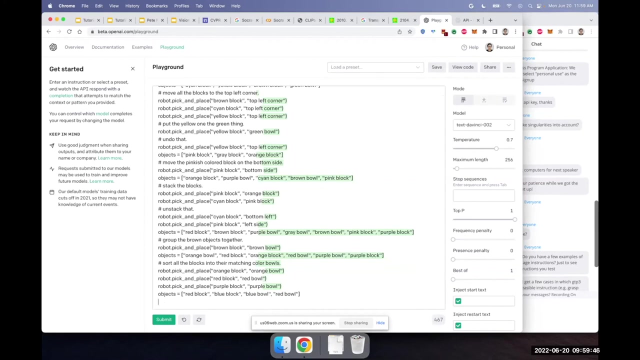 So say, for example: So we can take a list of objects, copy-paste that in say that we have a blue block and a blue ball and a red one. Here we formulated user input from a human as comments inside the pseudocode. 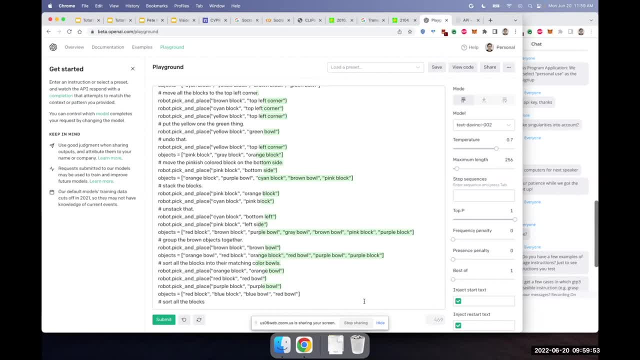 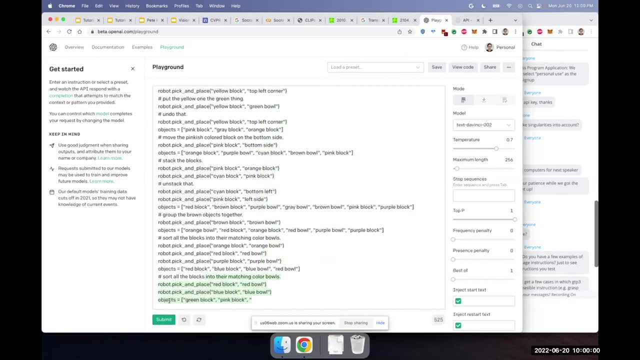 So let's say, sort all the blocks. So I prematurely- or I stopped it here because it was going on- to generate a new list of objects, But really the plans that are being generated by the system here- robot pick and place red block into red ball, blue block into blue ball- is an example of how we're using GPT-3. 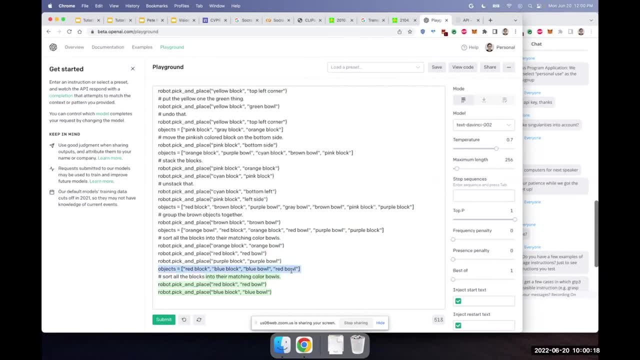 to generate these plans condition on the things that it sees from a visual language model. It's actually fairly cool the kinds of things that this expands into. So, for example, if you list out what objects could be instead of just a red block and a. 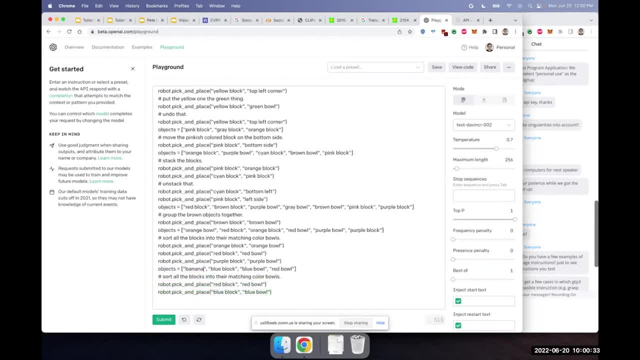 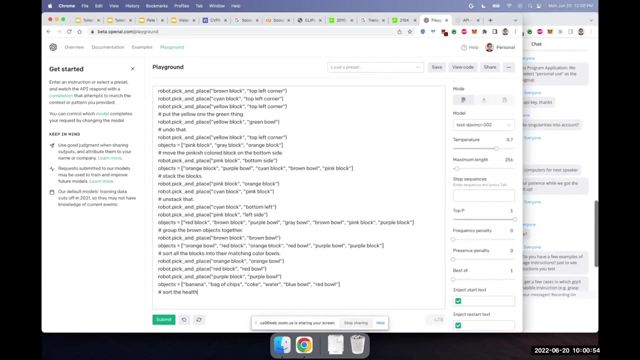 blue block if you say that you had a banana and maybe a bag of chips. add in cook, add in water, And we can change this. We can add an input prompt here to be something like sort the healthy snacks from the unhealthy ones. 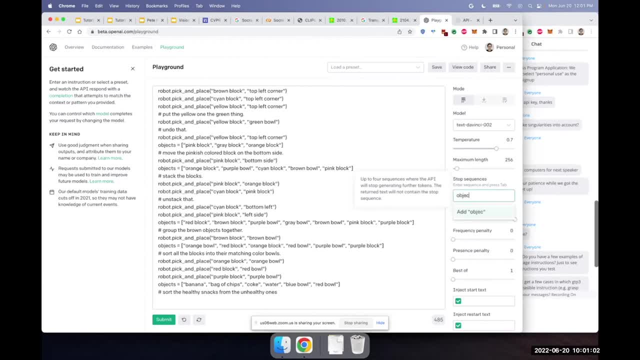 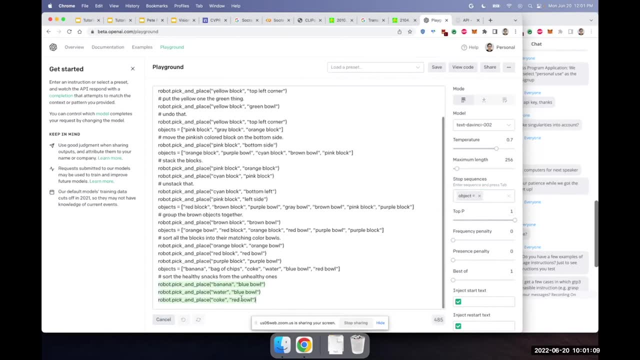 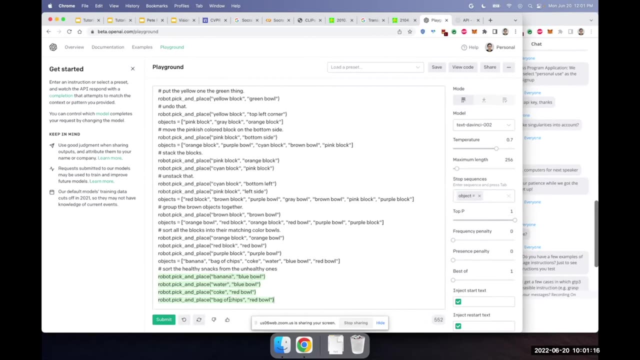 And we'll add a stop sequence here just so that it stops when it's about to generate a new sequence. And it'll respectively, give you a list of pick and place actions that we put the banana and the blue ball, water and blue ball and then cook into red ball and bag of chips into. 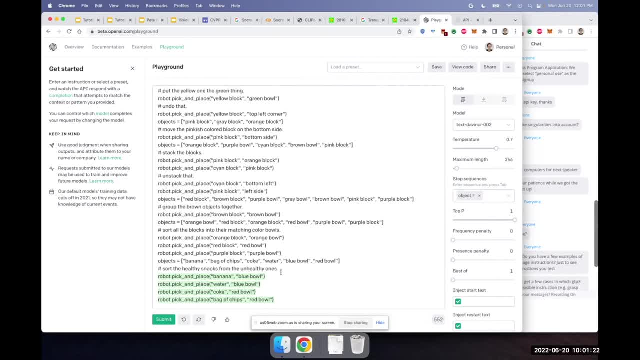 red ball. So it's pretty interesting because it's processing the code and the structure that you expect, but it's also leveraging a little bit of out of domain information to kind of figure out what's healthy and what's not. So the extent to which these planners are capable of these things is fairly unbounded. 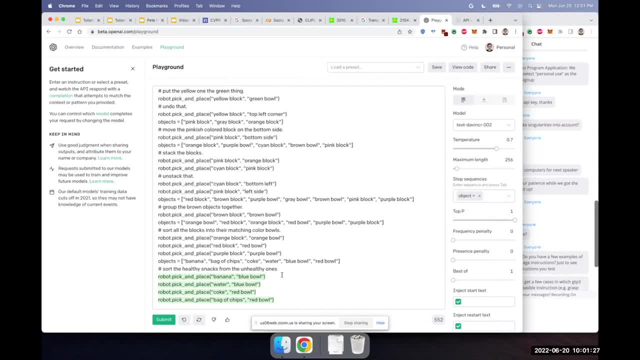 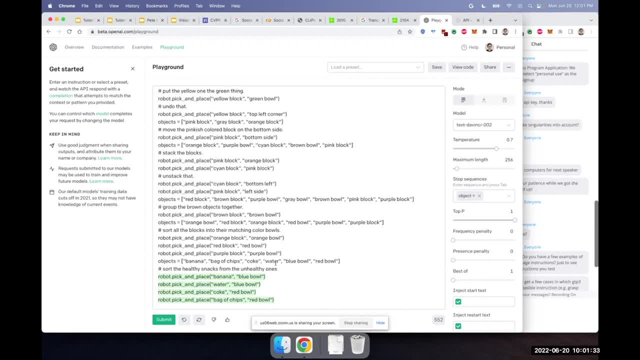 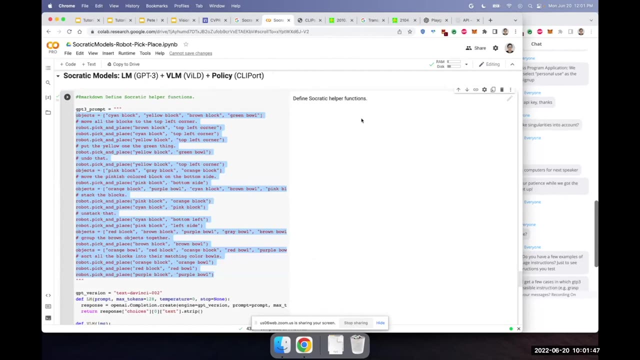 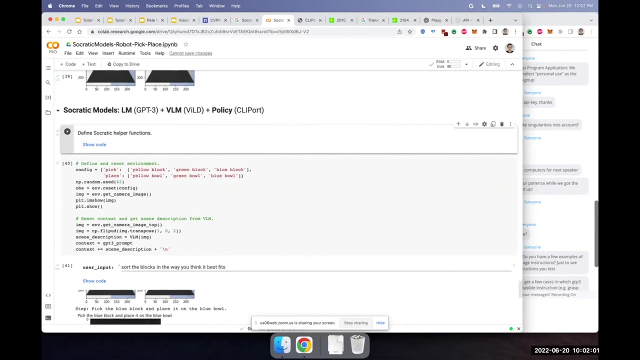 it's sort of a toxic language model from the Internet Data scale. So I'm sure that there's ways in which robots can leverage and help with this. Cool, So in the COVID-19.. So one thing, Oh, The Colab, once you've done run all the end part, and some of you might have been training- 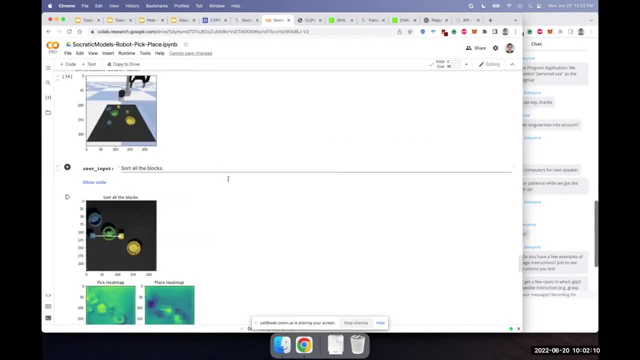 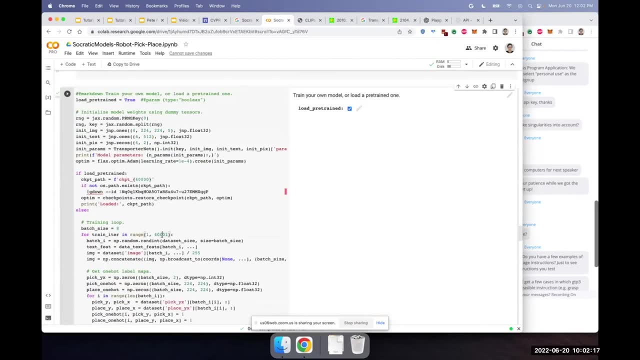 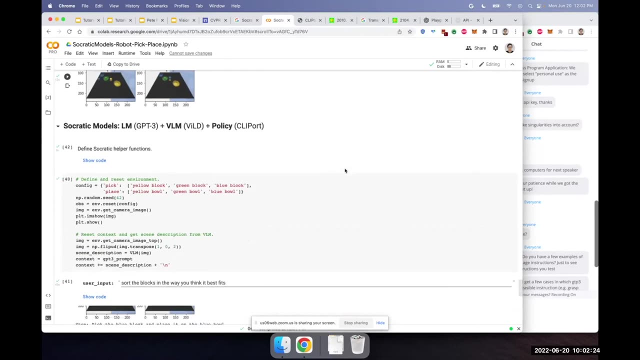 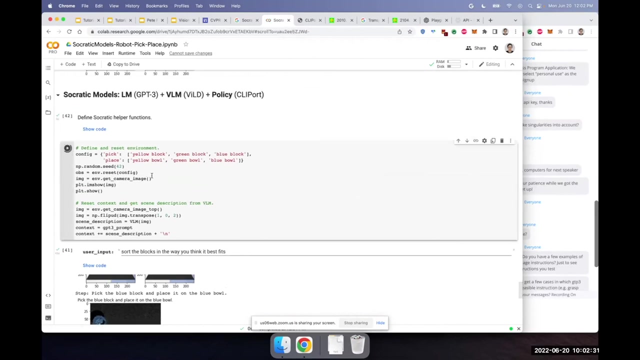 your own models too, and the Colab, at least, sets a max train step to be 40,000, but you can increase this to a higher number, just for more robust performance from the clipboard model. but the tasks that you can do now is: let's just reset the environment real quick. 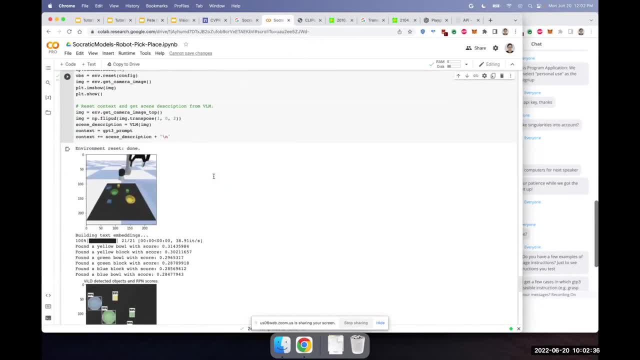 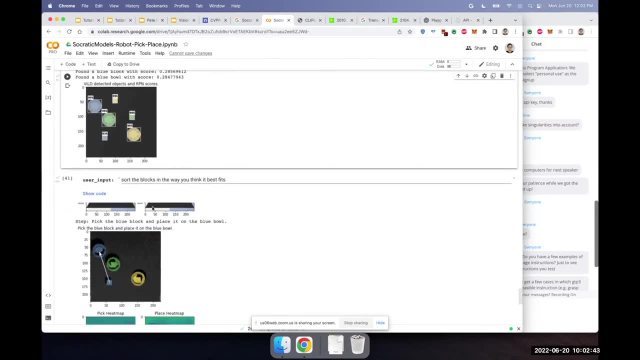 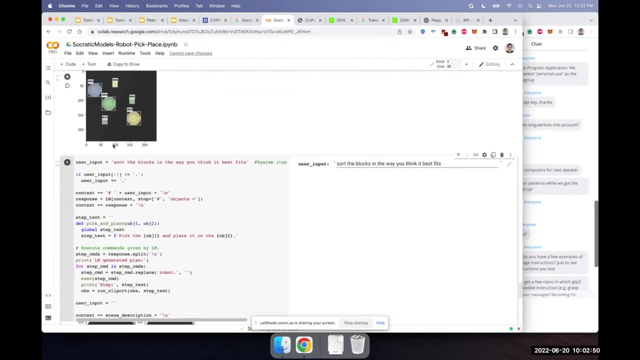 so here we're just going to add the set of objects that we have and run vile so that it can generate a scene description of what objects are available and what the code does is fairly simple: It takes in the outputs from vile and appends that as. 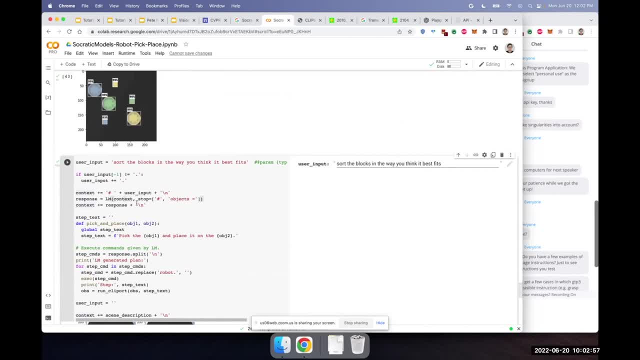 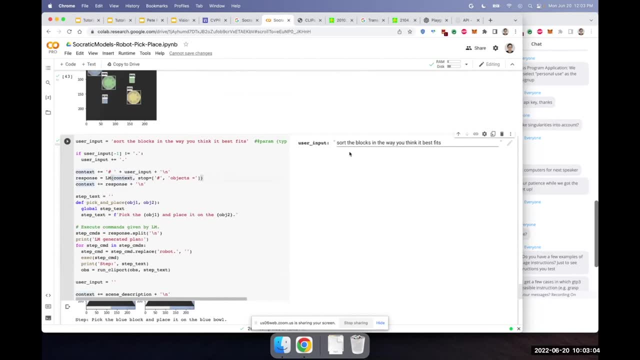 a scene description and then you feed that as context into the language model, and whatever is here in the user input is essentially the commons in the pseudocode. so here we'll just go ahead and run this, Sort the blocks in the way you think it best fits. 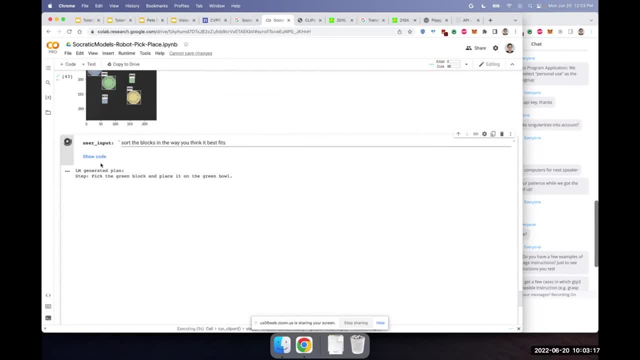 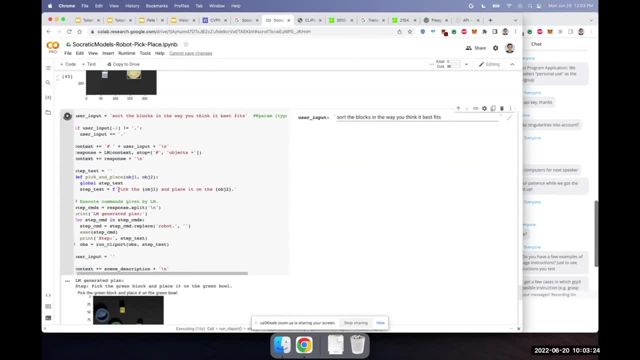 The LM will say: pick the green block and place it on the green bowl. Specifically, it was generating it in the form of pseudocode, but because clipboard takes in an actual sentence, that's of the form: pick the blank and place it on the blank. 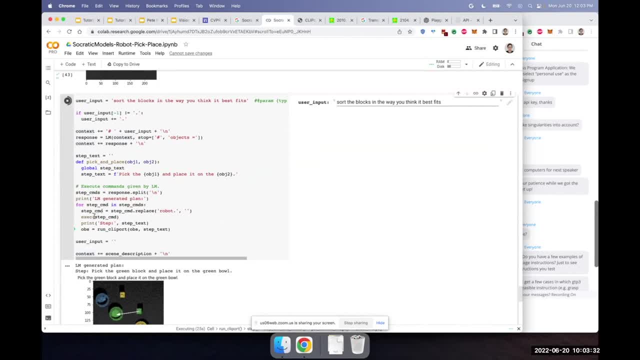 This is literally just using Python execution to run this function pick and place so that it generates the string that it feeds into clipboard. Our previous demos actually just directly would feed in the language step generated by the language model, but ever since we switched to this code-based version of generating plans, 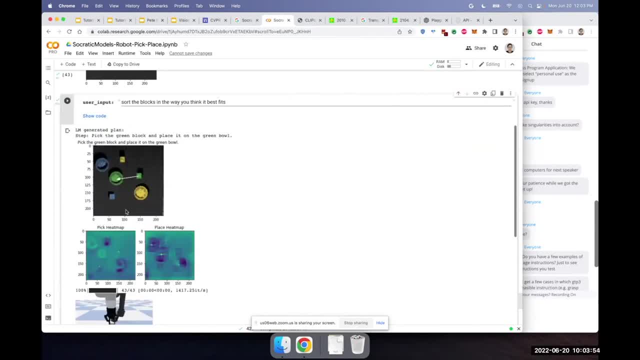 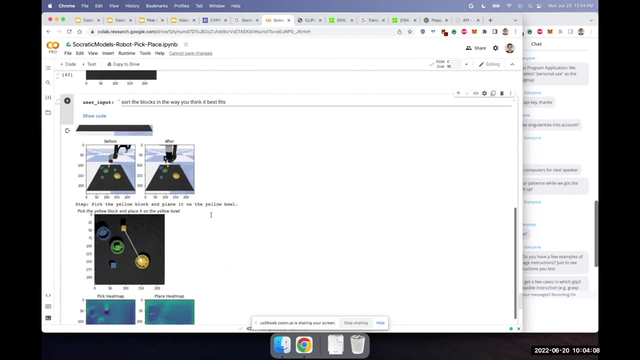 it started getting much more robust results. Yeah, so you'll see that the plan that's being generated- pick the green block and place it in the green bowl- and it looks like it's doing that for the first step. It'll generate the next step: pick the yellow bowl, place it in the yellow bowl and then 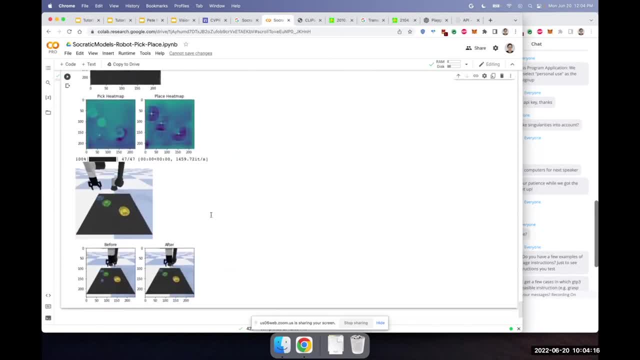 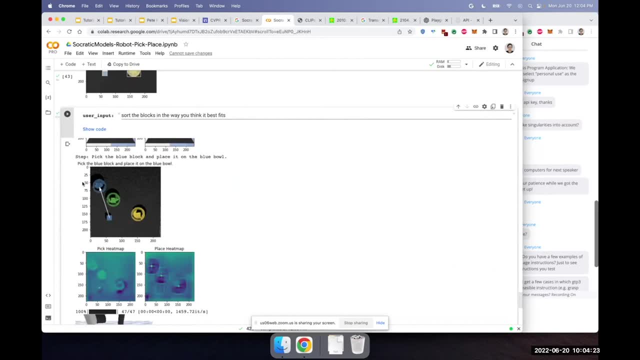 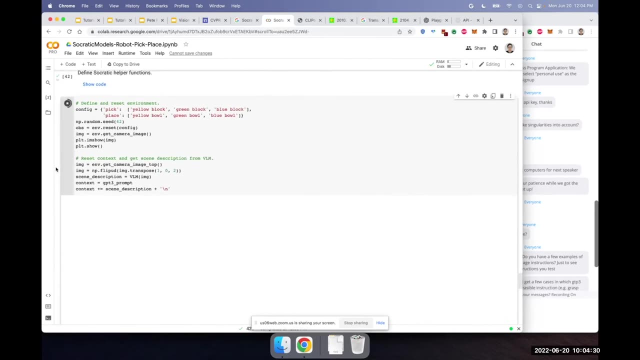 finally placing the blue block into the blue bowl. I think we can do all sorts of interesting things too. For example, we can do a little bit of a loop Okay, For example if we say we can reset this environment real quick. 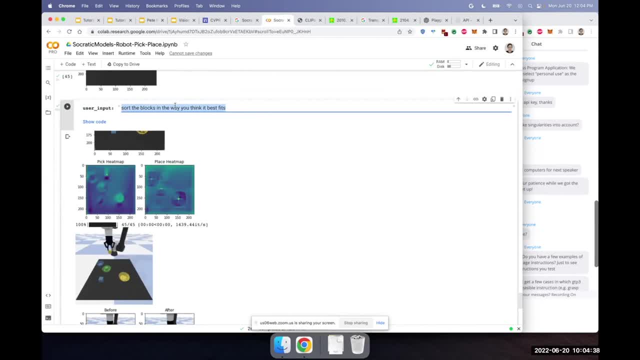 This is untested, but maybe we can say something like: mix the blocks or put the blocks into a loop, Right, Yeah, Well, yeah, So that's the first step, And then the second step is just to go through everything and do a little bit more of a loop. 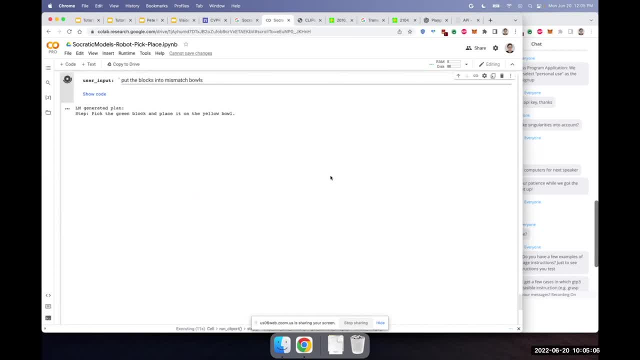 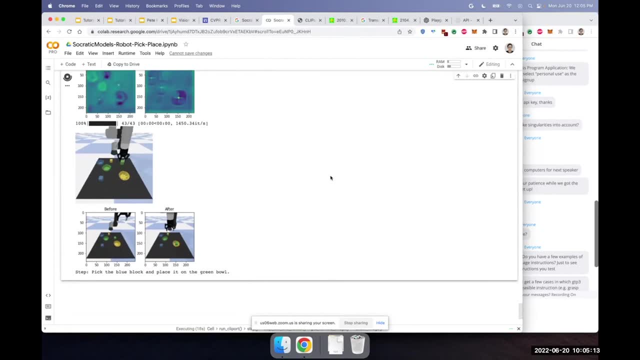 So again, you can do that for the blue block from here into the green block and then go through the blue blocks, put the blue blocks into the green bowl. So that's the first step, and then the second step is just to go through everything and see what we can do And when we do that. that's just going to sit in there, right down here, And then the second step is going to go through everything, and then the third step is going to be putting that into the green bowl. 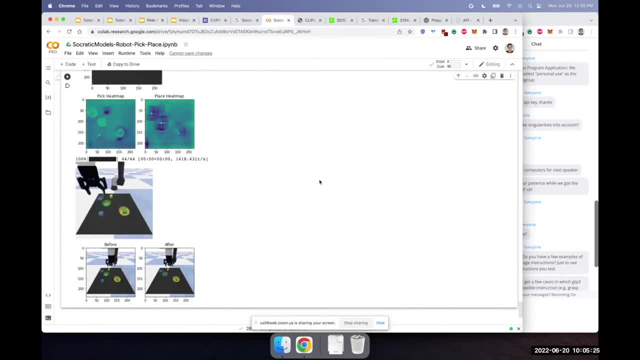 All of those things. Okay, Yeah, the time is just rendering the images from videos. yeah, um, yeah, pete was saying that- um, the vast majority of the time in which it's taking is just having a rollout in the physical environment, in the simulated environment, and then recording the video. um, so, actually, this, 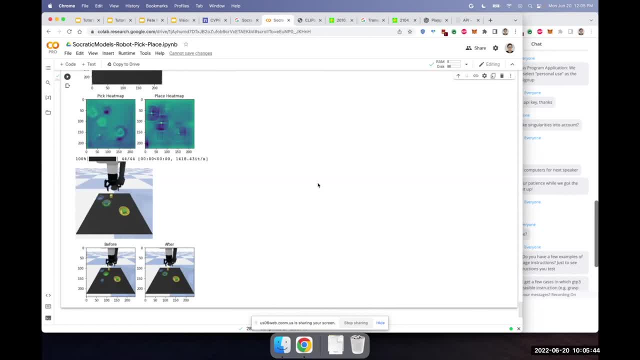 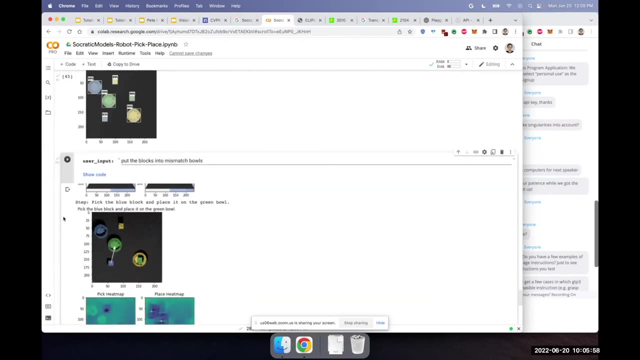 is an interesting point, because if you're doing research in real world, oftentimes you're also gated by just having the time spent on having your robot run. the thing looks like it didn't generate a third step, so i'm not sure what happened there, but yeah, so um. 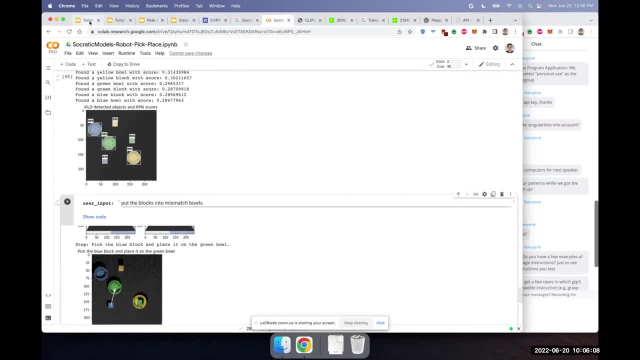 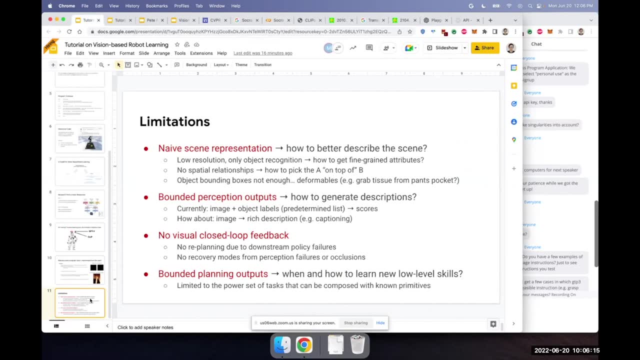 this is a kind of a great segue to go into limitations, um. so if folks are interested in taking this collab and pushing it further to see what our interesting research problems, uh, you'd like to tackle, here is a big list. so the first one is: in this collab we're using a very naive scene representation. we're just running. object: 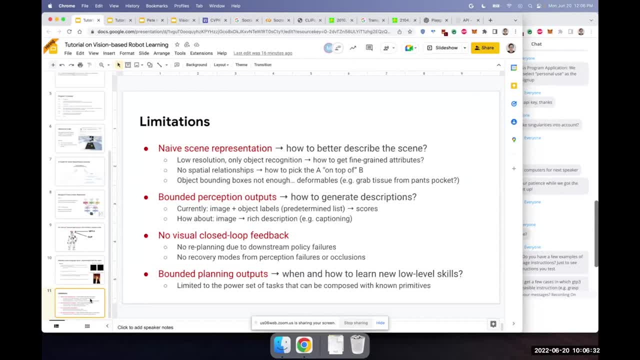 recognition. we're providing a list of that into the scene, but you can imagine that there's value in trying to figure out how do we better describe the scene. are there prepositions, ways in which you can describe the spatial relationships of the objects? do you have a bowl inside of a cabinet? 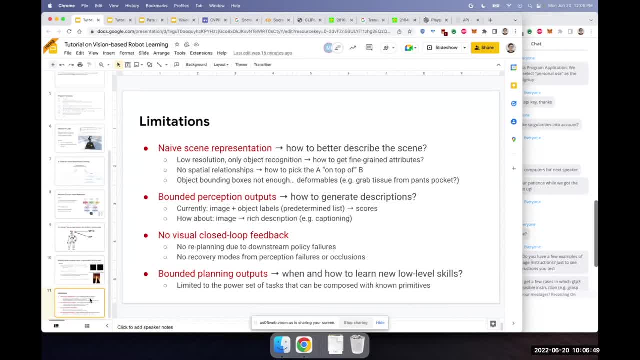 next to a kitchen counter. all of that information could be useful for planning but isn't actually being provided in this system here. so it'd be interesting to see how you can go into higher resolution kind of scene descriptions and and assign more fine-grained attributes even to the 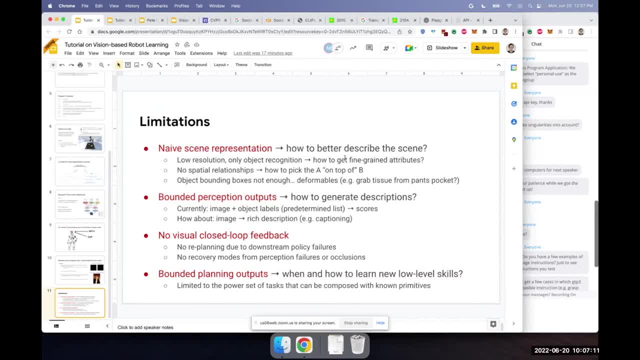 objects themselves, in addition to kind of the relationships between each other. um, yeah, and as i mentioned, there's no spatial relationships. say that you had an object on top of another. currently the system won't know how to say, pick the thing that's on top of the red block. so how do you specify that to the language model? 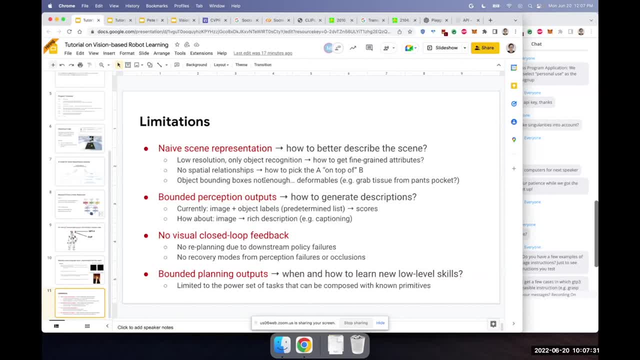 planner is pretty interesting. there's object bounding boxes are definitely not enough, especially if you're interacting with various different real world objects. you have t-shirts that are lying on top of beds, with blankets everywhere. how do you get a system to? uh, how to describe all of the nuances of how a deformable object can be rearranged? 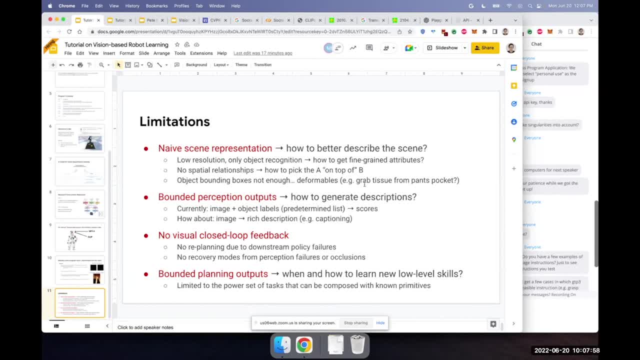 so another example here is: say the test was grab a tissue from the pants pocket, you might need to look into visual language models that are able to give you saliency or relevance detectors of where the pants are or where the pockets are in the pants, and 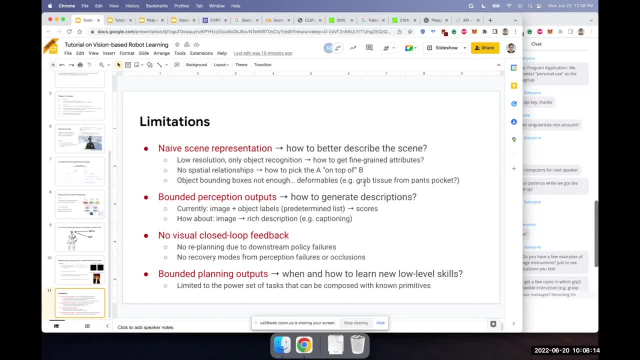 where is the tissue? there's also this question of how this links into low level action. so say that your robot needed to move to a different view to get a better sense of the scene around them. so how do you get the system um to, for example, do some of the 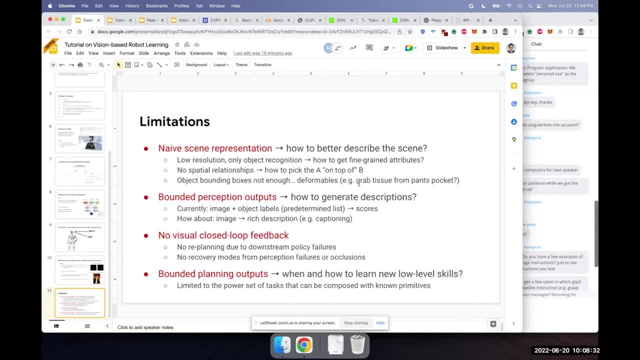 language-based exploration stuff that maybe some of your head mentioned as well. um, bounded perception outputs, uh, so the visual language models. here we are using vial, then we're using clip, um, and specifically with click clip it's using uh, image plus object labels, which is a predetermined list, and feeding them as input. 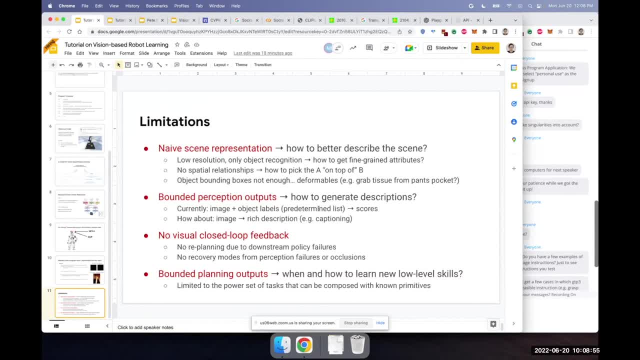 to get a similarity score, so that's okay, but what we really want is a visual language model that can give you sort of generate descriptions just by looking at an image understand where all the things that are in the image and then naturally generating it, because then that 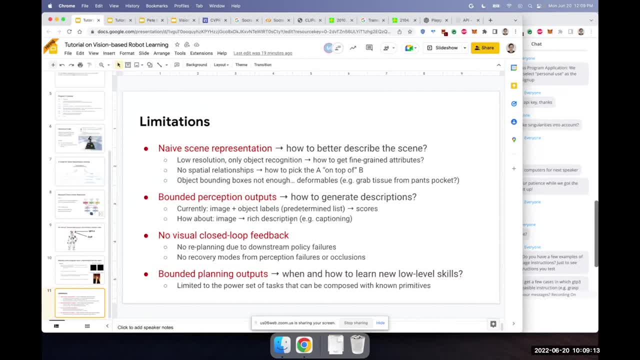 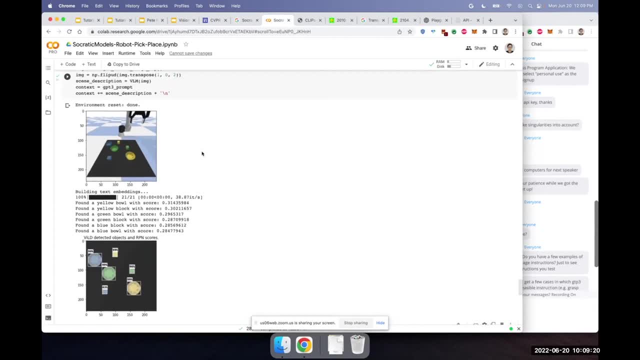 would mean that you don't have to provide the list to the system beforehand. so at least in this collab we've restricted it to say, okay, here are the full set of objects in which you could potentially grasp, and here are all the potential colors you might see it in. this is still a limitation. 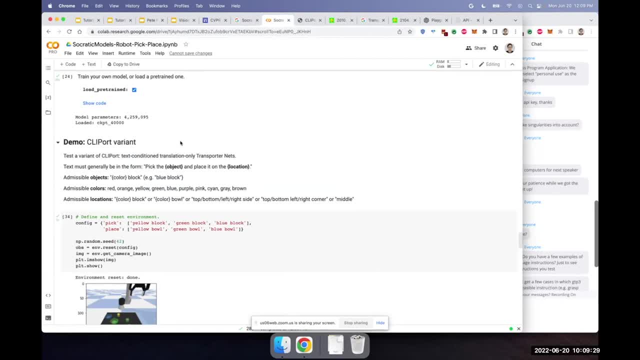 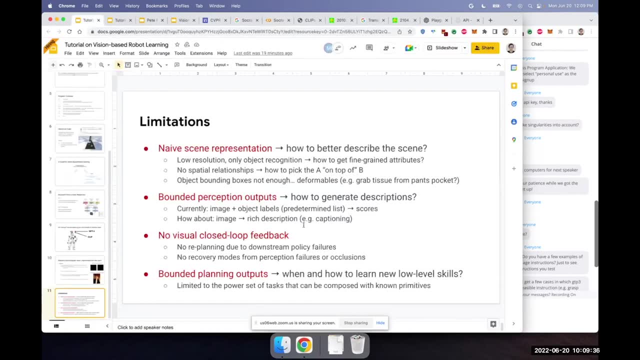 because what if your robot was put in a new environment? how do you get it to generalize the diversity that you might experience in the real world? um and uh. another uh follow-up on that is: uh, there's, there's no visual language model in place, so it's not a visual language model, it's a closed-loop feedback. 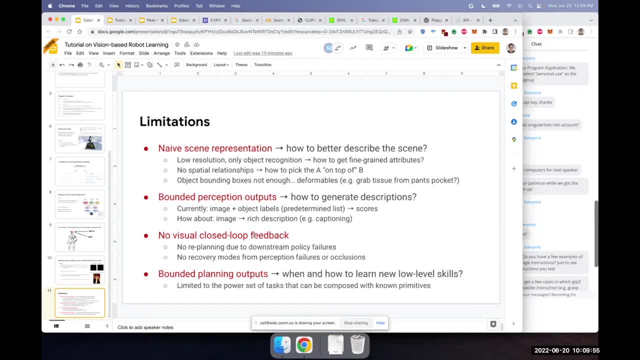 that's happening here, so you might notice that the plans are being generated, but there isn't, for example, a visual language model that's interweaved into the planner and constantly giving it feedback. did you do the task successfully? so this is interesting because if the policy for 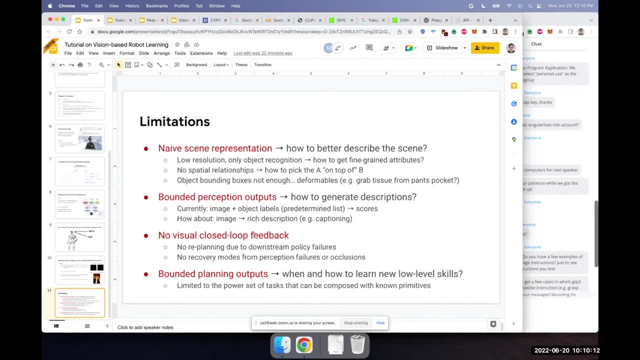 example, fails one of its pick and place actions, then it's just going to continue doing the next step. it's not going to be able to say let's redo that previous step. so if you read the description it's very clear that it's a visual language model. if you do the 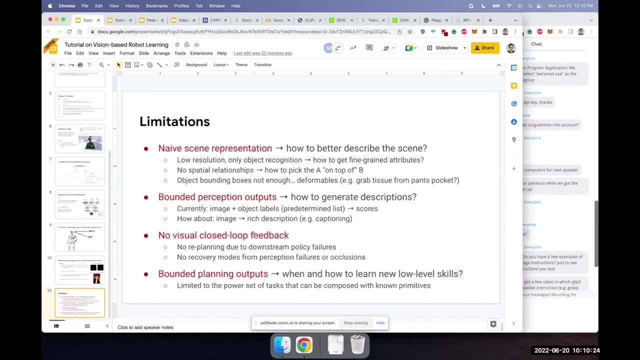 task, you should have very clear data focused on the context of the questions that these people are asking you to answer. so, then, this is kind of a overview, so you might think that these kinds of questions are just here to tell you that there's many more to be said. 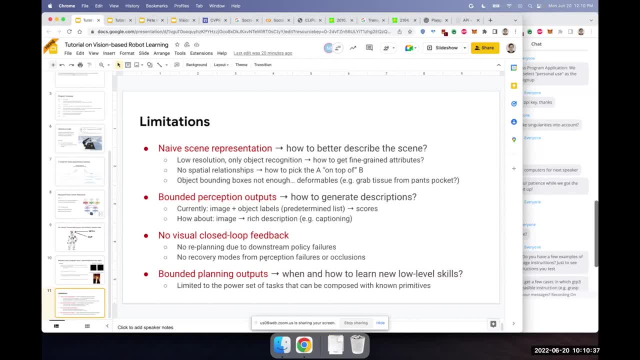 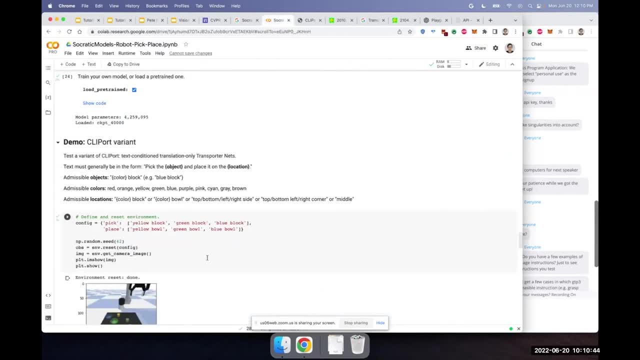 but all in all i just want to say that you know, it's very easy to take a deep breath and to think about how to kind of interweave the back and forth between the visual language model and the planner. are all very interesting problems to tackle. 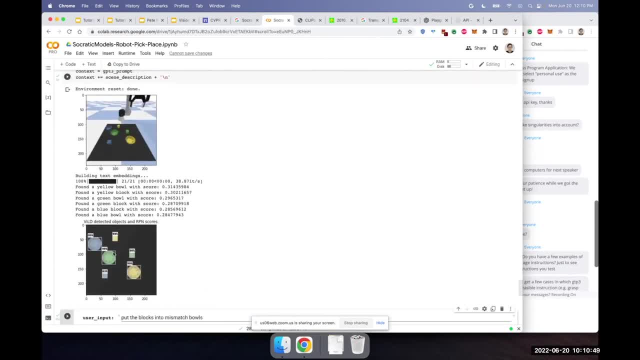 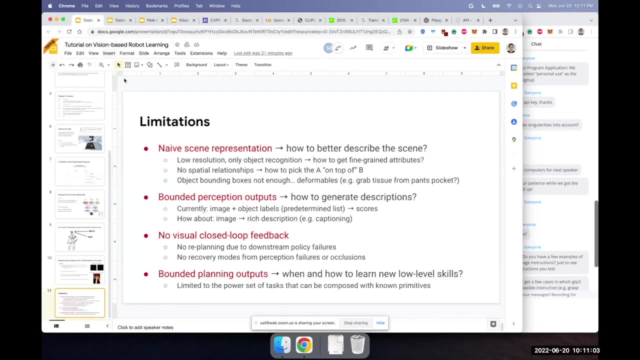 it detected the blue bowl and the green bowl, but it didn't detect the yellow bowl. So now the language model only knows that there exists these five objects, and if you task it to sort all of the blocks, it might not generate a plan that is correct. 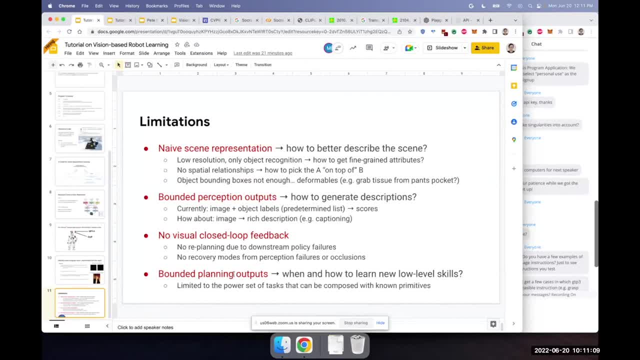 And the last point here is we have bounded planning outputs when and how to learn new low-level skills. So in the demo that we showed where it's taking in human feedback, it can only construct a plan based on the power set of all of the skills that it knows how to do. 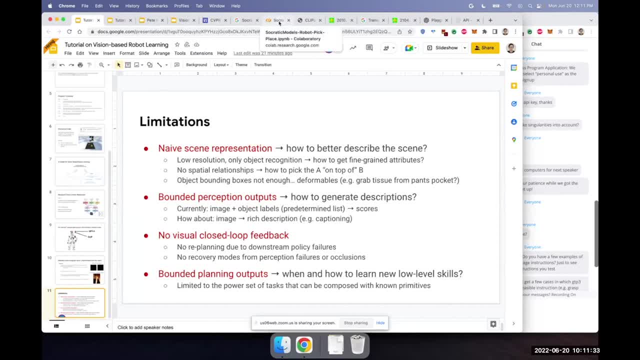 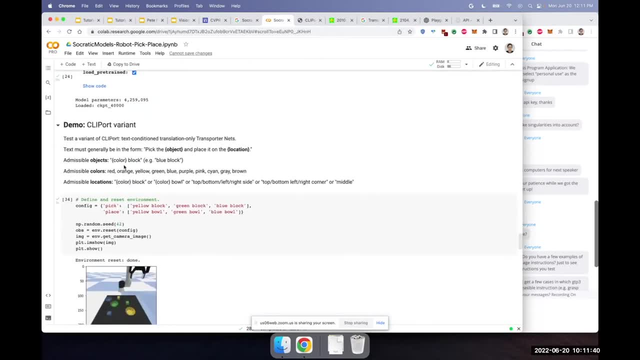 And this is the space of the skills in which we trained Clipboard to be able to execute. So back up here. if you're Clipboard, we've only trained it to be able to pick some particular color block. You can place it into a bowl, or also place it to the top, bottom, left, right side, or 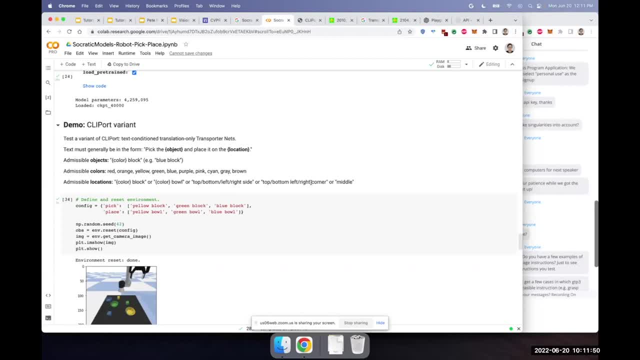 the top, bottom, left, right, corner or middle. If you ask it to do a task that requires training- it can place actions that are beyond these sets of actions- then the system won't be able to figure that out either. So, for example, if you ask it to construct a smiley face with all of the blocks, it may 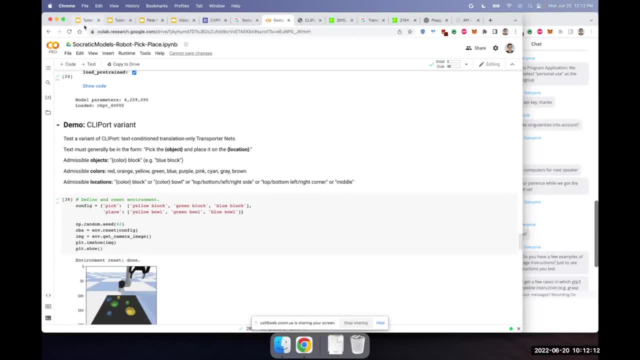 not be able to do that well, I think it'll fail miserably. So I think finding ways in which we can get these low-level skills to be more expressive, or at least including more low-level skills in general, and having a planner maybe also- 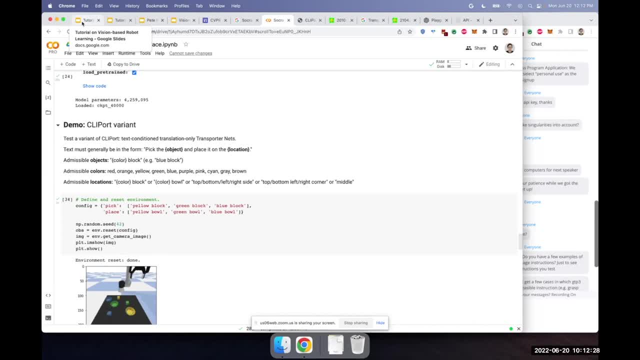 be able to say OK. if this high-level request generated me a list of steps and one of these steps is not inside the list of things that I know how to do, then I need to maybe train a new policy that can allow me to do that low-level skill on the fly. 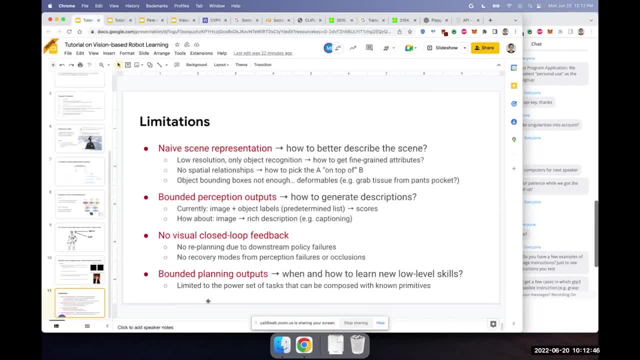 So there's really a question there which is how can we have the known primitives that we have trained to expand and be dynamic over time? So I think these are all just kind of different directions in which you can take this collab, and each one is sort of a very ripe research area. 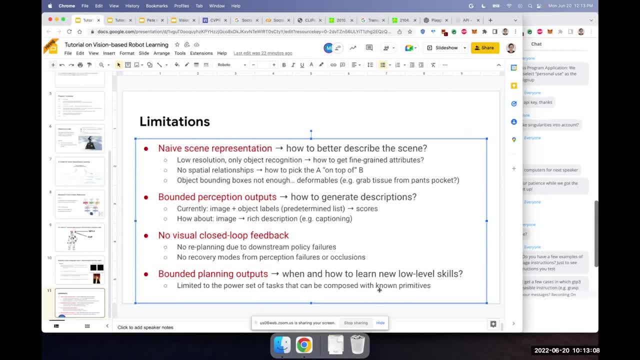 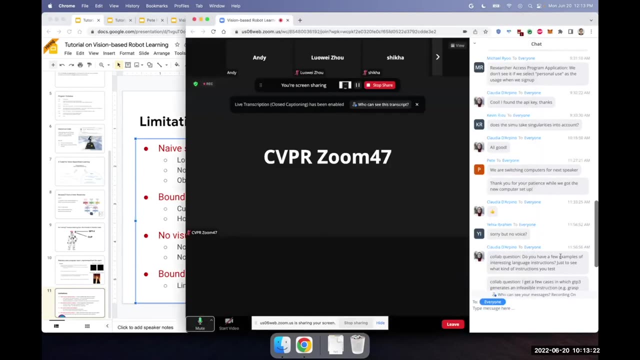 I think that it's all green fields, basically A lot of these things that if you tackle in the next couple months, it's definitely going to be new stuff. So, yeah, definitely worth thinking about. Well, any questions? There's one from Zoom. 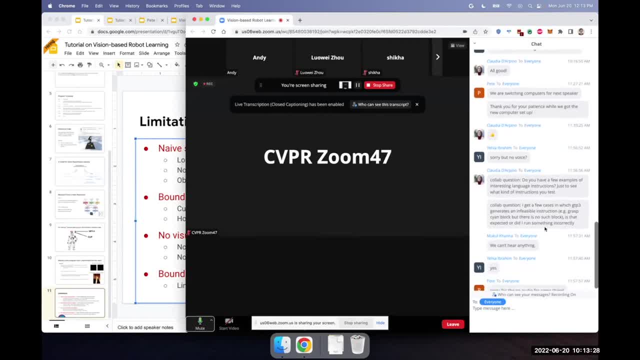 Do you have a few examples of interesting language instructions, just to see what kind of instructions you'd test? I think it was before you did some examples. Oh OK, All right, OK, The second one's a good question. I guess it's a good question. 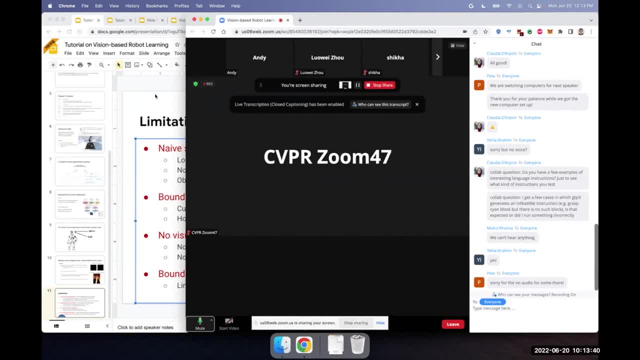 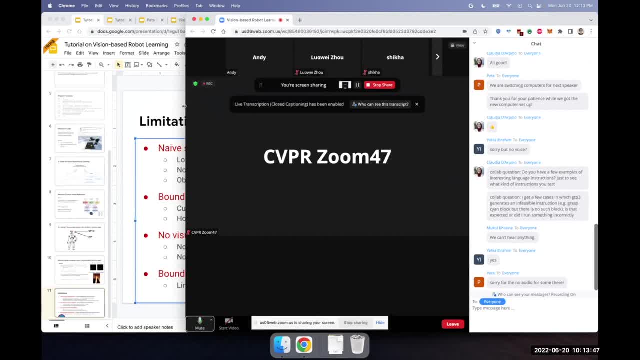 The second question says: I get a few cases in which GPT-3 generates an infeasible instruction ig grasp a scion block, but there is no such block. Is that expected or did I run something incorrectly? One thing to double-check is to ensure that you fit in the object description right before. 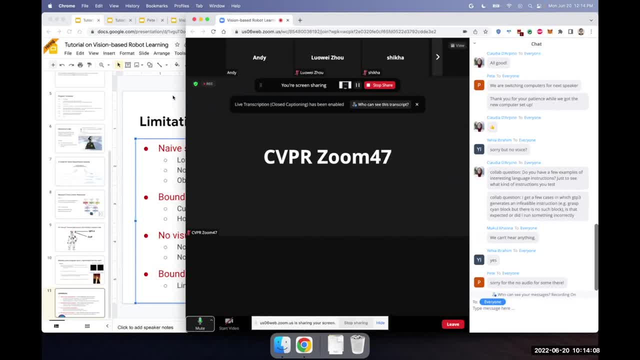 you asked it to generate the plans so that it knows what objects are available in the scene. It's possible that, for example, if you prompted it to do a new test, that it would be able to do a new test task. then it might be relying on the object list. that is far inside of its context and that would 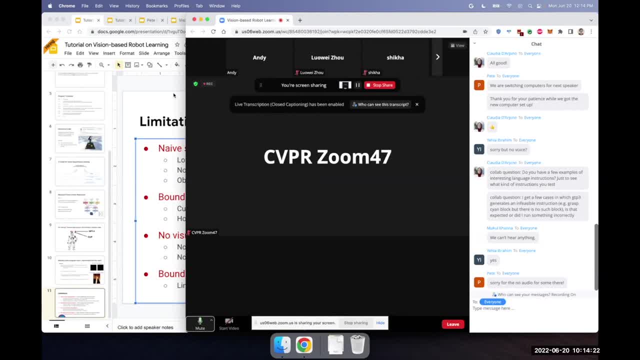 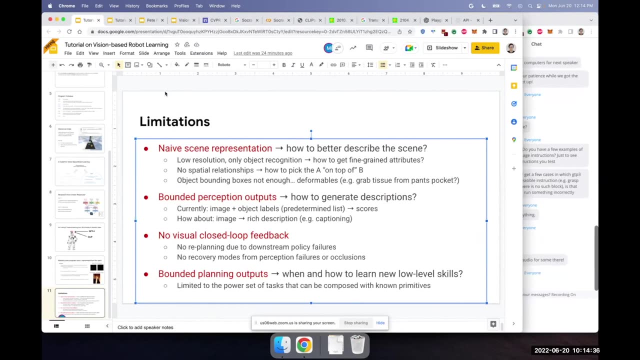 be no helpful at all. so updating that list of that same description is one way to fix that error. are there any other questions? um, yeah, the question was related to using language models for exploration. i think, uh, i, i think that's definitely a very exciting area, and in particular because these language models have 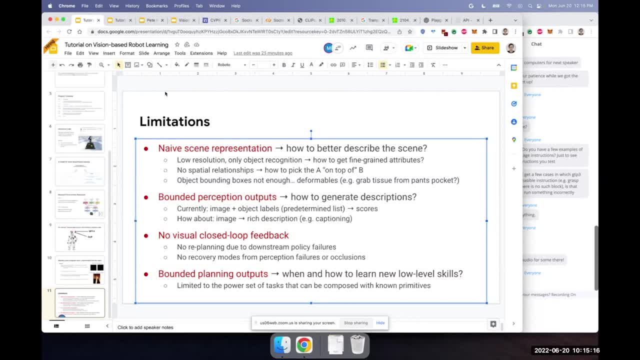 seen so much. they've read novels, and some of these novels have captured what indoor environments typically would have. you would have a kitchen, you have an oven, various objects inside of it, so leveraging that context as a way to potentially build, for example, a- uh, a graph of sorts. that's sort of storing, treating it as a knowledge base of what potentially could. 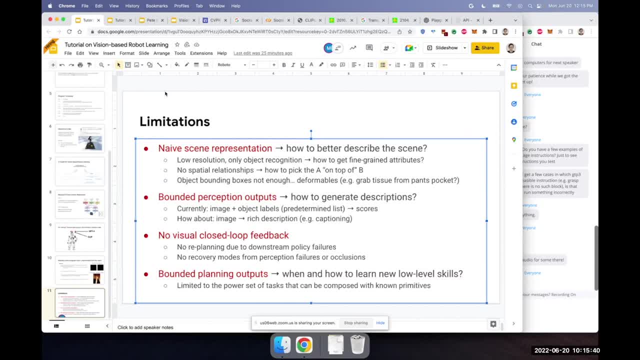 be inside of environment feels very promising, and then maybe having your robot sort of digest individual steps that iterate through that kind of representation might be very cool. that's just like a very specific thought, but i think in general anything that you do in this space could be very exciting. 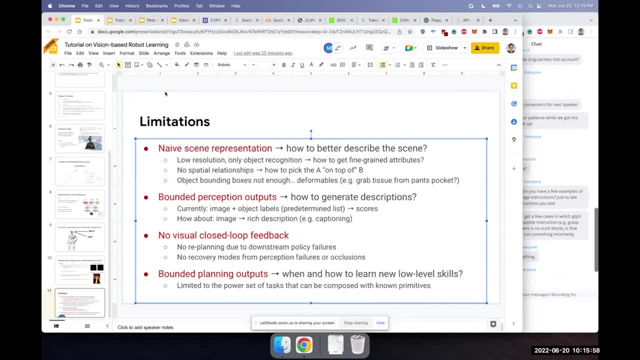 how would you? what would be the way you? yeah, and i i think that's a great question and ties into, potentially, representations of uncertainty. so when you're exploring and there's parts of the space in which you're more curious about than others, maybe there's a representation that is outside of the language model space. but 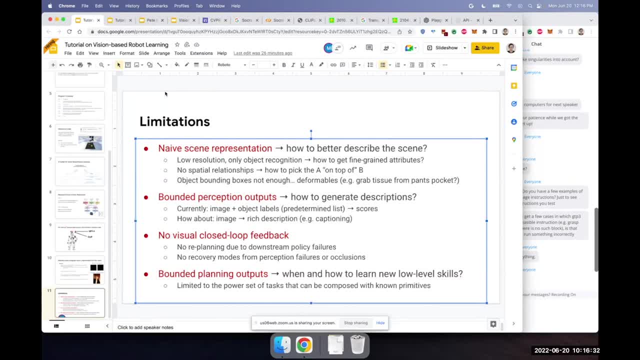 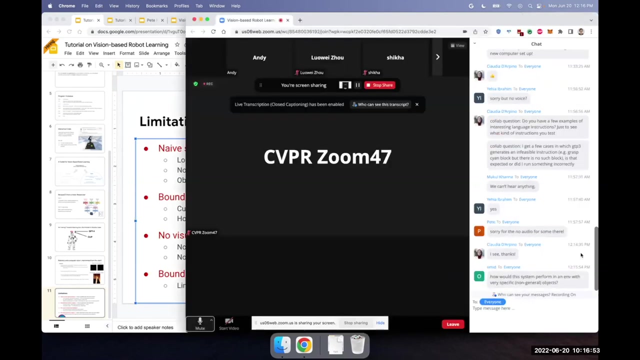 you have information, of storing what the robot is most curious about and then maybe finding a way in which the more that you traverse the most uncertain areas, the lower the uncertainty score, etc. um, so i i think that is, yeah, very interesting indeed. yeah, another question: how would this system perform in an end with very specific, non-general objects? 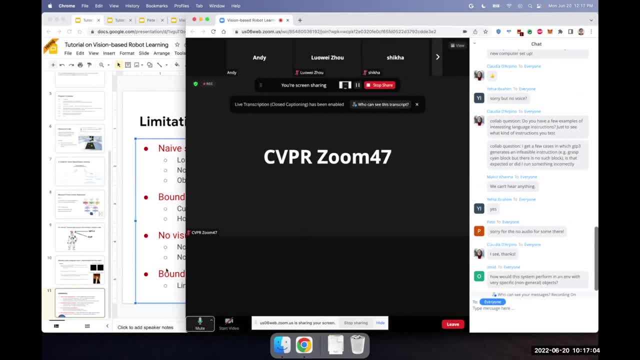 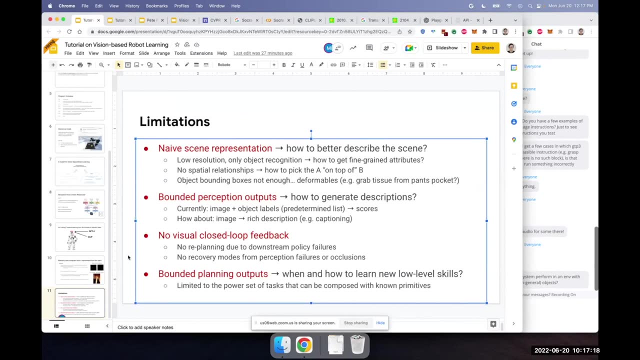 and how do you make it so that you can actually do a lot of work on it? um, i see so. um, specifically in industrial automation tasks, for example, if the object has a very particular geometry, um, i think one way in which you can make it work on those specific 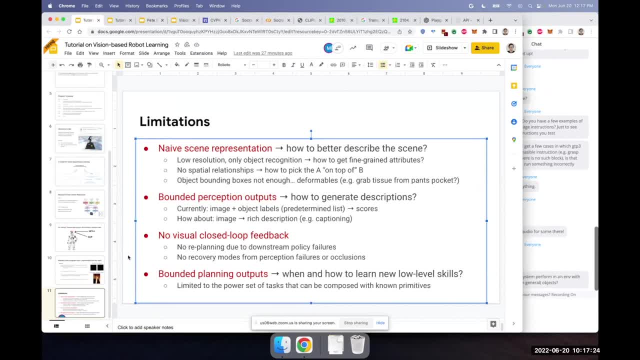 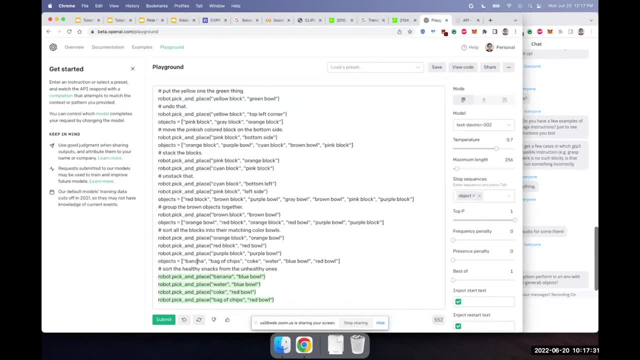 objects is to still have some way to id them or reference them. so, for example, um say that in the language model planner we replaced um the strings with ids, for example uh obj 345 and uh- obj 321, and then maybe the replicate that list: uh. replicate the string inside the list: multiple. 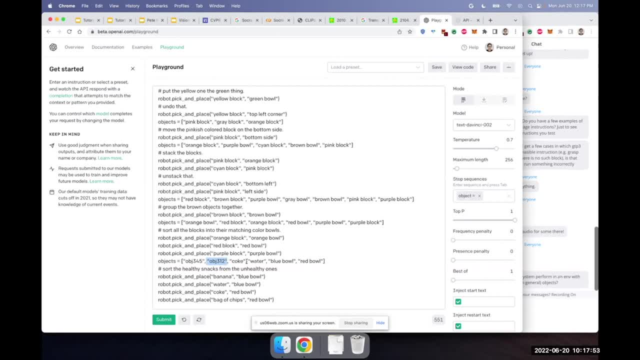 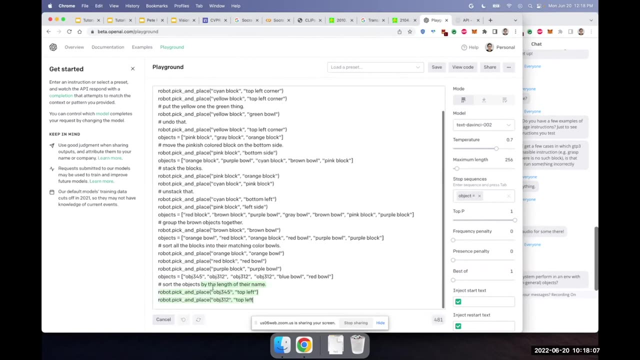 times in order to show how much frequency you have, and then just have it be able to. let's say that we have three of obj 321. then let's say that we have three of to by the length of their name. that's the objects. okay, not by the length of their name. um. 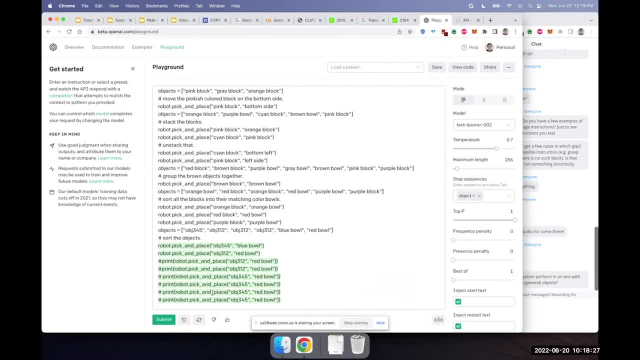 period. it's adding in uh comments, okay, uh, so I think maybe being creative about how you reference the objects. One thing that's interesting about language models is that you can try to formulate a a unclear problem in one domain into a clear problem in another domain. 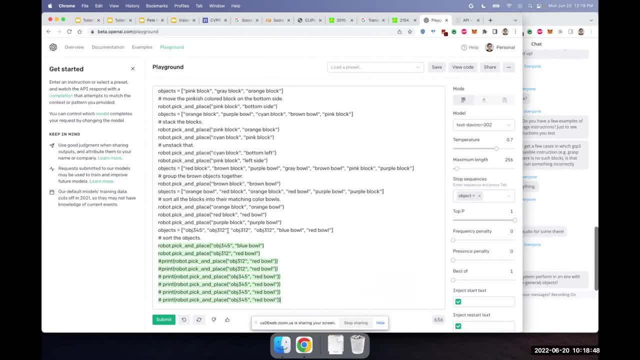 So what I mean is that if you, for example, gave one of your objects an alias red block and then you just had a dictionary that was sort of mapping that to the cat name or cat file, then you could potentially still have the system be able to benefit from the reason high level reasoning- of putting in general objects into each other but still being able to reference specific objects. 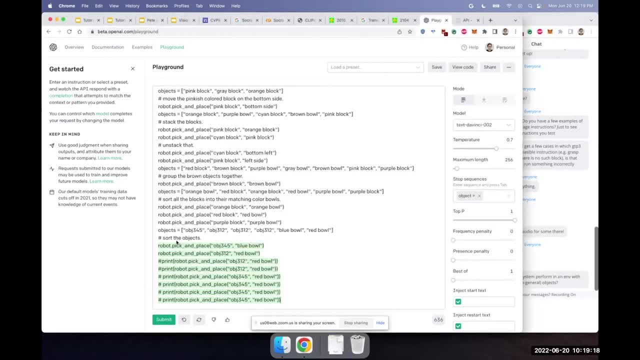 That's true. So Pete says you can also describe the object and language. So if you have particular Steve the bunny, you could, like describe everything that needs to know about the Steve the bunny. Yes, Yeah, you could. If there are objects that you want to work with and the attributes are relevant for how the robot should manipulate it, you can add in a bunch of different descriptions to it. 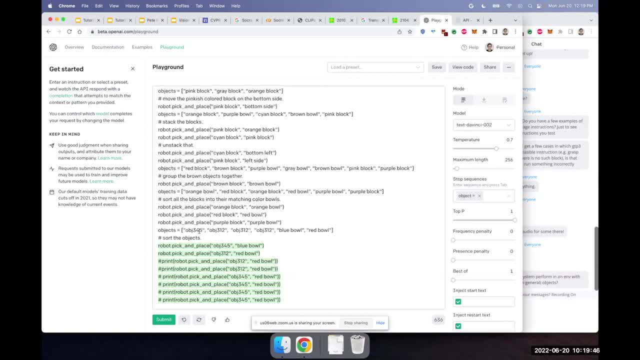 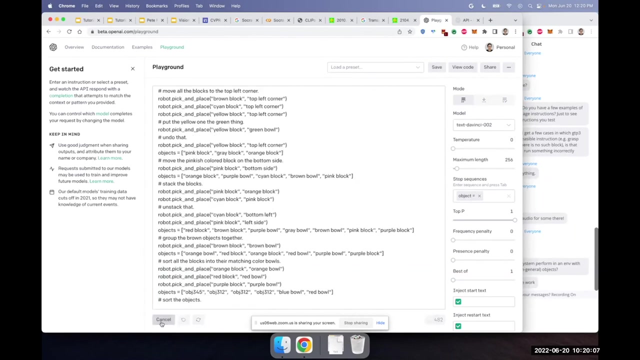 The example that he was mentioning is the Stanford bunny. You can have a description of everything that you know about the Stanford bunny being appended to information about that object. Oh, you know what? I think temperature term was responsible for these things. So what happens if we fix that? 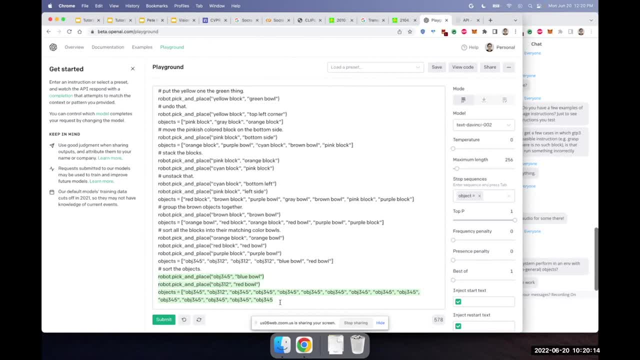 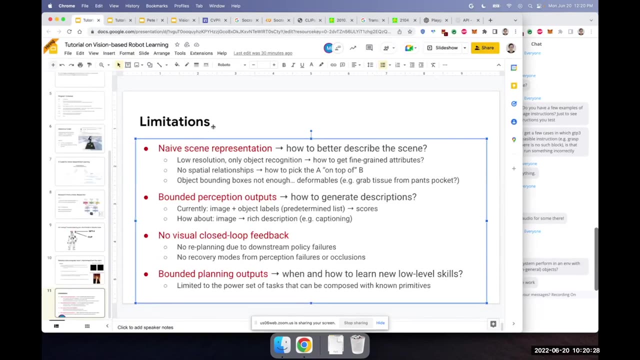 Okay, just kidding. Okay, so these things still require a little bit of prompt engineering and it's worth playing around with. Okay Cool. Any any other questions from the crowd? Yeah, Thanks, So Do you think the way the board is called this is the way that the model is designed? 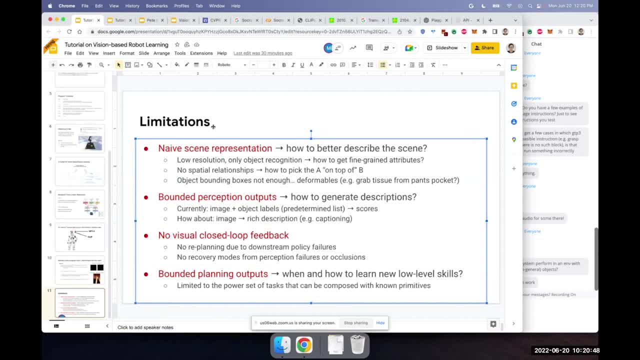 Is it just me training on the bigger, bigger scale, or is a complex That's getting into work? Yeah, I think, in order to at least tackle some of the specific problems that we've shown today, one very easy fix is just through adding the examples. few shot front two: 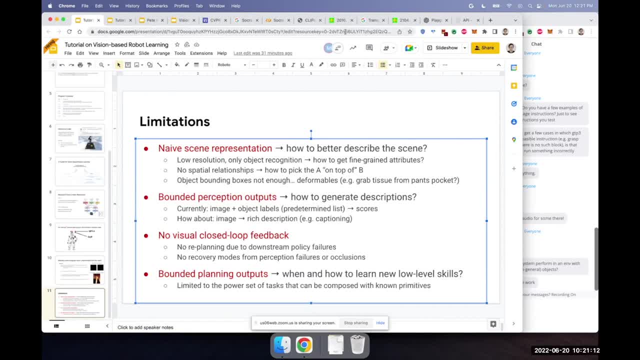 So adding in several examples of the tasks in the mode that you expect it to be in inside of it. Yes, I can't explain everything Very much. Yeah, I think it's just as you said. there's like a lot of things that you can do to help. 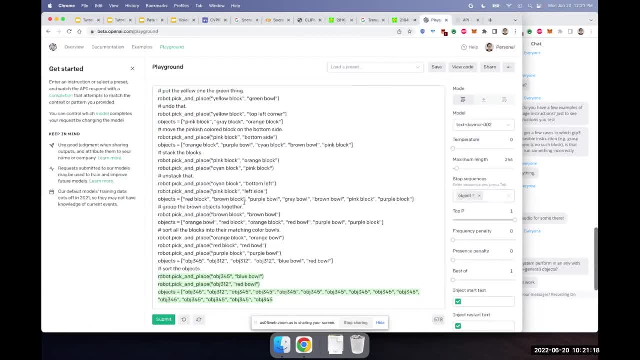 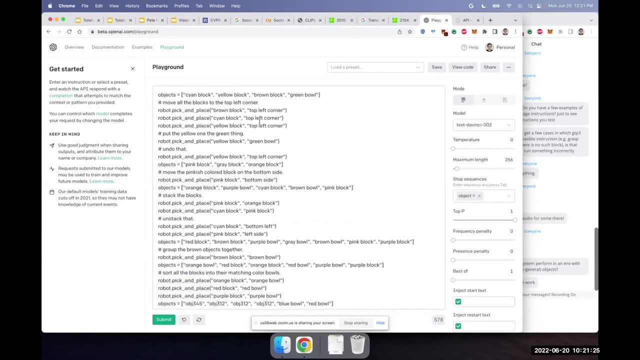 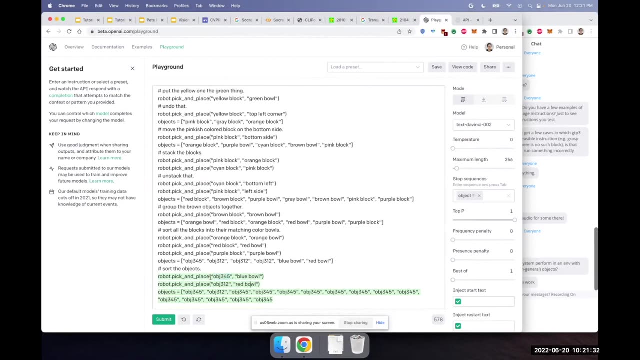 of the text prompt. So one potential failure case for why this happened is because up above we've been using yellow blocks and holes all the time as examples for a few shot context. But say that you started copy pasting some of these examples into the prompt as well. then you might be able. 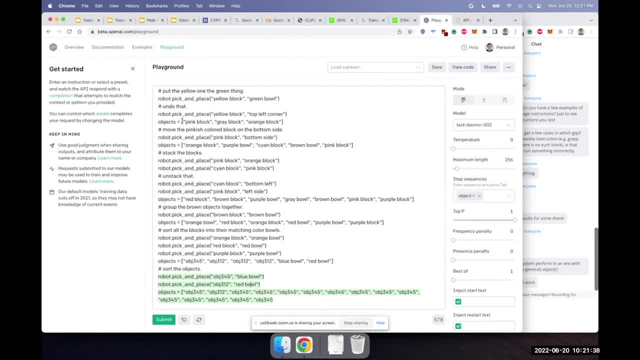 to get the system to get better performance. So that's one way to immediately use the existing models that we have. I do think that at least we've seen a couple newer language models, including Palm from Google. that shows that as you scale these models, they also tend to become more.